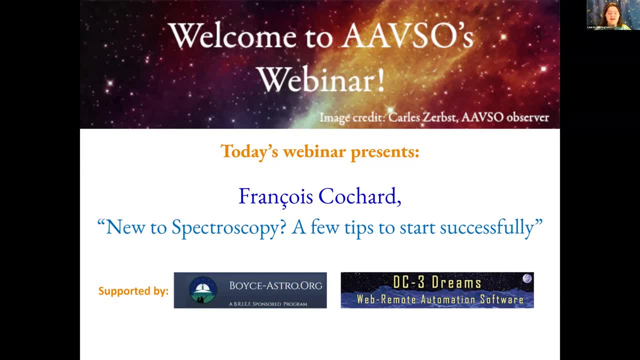 about 99% of the sky. The Boyce Research Initiative and Education Foundation provides online astronomy education, observatory resources and research experiences to students, student teams and schools. In order to learn how to do this, you need to know how to do it. 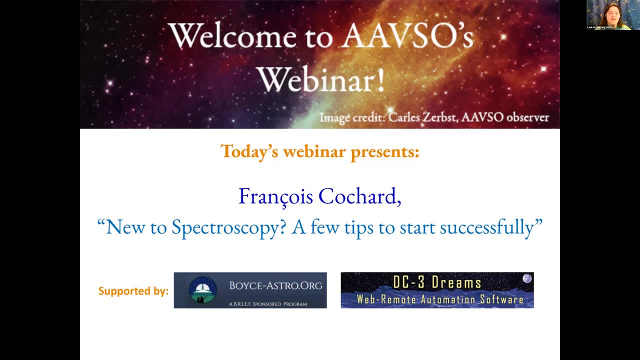 You need to perform observations, conduct research and publish their results in scientific journals such as the Journal of the AAVSO. Please check out their webpage to learn more about their work. Okay, on to the good stuff. Our speaker for today is Francois Cochard, who is an expert. 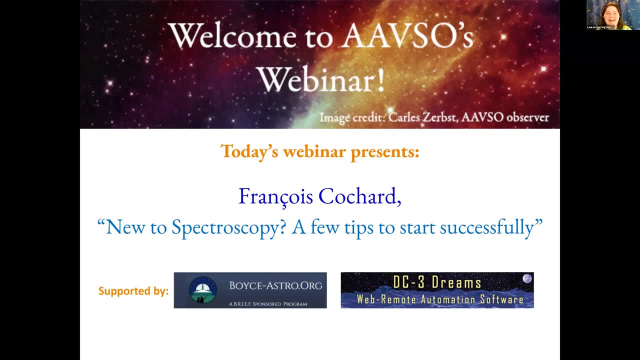 amateur spectroscopist that you will probably recognize. Francois has been deeply involved in spectroscopic education for years and has taught at dozens of educational events, including several programs. His list of accomplishments is long. He's the organizer of the annual OHP Spectro Star Party in. 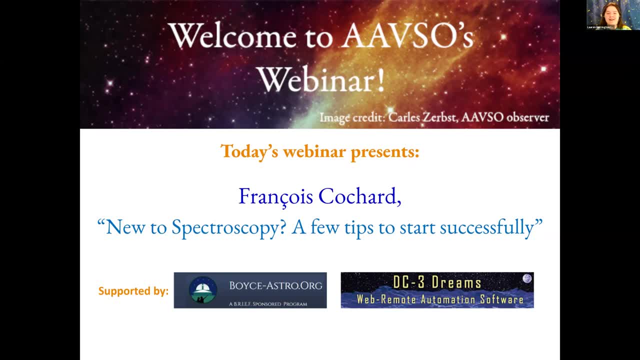 France, the author of the book Successfully Starting in Astronomical Spectroscopy: a Practical Guide, and the co-founder of Cheliac Instruments, where he produces many of the standard spectrographs which are in use by amateurs today. In short, Francois is an expert not only when it comes to 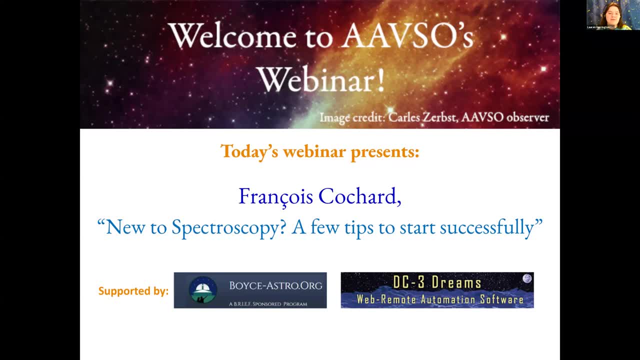 spectroscopy, but also in the field of spectroscopy. He's also an expert in the field of spectroscopy, but also when it comes to teaching people about spectroscopy, which is why we are all very lucky to have the chance to learn from him today. Ladies and gentlemen, I give you Francois Cochard. 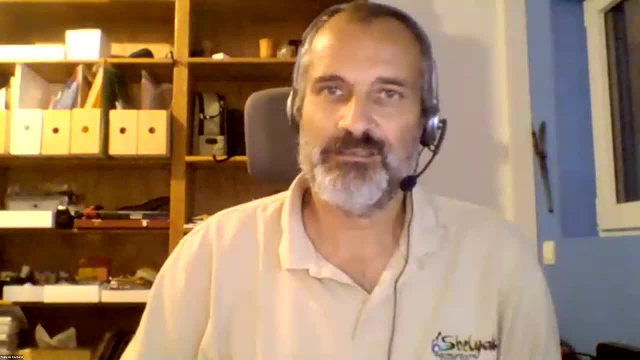 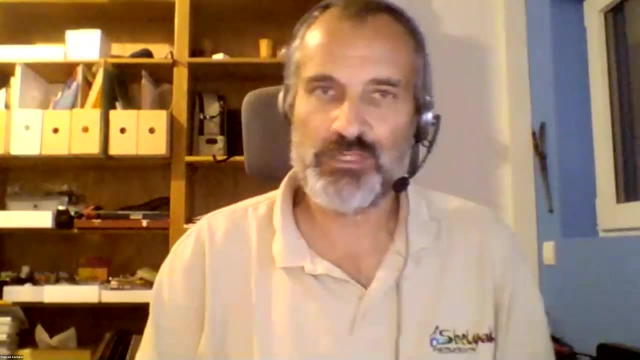 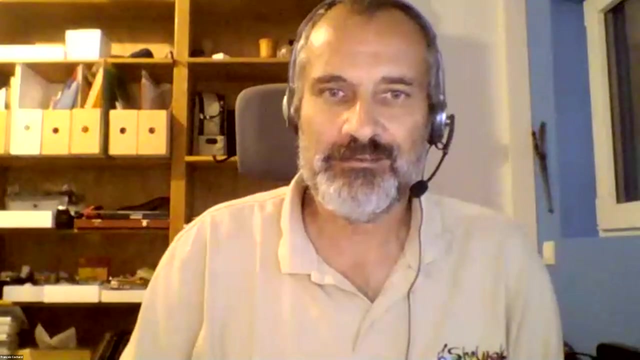 Hello to everybody. Thank you so much, Lauren. Thank you for your impressive presentation. So now I do have the pressure on me. Thank you so much. Hello to everybody. I will share my screen to show the slides I will work with. I hope that you can. 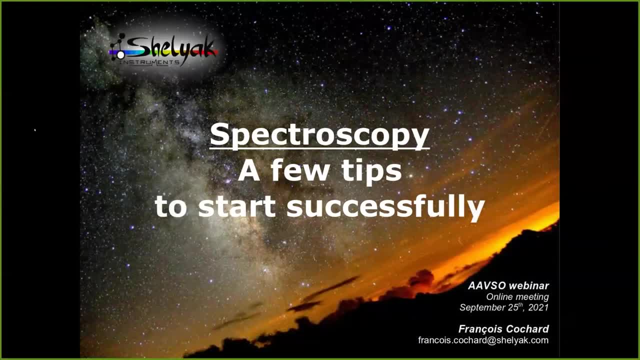 see my screen now. Perfect, Thank you, And this is really a great pleasure to talk to you. When I see the list of the names, I know a few of you, but not a lot of them in fact, So I think most of you are really beginners. 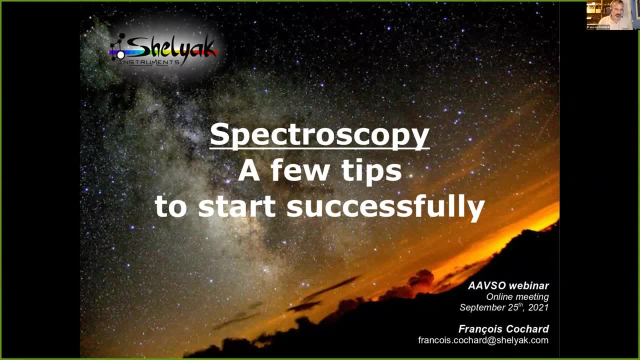 which is a great good thing, great news, because it means that more and more people are jumping into spectroscopy. and and then the idea for me is really to talk about you as beginners tonight, well, tonight in france, today for you, and, and so i will not talk about the spectroscopy itself, but i, i think, i consider that you, you are. 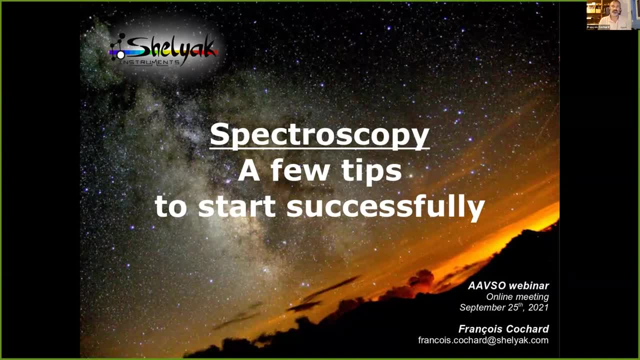 interested to do spectroscopy by yourself and you don't know exactly how to start with, or you have some ideas, but you would like to have some advice and and then i will give you this advice to to start. okay, so what? um, what i will talk about, if it's okay for you. i will have a quick introduction. 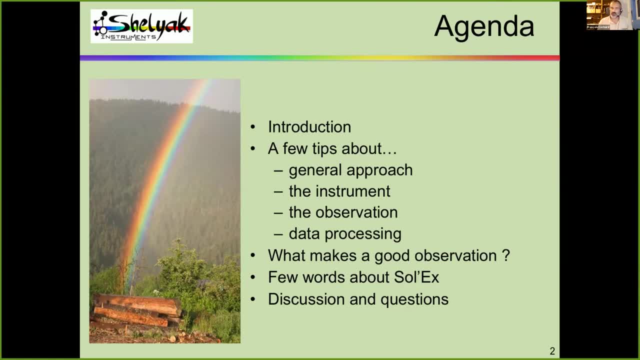 i will give you a few tips about the general approach when you are doing spectroscopy, about the instruments, about the observation and, of course, about data processing. okay, and then we'll see very quickly what makes a good observation. and this is very basic, in fact. and i will also give you a few words about the 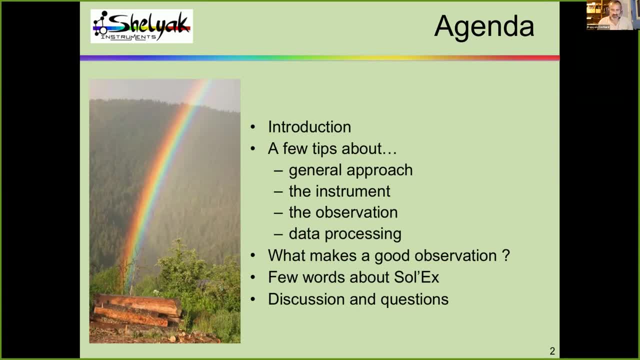 solex project, which is a a new instruments proposed by christian real, and this is something which is very amazing, i think, and it which is a wonderful instrument to start with in spectroscopy. and, of course, we'll finish by uh, the discussion and you, you can, it will be really a pleasure for. 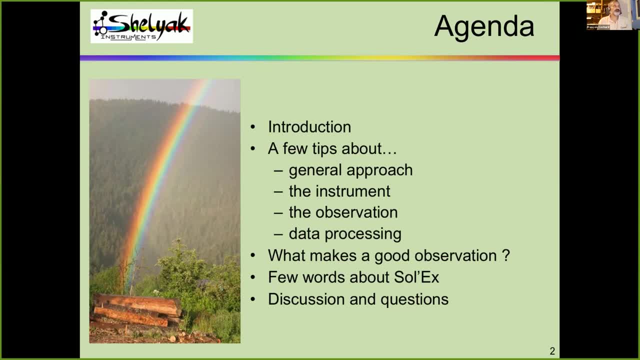 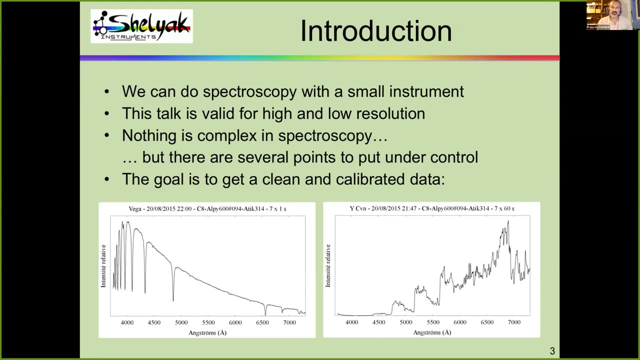 me to reply to all your questions, um, and well, i hope it's okay for for you. so i start with that, and the first thing that i want to tell you is that we can really start in spectroscopy with a small instrument, so there is no need for a big telescope. 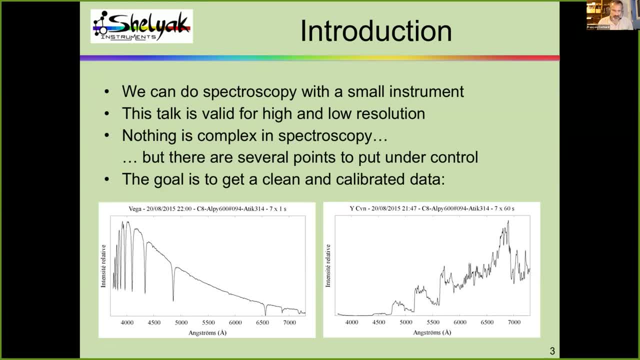 big setup, dome and so on, so you can start with a simple instrument, and this is something very important for me and, in fact, very amazing. so the, the quality of your data doesn't depends on the doesn't depend on the quality, on the size of your instrument. okay, the, the quality of your data. 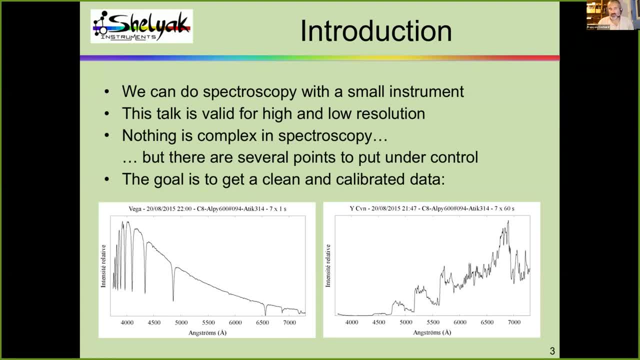 will depend on the way you are managing your observation, but you can do that with a small instrument. of course you will not have the same result with a small instrument, but you can do that same result with a small and a big instrument. there is a real interest to have a big telescope. 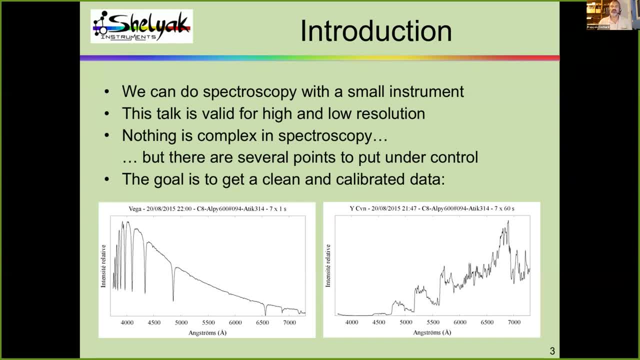 to go for fainter, fainter targets, but the quality: you can have a very high quality observation with a small instrument, okay. so also something important for me is this talk is valid for high resolution as well as for low resolution. you know that when we are doing spectroscopy, 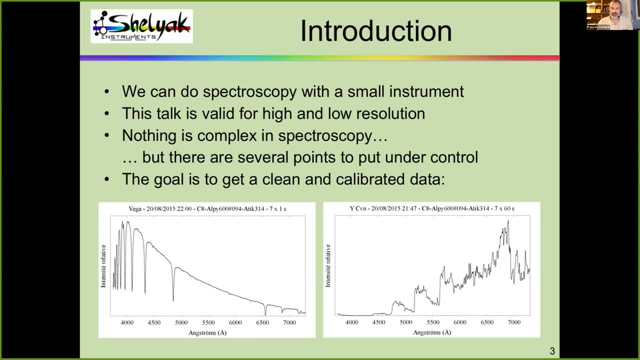 we can have low or high resolution observations. so when we are doing low resolution, we have a wide bandwidth covered by the spectrum. we can observe the whole visible spectrum in a single shot and when, when we are doing high resolution spectroscopy, we just focus and we zoom, in fact, in. 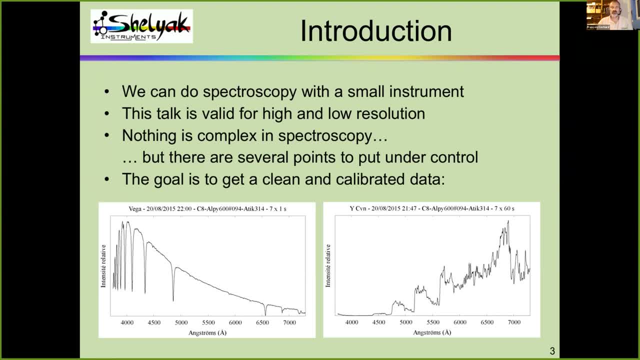 a small part of the spectrum and then we see much more details, for example in the, the line profile of a specific line profile. but both are quite different, but although what i will tell you tonight, today, is really valid for both of them. okay, the the something else which is a key. 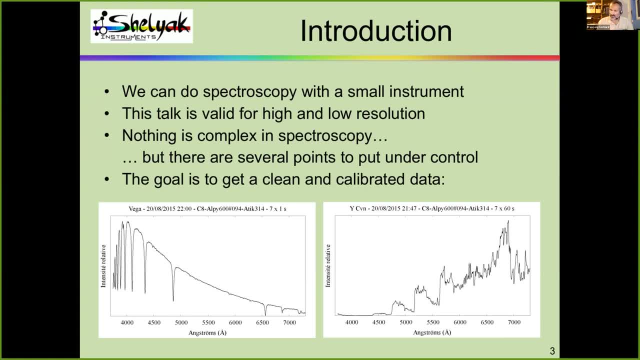 for me today. this is to tell you- this is very important for me- when we are doing spectroscopy, we are doing where we are doing, simple things. okay, spectroscopy is really simple. there is one thing which is a little bit complex, which is that we have to to put under control several points, or maybe a lot of points. okay, 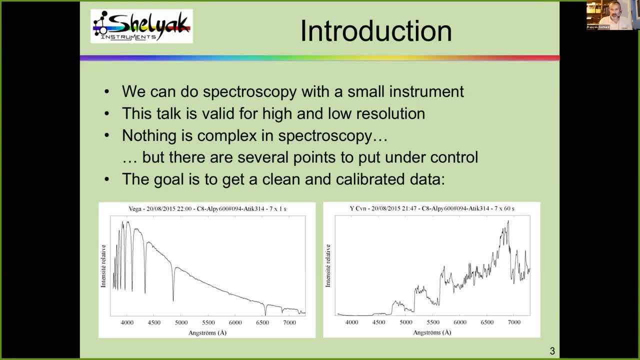 and we will cover most of them, but each point is very easy to manage. okay, so we are not doing, i mean, when we are doing astronomic observations in spectroscopy, we are not doing astrophysics- that can be quite complex. we are not doing quantics, mechanics, which is, for sure, quite complex. 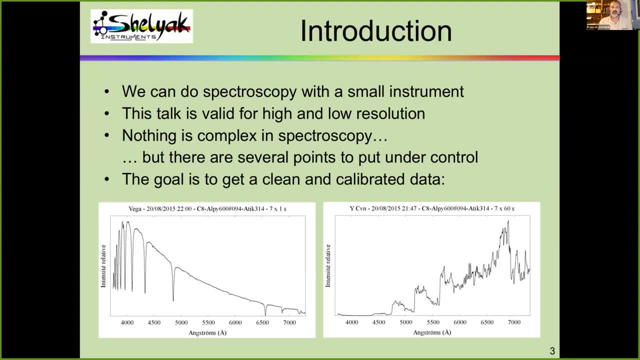 but taking spectra is something in fact very basic. but we have to put a lot of things under control. and of course, if we, if in spectroscopy observation depends on, say, 10 different parameters, if each parameters is not really under control, so for sure at the end the observation will fail okay. so we must be very- uh, methodic. 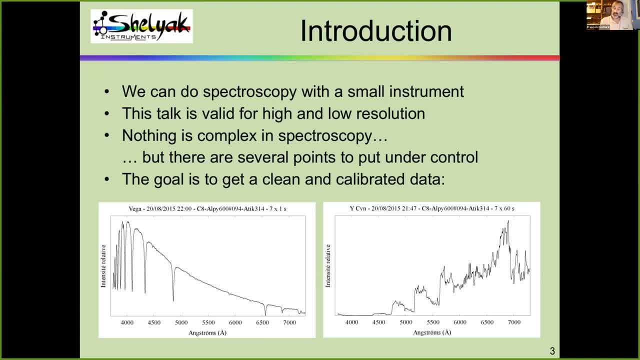 and and put every uh point under control, and the idea is really to to put them under control step one by one, okay, and it's much better to not try to put to control them all at the same time, okay. another important point is when we are doing spectroscopy, the goal of the observation is to get a clean and calibrating 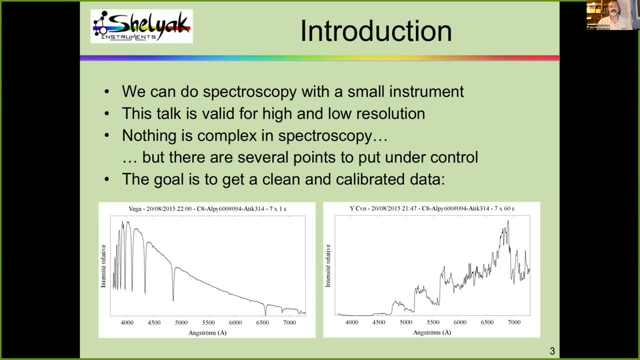 calibrated data. okay, the idea is to have. i would say i don't want make you afraid, but we have to have a scientific result. okay, again, it can be a simple scientific result. so don't be afraid, please, but the we, the result, is something that i have in the screen here, so i hope that you can see my mouse on the screen. 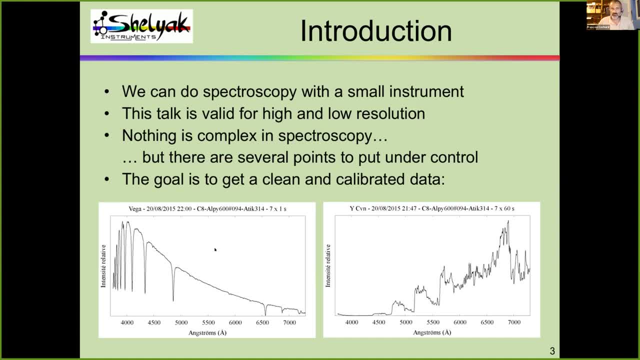 and these are, for instance, two, two different spectra, one from vega and one for ycvn, which is a carbon star, and taken with the same instruments, in same conditions. and of course, we can see the difference between the, the different observations. the idea is really so. this is the result of an 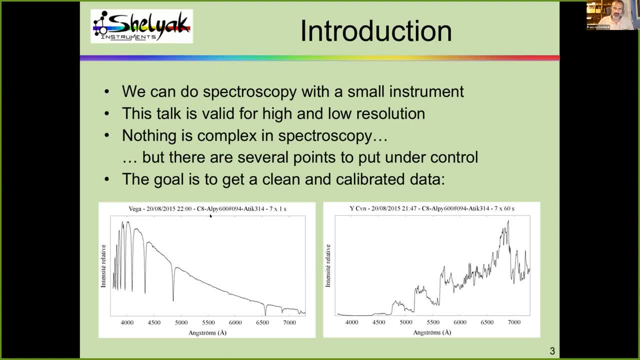 observation. so you have a spectral spectrum profile which is corrected from all the instrument, not instrumental effect, okay, and which is properly calibrated in flux and in wavelength- okay. so this is the result. so keep in mind that doing spectroscopy is not only um taking images on the telescope, but it's also to to to go up to the final result, which is 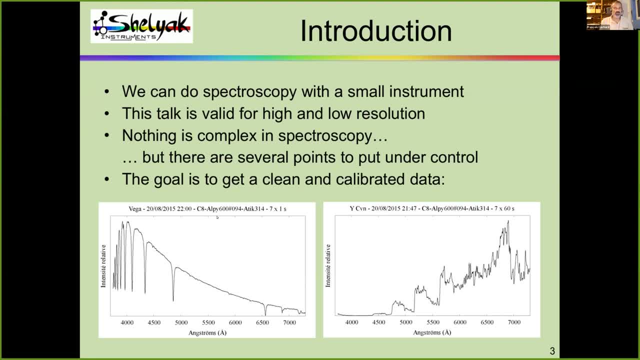 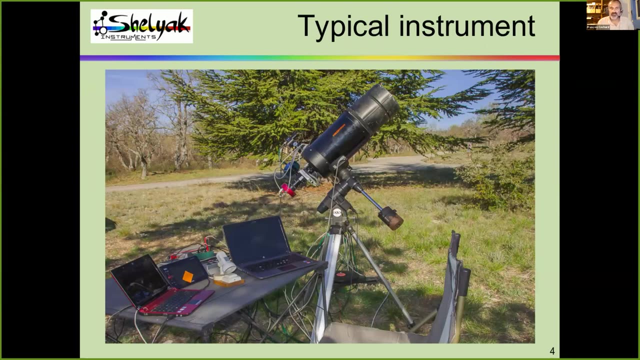 this calibrated profile. okay, um, when i'm preparing, uh, this talk, this presentation, i do have in mind this kind of instrument. well, this is my old telescope, my previous telescope. have a new one now, but it's not really bigger than that, so i have a better mount. but the idea 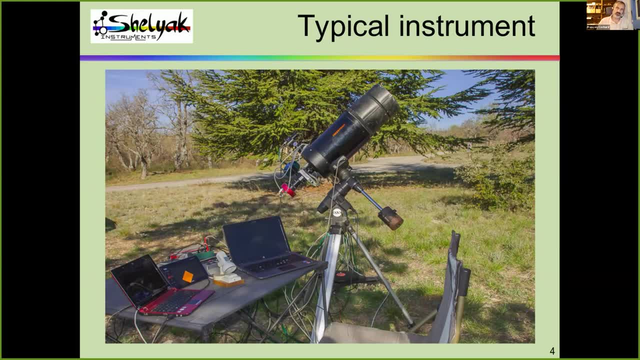 is the same and this is on the picture. so it was taken at the ohp, so at the observatory of the old province, a few years ago. and this is really. this is a c8, you know, on an old mount and you can see, here there is an lp. you can see the lp, the calibration module, you can see the. 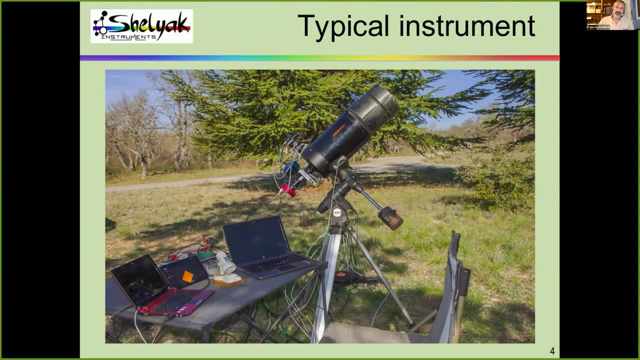 acquisition camera and the guiding camera and the, the. i do have two computers, um, well, i did have at this moment two computers, which is better, because one is controlling the uh, the, the telescope, and the other one is controlling the acquisition. and just a small detail about that, uh, it's, it's more comfortable to have. 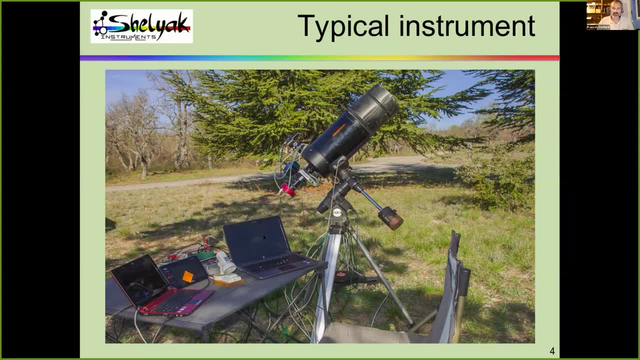 two different computers because you have more screen surface and more information at the same time, but really there is absolutely no need to have several computers. uh, regarding the, the, the, the computing power of the computer, all the software that we are using during the acquisition and the data reduction can be done with a single computer with no problem. 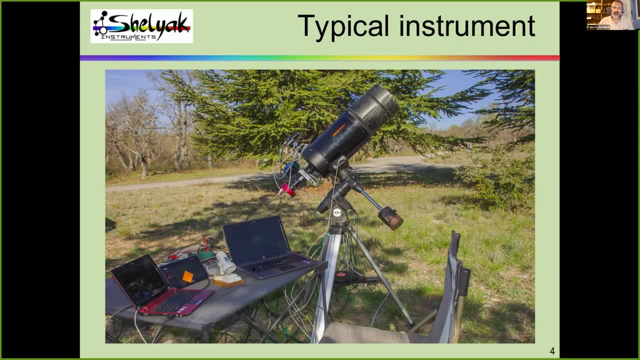 but this is just, uh, the advantage of uh having uh, uh, different, uh way to control the different elements, and we have a better control. okay, so again, i'm not talking about big instruments. even, of course, if you have a big instrument, if you are lucky, you have to have a. 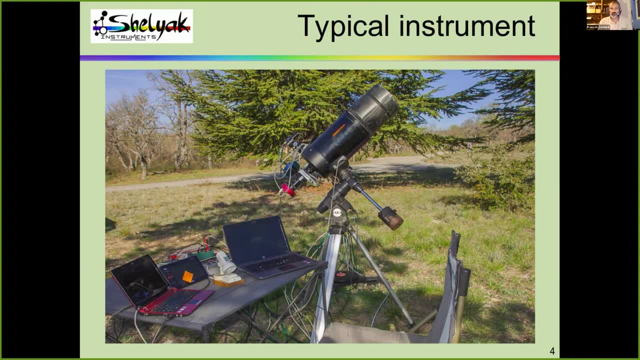 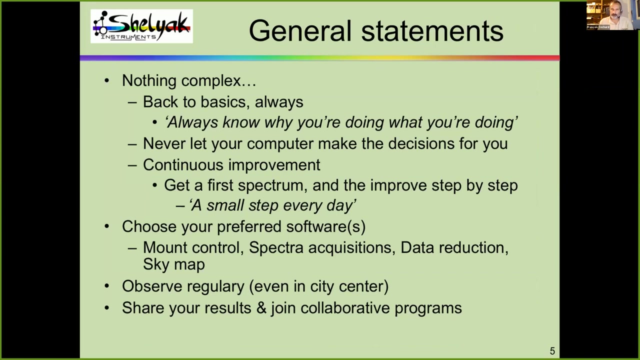 big instruments. all the recommendations will be also absolutely valid and and the idea will be exactly the same, but, generally speaking, it will be easier to start with a small instrument, now one. when i start with some general statements about spectroscopy, i told you that nothing is complex when doing spectroscopy, but we have to put several points under control. 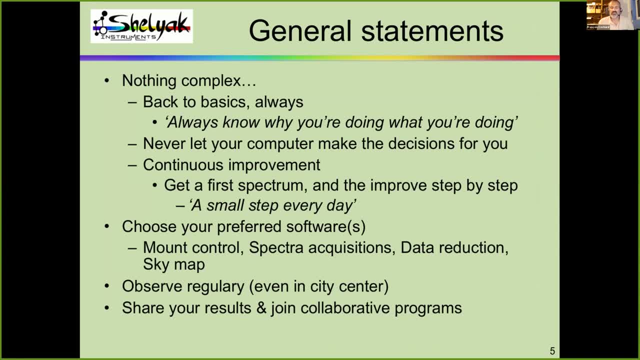 knowing that i think it's important to start with these kind of recommendations. please go back to basics always. this is a a sentence from steve shaw that i love. he told us a few years ago: well, always know why you are doing what you are doing. i like this. i like this because, well, this is. 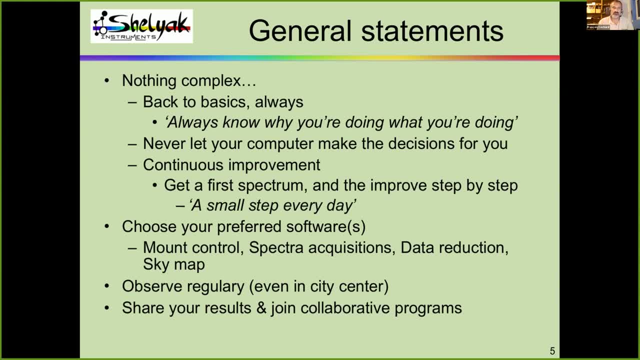 obvious. of course, when you are doing an observation, it's so. of course we are doing. we are going back to basics. the problem is that when you are in the middle of the night, when it is two or three o'clock in the morning, uh, you probably know that we don't think the same way. 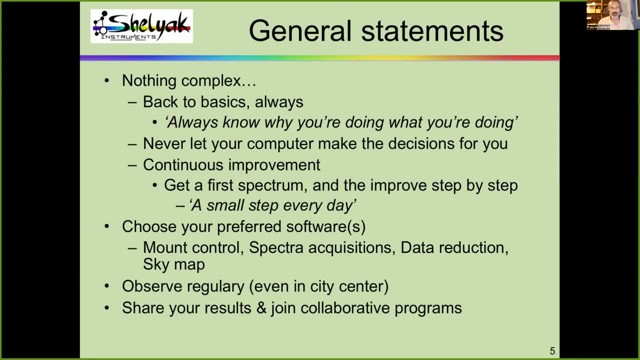 and and we we are maybe less clever than during the the day, and it's it's very important to say okay, so if something is happening during my observation, please keep in mind that things are simple and the astronomy is something very rational. okay, and and let's try to to keep things simple and take some time to to to understand what is. 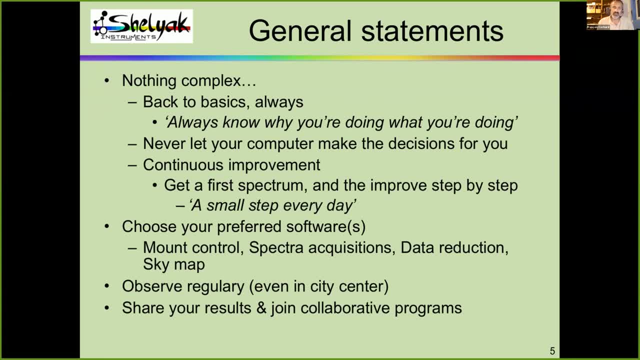 happening. okay, this is the same idea. never let the computer make the decision for you. uh, it's, it's so, you are the boss. this is not the computer or the software, or the acquisition software or the data reduction software which is the boss. you are the boss, and then the computer is here to make. 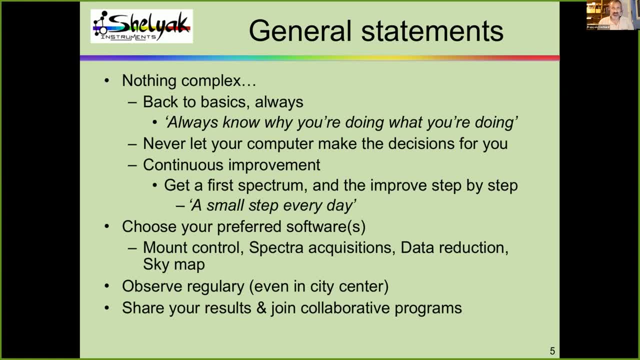 what you have decided to do. this is basic. this is even stupid and i'm sorry for that, but really this is something important. i know that in the middle of the night, we may have some strange behavior and and then this is a pity- also something which is 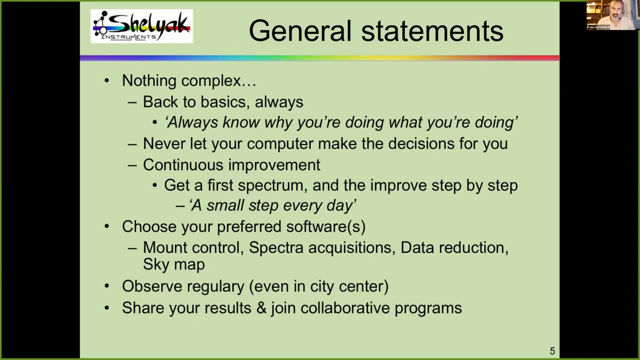 important for me. i love the the continuous improvement approach, so it means that the the idea is: do your best to have a first spectrum, even if it is a poor observation, but try to have a first spectrum and then improve it step by step. and look at your data. you get your results. 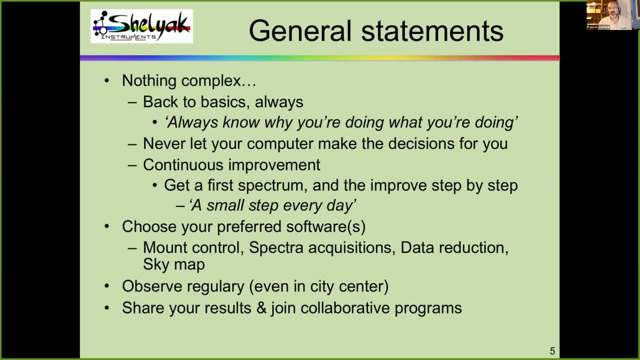 and say, hey, what can i improve? uh, to, to, to have a better observation for the next. uh, next time, and this is very important, to have this approach, a small step every day. so, in this mindset again, do your best to have a first observation as soon as possible, as fast as possible. 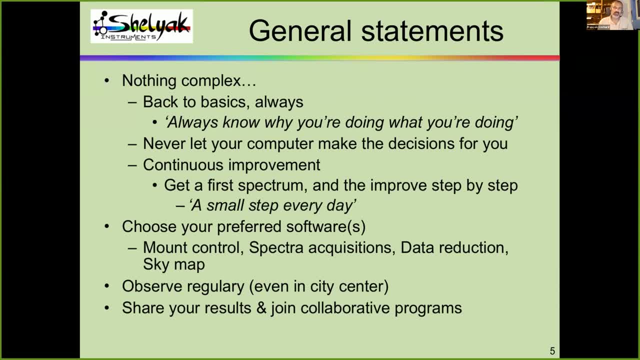 even if it is not good. but do that and then look at your data. you get the result and say okay. so now i've done this first observation, what can i improve? redo it several times and then compare the results. are they always the same or are they? 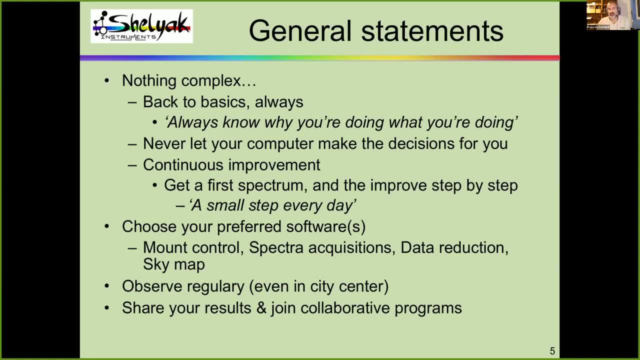 different. what did you change to to to change the result. is it an improvement or is it worse than before? okay, so this is a a general approach which is very important when doing spectroscopy. of course, it can be applied for many, many other areas, general astronomy, or even elsewhere, of course. 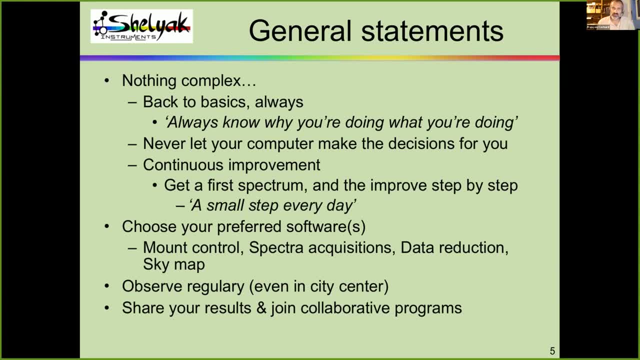 uh, you have to choose your preferred software. we have to use different software. generally speaking, you have, you need one software to control your mount. and control your mount means going to you to the target, but also guiding or auto guiding the mount and to make sure that you you put the, the star in the slit of the spectroscope. 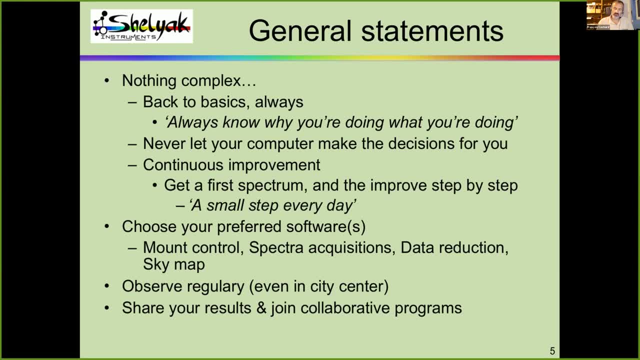 uh, you need a spec. um, so sorry. you need a software to do the spectra acquisition. you need another piece of software to do the data reduction and, finally, you you usually need a sky map to know where you are looking at and to control that you are looking at the right star. 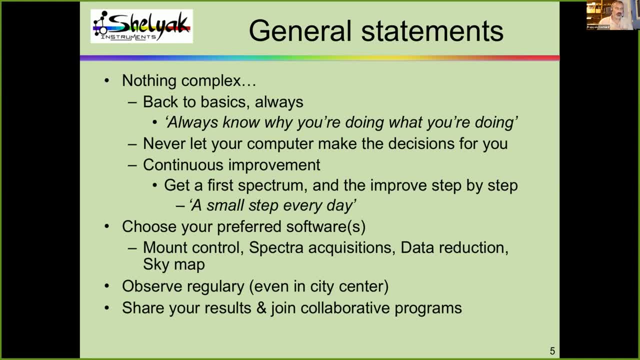 well, by the way, i can promise that even the most experienced people i know have already made a mistake to shoot to, to observe the wrong star. so well, i will not give you some names, but i can tell you that everybody has made a mistake at least one day to say okay, so i want to point a point at this time and finally, this is just the. 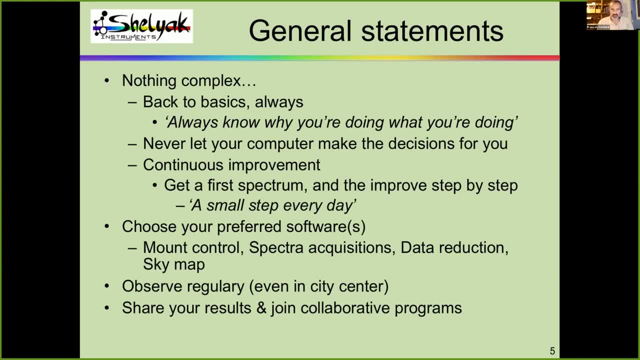 the star behind beside. okay, so don't be afraid, this is something quite normal, but also put this under control. so make sure that you you have some ways, some tools to make sure that you are observing the right star. uh, something else which is very important when doing spectroscopy: 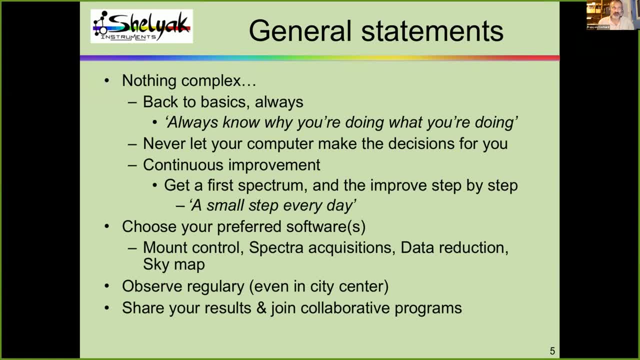 is: uh, do your best to observe regularly. uh, this important. i know that, um, we have people coming at the uhp every year and and some of them uh come every year, every year, saying, uh well, i didn't have the time to observe during the year, and if you do that only once a year, i can. 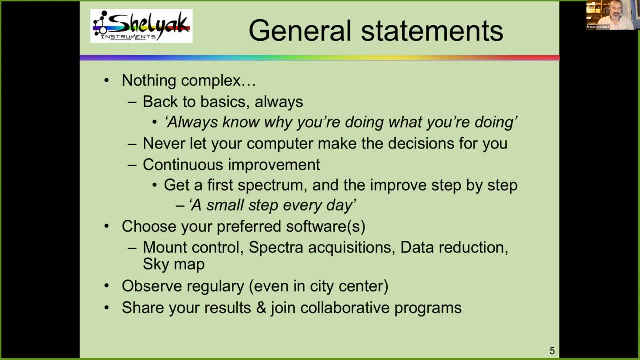 promise that it will be very, very difficult to do some progress, because from one day to one year, to the other, to the next one, you, you will forget, uh, all you have learned. so it's important to do regular observation. the good news, the good news which is very important, is that 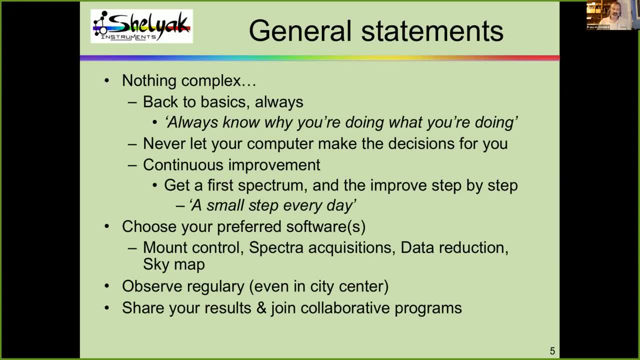 you can do spectroscopy even in city center, even at home, um, personally. uh, well, now i do have a home garden, so i'm in good conditions. uh, but the? um? for a long time i was in a flat in city center and my, my instrument, my telescope and spectroscope, was on the balcony and i just saw a small part of 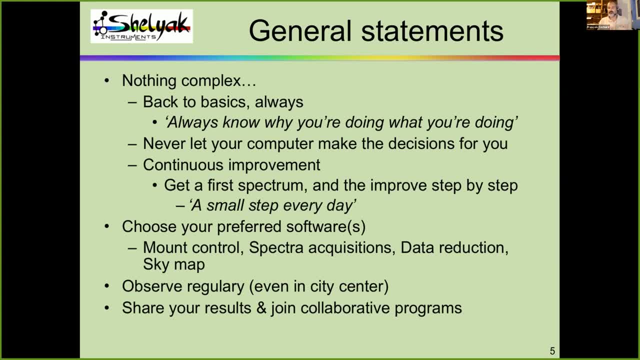 the sky, but it was enough to do some tunings. and how to play with the software, make sure that the connection with the camera is okay, how to select the parameters for the auto guiding and so on. all these things can be done even with a poor sky. so it's it's something which is very important. so 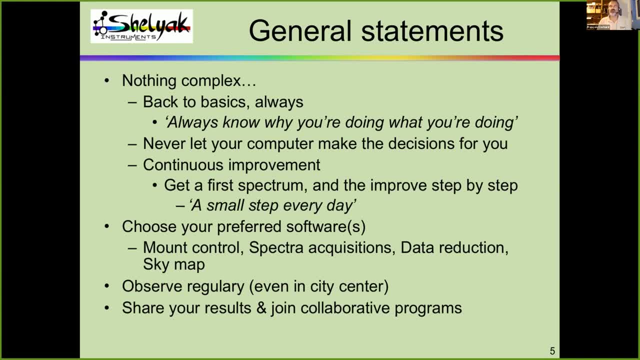 when doing spectroscopy, you don't necessarily need to have a wonderful sky, like it is usually when you are doing great pictures. okay, so it's an important point: observe regularly and and do some capitalization of your experience and again improve step by step by observing regularly. 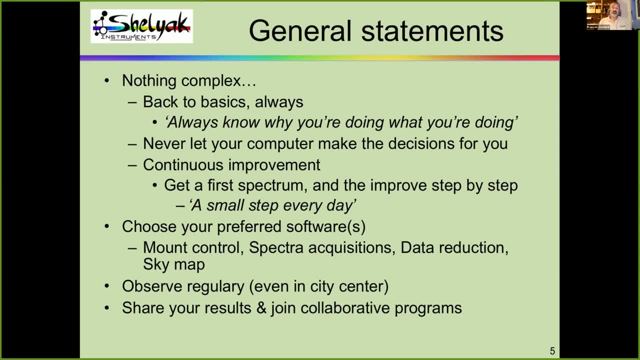 and a very good way to have to make great progress is really to share your results and to- why not? to join collaborative programs. i know that when you are a beginner, you you often think that's okay. so you, you are beginner, so you are not an experienced guy, experienced guy. so 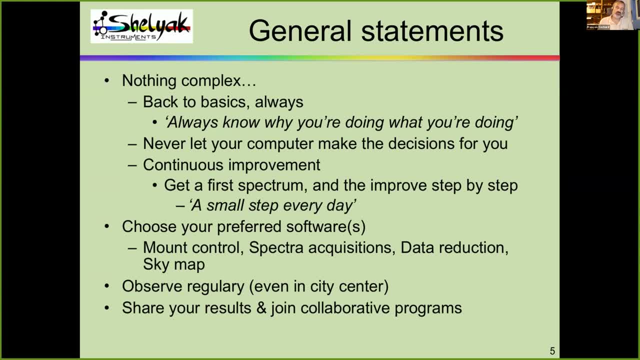 you, you cannot show your results and you, you will keep them for you and you, you don't dare to to show what you have done. i can promise that this is showing your result, even if they are bad, even if they are poor, is the best way to have advices for from the, the, the community, and you know that this 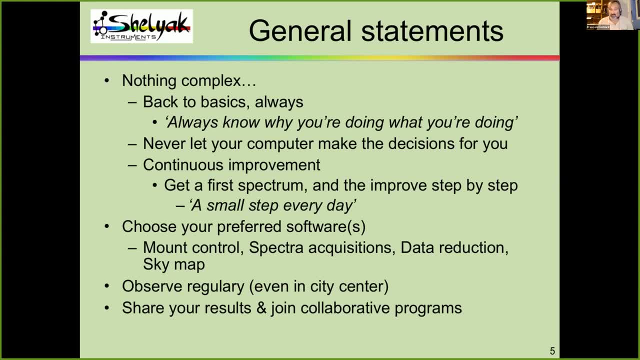 astronomy community is a great community, so i'm sure that you'll have a lot of advices and for me, this is the best way. if you are a beginner and you have done in your backyard, and you if you never want to share what you have done, 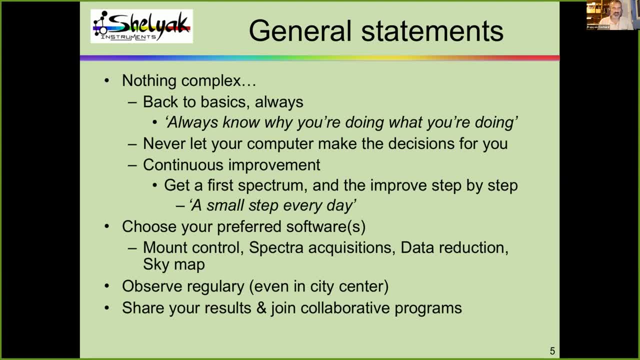 it will take much, much more time to do some progress. so my recommendation is really share your results, show what you have done and and, by the way, if you, if you attend, if you participate to a collaborative program, then you will have a community of experts that that will help you to. 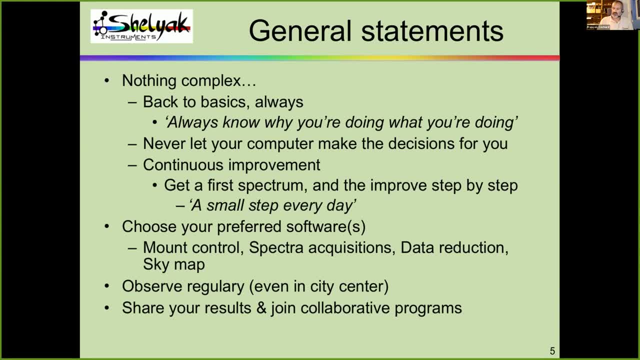 improve your observation. this is also something i like to to tell to people starting in spectroscopy. the experience i have is when you are doing photography, when you are taking great pictures of nebulae, galaxies and so on. this is a never-ending story. so you you always have to improve you. you can always improve something you can exposure for. 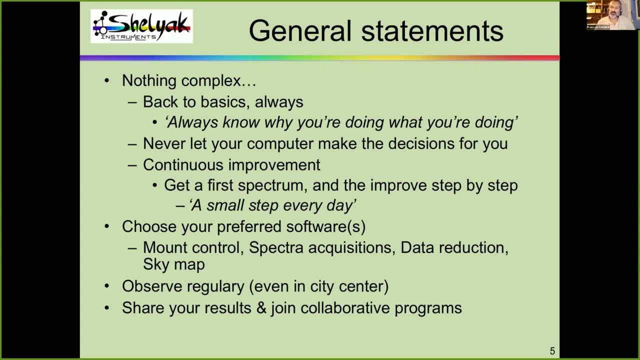 expose for a longer time, you can have better filters and data processing and so on. really, it's strictly a necessary aspect to develop crying for the field, because starring can happen to perfectly flat surface. when you are doing spectroscopic, GREG are taking into its own picture. when you're Darling freaking also, stone Bush, ya ready to arrange like songs. 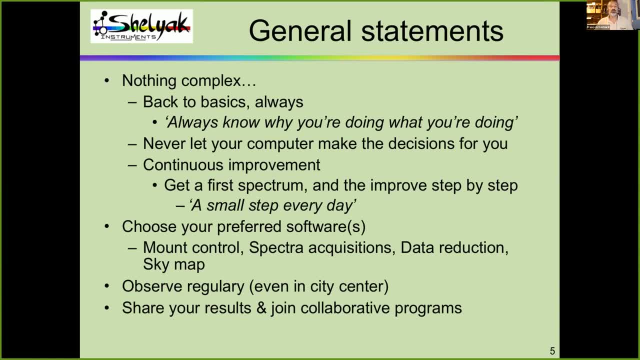 one voice in form, miten that, but at this time several sites. commander is me, so i'll. Manufacturers who are coming soon to spend every day. i was there last night. i am threw the old palsy be pseudos. this is a reallyqueel. that. it's really the with an interesting business story when you are doing spectroscopy. 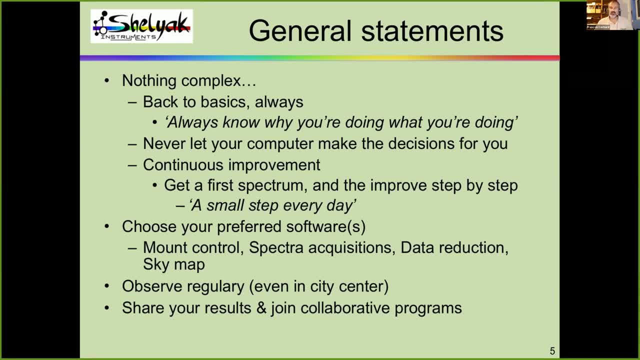 it's a little bit difference. you need to have some time to learn how to take a spectrum and process data and produce a clean and calibrated data. but once you have done are done with the technical size side of the the story and then you can switch to the science. okay, 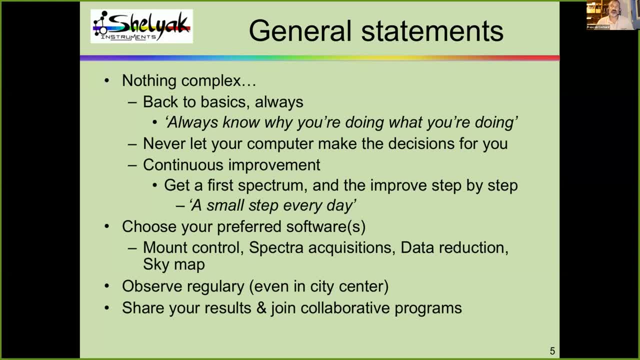 so this is really something important. so of course, the the it will depend on your instruments and if you change your instrument or if you change something in your instrument, you'll have to go back to technical stuff to to put that under control. but really this is um something very. 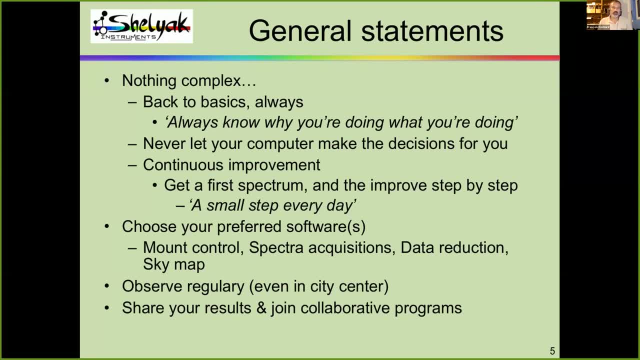 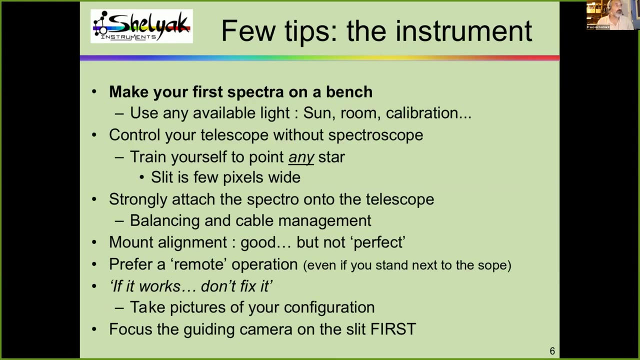 important. when people know how to take a spectrum, then you, you know how to repeat it every day, every night, and it's really a pleasure to switch to science. okay, um, well, by the way it's, it's it's really a pleasure to have all of you. i see that there are 77 people online. it's a little bit. 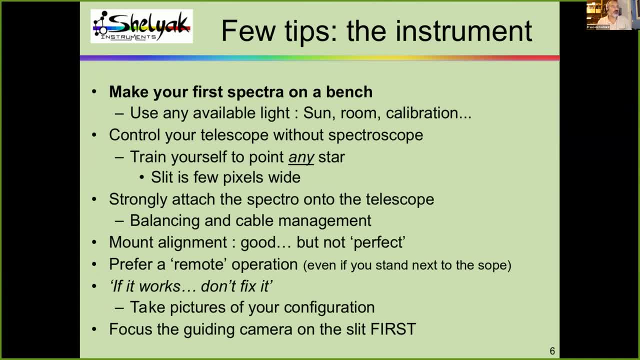 frustrating to not see you and do not have your questions in direct and questions. so that's life. anyway, i know that we will have some time for the questions at the end, but, um, i i would like to make sure that it is okay for you and, uh, and tell me if. 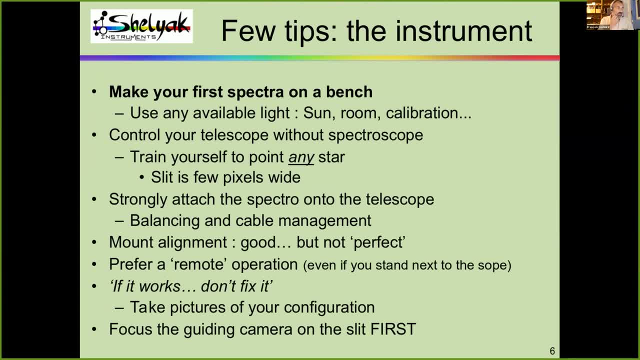 if you have any questions, i will look at you, i will look at the the questions and question and answer. okay, so now let's switch to, uh, some tips about the instruments. okay, the instrument itself. um, something very, very important maybe. if you have to keep in memory one advice tonight, it is this one. 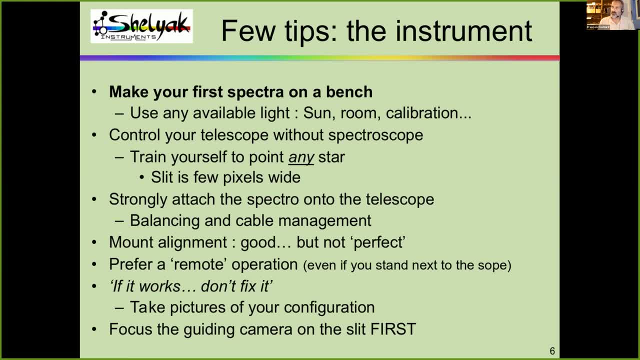 make your first spectra on the bench on the table. so don't put the spectroscope when you receive it on the telescope immediately. take some time to use your spectroscope on a bench and once it is under control and once the telescope is under control, then you can put the spectro onto the telescope. 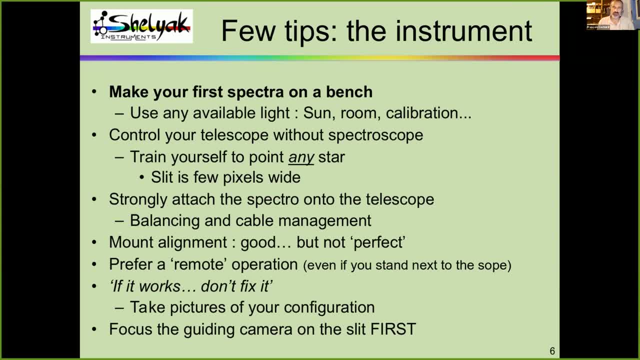 but these are two different instruments and both of them must be controlled, must be a master, and this is really- i repeat it very often. i know that when you receive your spectroscope, the temptation is huge to to put it on the telescope and try to catch the spectrum, star spectrum, as quickly as possible. 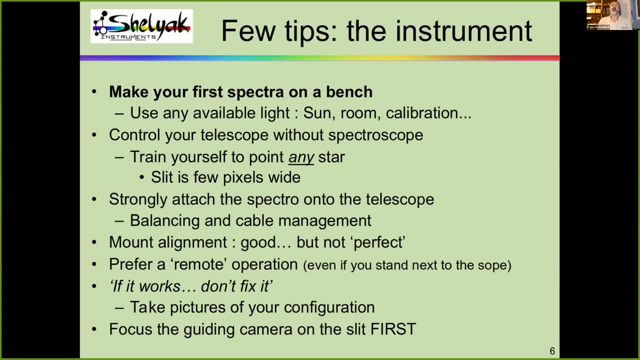 i can promise this is a mistake, okay, and even if you can do it, even if you your success, you are successful to take a spectrum of a star the first night, i'm sure that it will be because you are lucky and you are not able to do it and you to do it again the next time. so really, 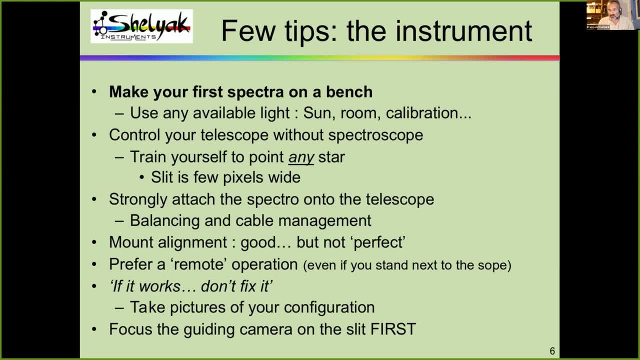 consider that these are two different instruments that we use together to take a star spectra. but when you are using your instrument on the bench, on your table at home, in good condition, during daylight, you can use the lights. you cannot use any light source that you want. so the sun light, of course, that's the light you have in your room. 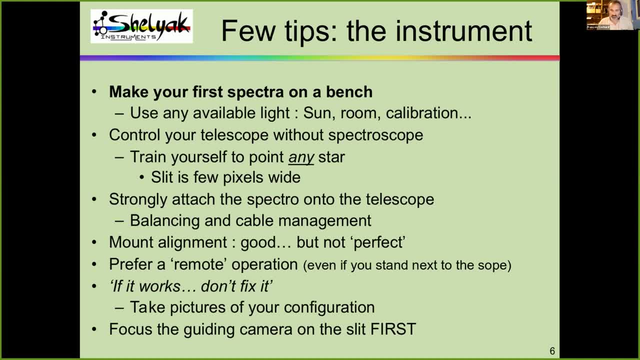 you can. you have calibration lamps, you can use flames, you can use any lamps that you have in hand and and in fact, all the light that goes into the spectroscope through the slit can be analyzed. so you can really start by taking some time to analyze the exertion of the light cutting to the spectrum, to see what happens, come out at example, when at one moment you can do it during daylight. 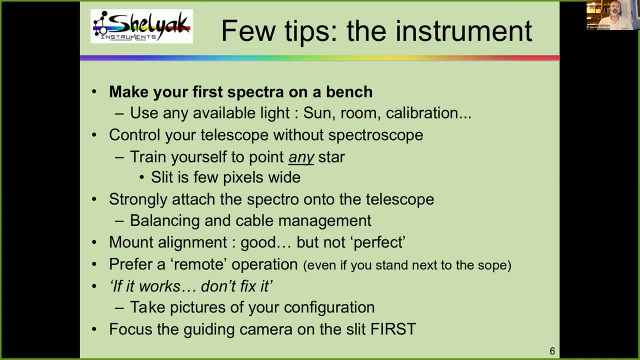 spectra of any light you have you have at home, okay. so this is important. and then you also have to control your telescope without the spectroscope. so I know that for most, most of you already have know how to control the telescope because you are observers, because you are IEVSO members. 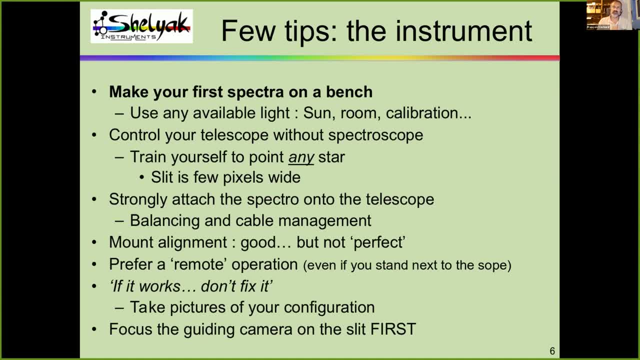 just keep in mind that there is a specificity in spectroscopy is that we are not looking at a region of the sky, but we are looking precisely at one star, okay, and a given star, and there is something which is not easy at the beginning. if I ask you, for instance, to well, the recently. 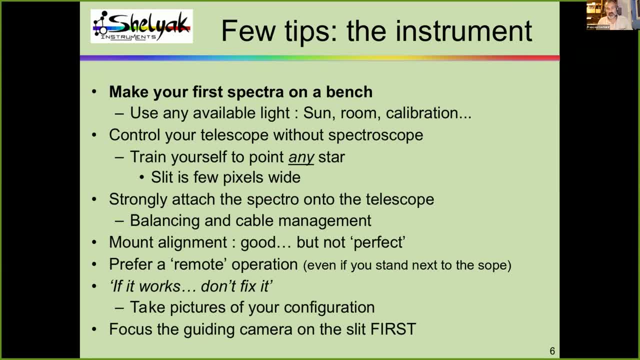 at the beginning of August we had a nova in the sky, which is a rest of focus and the the first time. if I ask you just to point at d star, it can be quite difficult for beginners because you know, okay, where is this, how, how can i, how can i find it okay? so so we will. i'll come back on that later on, but this is something that 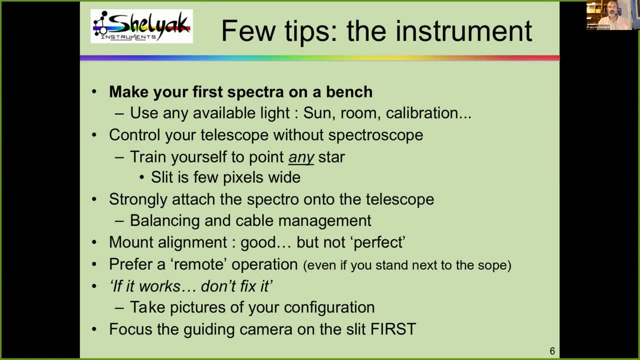 you have to keep in mind when you are doing spectroscopy. you must put put a given star at a specific position in your image, and when i say specific, i mean at few pixels of precision, because the slit image in your guided image is few pixels only. okay, so it means that you must. 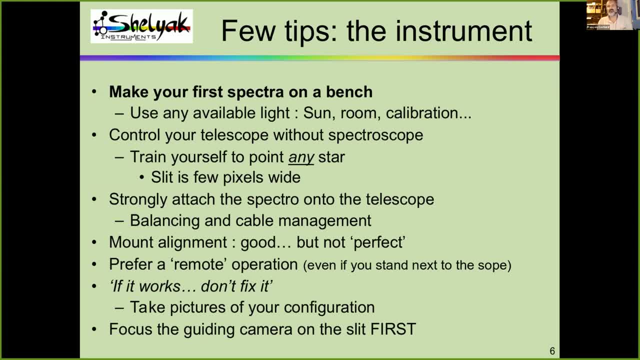 be able to put exactly one star at a given pixel. okay, so it can be impressive when i present that this way, but in fact it's. it's quite easy to do when you have the right, the right setup and using the guiding camera and so on to when the instrument is properly tuned. 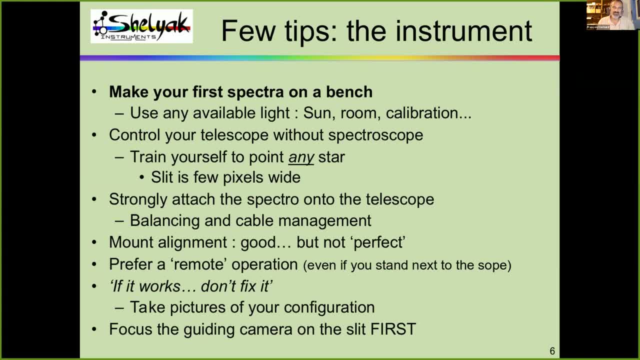 this is something that we can. really, this is not difficult to do, you, but this is something. i'm just mentioning that because this is something which is different between general observations- and well, i mean general observation when you are doing imaging or or astrometry, or the measuring, the photometry of variable stars, and you don't need 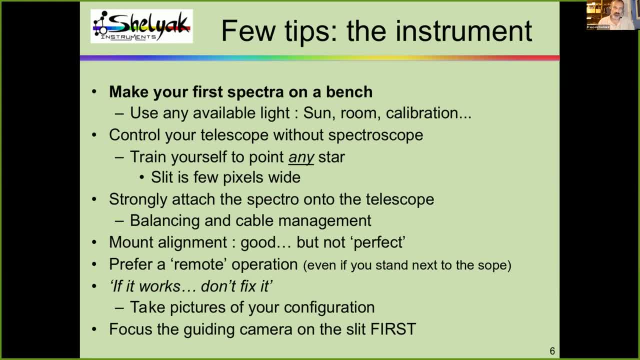 to have the same precision to point your telescope. okay, well, one one. both the spectroscope and the telescope are under control. then you can attach, you can put the spectro on the telescope. okay, in this case you have to make sure that it is strongly attached, because if there is any, 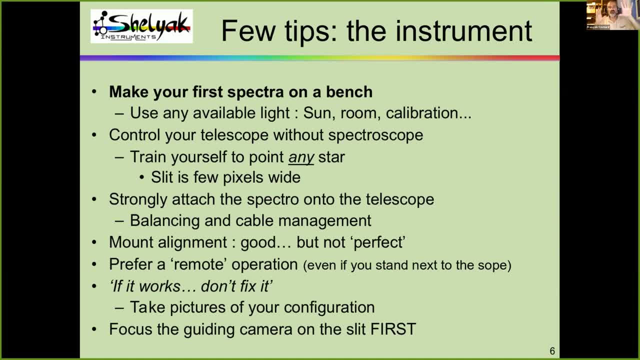 any gap, any free movement, you will have big problems to to put the point at stars, because, depending on the position of the telescope, you'll have the, the, the spectra will be moving and then it will be very difficult to put the star in the industry. okay, and also you have to take care of the, the balancing of the mount and the cable management. 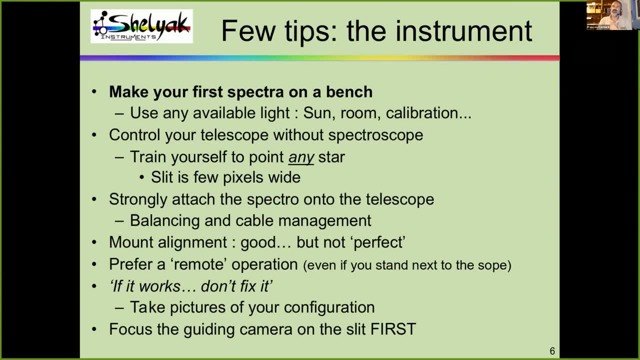 when we are doing spectroscopy, we have usually two or even more cameras. you have the cables for the, for the mount itself, you have the, the, the cable for the different power supplies, and so on. so you may have a quite a high number of cables and and make sure that you have a proper. 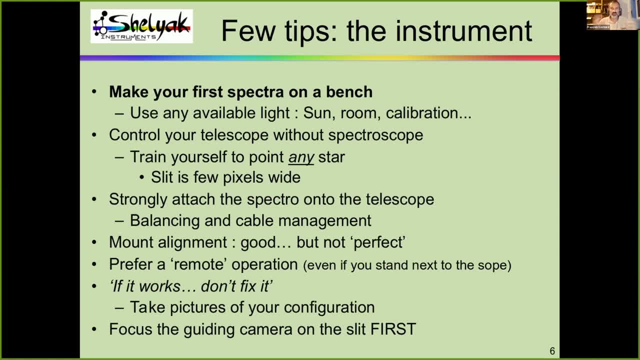 pass for the cables to make sure that when moving the telescope there is no risk to unplug any cable. okay, or unplug cable or pull on the mount and make the guiding failing. okay, of course you must have to have a good alignment or the good mount alignment. so 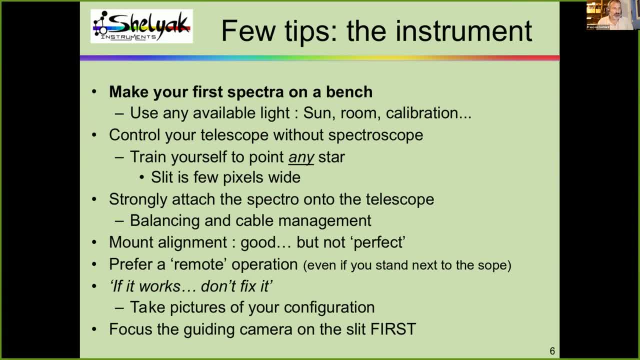 you must align your mount to the polar star or the rotational axis of the earth, and so these alignments must be good, good enough. it is not necessarily perfect at the beginning, okay. so remember, at the beginning i told you that you have to get the first spectrum, and 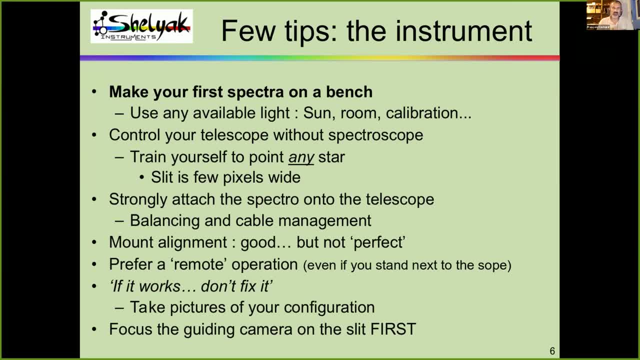 then improve it step by step. so this is typically- typically- a step that can be improved over the time. there is no need to have a perfect mount alignment. i've seen several people saying, wow, the lighting is really good, but also the instrument is not perfect. okay, so the 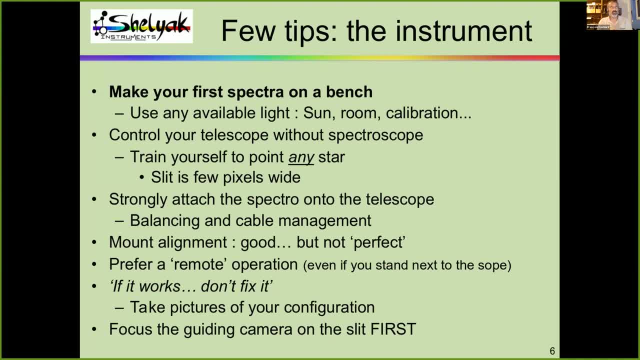 the elevation of the instrument is quite complex, and then i will spend a lot of time to do that and in fact maybe it's not necessary, especially because if you are observing bright targets, which is a recommendation for the the first observations, of course, then the exposure time. 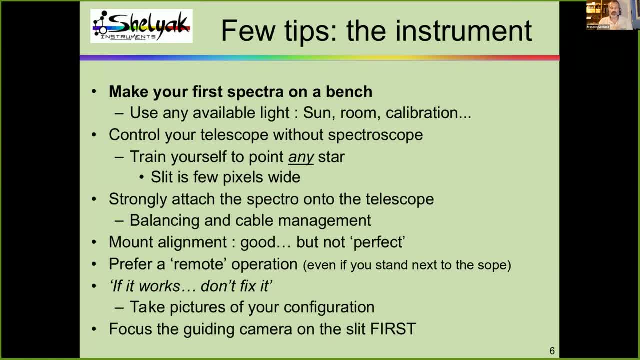 will be very short. so if the exposure time is short, you don't really care. if the guiding is not perfect, okay, so you'll have to improve the, the mount alignment, you have to improve the guiding and so on, but at the beginning this is not a very high expectation, okay, uh, a small advice also prefer. 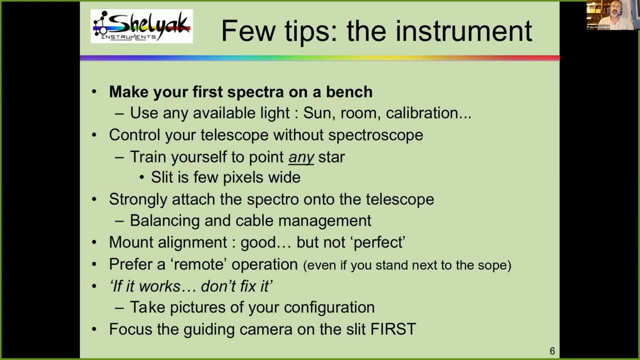 a remote operation. when i mean remote operation, i mean usually, uh, when you're starting spectroscopy, you have the telescope and and you have a table, uh, just beside the telescope and your, you work from the table and it is better if you don't have to go to the telescope, for instance, to switch on. 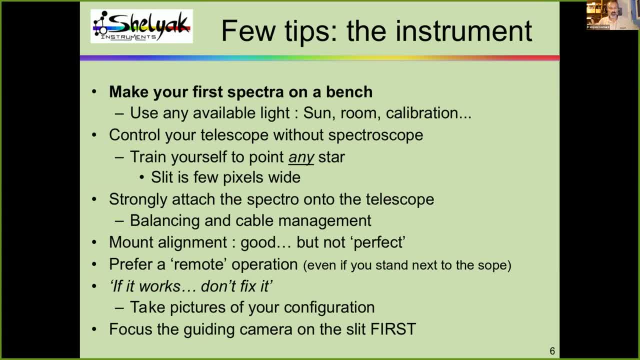 the calibration or the flat light, or or maybe to to uh to point, to point at the star if it's better, if you have a way, uh, for instance with the go to mount, uh to have to point automatically, or at the star, uh, not using to to put the high uh in your eyepiece or in your sky finder. 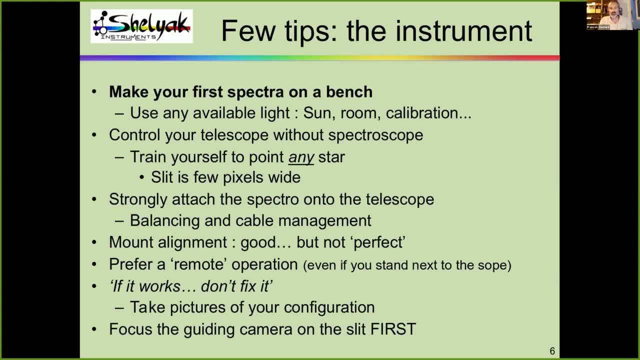 or as soon as you, you touch, you put the, the hand on the telescope. there is a risk to move something, to applying, unplug a cable or something like that. so it's always more comfortable, uh, to to work remotely. so of course it really depends on the instrument you have. for some of you it's very easy and it's obvious some. for some other, 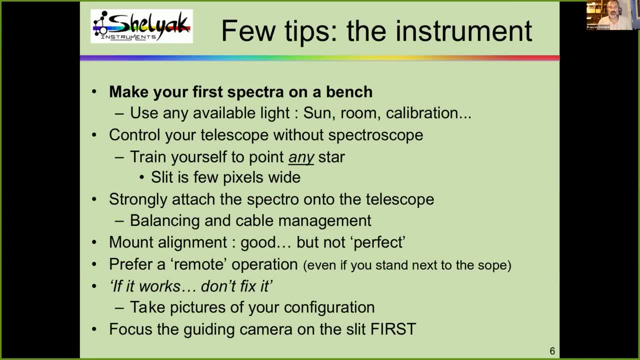 you have an instrument that you really use manually. so if it is the case, don't change it. keep this instrument and do it manually, but just have that in mind. it's it's always better to not touch at the instruments during the operation, okay, so i like also the idea: if it works, don't fix it. so it means that 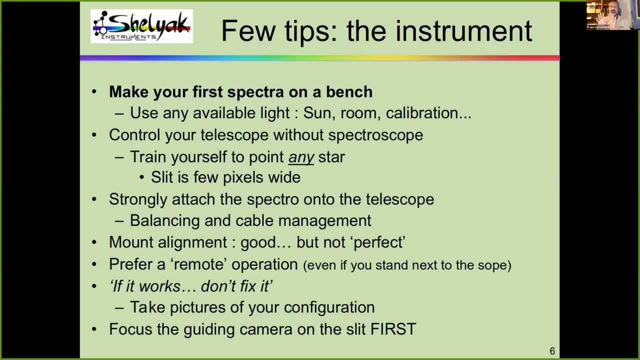 you have to tune your instruments. but once it is tuned, please don't change anything else. keep the instrument as it is. and also i recommend to take some pictures of your configuration to look at the orientation of the camera versus the spectro, to the orientation of the spectroscope versus the 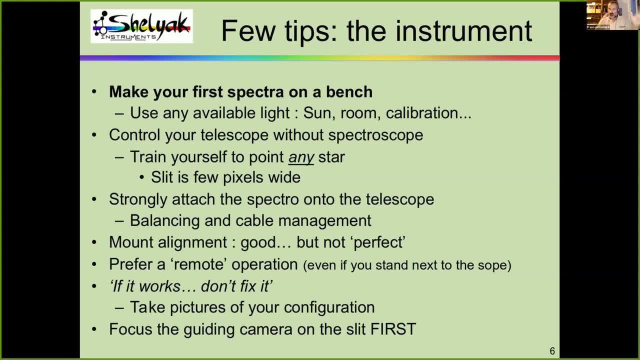 telescope and so on, to make sure that next time you will, you will recover exactly the same configuration and then when you will work, uh, on your computer to take the images, you'll have exactly the same behavior. okay, if you rotate the camera, for instance, on the instruments. 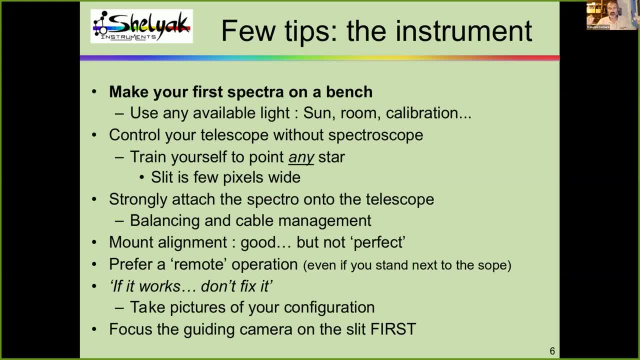 maybe the, the today, the- the spectrum will be horizontal in the image, and, and then the two more. if you rotate the camera, the spectrum will become vertical, which is not a good idea, in fact. okay, so when the configuration works, please don't change anything else and keep it as it is. 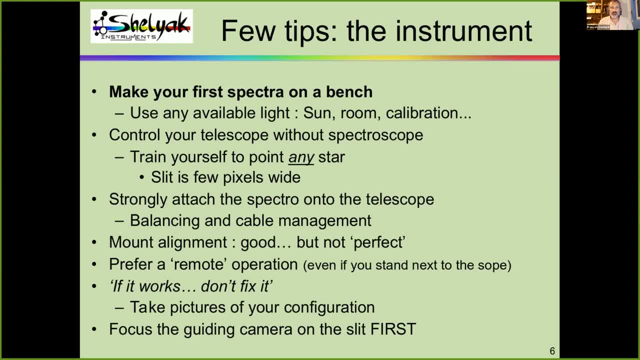 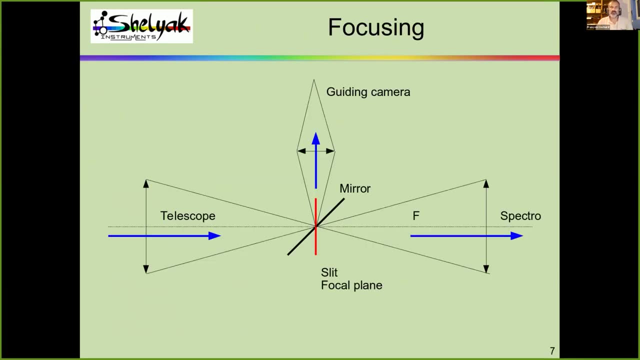 and another point regarding the instrument. again, this is an important point: focus the guiding camera on the slit first. okay, so i do have an image? i think? yes, i do. so this is symbolic representation. so you have the light coming from the telescope here and the the. the job of the telescope is to collect all the light from the star and to focus it. 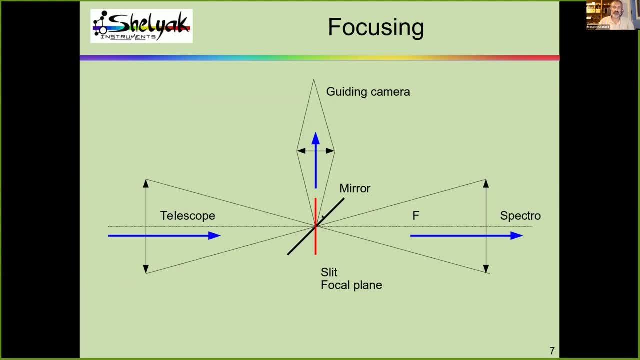 in the focal plane, okay, and in the focal plane we have the slit, which is here and we have usually. the slit is put on the mirror and this mirror allows to send the field, telescope, field image towards the guiding camera where the light that goes through the slit goes to the spectroscope. okay, what i'm seeing saying here, i'm 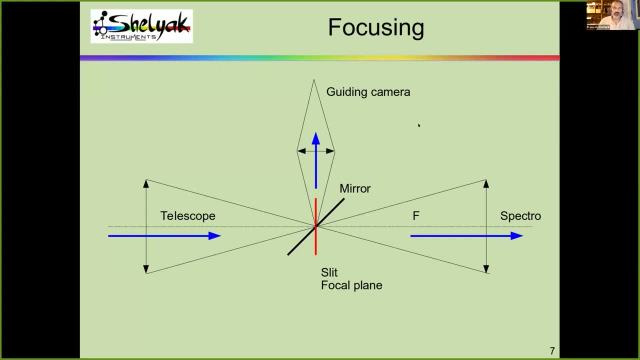 talking about the focusing of the camera, guiding camera- sorry, guiding camera here- and the telescope. okay, it is absolutely important to focus the guiding camera first- and generally it is during the light- and to make sure that you can see the slit perfectly sharp in your guiding image. okay, 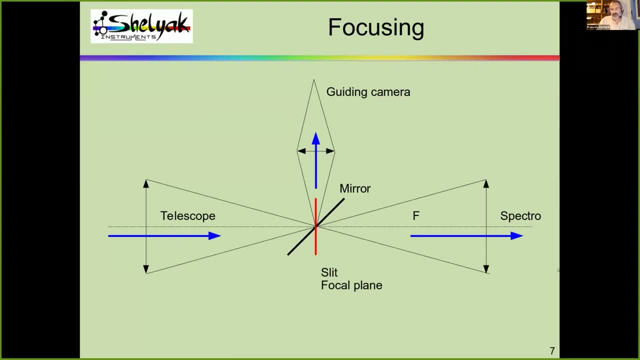 why do i say that? well, the spectroscope is quite independent, so you have to focus the spectroscope on its own and we usually use the calibration lamp. so it depends on the instrument, but we use the use the calibration lamp and make sure that the calibration lines, emission lines, are as sharp as 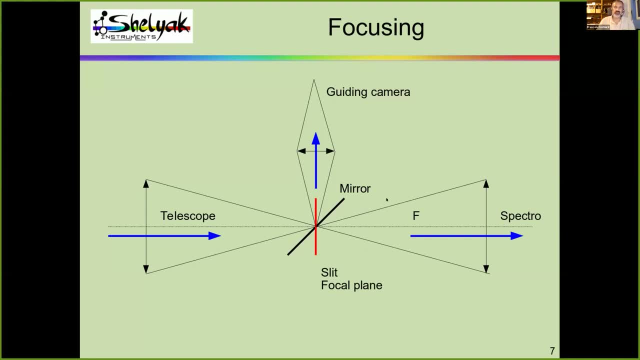 possible. okay, so this is for the spectrum, but now here i'm talking about the guiding camera and the telescope. why i'm saying that? because you may have this situation. i've seen that many, many times. a lot of users are doing this mistake. this is a very basic mistake if you are doing that, so 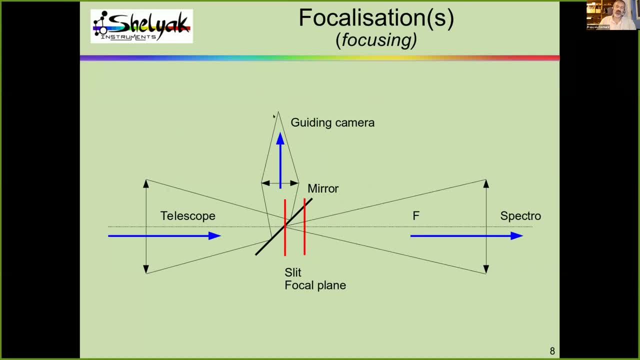 in fact, if, if you put the camera, the guiding camera, and and you you don't really take care about the focusing of the guiding camera, and then you wait for the night, and during the night, you, you change the focus of the telescope and then, in this case, you can have the telescope, which is 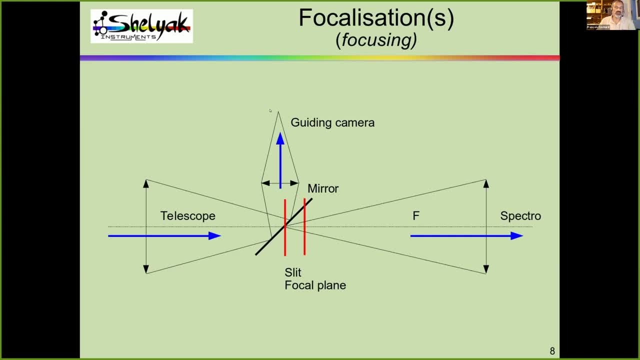 perfectly focused on the guiding camera and then you can see the stars that are sharp and perfectly sharp in the guiding camera. the problem is that if you do that, you are totally unfocused. or this slit, and then you cannot even see the slit, or maybe you can see it, but it is quite fuzzy, okay. 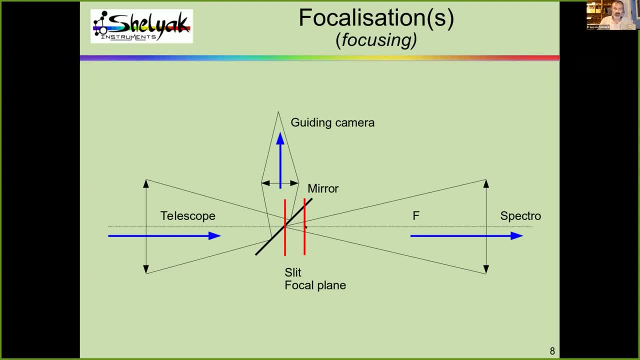 and you have to understand that in this case the telescope is focusing its image at the. so this is the, the telescope focal plane and this is the slit enter. so if you look at that, if you look at the image, the size of the image of the star at this position in the slit, 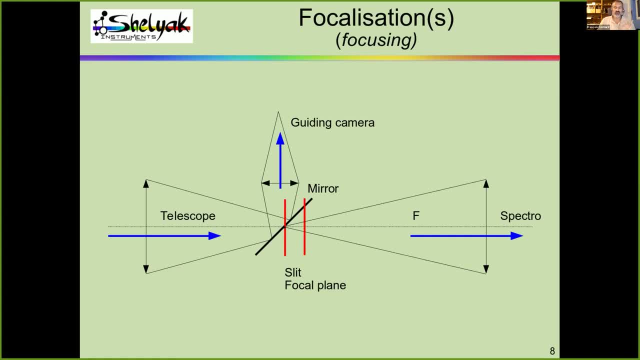 it is huge, okay, and it is totally unfocused. so you feel that the, the focusing is correct in the guide, because you can see a sharp star in the guiding camera but you cannot see the slit, okay. so this is why it is so important to have the, the, the guiding camera. 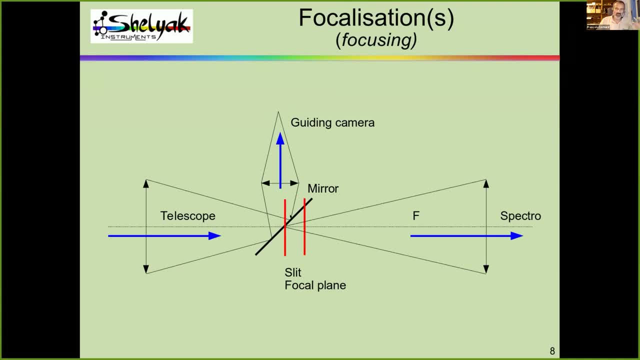 focused before uh during daylight and make sure that you can see the, the slit of the of the spectrum perfectly sharp. and then during the night you will have to focus uh the telescope to make sure that the star is focused in the seat. but at this time during the night you never. 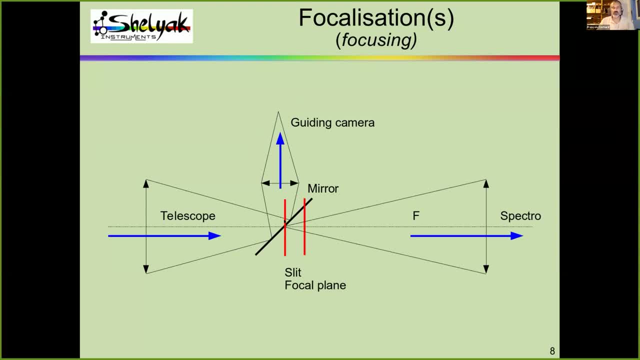 change the guiding camera focus to make sure that it is properly focused on the slit. okay, um, so i think, uh, that's it for, uh, most of the, uh, the, the, the, the, the instrument itself, we. we could spend hours, of course, on this subject, but i'm i'm going fast uh, to these different uh. 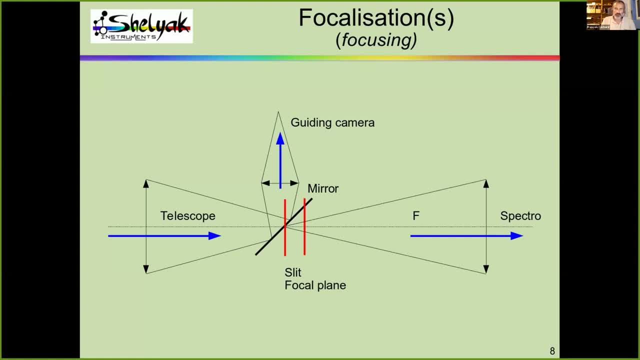 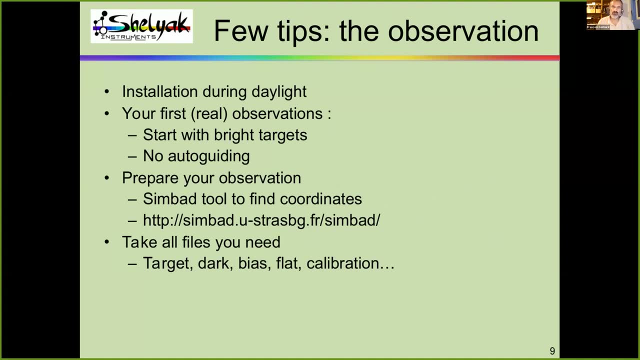 uh topics. um, now i will switch to the uh the observation itself. okay, so here are some uh recommendations. um what i didn't say that at the beginning of the of my presentation, but all what i'm telling you tonight is for me it is really based well, first of my own experience. so i can't tell you that i've made many. 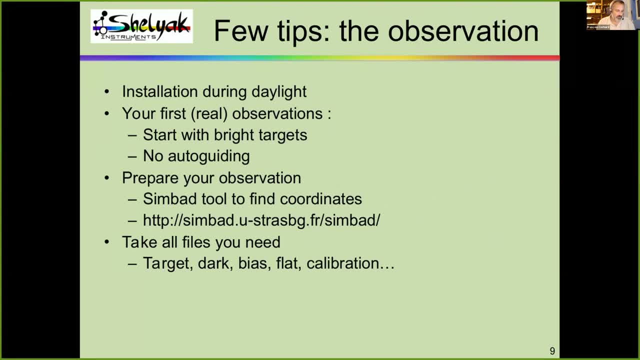 almost most of the of the mistakes that i'm describing here and- and you know, lauren, you, you told at the beginning that i'm an expert in in spectroscopy, so it's quite impressive, but my definition of an expert is this: is somebody who has already made all the possible mistakes. 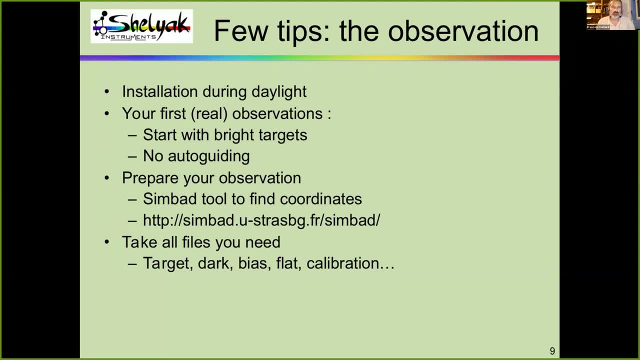 so maybe in this case i can tell you that i've made the most of the mistakes i'm talking about. so it is better based on my experience, but it is also based on all the beginners i've seen and all people i've seen, especially during the uh, during the, the sessions at the ohp, at the observatory. 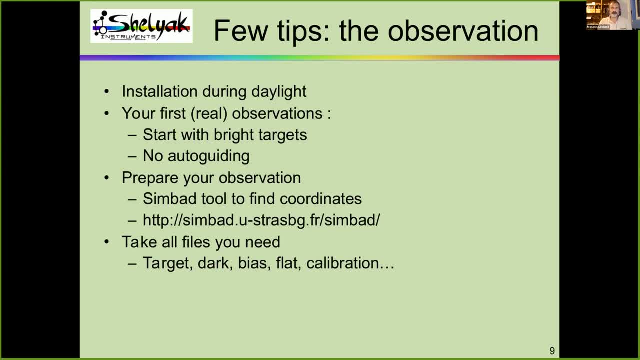 province that we organize, organize every year, and we have seen a lot of people, we have helped a lot of people, and so this, what i'm telling tonight is is really, uh, really, based on what i've seen there and i- i well, i guess probably we, you will do- uh, some of these. 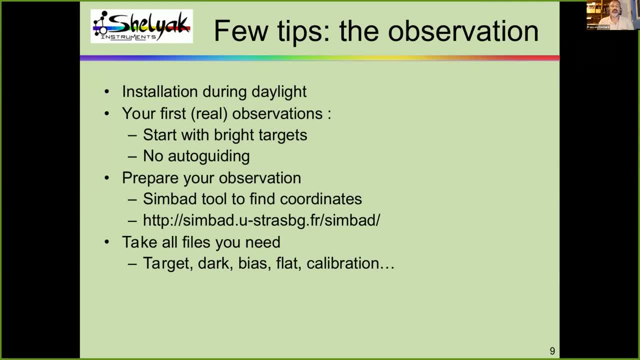 mistakes, uh, but now you, you will be aware and, uh, and, and i hope it will help. anyway, i come back to my presentation, uh, regarding the observation itself. so you have, you have put and not under control. so you, you, you masterize the, you or your master, i don't know- the, the spectroscope and the 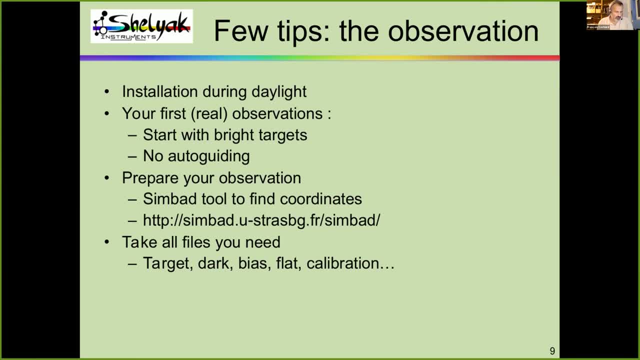 telescope and you have assembled the spectroscope onto the telescope and everything is is ready for a real observation on the sky. so first, again, this is something obvious, but i've seen many, many times this mistake due the installation during daylight. okay, so so the night is only made for the observations. 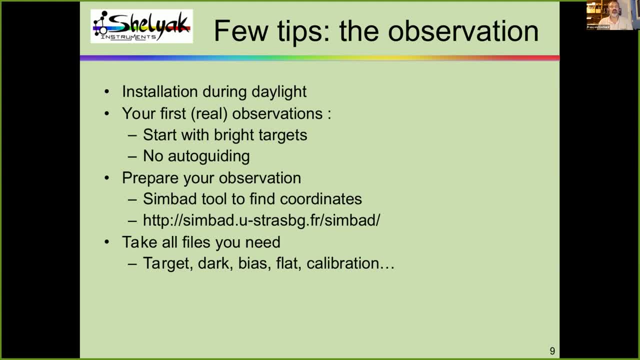 but don't wait for the night to install your setup, and night, during the night, and uh, uh. this is basic recommendation, but it is much, much more, much easier to doing during daylight. and and well, for instance, is, if you have to- uh, i know that- uh, if you are doing some high resolution observations and you, you want to observe the h alpha. line. if you want to know exactly why is the h alpha line during the night, it will be very difficult where, if you do that during the day, during the day, we have the sun cause. during the day the sun is Yeshua sun, so struck. the sun is convenient and because the sun was summer and this와ij, 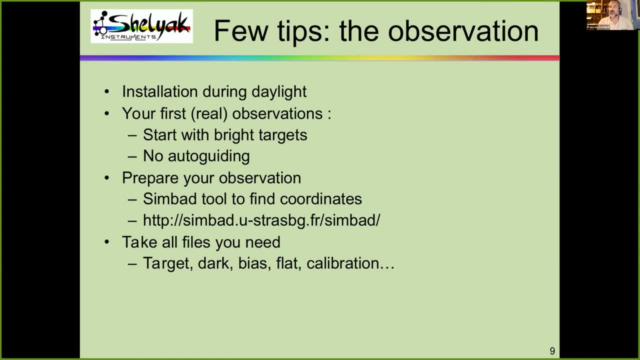 ு light and and you just have to look at the sky and you have immediately the, the h alpha line and it's very easy to find it. so this is an example. but you, to install everything, do that during daylight, of course, when you are starting for real observations, when i mean really. so i mean 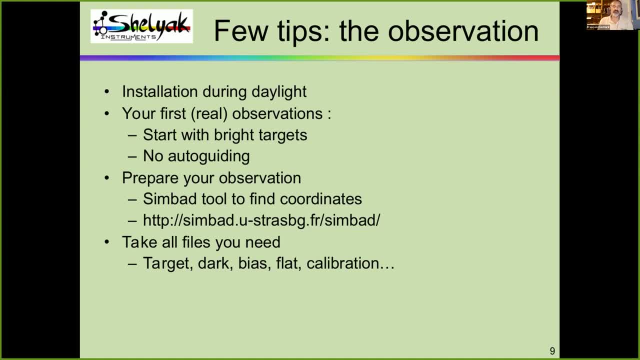 the different observation, so the star observation and and star other than the sun observations. so after you finish to do your, your first uh observations on your bench or on your table, you, you can really switch to stars. and then the first recommendation is: uh, shoot from bright stars, and it will. it is much, much easier. the exposure time will be very short. 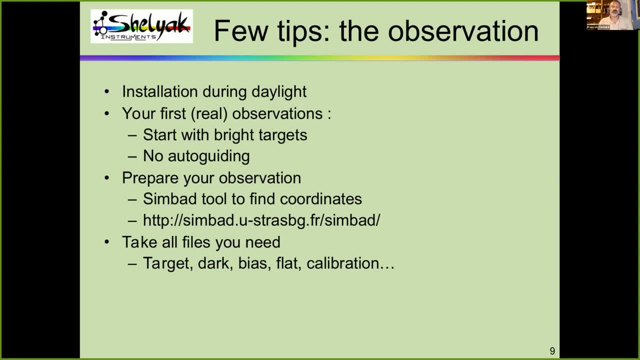 if you, if you take for any instrument in your resolution, uh, you, if you approximate and any telescope, i would say, if you observe vega or bright star like that magnitude, or 012, the observation that your acquisition will take, i would say one second, less than one second for vega, and then it is very easy to do and even if 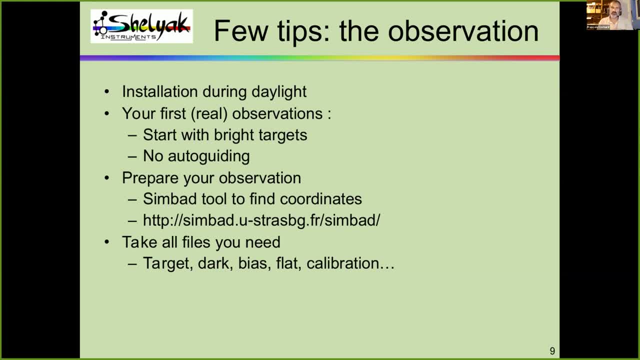 the conditions are not optimal. again, i tell you again what i told at the beginning. so you have to have a full spectrum and then improve it step by step. so even if the the, the tuning of the instrument is not good at the beginning, and if you look at at vega, for instance, well, if your acquisition takes 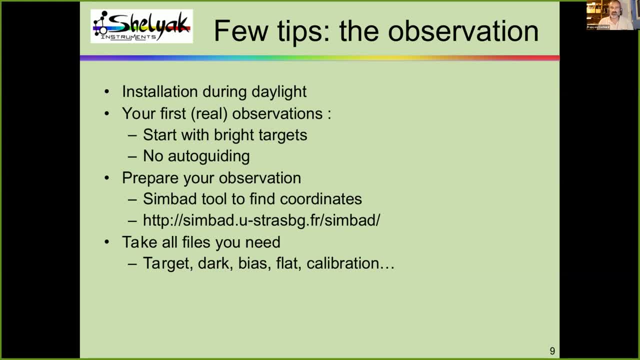 five or ten seconds instead of one, we don't care. so it's really not not a big deal, okay. so start with bright targets- it's always the best. and then, when you start understanding how it works and have great observation, then you can go fainter, and fainter, and and and, up to the limit of your instrument, of course. 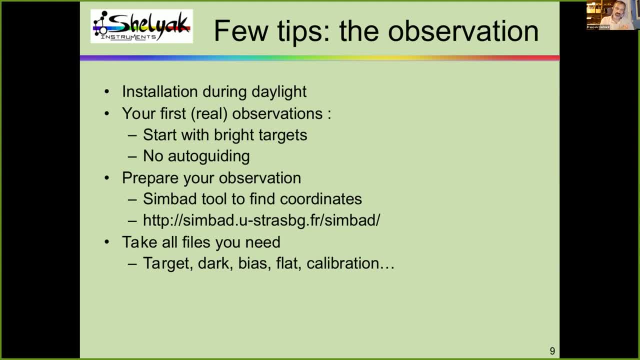 so at the beginning the observations will the the exposure time. exposure time will be only few seconds and then when you go to find a fainter object, it will take few minutes or even few hours and of course, if you are shooting for a very faint source, that 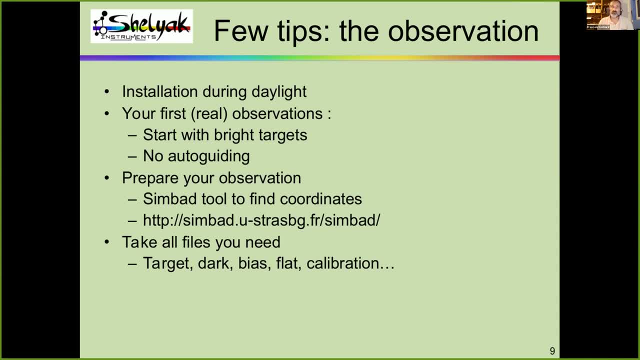 require a few hours, then you'll have to put under control everything: defocusing, defocusing the, the, the auto guiding parameters and so on. okay, um, the other recommendation for your first observation is to not use the auto guiding. prefer to guide manually. and again, if it's just one or 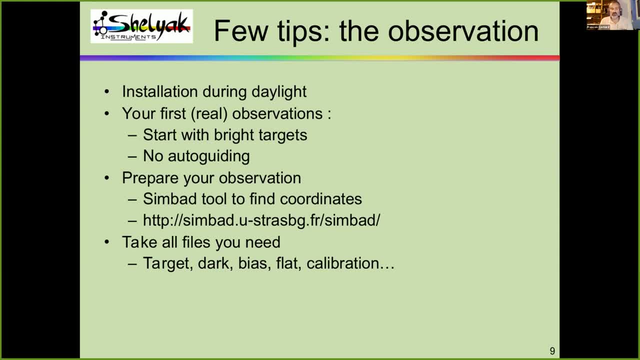 two second observations. it's quite easy. you just make sure that the, the star in this is in the slit of your spectroscope and just run the acquisition and that's it okay. um the the. this is only when you have go to feiedzora targets that you have to to have um to set up the auto. 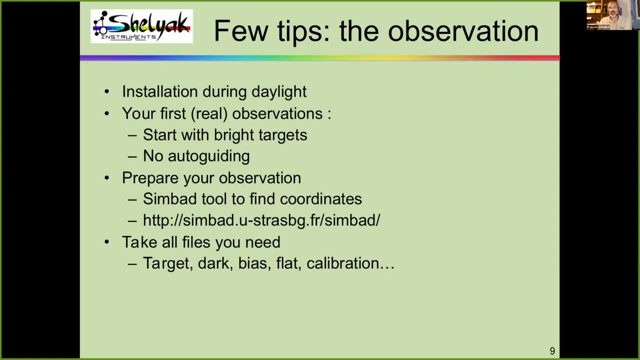 guiding and and set up the other. guiding is one of the step uh that you have to put under control, uh, but this is not necessary at the beginning, okay. another recommendation to have a good observation is: please prepare your observation. if you, if you just uh install your instruments in the field or inner field. ل fundamentals. there is not to avoid, especially in a very close focus position organization, to properly optimize your observation on in the field or inner field of you이ы BMWing. It is, in practice, the only cosasimple in this process. also, you canUp to 5-10 minutes. 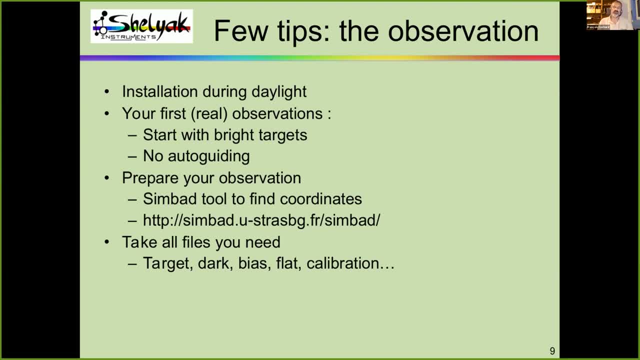 that you have to pre-set your observation. Okay. another recognition: to have a good observation, please prepare your observation. tom mixtion too. and other if you, if you just install your instrument in the field or inner field or in your backyard and say, when the night arrives, you say, okay, what do we do? i observe. 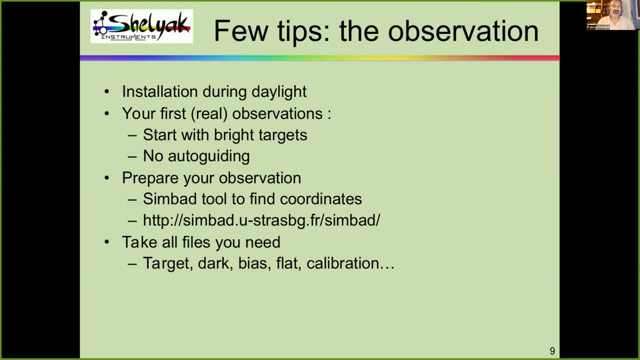 tonight, i don't know exactly. i'm quite sure that the result will not be enough and will not be satisfying. so, before that, prepare your observation, select the stars that you want to observe, make sure that the stars are visible where you are during the night, and so on. so if you do this, 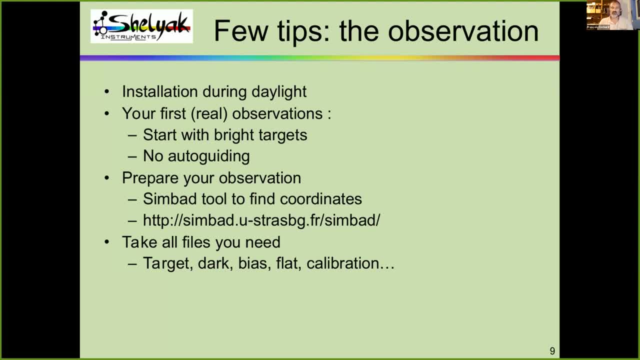 preparation, you really will be much more efficient. okay, and, by the way, if you want to have any coordinate of any star, use the, the simba, the tool, from the cds, so from the, the, which is the center for documentation of stars, i think, which is the worldwide database for all the coordinates of any, any star. it is really a. 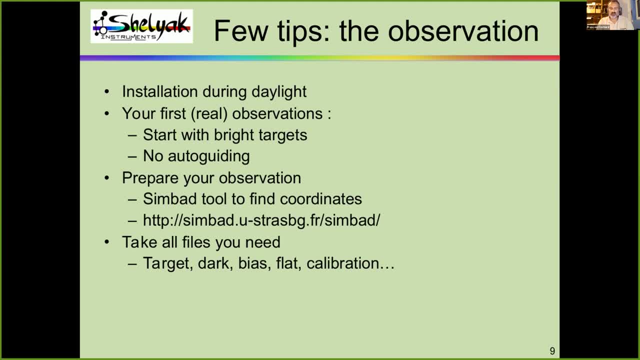 key instrument for us. i told you that if, for instance, i give you the name of rsof, which is a nova that exploded at the beginning of august, done the first time, it's not easy to find and using this tool you will find the exact coordinate. and, by the way, it comes back to what i said before. 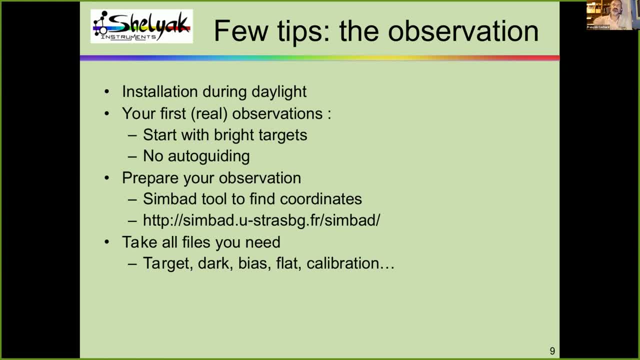 so you have to be able to put, to give the detailed coordinates of any star to your mount, to make sure that you can point at this target. of course, if you, if you are, you playing with bright stars like vega and arcturus and things like that, so your, your mounts, will know it and i'm sure that you can find the name of the star in. 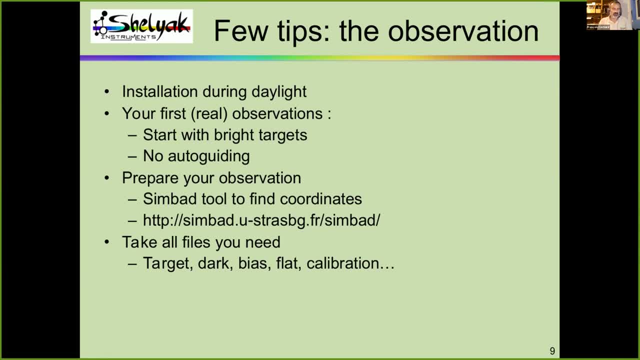 your in your mount pad and and it's easy to do. but now, if you are going, if you are looking for fainter target, uh, i'm not sure. i'm even i'm sure that it will not be in the database of your mount and you have to to give the exact coordinates to the system. okay and um, so this is the way to to get. 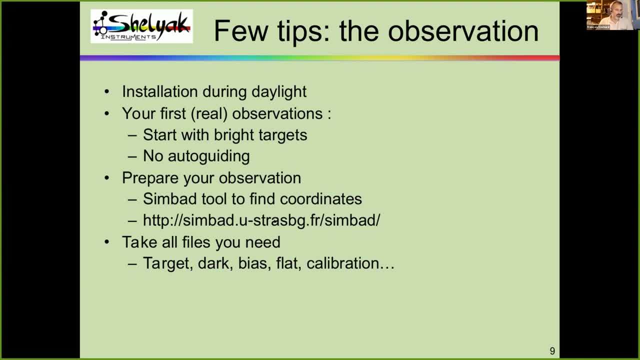 these coordinates and and try to point a star by giving the coordinates to your mount and not only the name. uh, if it is a common name, okay, uh, the. the last point, uh regarding observations is: um, to look at the uh, make sure that you have all your uh, the the files you need. 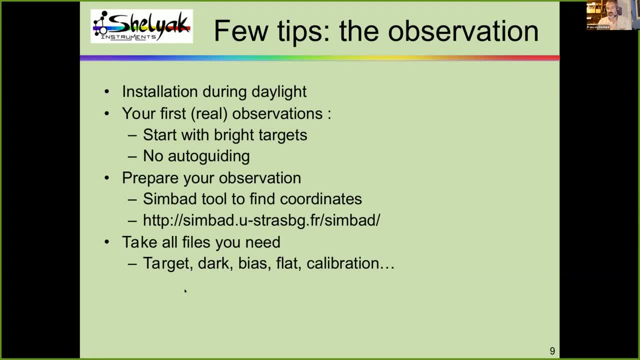 so you have to have a spectrum from the target, but you also have to have dark uh image, bias image, flat spectra, calibration of spectra, and all of that is required to have the full um observation and your full data properly processed. it's a pity if you, during the night, you just it, it happens. 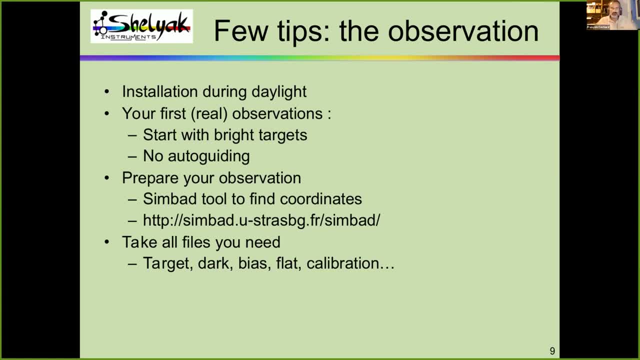 very often also, you take the, the targets, you take the darks and so on, and the day after you say, okay, so i will process my data. i'm very proud of what i've done. last night and i take my file, i say, oh, i forgot to take my flat images and then in fact, i cannot process properly my images, so it's a pity. so also. 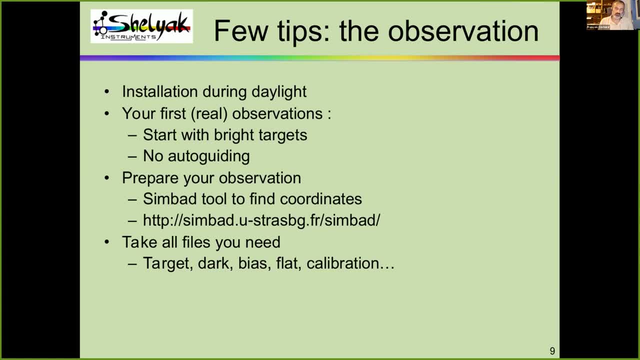 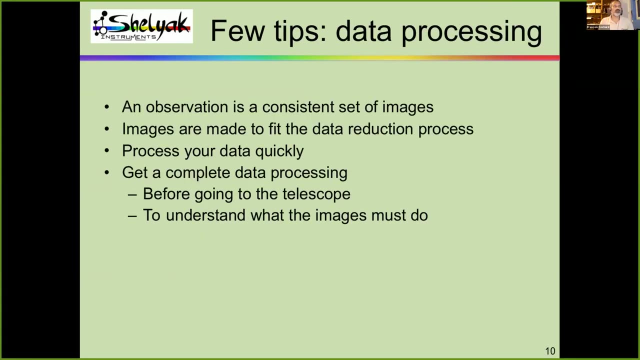 be prepared for that and make sure that you, you don't, uh, don't- forget anything during the acquisition. this is another reason to prepare your observation. in fact, okay, regarding data processing, uh, maybe i'm going fast because i'm a little bit late regarding data processing. so, again, it's important to consider that. 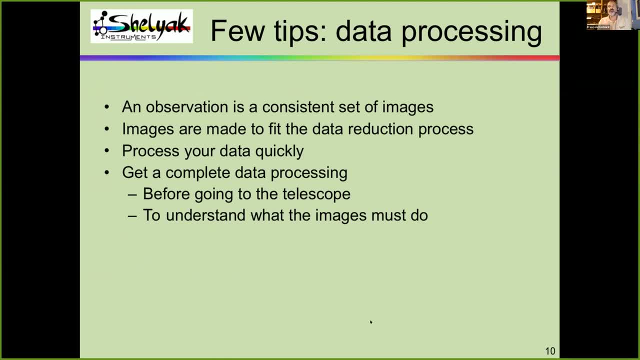 doing spectroscopy is not only taking images, but it is also process data, because the raw images are are not usable and and then we have after the acquisition. we have to have this, this task to process the data well. today, if you are using some well-done software like Isis or Demetra, for instance, 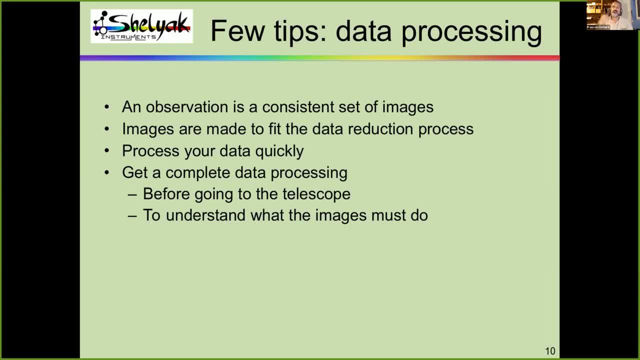 it can really be done in a few clicks. And when you experience, you can really do that, do the data processing, just after your observation. And I can tell you that when we started to develop the Demetra software, for instance, one of the goals was to say: 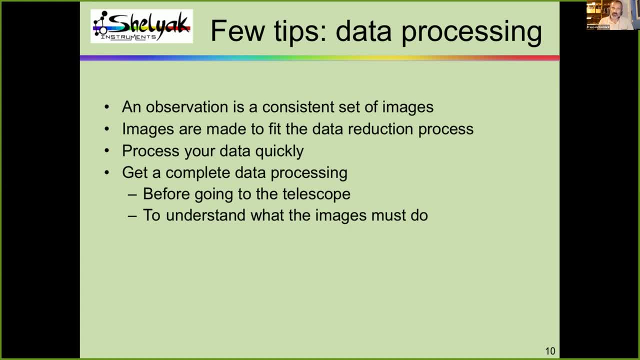 okay, when I finish my observation and when I go to bed, I want to have already processed my data. okay, Because I know it's very dangerous to say: okay, I take the data tonight and tomorrow or the day after or next week or next month or next year or whenever I will process the data okay. 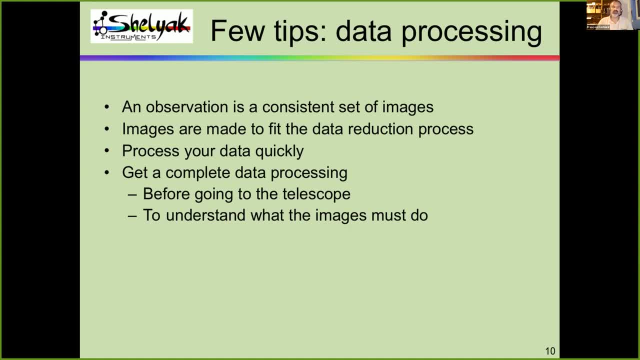 So it can be very simple, but make sure that you have all you need to process this data in an efficient manner. Keep in mind that an observation is a consistent set of images. Well, by the way, this is something which is very important in Demetra. 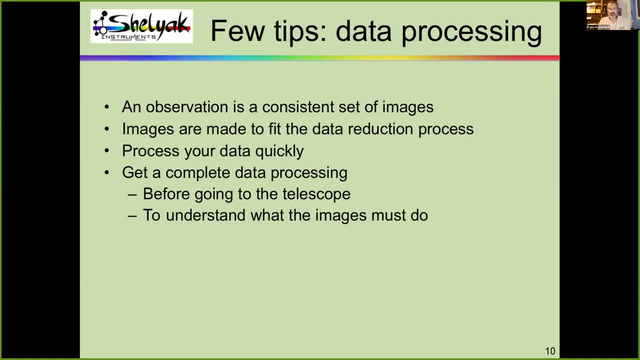 because we talk about observations and not only about images. And but to take a good spectrum, at the end you need to have the target spectra, the flat spectra, the calibration spectra and so on, And the observation is this consistent set of images. okay, 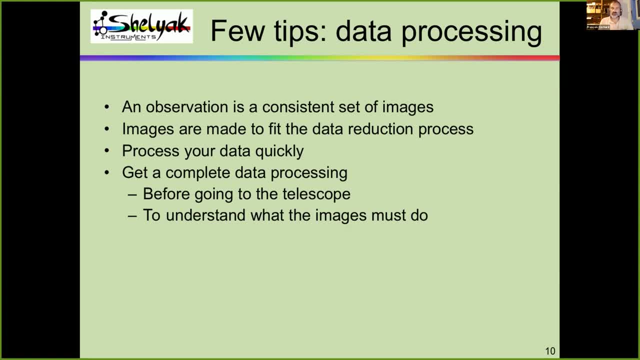 The next point, for me very important also. please keep that in memory. So this is a very key element. The idea is not to take images and then after that process your images. It should be the reverse. Define your data reduction process. 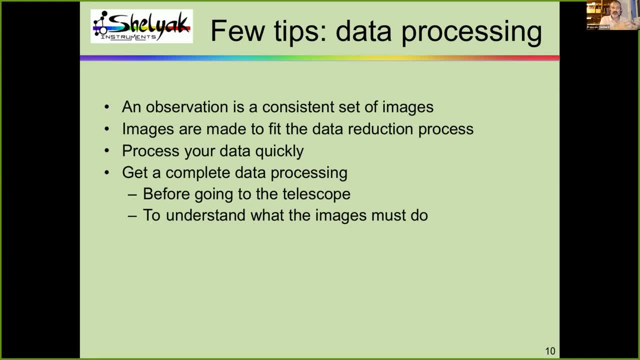 And then, during the acquisition, make, build, do the correct images that will fit the data reduction. This is the key to have a very precise, very efficient way to proceed. OK, so consider that the data reduction process is the core of the observation. 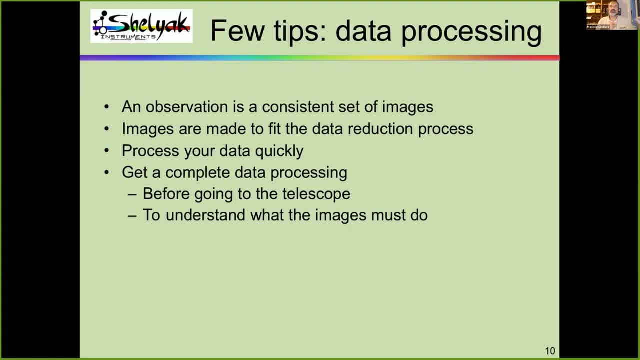 And the telescope is just a simple device to take the data that will fit the data reduction process. OK, it can be a little bit strange, but I promise that if you do that, you will have a very efficient and easy way to process data and you'll be very reproducible. 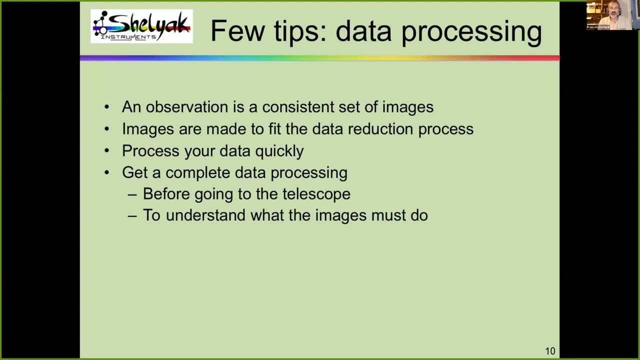 So, from one day to the other, you'll have always the same process and you'll have always the same quality of your data. OK, so again, process your data quickly, because if you wait for next week, I'm sure that you will never process them. 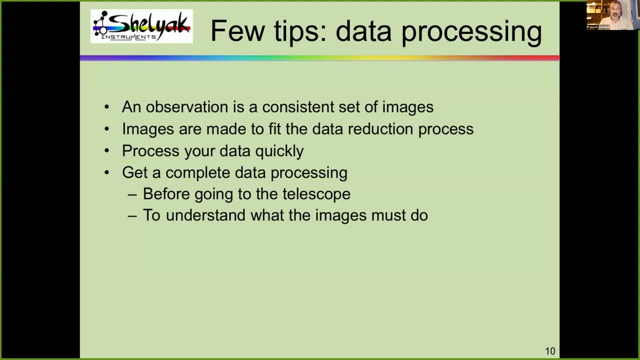 Most of the time this is the case, And then do that very quickly. And again, with the recent software and software, all the tools we have today, the idea is really to do the processing just right after the observation itself, And this is very important: When you are close to observation, you know exactly what you have done. 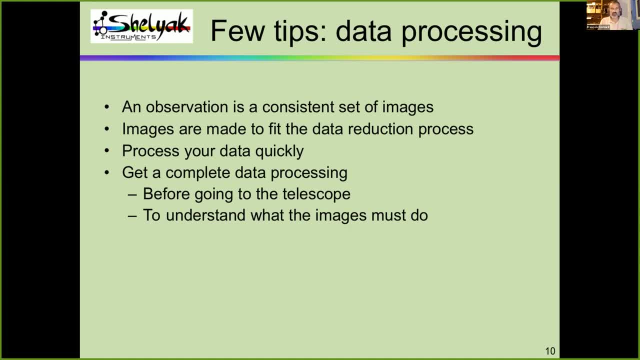 You know why you have different set of flats or darks or things like that. So you have that in mind and it's much easier to do it. OK, And, by the way, this is at a later stage- I told you before that I recommend you to start by using your spectroscope on a bench, on a table. 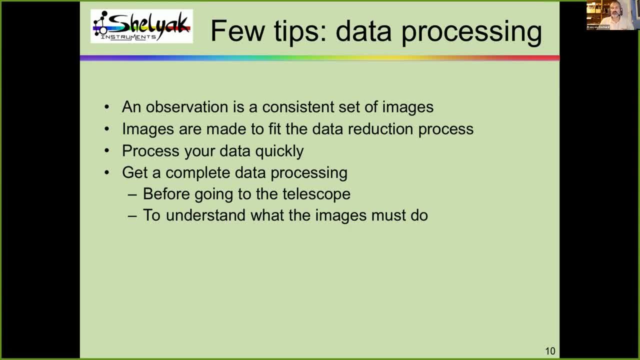 And this is the same idea: When you have done that, process your data on the bench and make really before going to the telescope, because if you do that, you will control, you will understand the data reduction process, You will understand what the images must do in this process. 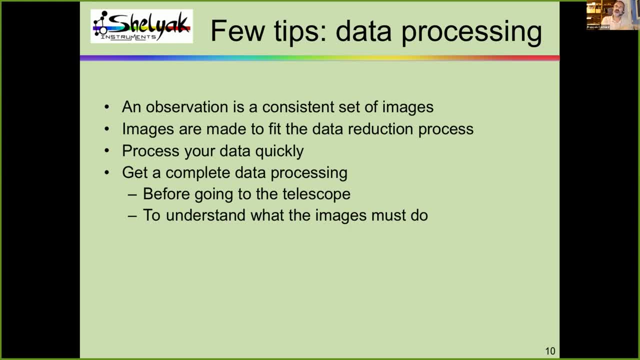 And then you will know exactly what you have to do during the acquisition session. OK, I hope I'm not going. I'm not speaking too fast. Anyway, we will have the discussion afterwards. I've almost finished. I just want to go to this important question. 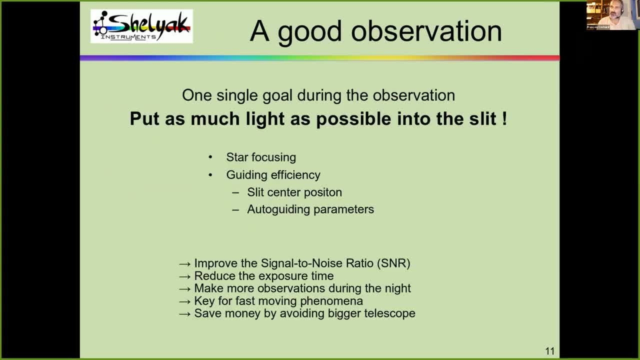 What is a good observation? What makes a good observation? For me, this is very simple. The difference between a good and a poor observation during one night is, in fact, you have to understand that you have to take some time to install your instrument. 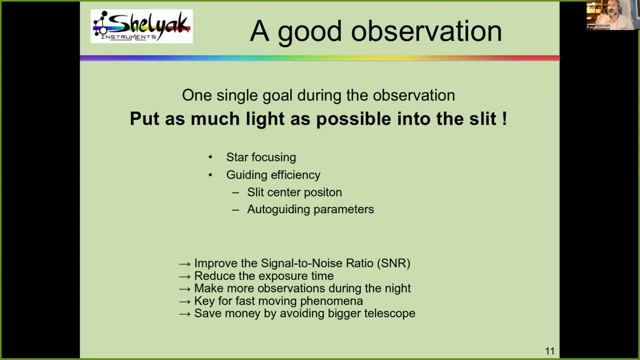 to tune your instrument and to make sure that the spectroscope matches the telescope and so on, And everything is well balanced and is quite homogeneous. But when you start observing during the night, you cannot change the telescope diameter or the telescope focal length Or the spectroscope resolution or whatever. 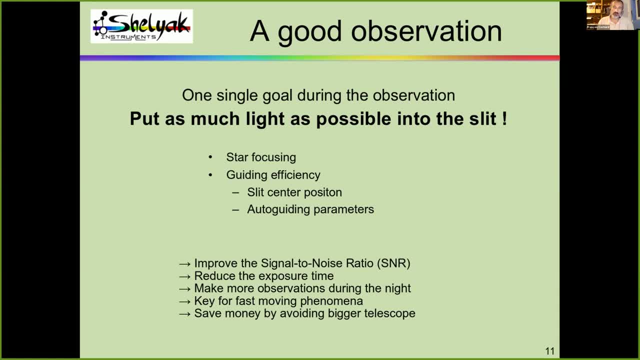 So everything is fixed, And during the night, your only mission is to put as much light as possible into the slit. OK, so this is really the idea: is that the more photons you put in the slit, the better the quality of the observation? 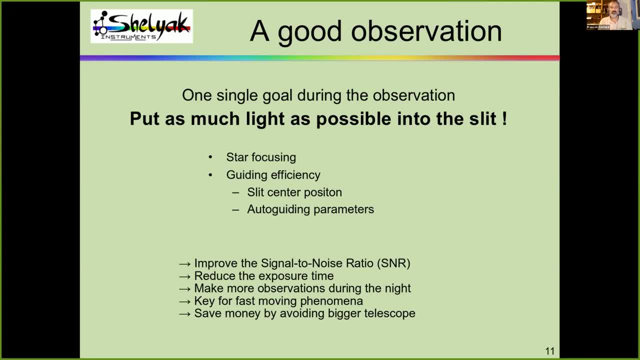 That's it. That is simple like that. So your mission during the night is to put as much photons as possible in the slit. To do that, you have to make sure that the star focusing is optimal, OK, and you have to make sure that the guiding is also good. 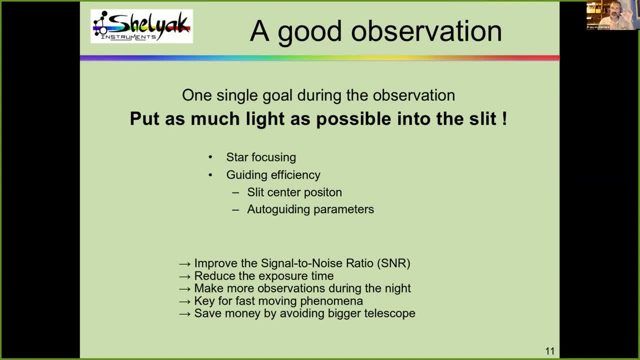 So by guiding I mean that the target, you ask the mount to put exactly the star in the middle of the slit and not three pixels above or below, Because the slit itself is few pixels wide. OK, so it's fairly precise. And the other point is that make sure that the auto-guiding is correct. 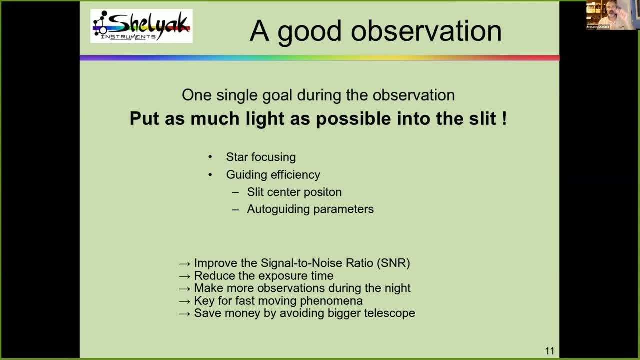 Because if the auto-guiding, if you don't have the right parameters, probably the mounts will oscillate around the slit And each time that the star is beside the slit there is no light that goes into the spectroscope. And this is some time which is lost. 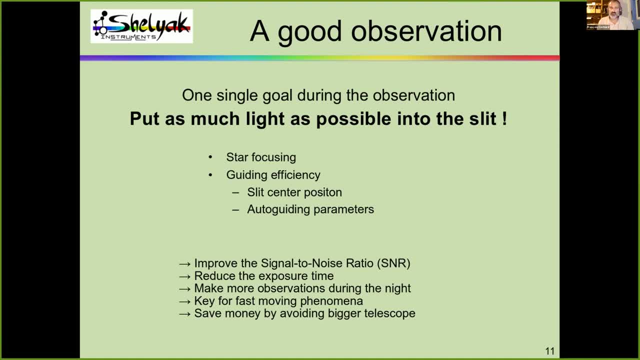 OK. so if you do that, if you put as much light as possible into the slit, whatever it is The size of your instrument, It means that you will improve the signal to noise ratio of your result. OK, so the spectrum will be less noisy if you have a good high quantity of light going into the slit. 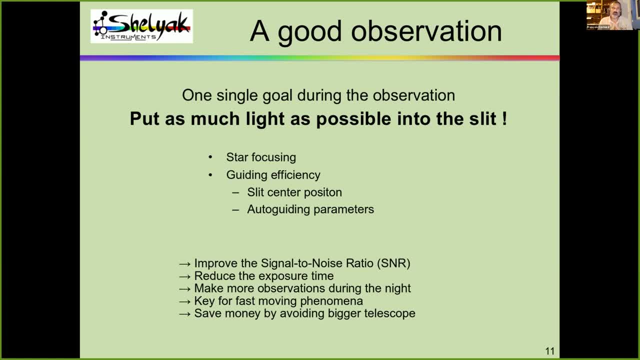 It will be less noisy And this is really the main quality of your observation. You can see that in another way. You can consider that If you do that, You will reduce the exposure time. I told you at the beginning, if your instrument is not properly set up or tuned at the beginning, 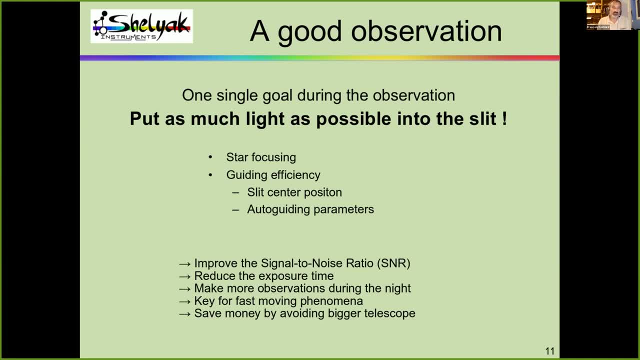 If you observe Vega, maybe it will take five seconds, Where normally it should take 0.1 seconds. So if it's only five seconds, we don't care. It's not a long time. But of course, if you go to a fainter star, if you have to observe it during 10 hours or 10 minutes would be enough. 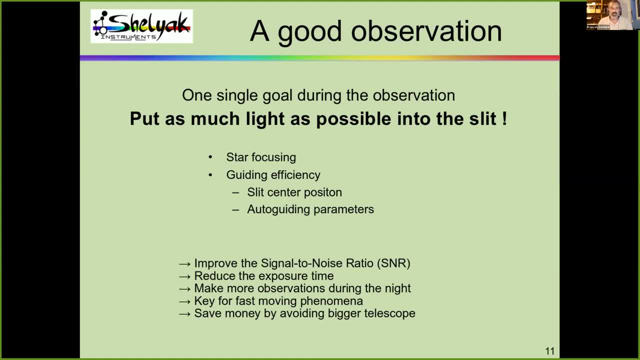 This is a very, very big difference. OK, And if you do that, you will make, of course, more observations. during the night, And also at the beginning you will not make a lot of observations, But when you start being productive and when you want to collect as much data as possible, it becomes important to know how many observations I can do during the night. 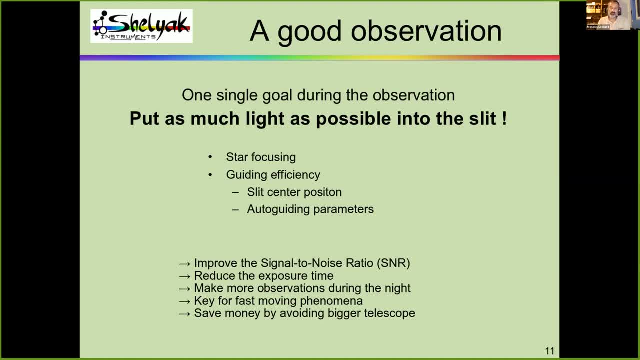 And if your setup is not tuned, you will lose time And you will lose observations. So you have some observations, some phenomena in the sky that are moving fast in two minutes. for instance, If you take the RRI stars, they are at some moment at the maximum, the Blaschku maximum. 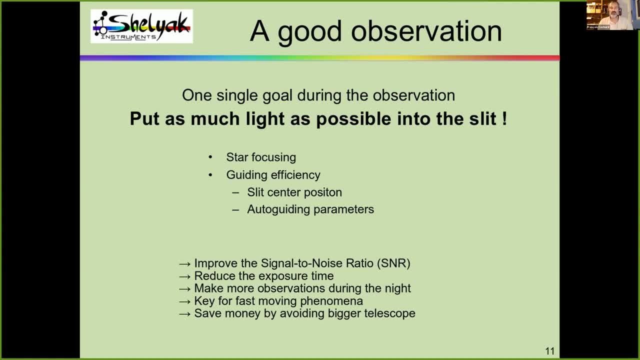 They change in a few minutes time range And in this case you are very limited by the time of the observations. So in this case also, you have to have the best conditions to have a better SNR. And again, another way to see this problem is that you may save money. 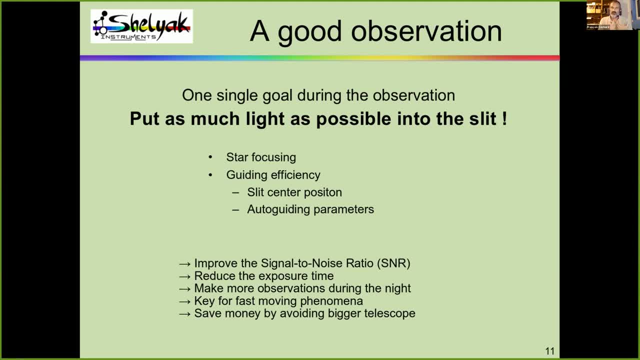 Because another way to compensate a bad tuning of the instrument is just to have a bigger telescope to collect more lights, And then you will also by increasing the telescope diameter. of course you will reduce the exposure time, But it's much more efficient. 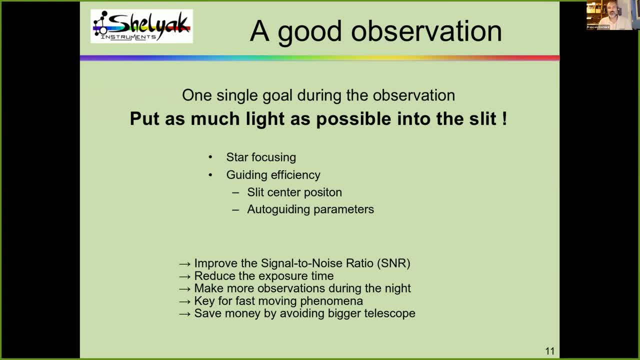 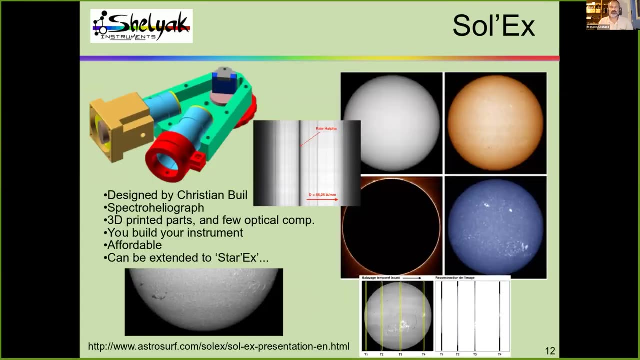 And it's less expensive to do that by tuning the instrument properly. Okay, Well, I still have, I think, very few slides. I want to talk to you about this SOLEX project. So this slide I've already shown it during the last webinar I did present some months ago about the SOLEX project. 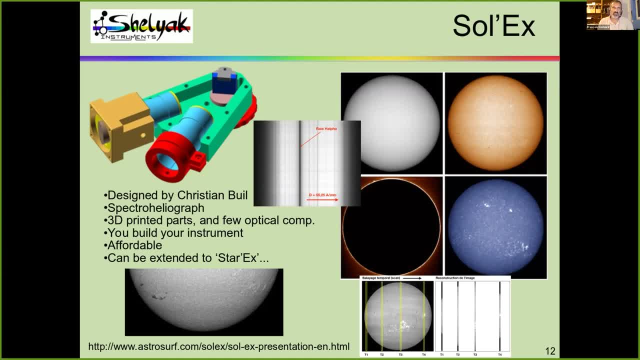 So the SOLEX project- This is a project which is proposed by Christian Grill And well within Celiac we do. we propose a kit of all the optical elements And this instrument is made by 3D printing. So you make your own instruments with the available STL files on the SOLEX website. 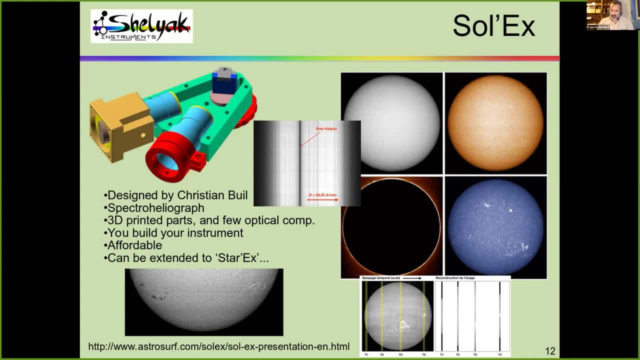 And we at Celiac we propose a kit of the optical elements To make a SOLEX And even a STARx. So the SOLEX is a solar explorer- It is made mainly to take images of the sun- And STARx is the usage of the same instrument on the stars. 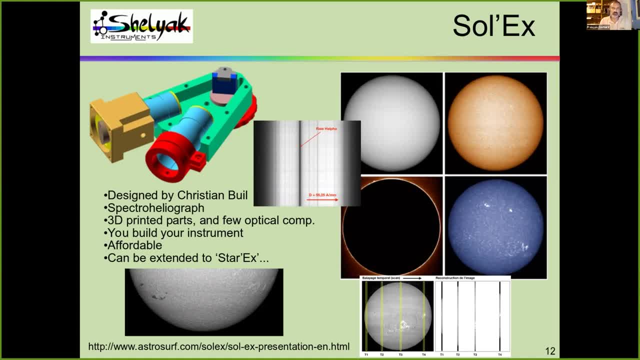 Okay, So we just had a guiding unit to make sure that we can see the star we want to observe. But this is exactly the same instrument And the idea is really to have something very basic, Very easy, That you make yourself, So you perfectly understand how it works. 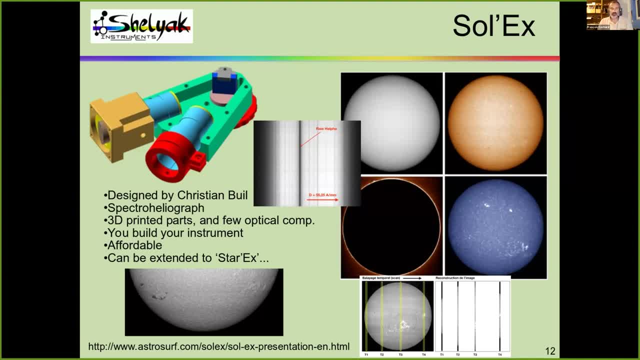 It is easy to build and to tune and so on, And it's a wonderful instrument. So, to take a solar image, in fact, we scan the sun And you can even have. well, we need a small instrument. A small instrument is enough. 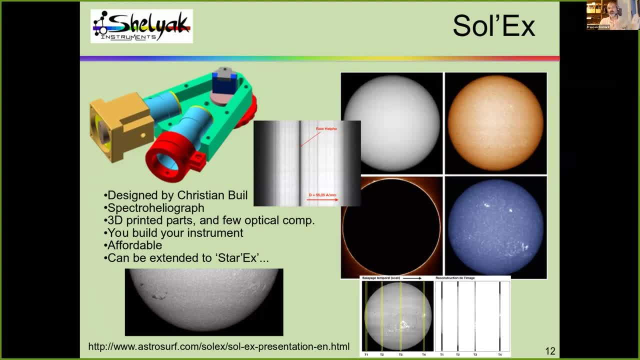 And you can just stop the mount and let the sun moving across the slit For a few seconds. Well, in this case, two and a half minutes roughly, And the idea is that you take a spectrum at any wavelength you want, Because you can rotate the grating. 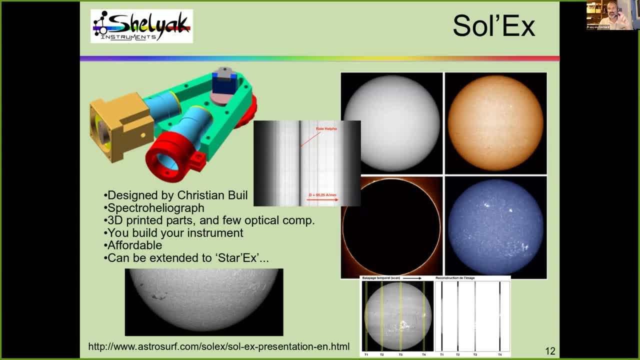 And then, after that, we rebuild the image that we extract in a given wavelength. Well, we scan the sun, So we take columns by columns And we use the software to rebuild the images that we have behind here. So this is a spectral helioscope. 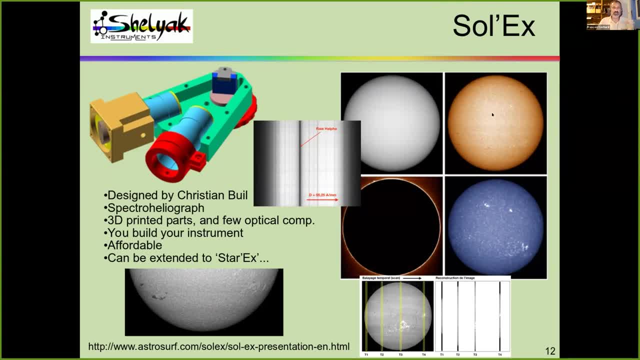 So the idea is to take an image at a very thin wavelength So we can even see the Doppler effect. If you look at some detail it's just incredible, And you can take images at any wavelength you want. So it's really a small fun instrument. 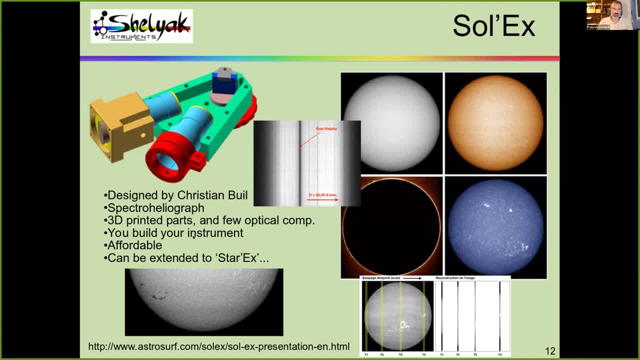 And you make it yourself And, of course, it is affordable. So I've put the website, The website, here, if you're interested. Really, I think that for the AVSO it is something that is incredibly interesting to start in spectroscopy. 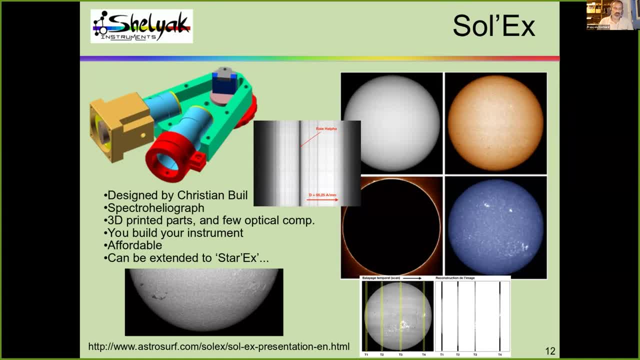 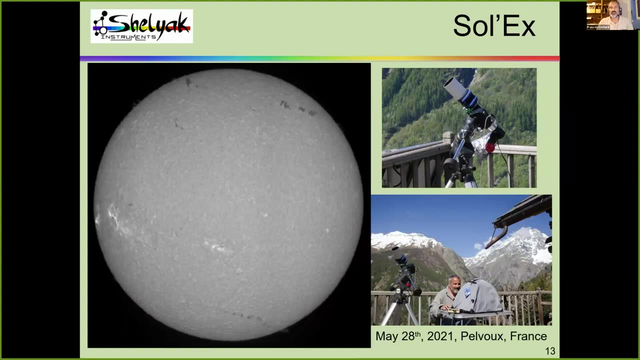 And at the beginning we start by taking sun images And afterwards we can switch to D-stars. Well, by the way, I've built my own Solex And we have this small instrument. And again, this is my old mount. 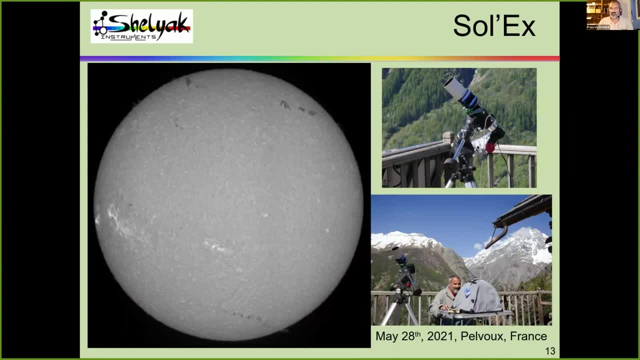 And so the Solex is here. We do protect it with aluminum paper to make sure that there is no what this is, to protect from some light leakage And to protect it also from the heat of the sun. So I was lucky because I had some great opportunity to observe in wonderful conditions. 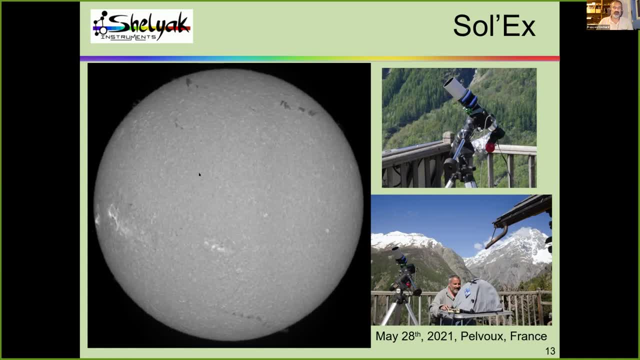 It was in last May, And here is my own pictures that I took with the Solex using the Inti software, which is a software in which you just have to put your file that you've taken during your observation And all the processing is done totally automatically. 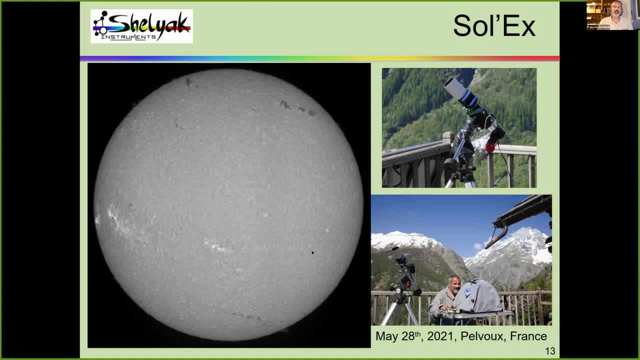 So, really, the image I show you here is what goes out from the Inti software With absolutely. I just have to select the file and to click on OK And one button runs And that's it. That is the result. It's incredible. 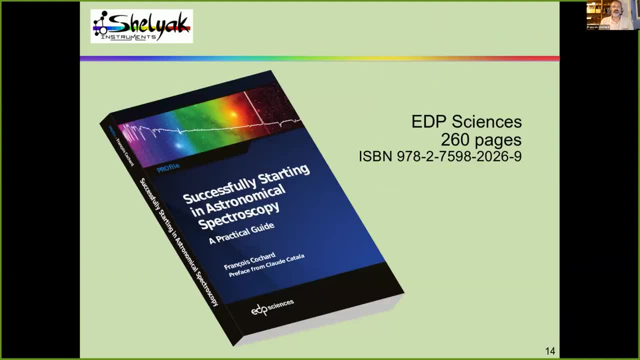 OK, I've finished. So, Lorraine, you did talk about it, But I've written a book some time ago in which you can have a lot of information on how to start spectroscopy, And, of course, a lot of things that I told you today are in this book. 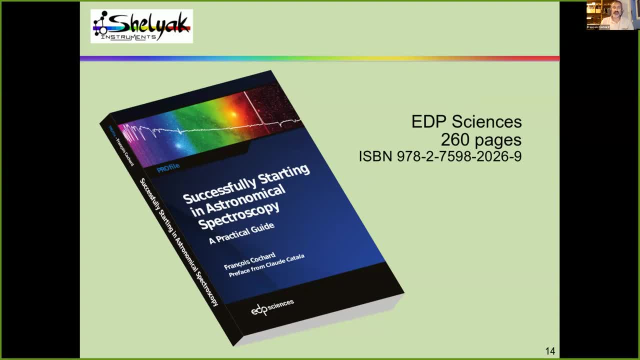 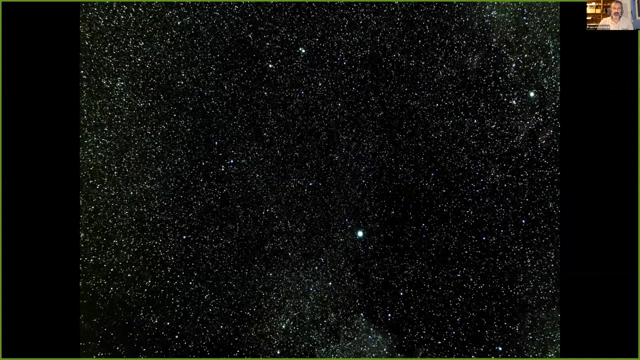 OK, I think I'm done. So now here is our job. This is a picture that I like. This is in the Milky Way, Of course, close to the well, I don't remember exactly. This is the Cygnus, one star Cygnus. 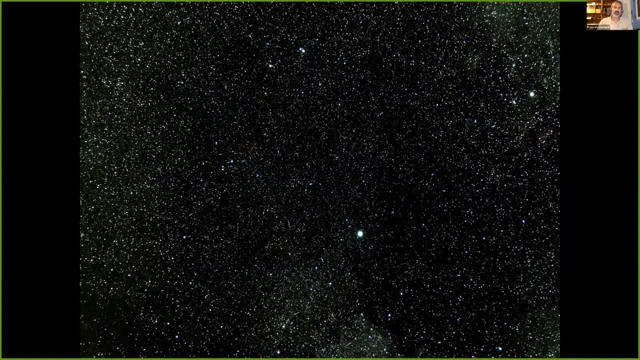 Each of these stars is interesting to look at. So you know that if you are doing imaging in a single image, you have many, many, many stars. Now let's work. Let's work all together to take every single, each single star in this image and extract the spectrum from this image. 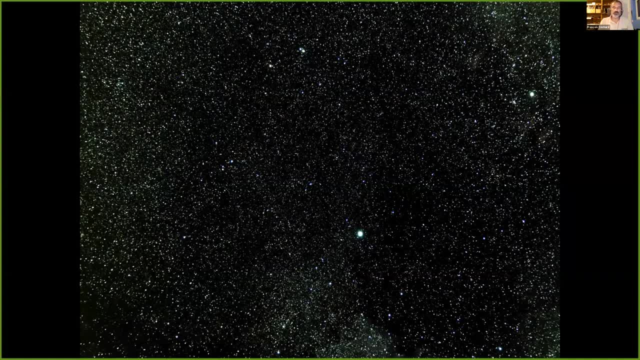 It gives you an idea of the huge and wonderful task that we have in front of us. OK, Thank you very much. Thank you for your attention And, of course, I would be happy to have some questions and discussions. Thank you very much, Francois. 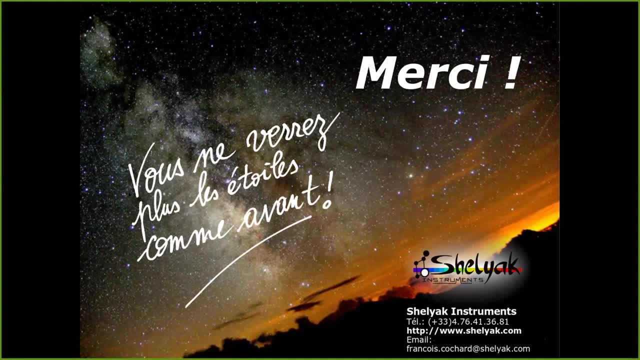 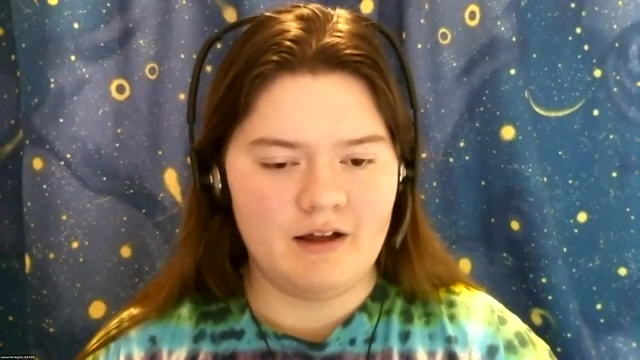 That was excellent. Can you hear me? OK, Yes, Perfect, Yep, OK Great And OK good. My video still works. So I did have a minor technical issue about halfway through your presentation. So there were a couple questions that I think may not have come through. 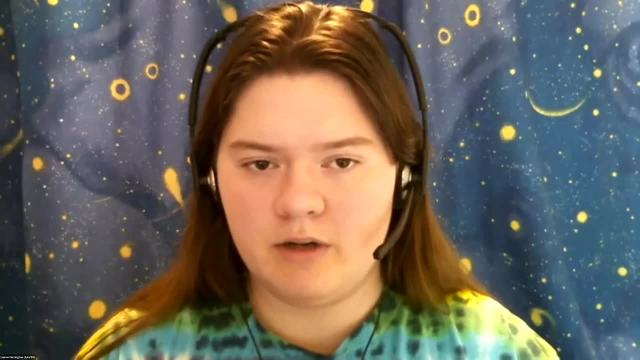 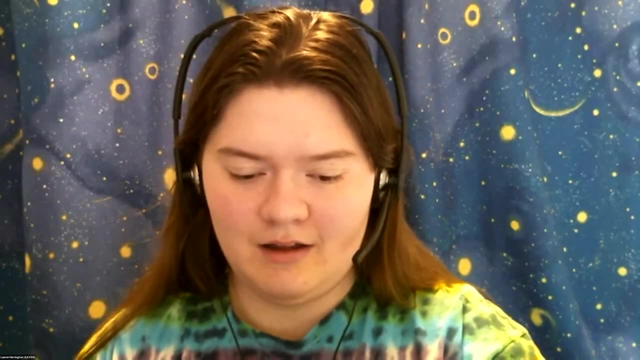 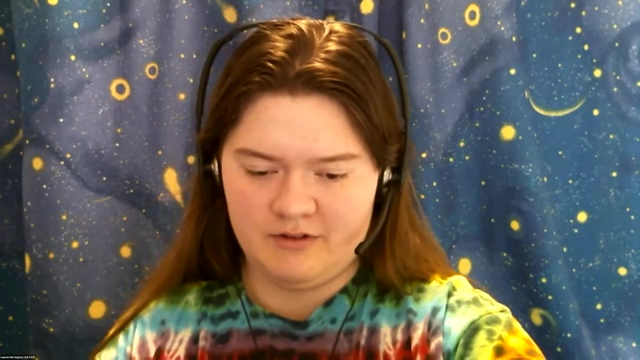 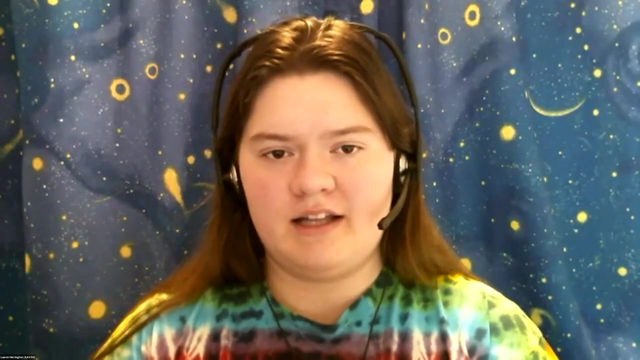 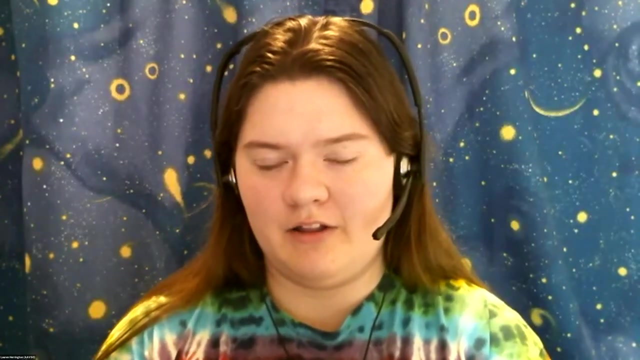 If we get to the end of the Q&A and one of your questions was simply not addressed, please just go ahead and submit it again. So let's start out with a question that was there before the Q&A box got clear for me, which was with a: or is a star analyzer grading sufficient for recording the redshift of quasars, or would a different instrument be needed for the job? 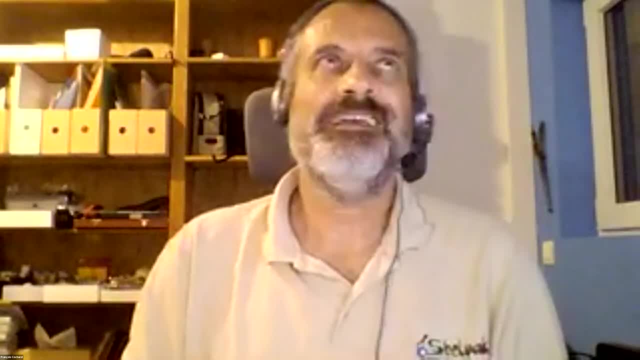 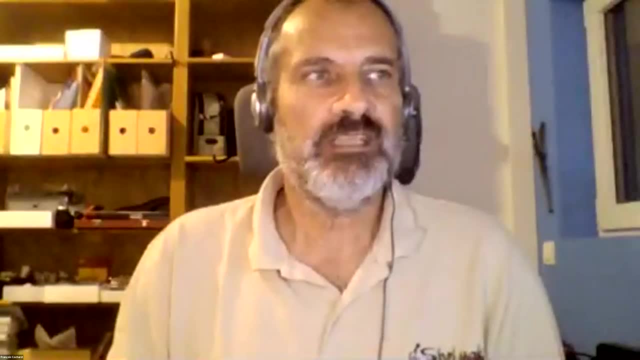 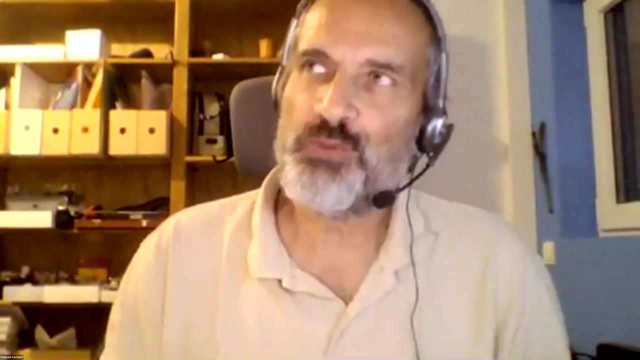 Well, it depends. Well, it's. my first reaction would be maybe not, But I know I'm very because. well, maybe, Lauren, you would be able to reply to this question better than I do, because I'm always surprised by what we can do with a star analyzer. 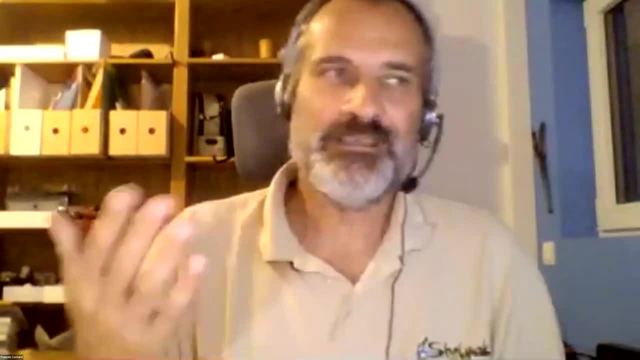 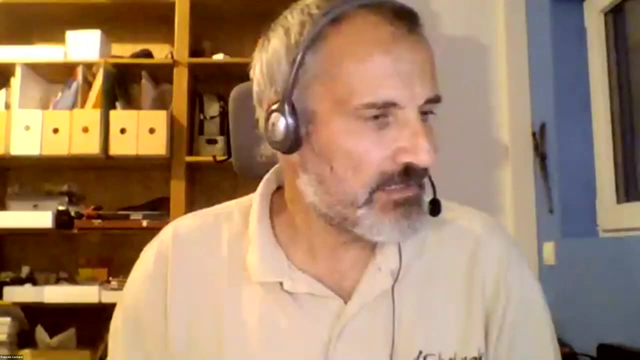 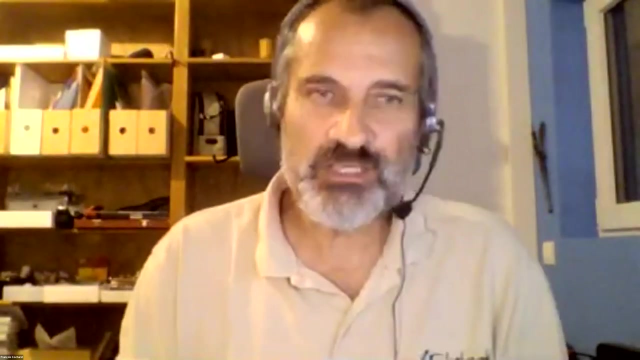 And what I can tell you is that a star analyzer is not a slit spectroscope, And what I thought about today is about mainly about slit spectroscope. And if you use a star analyzer, for instance, you cannot use a calibration light to do the calibration. 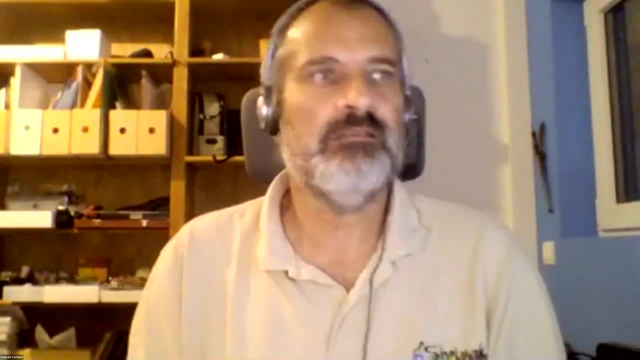 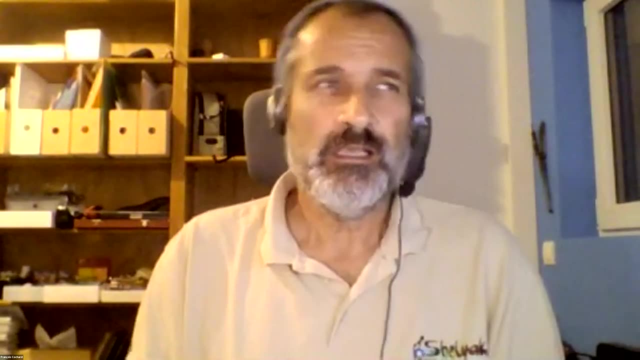 Well, for technical reasons, I could explain how to do it. So you may have some difficulties to have a very precise wavelength calibration And when you want to measure redshift, In fact of quasars, Of quasars Or anything else, 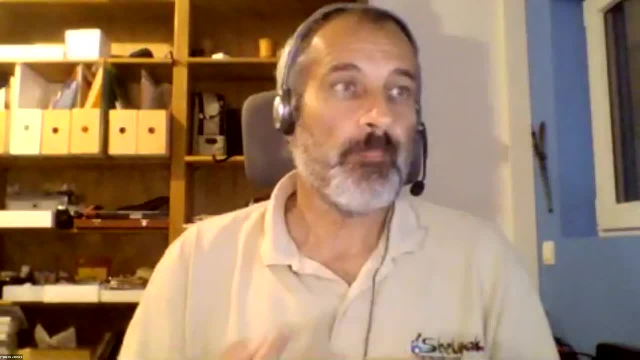 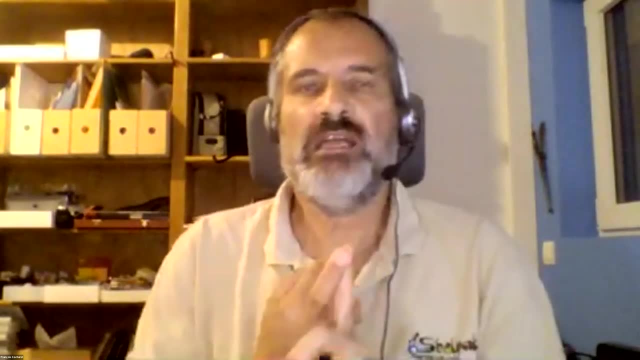 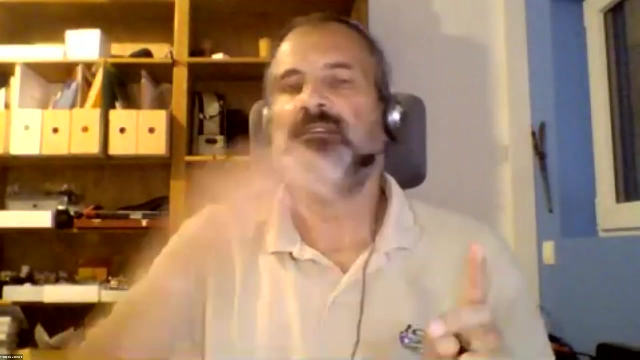 You have. you need two things: You need to have a very good calibration And also, depending on the object, you have to have a very good, good resolution. So the case of the quasar is a little bit different, because the quasar has a very high redshift. 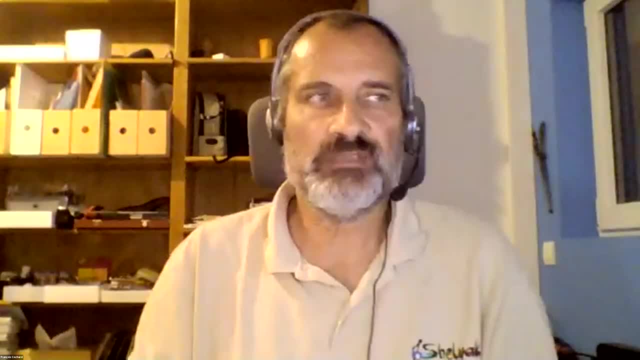 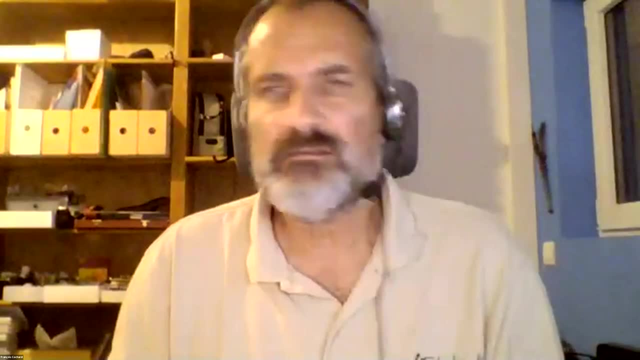 So it's, it's obvious, And you don't need a high resolution. So well, I cannot tell you. Probably, probably, yes, I think that the 3C, 3. 3. 3. 7.. 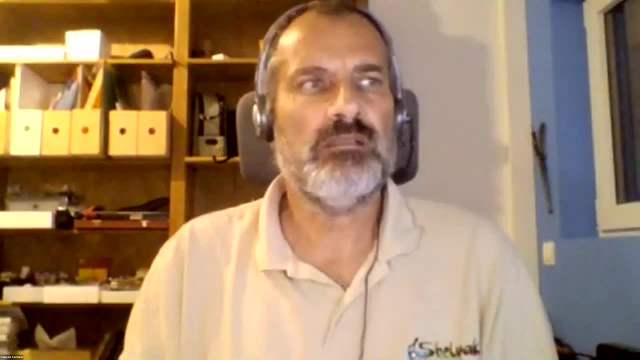 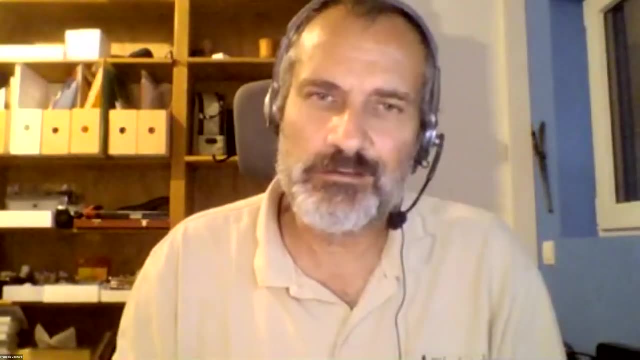 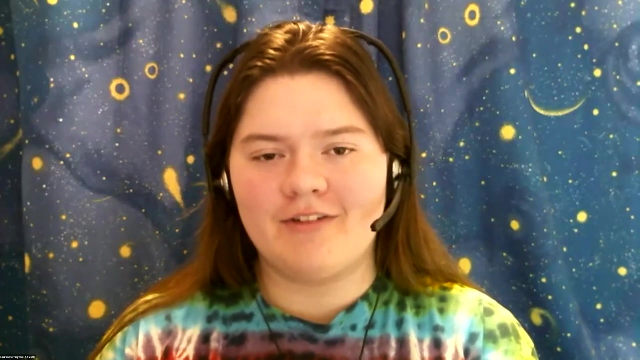 3. Quasar, The most well-known one, has been observed with the star analyzer. Do you know it? Maybe you did it, Lauren. I have not done it myself yet because I can't do it with a non-tracking telescope, But I have seen several examples of amateurs measuring quasar redshifts using tracking telescopes. 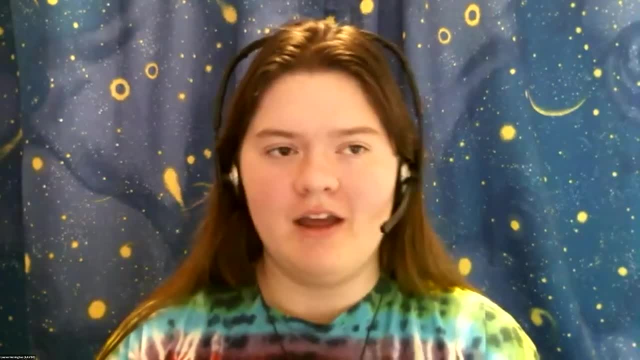 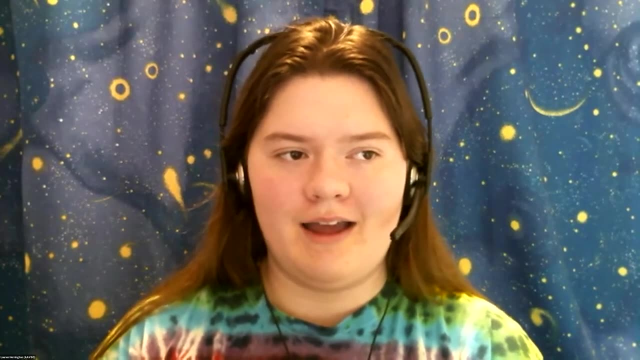 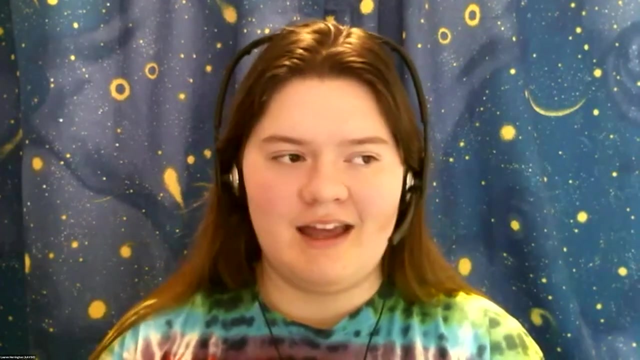 It seems like for the brightest, like you mentioned, 3C273.. Yeah, Biala Sarte is another. For those it's fairly easy because, as you said, the redshifts involved are so high. As long as you can get enough exposure time, probably 20 minutes or more of exposure time at a low dispersion, then yes, it's, it is quite possible. 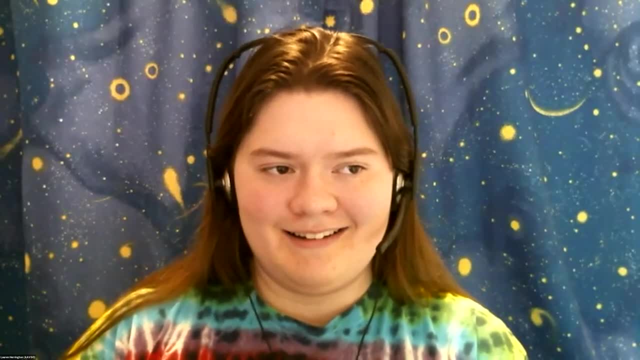 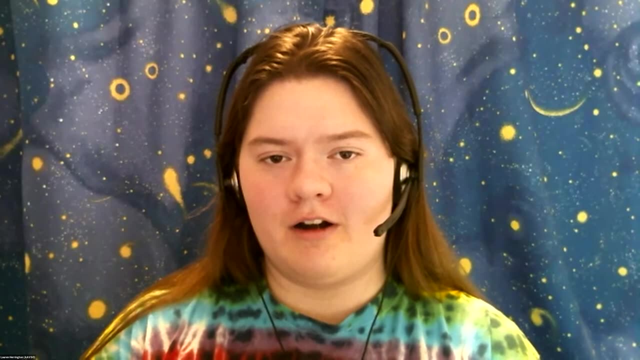 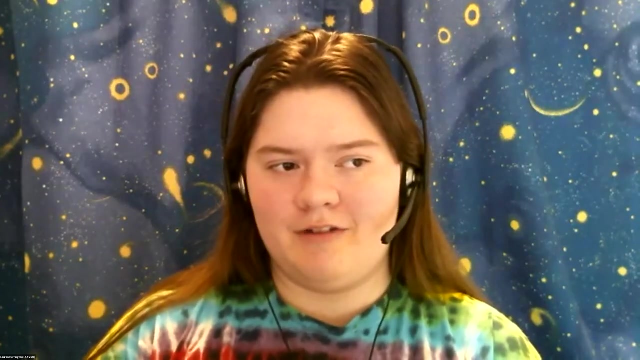 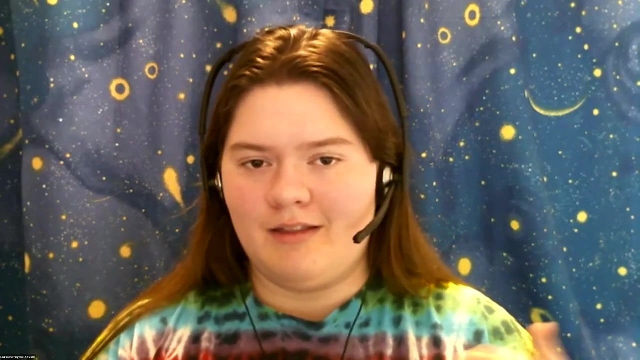 You mentioned that you can't use a calibration lamp. That's correct And that makes it tricky to measure- measure redshift- when you don't have a zero order star as reference in the frame. Generally, at star analyzer resolutions you can build a reusable calibration for given equipment, set up by shooting a star that's like Vega or something where you can easily measure the central line wavelengths. 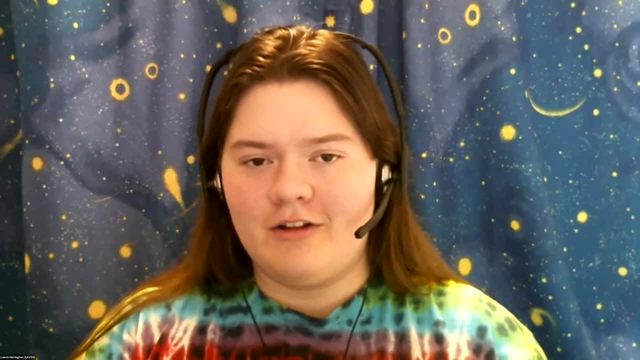 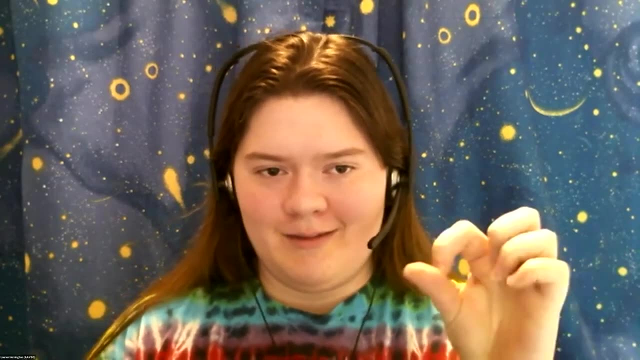 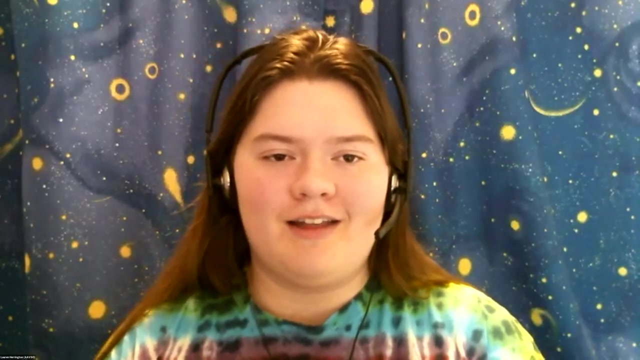 And then the resolution of the star analyzer is so low, to begin with you can assume that you're not seeing any radial velocity effects, And then you can use the zero order star image next to the spectrum as your calibration point. So you probably knew that, but I'm saying that for the other people here. you can use that technique to measure quasar redshifts. 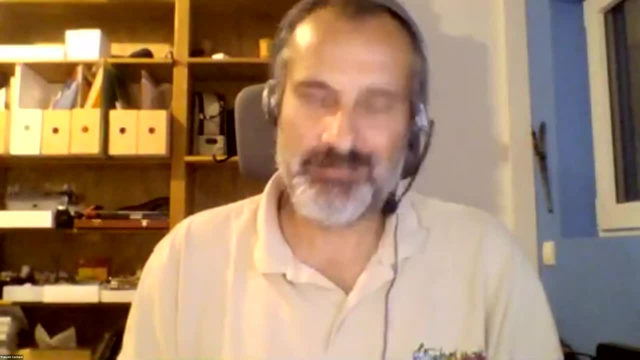 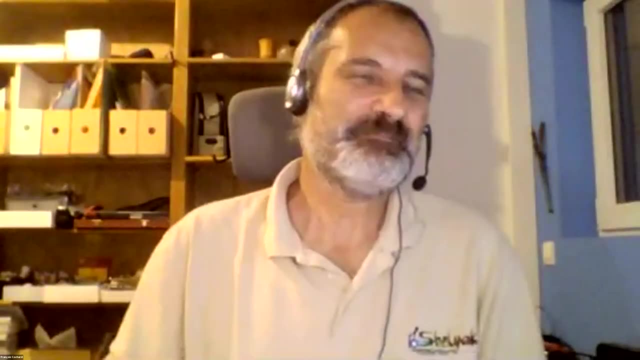 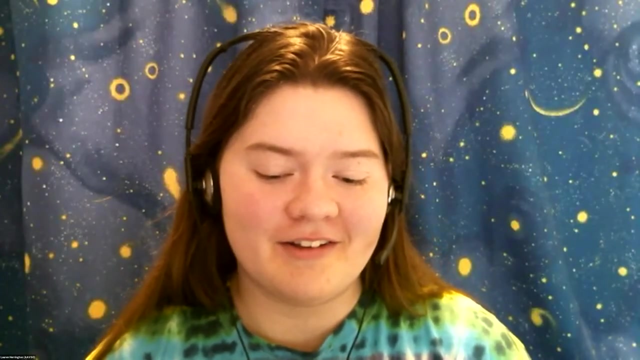 And I like the way you said. you have not measured it yet, Not yet. Hopefully soon. Yeah, All right, Okay. So next question comes from Patrick Cavanaugh, who asked: is it okay to spend some nights doing spectroscopy and other nights astrophotography or photometry? 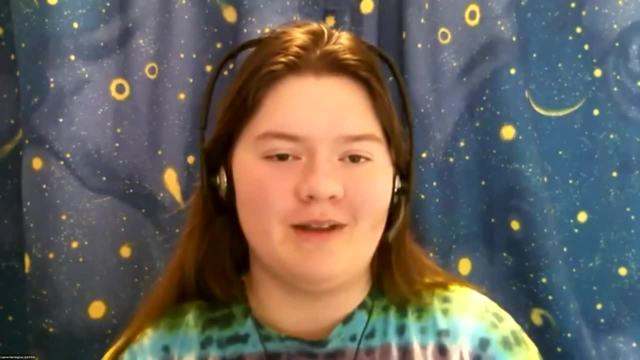 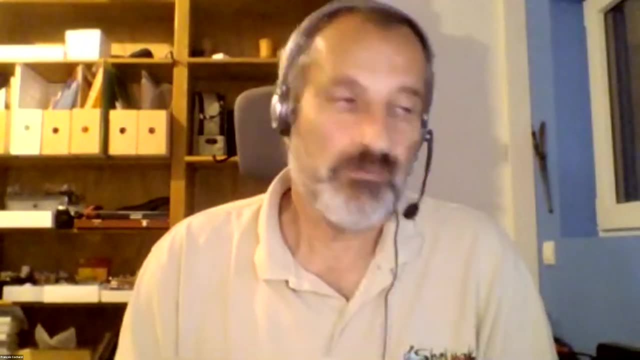 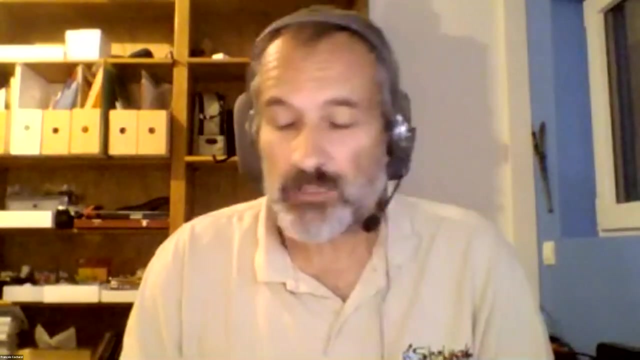 Yeah, Presumably. is it easy enough to switch between the two? Yes, Well, it all depends on your equipment. Well for sure, This is very useful, in fact, to have imaging and to do photometry in parallel to spectroscopy. Because if you do photometry, you have the overall magnitude of the object you want to observe And if you are doing spectroscopy, in parallel, you can see how this energy is spread out along the wavelengths. Anyway, maybe your question is more technical regarding so, can I switch from one instrument to the other? 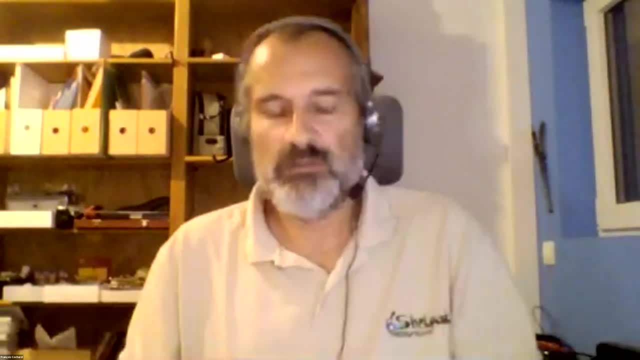 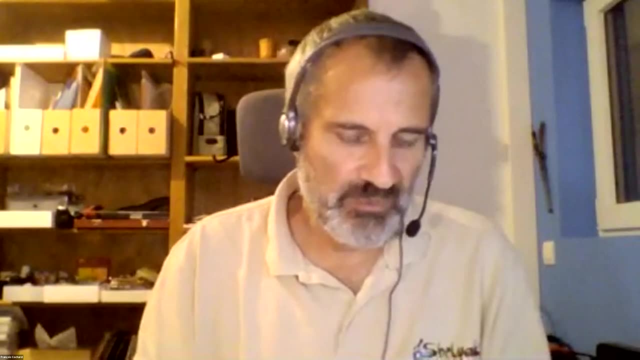 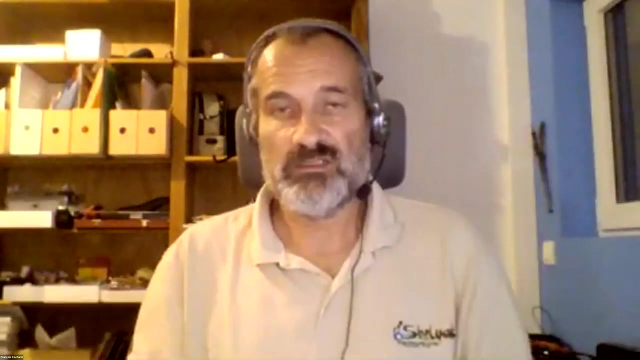 I would say, if you remove the spectroscope from the telescope and replace it by your acquisition camera, your photometry or imaging camera, that's not a big deal. But you have to rebalance, you have to manage the cables and so on. 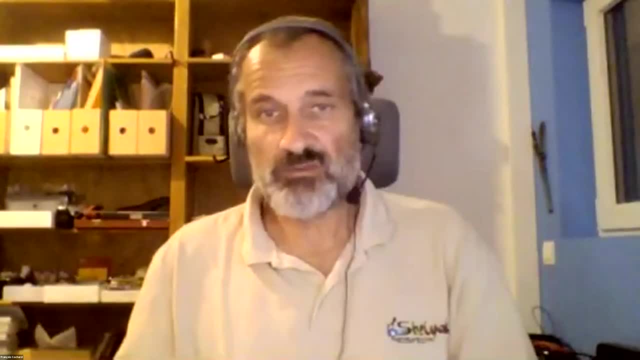 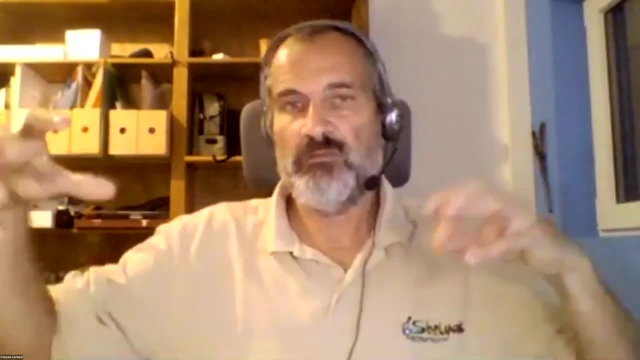 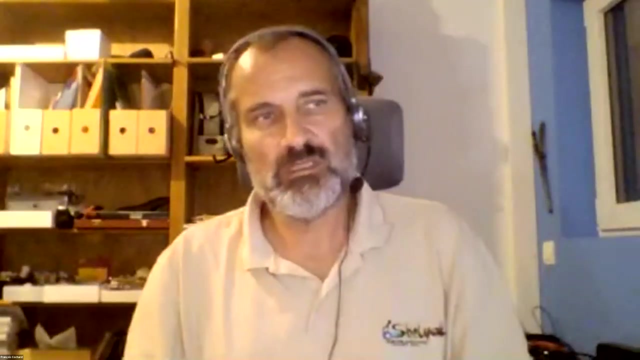 So I know that there is a lot of people who have a dedicated instrument for spectroscopy and a dedicated for photometry or imaging, And you also have people with bigger instruments that have multi-port system on which they can put several instruments, And then they have one spectro in a port, one camera in another port, and so on. 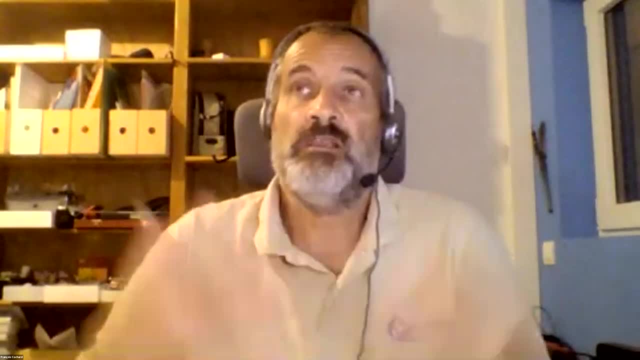 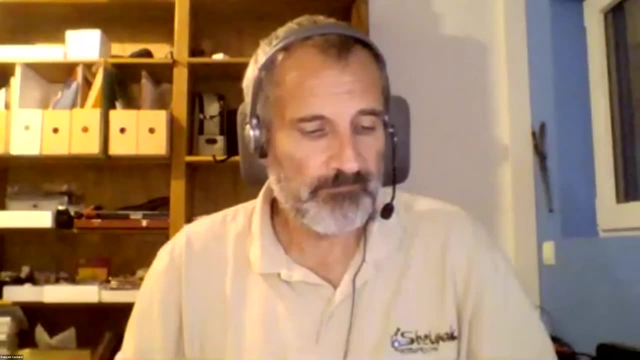 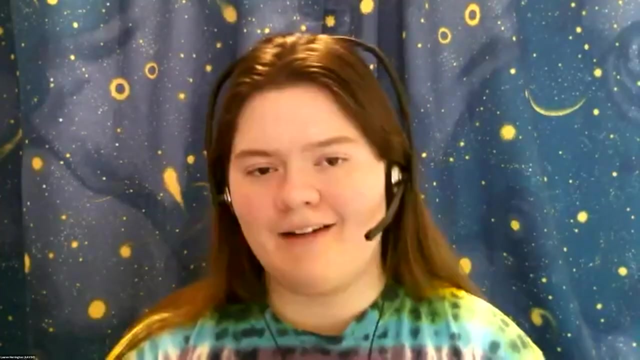 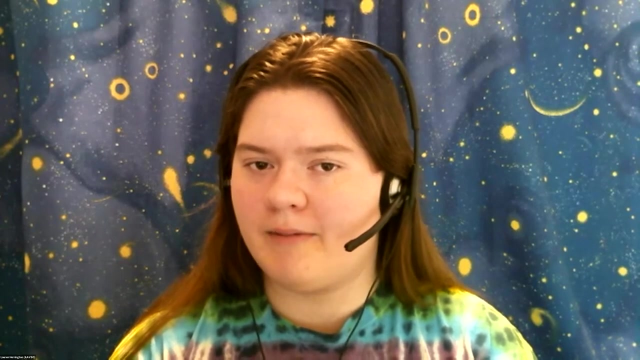 So you may have anything from any configuration, But of course you can say: one day I observe in spectro and the day after in photometry, And this is again scientifically useful, Thank you. To add on to that, I believe that I've heard of amateurs doing spectrophotometry using piggybacked telescopes like a smaller piggyback telescope to do the photometry. 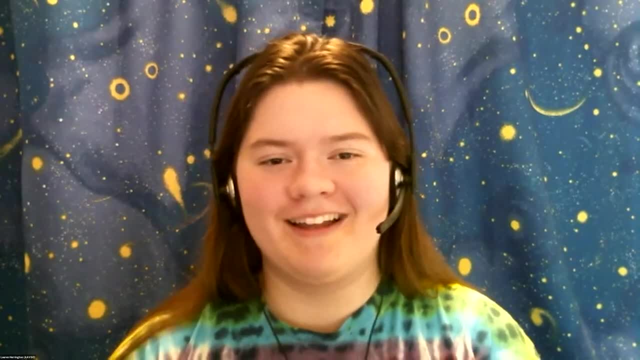 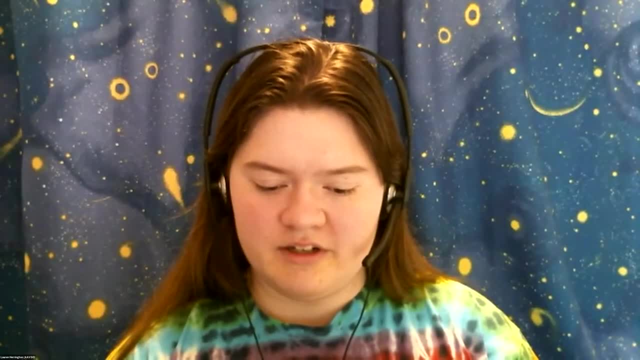 Yeah, yeah, Well, in this case, the advantage is that you really can do the same at the same time. Yeah, yeah, Well, in this case, the advantage is that you really can do the same at the same time. The next couple of questions that we have here. 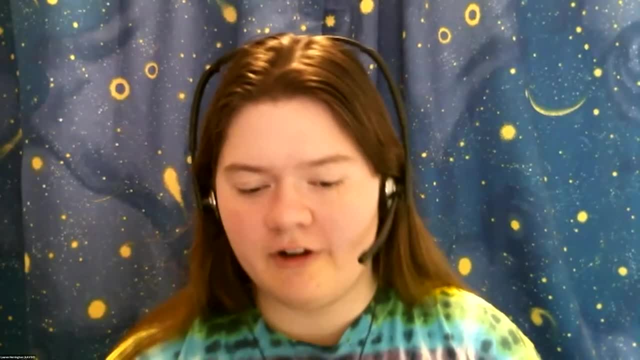 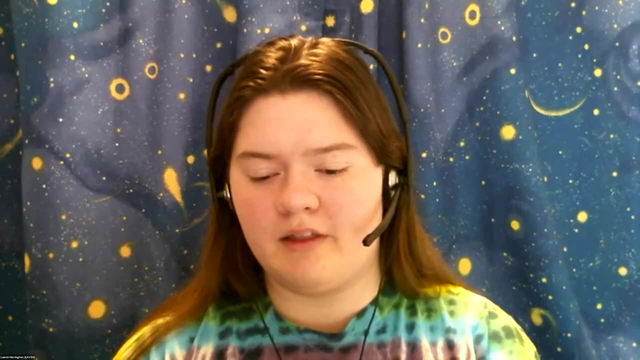 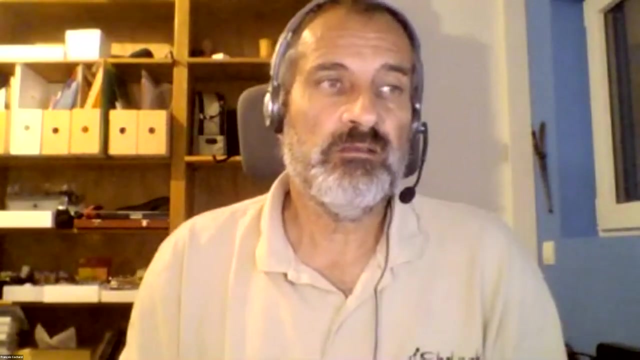 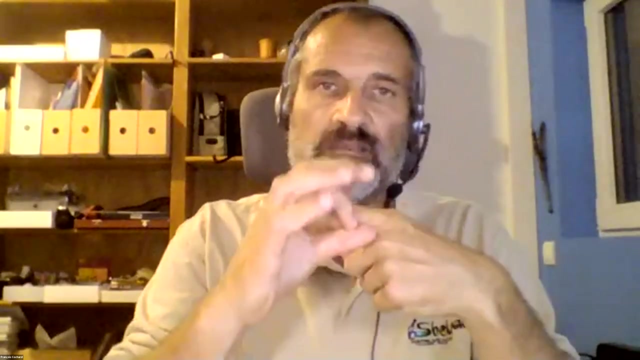 are about guiding, So Nathan Crumb had asked what is the best way to autoguide when the star is being split apart by the slit. This is a good question, In fact, of course, when you have the star across the slit. 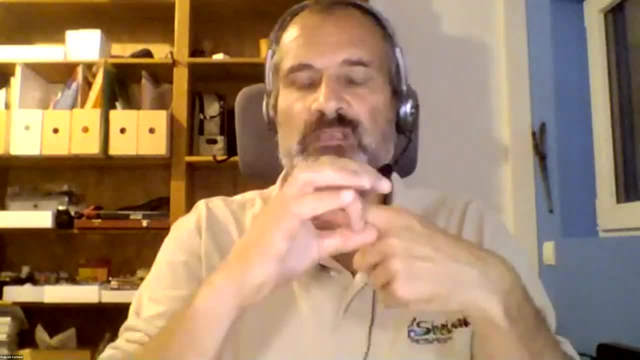 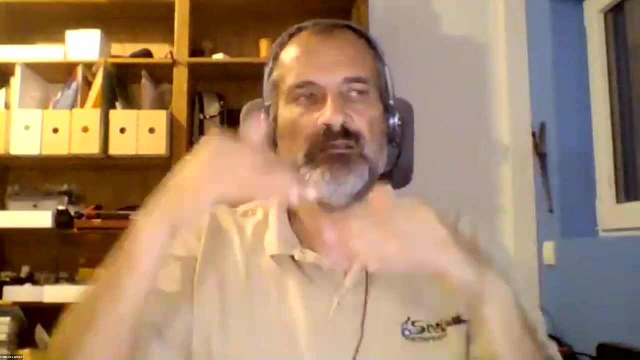 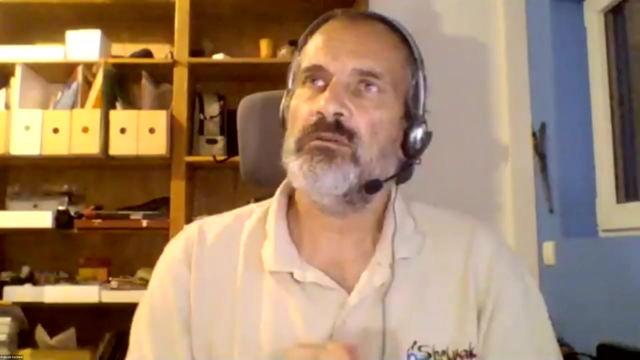 in fact the star almost disappears in the slit, But in practice we always have some light, So we have the wings of the star that are still visible around the slit, And I know that a few years ago there was some system for the autoguiding. We have specific algorithms that were able to manage the star split by the slit. As far as I know today, I think that nobody cares about that. You just use the autoguiding software, as it is even for a normal star, and it works perfectly. 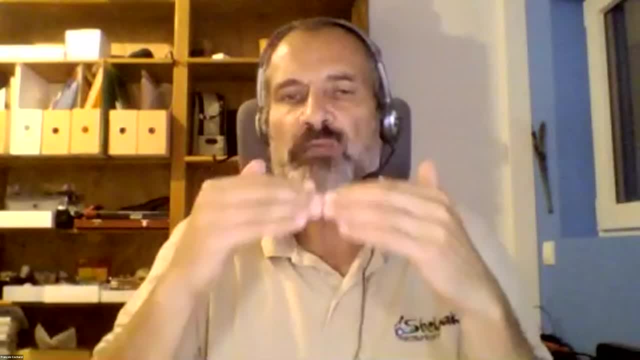 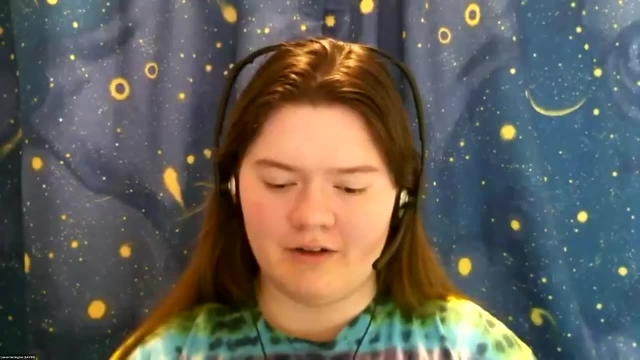 And you don't have to care about the fact that this is not a problem, in fact, for the autoguiding process if the star is split by the slit, Interesting Thank you. I would say that, in fact, the fact that the star is split, 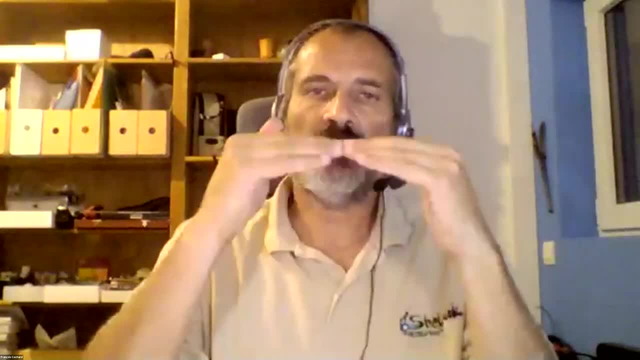 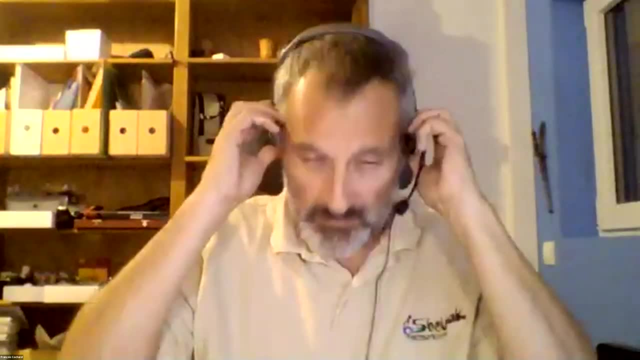 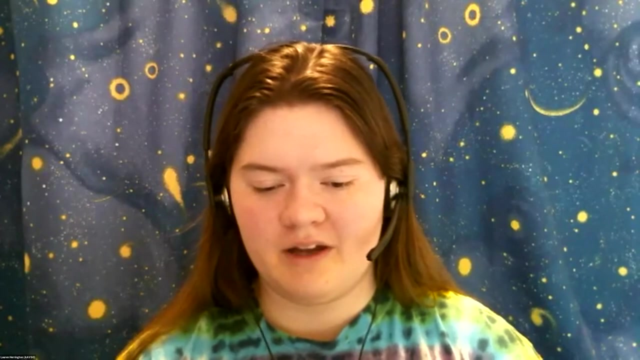 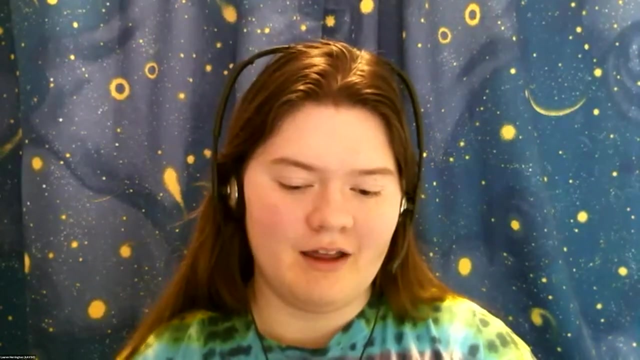 by the slit Increases the sensitivity for a misalignment of the star, So it even improves the system. Very interesting, Thank you. So the next question about guiding comes from Patrick Cavanaugh, who had said that for bright objects he assumes that a guide scope is not necessary. 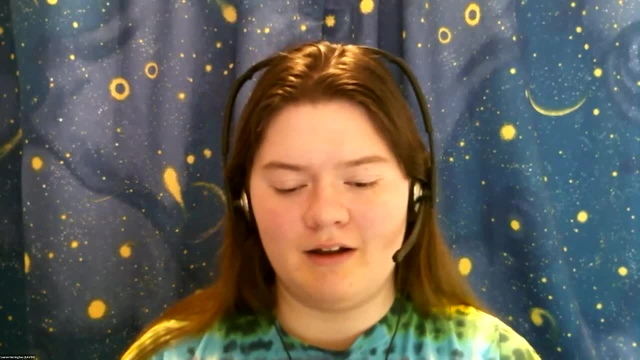 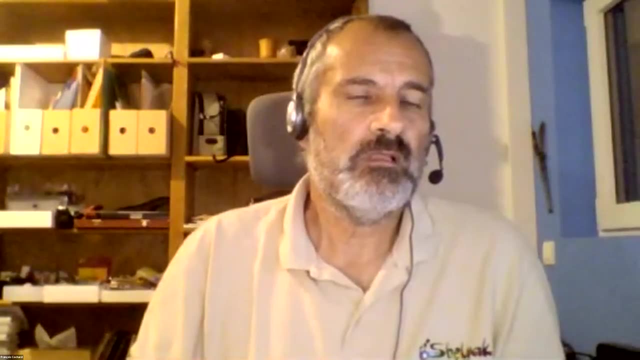 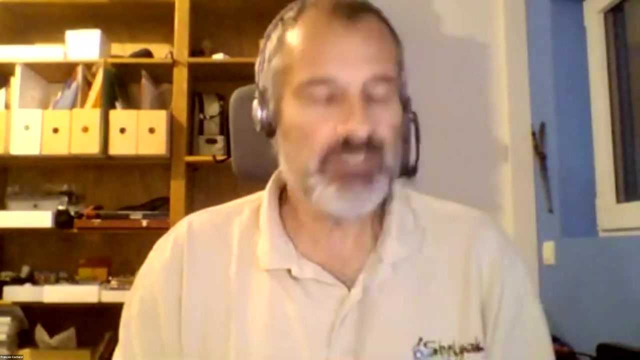 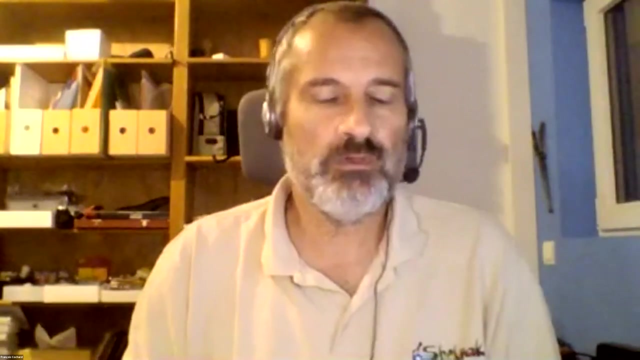 And he'd like to know where is the borderline between using and not using guiding programs like PHP? Well, there are two things. There is one thing which is, of course, the plate solving Today. it's very useful to make sure that you are pointing at the right star. 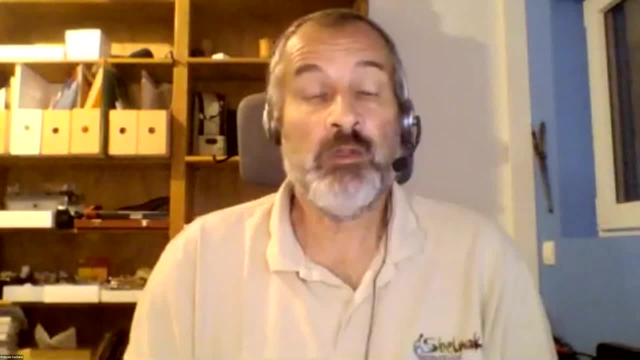 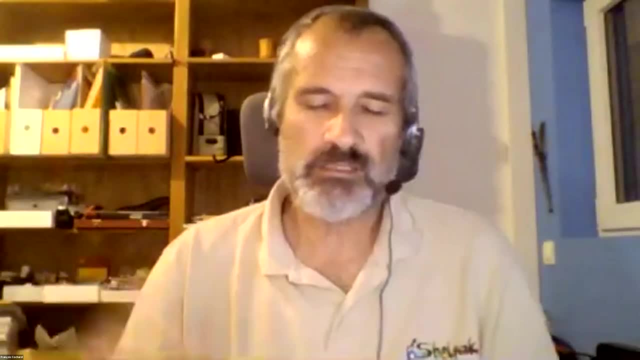 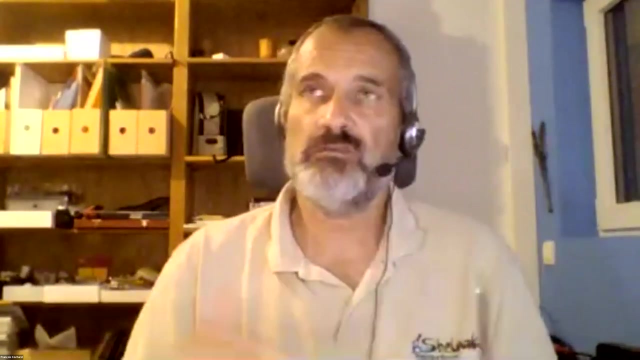 And it works perfectly And, generally speaking, it helps to control your mount And with this plate solving in the guide scope, you can do a t-point model to have a very precise pointing of the mount and so on. So it's really a wonderful tool. 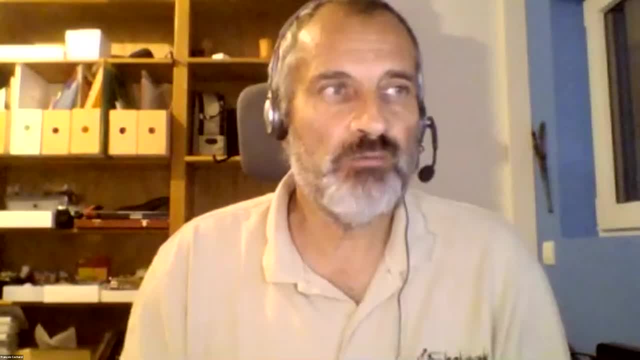 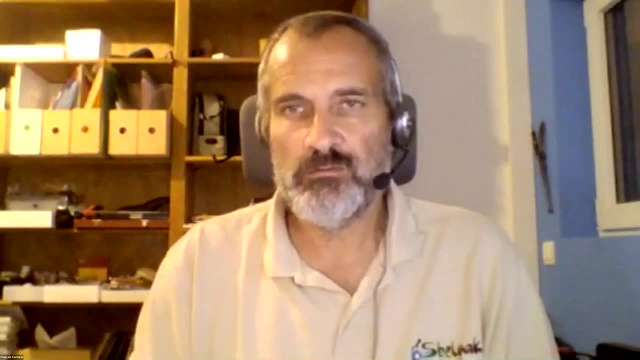 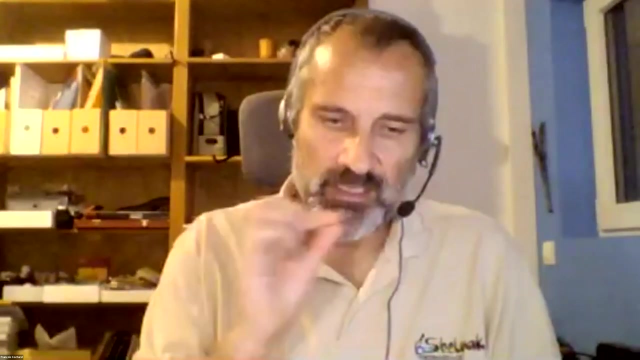 And I know I'm very impressed by the plate solving, how it helps to point at a star And with this system it becomes very difficult to observe the wrong star. In fact, it's very efficient Now having a A plate solving system to point at the right star. 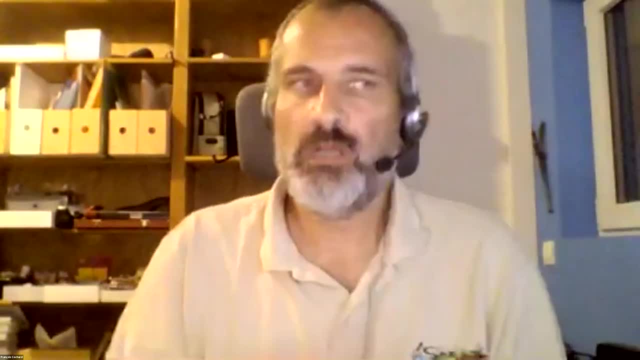 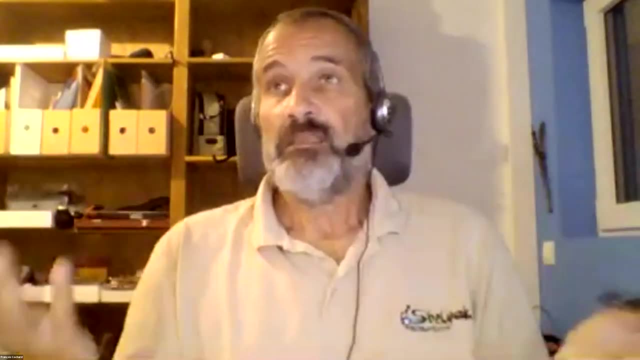 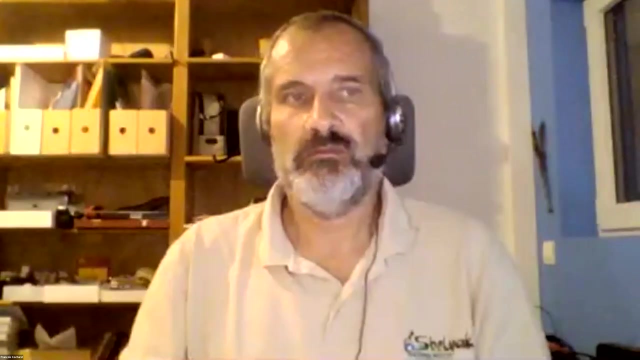 doesn't mean that you don't need to use a guiding software, like PhD, for instance. It's always important to have a guiding system. Again, it depends If you have a very good mount, if you have a wonderful t-point model for the mount control. 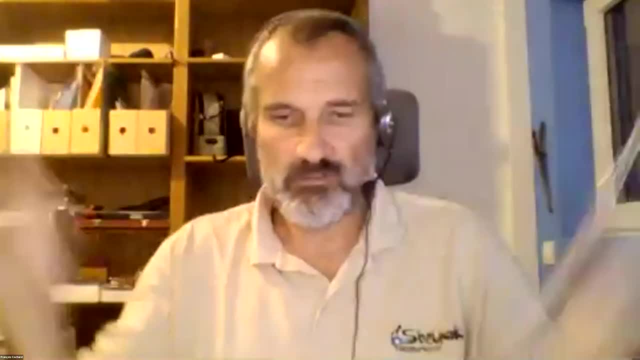 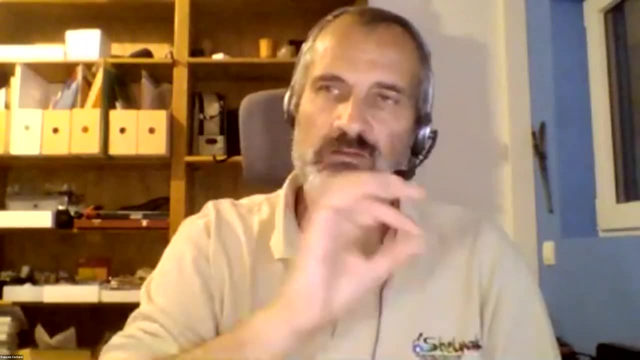 and if you have short observations, say 30 seconds, one minute, maybe you better have not, not to use the guiding, the auto-guiding, Because in this case the mount will have a very smooth movement where the auto-guiding may. 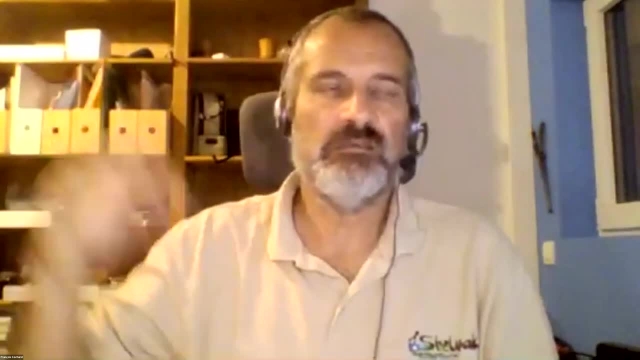 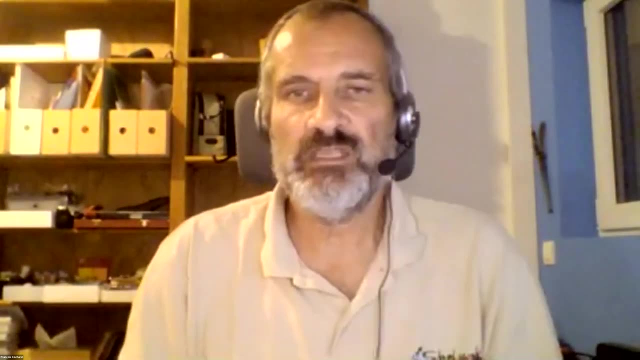 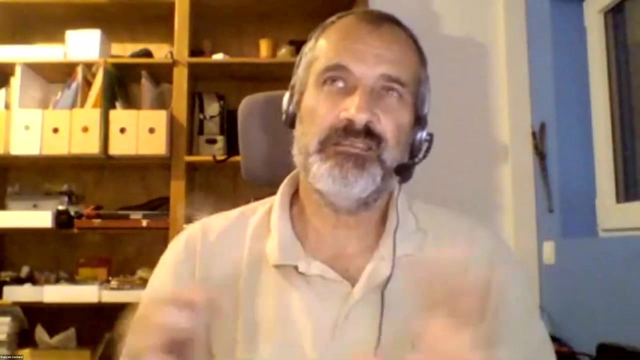 have give some oscillations in the guiding, So it may help, But generally speaking, you still have to have the auto-guiding ready and properly tuned. OK, This is something that really changes nowadays, because we can access to one. There are wonderful mounts and wonderful tools. 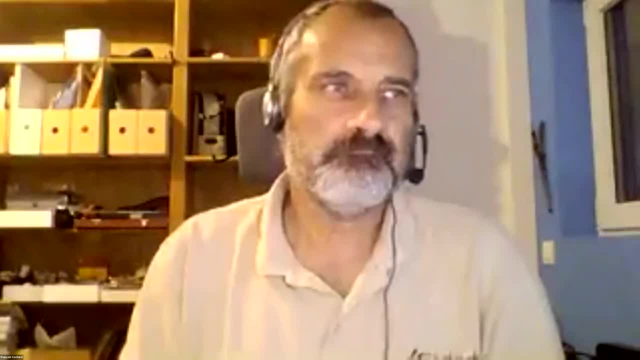 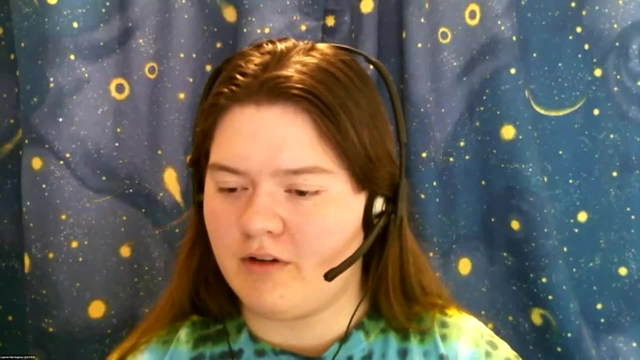 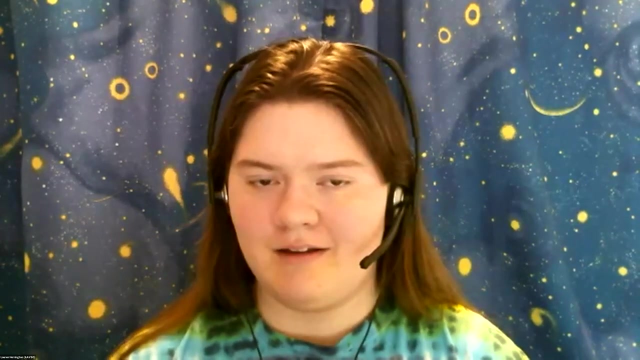 So this is changing a little bit, Thank you. The next question comes from Jason Adamic on Facebook, who had asked: is being very accurately polar-aligned essential for spectroscopy? So again, what is important, What is important at the end, is that you 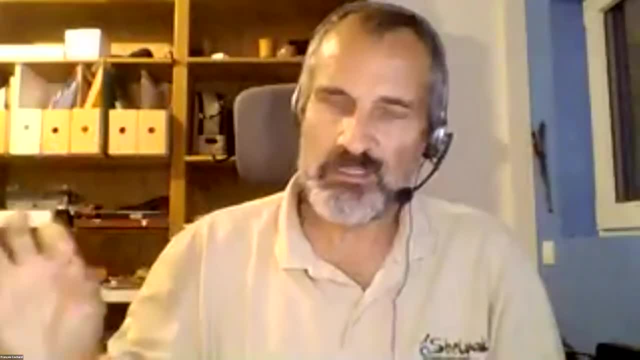 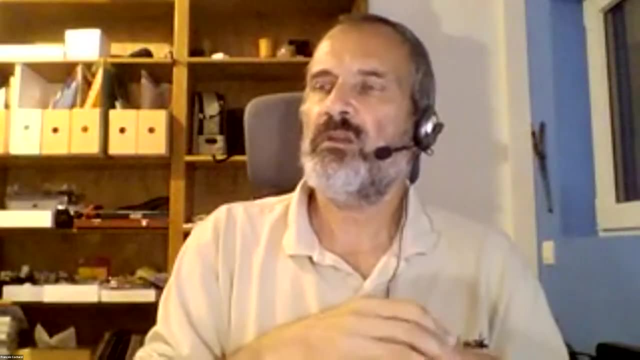 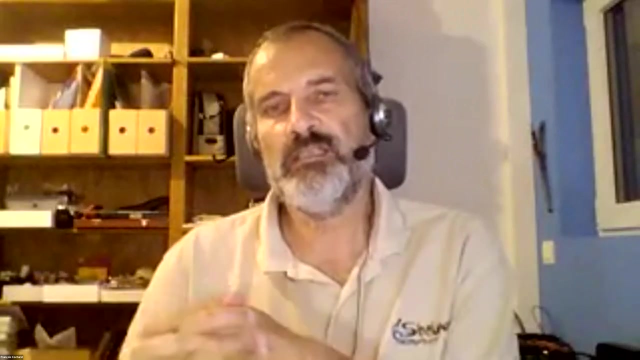 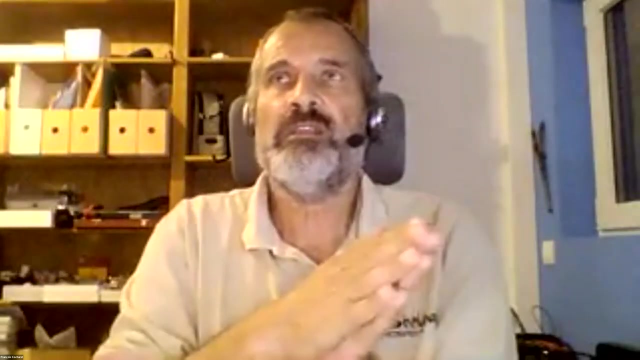 put as many photons as possible in the slit So you can, in some ways, the poor mount alignment can be compensated by a good tracking and auto-guiding system. OK, And even depending on, in some situation when you have it happens that you. 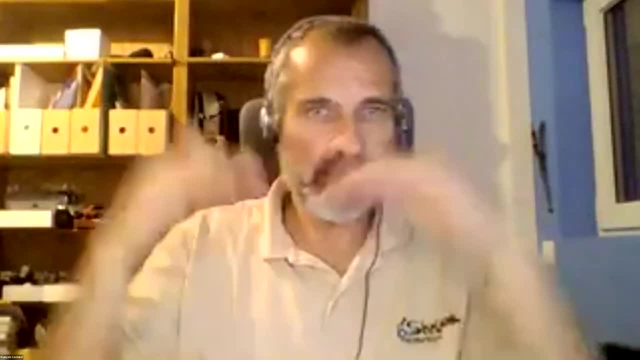 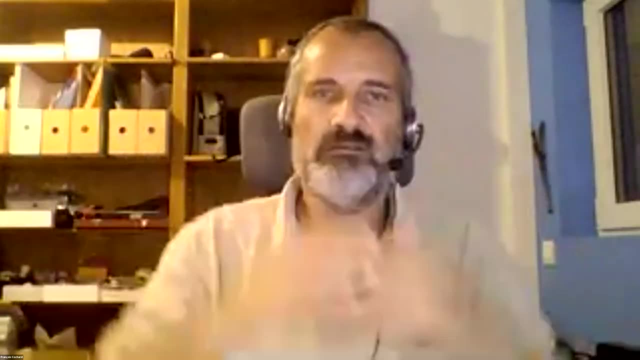 have some gap in your mount, in the delta axis of your mount, and then the guiding will make some, some, some, you know, some random movement vertically. in this case it could be better to have a small misalignment of the mount. 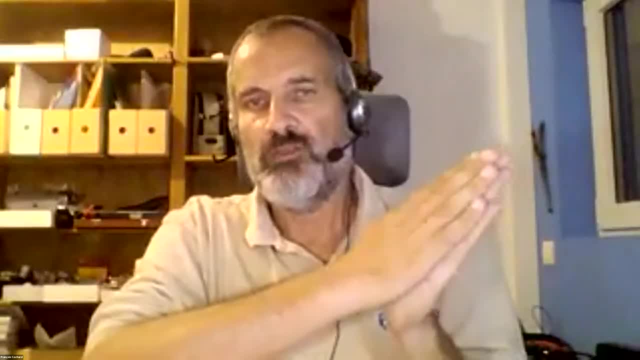 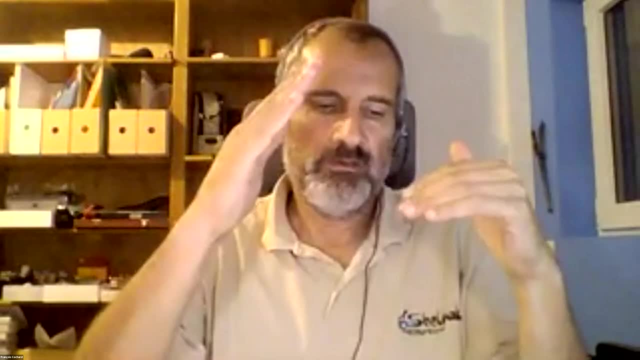 and use the auto-guiding to compensate for that, Because if you do that the mount will always compensate in the same direction And then you will avoid having a high large movement of the mount. But again, I know I did have this problem with my old mount. 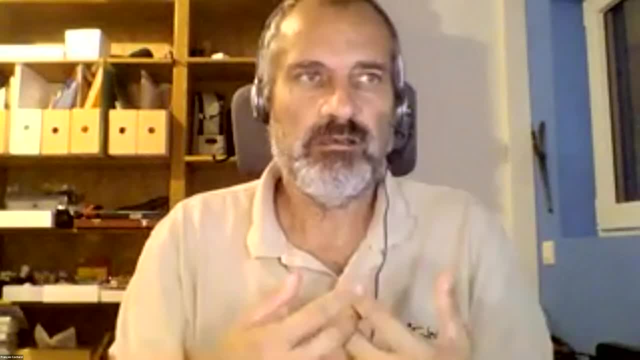 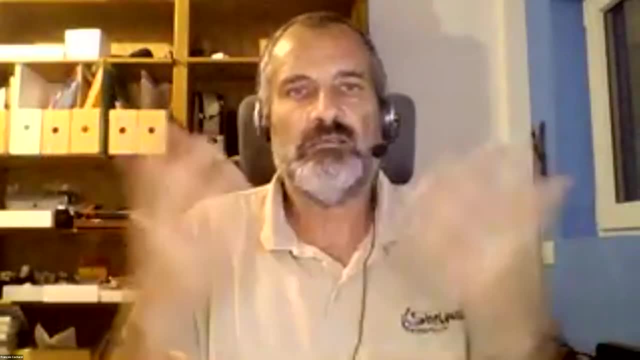 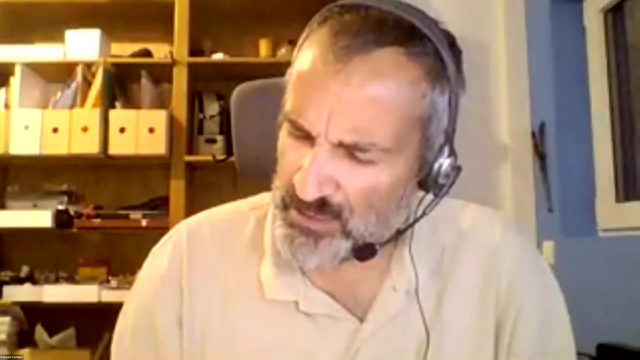 the one that I showed you in my slides, But today, with the mount I have, I have a 10 micron mount, which is just wonderful, and I have absolutely no gap, And in this case the problem doesn't exist. Sorry, can you tell me again what was the question? 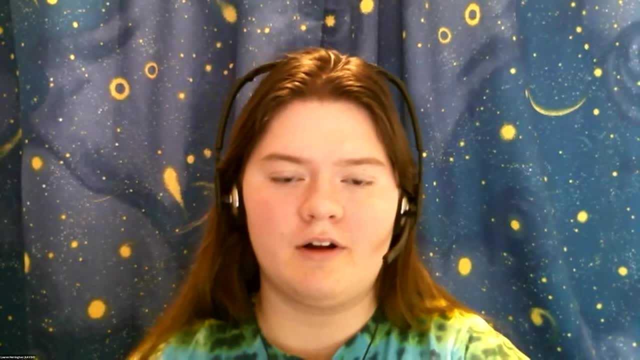 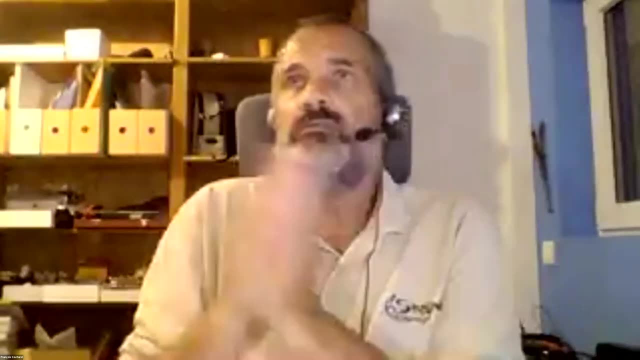 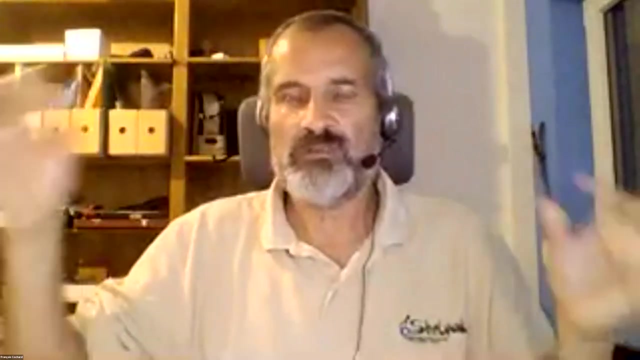 The question was about whether a very accurate polar alignment is essential for spectroscopy. Yeah, So again, the polar alignment depends on if you, if you have an observation that lasts for two hours, you have to make sure that during these two hours, 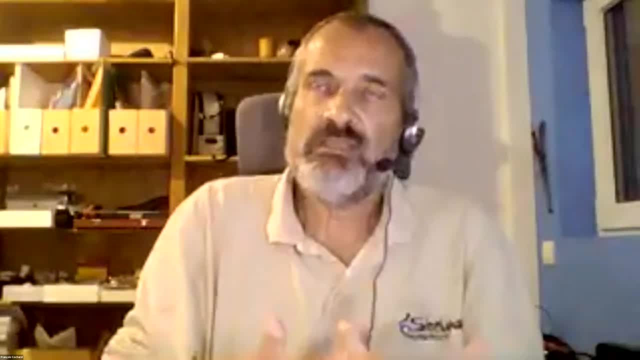 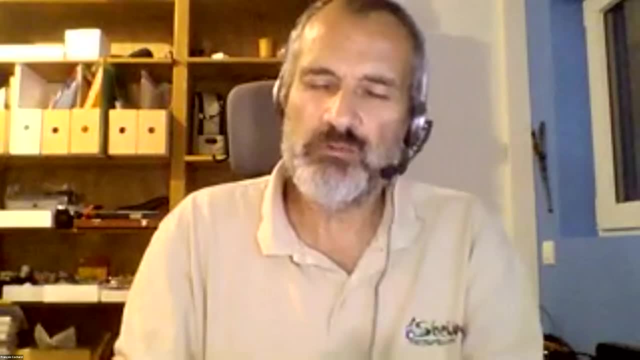 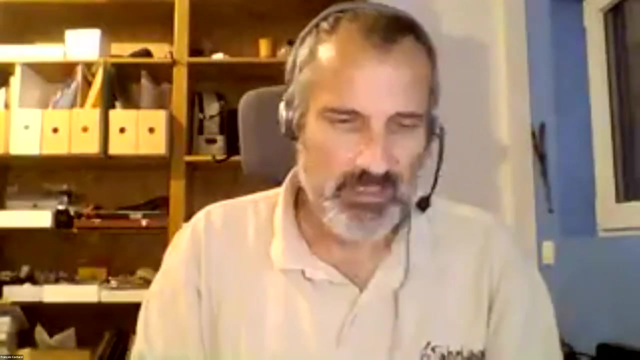 you put the star in the slit And in this case, depending on your setup- and again I come to this sentence- always know why you are doing what you are doing. It's important. what will you do to make sure that you have this control of the star inside the slit? 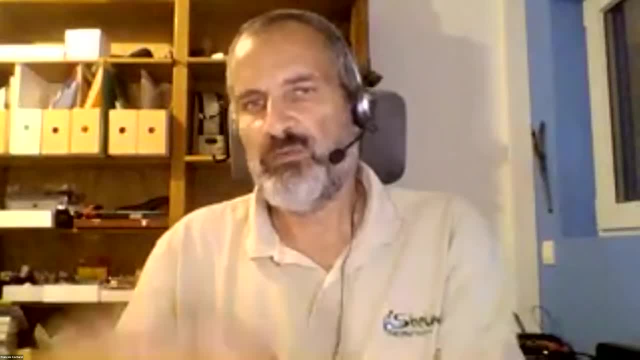 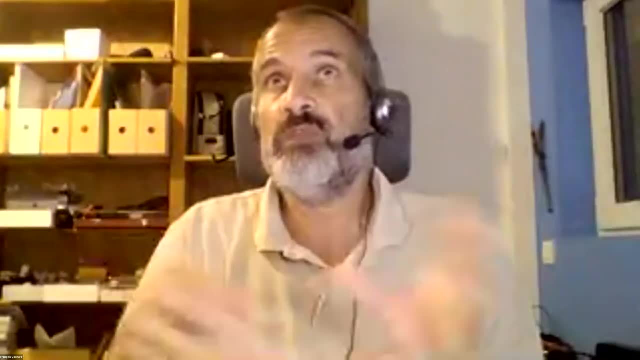 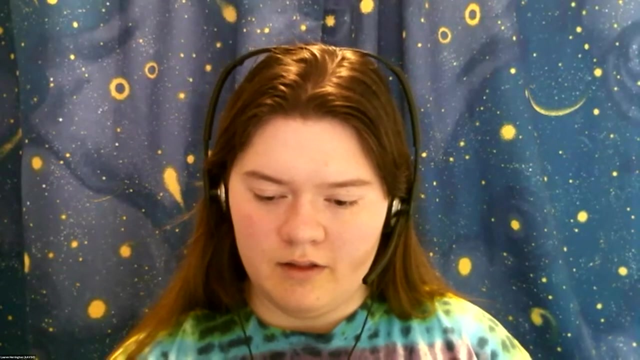 I've seen a lot of cases where the auto-guiding is more efficient than a perfect polar alignment, But this is always the same: a good polar alignment will always help to have good tracking. That makes sense, thank you. OK, so the next couple of questions. 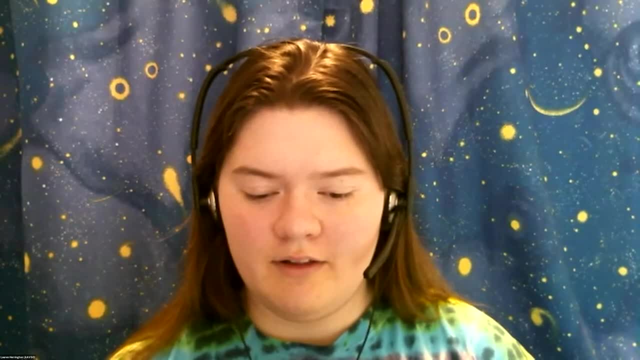 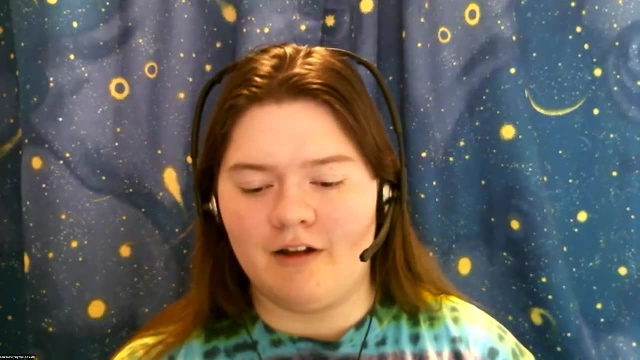 have to do with various kinds of calibration. First of all, Michael Knapper had asked: when you are taking spectroscopic images, why do you need to take darks, flats and et cetera? This is a good question. this is an important question. 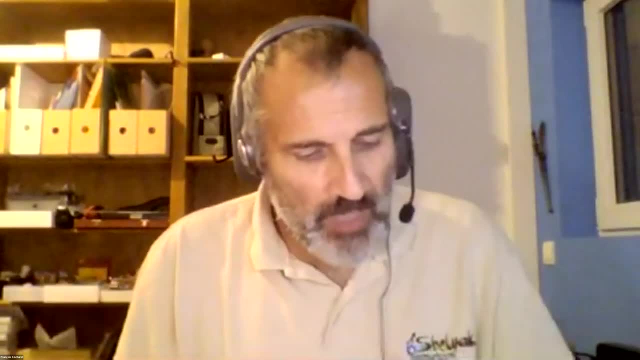 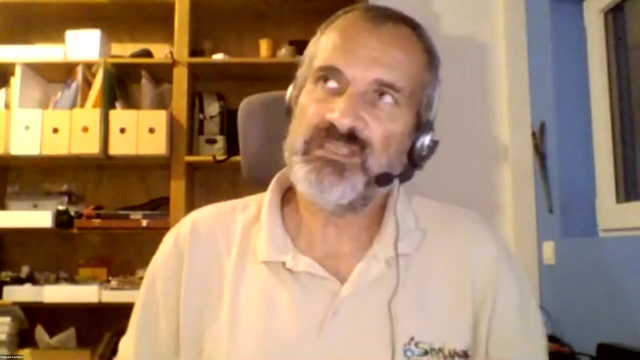 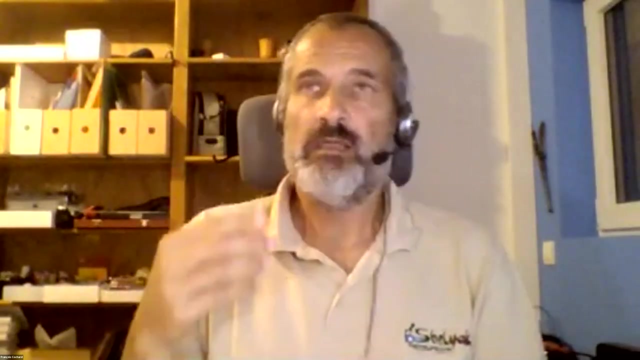 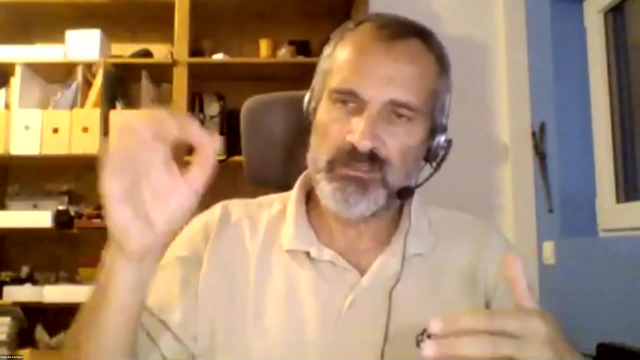 You. well, I would say that for dark, flat and various images, it is almost for the same reason than for imaging. OK, And you have to understand that. I take the example of the bias, for instance. We are looking for what energy is coming from this star. 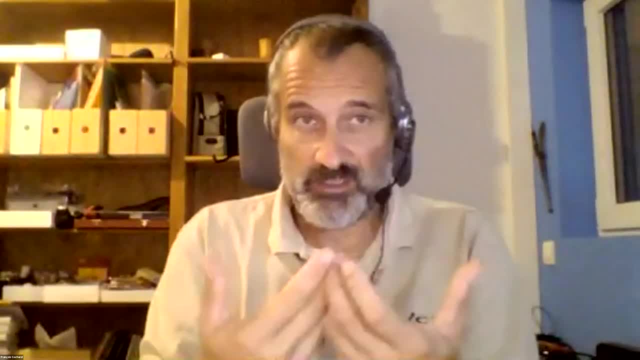 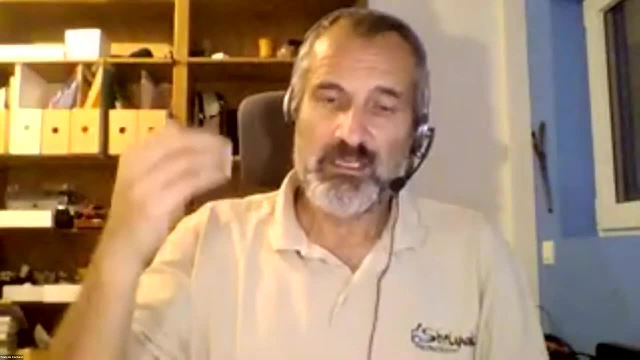 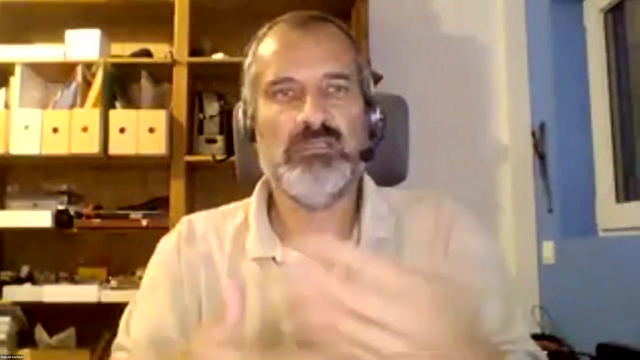 at a given wavelength and we'd like to measure this energy relatively to the other wavelengths, And to do that we have to make sure to know exactly what is the intensity of the light coming from the star. And the problem is that if you take an image with your CCD, 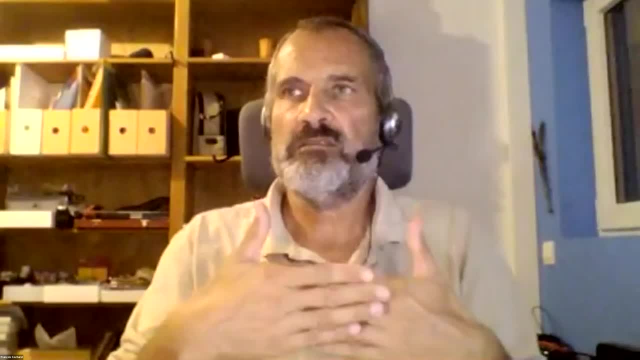 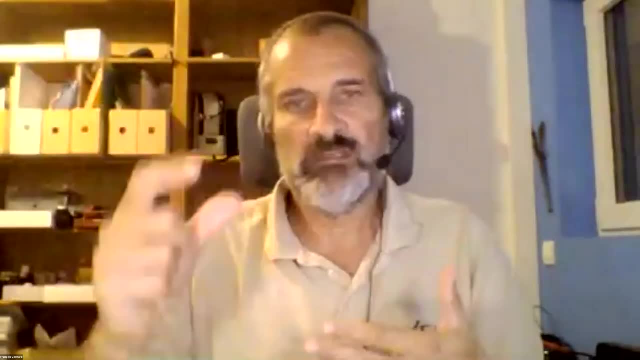 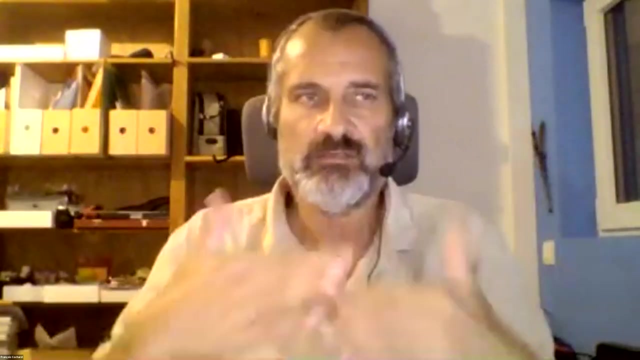 or your CMOS camera. the intensity of the light of a given pixel will not be only dependent of the intensity of the light source, because you have an offset in the camera. you have an offset in the camera design. The offset is made to make sure that all the measures 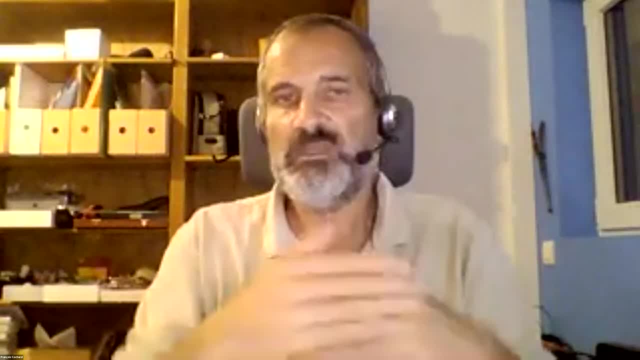 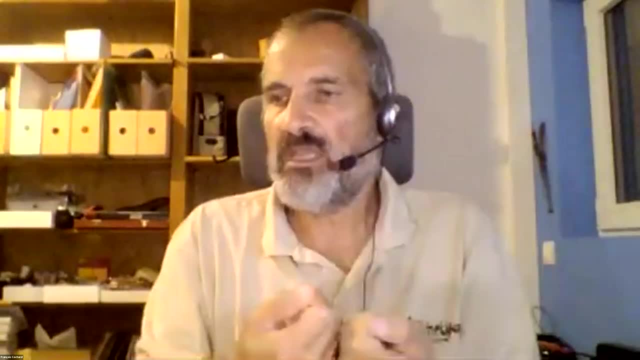 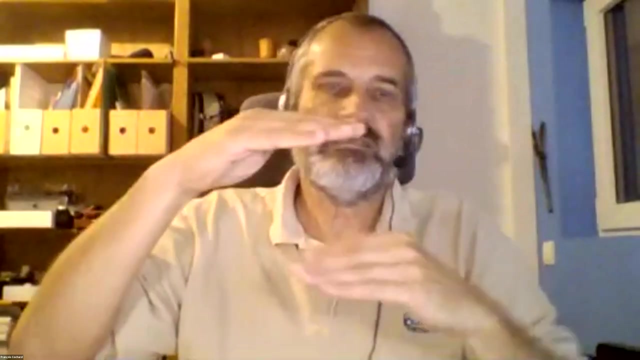 of the light are always positive and there is no risk to have negative values because the converter, the analog to digital converter inside the camera cannot manage negative values. So to avoid that we put an offset in the camera And then it means that if we have, I would say, 100 IDUs. so 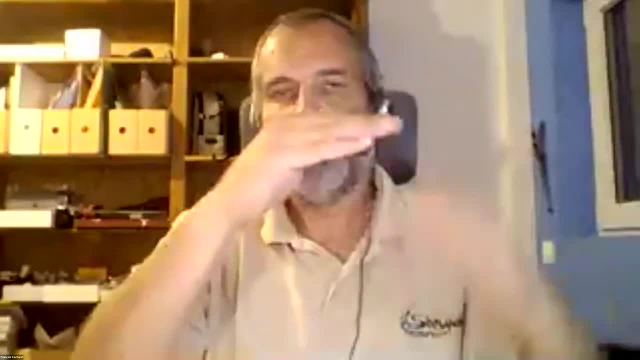 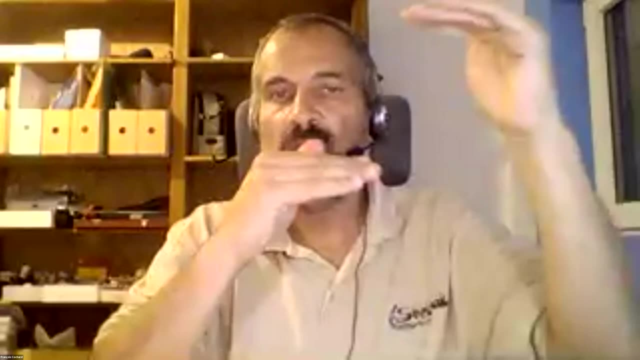 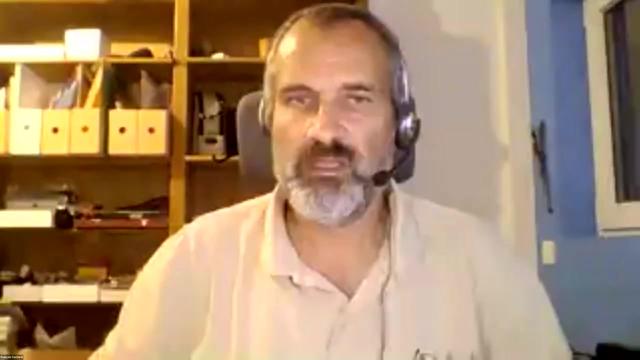 if we have a count from the star, we add some of the IDUs for technical reasons. But what is interesting is just to have the real value coming from the star and we have to remove it, to remove the effect coming from the instrument itself. 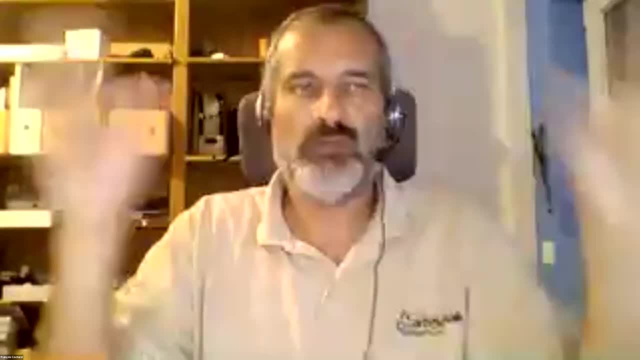 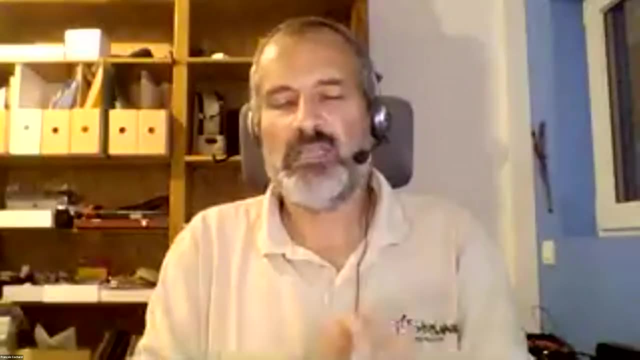 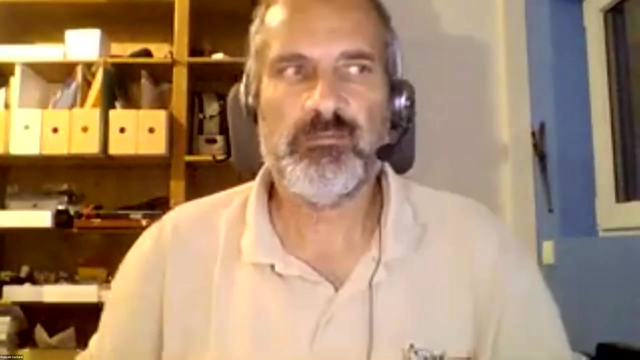 So this is a- I take one example. You have other reasons to do it, But you need to take bias, dark frames, flat and calibration images, Generally speaking, to make sure that you will be able to process properly your data afterwards. 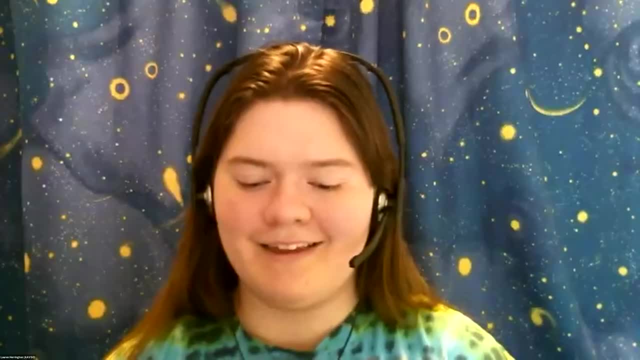 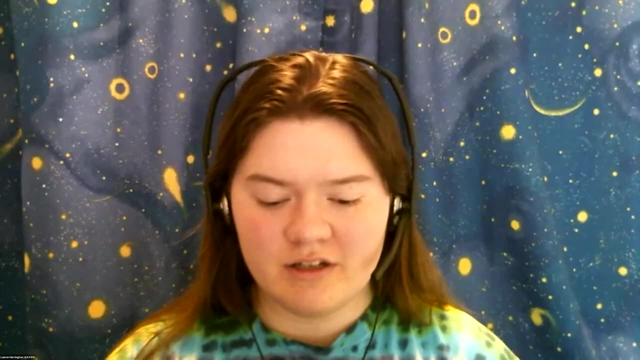 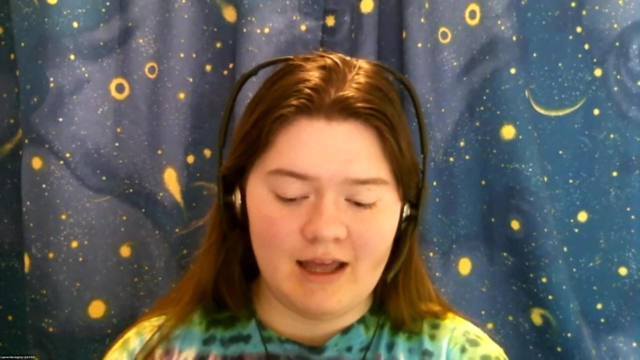 I hope I'm clear enough. I think so, Thank you, OK, and our other question about calibration. OK, so Tetsuji Tanaka had asked: how can I calibrate out the light pollution in a city? I mean, will I need another data set of an area? 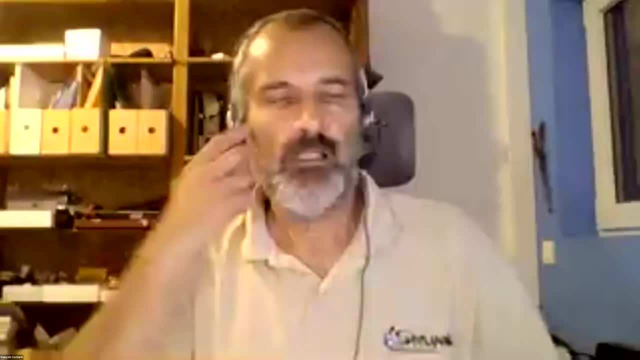 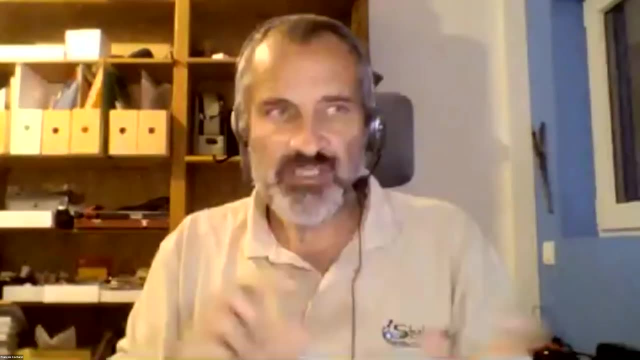 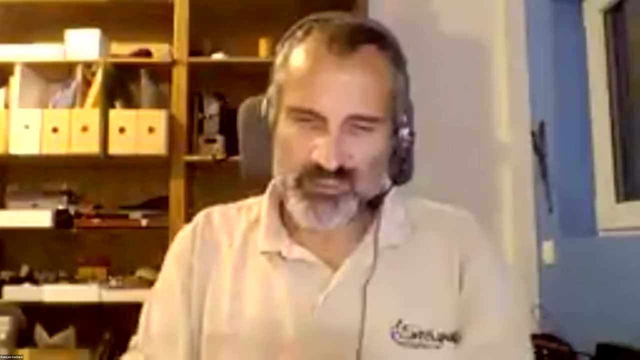 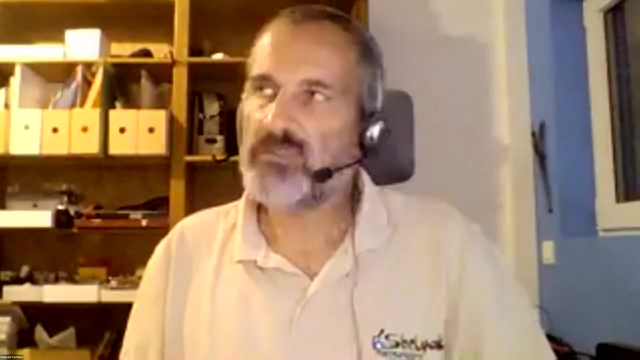 with no stars in it. How would I do that? It's a good question. Well, it depends if you want to measure the light pollution in your city or if you want to compensate your observation from the light pollution. Of course, if you want to measure the light pollution, 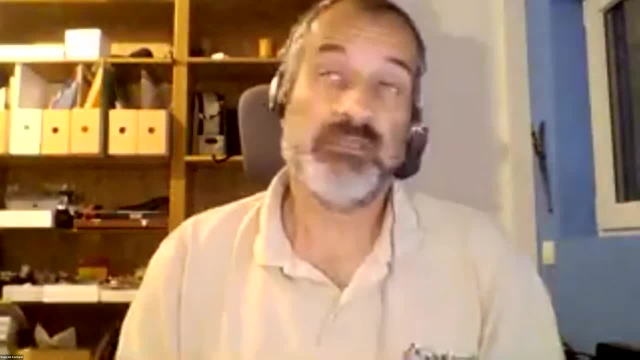 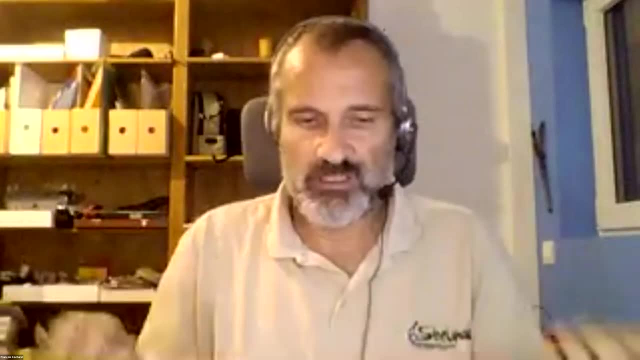 you have to have a reference, a perfect reference, But again, using the, if you are using the flat dark frames and so on, you would be able to measure what comes from the sky really, And you just have to not point at the star. 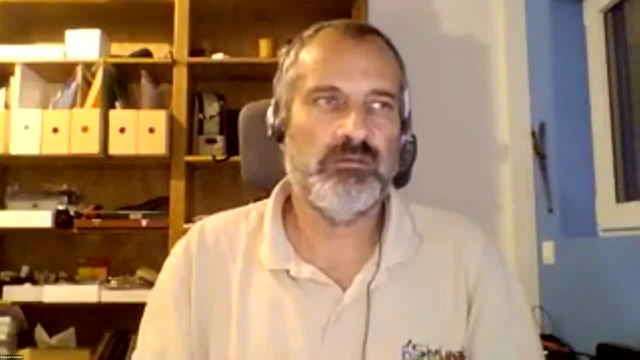 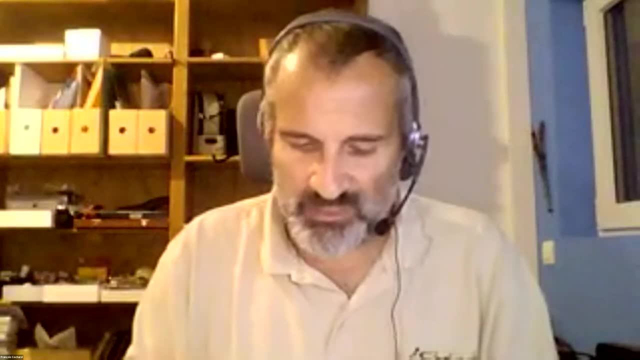 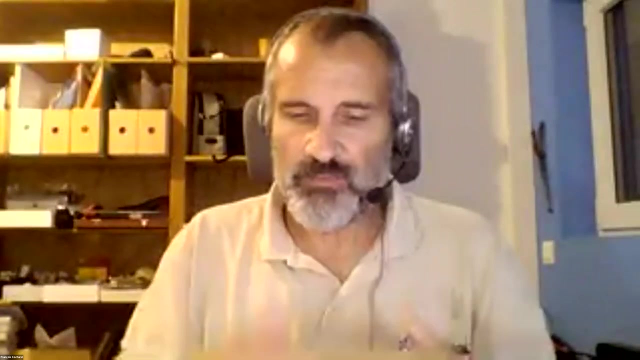 and just point at the sky itself And you will measure the light coming from the sky. Now, if you want to compensate your observation, your star observation, from the light pollution, skylight pollution, it's quite easy if you have a slit spectroscope. 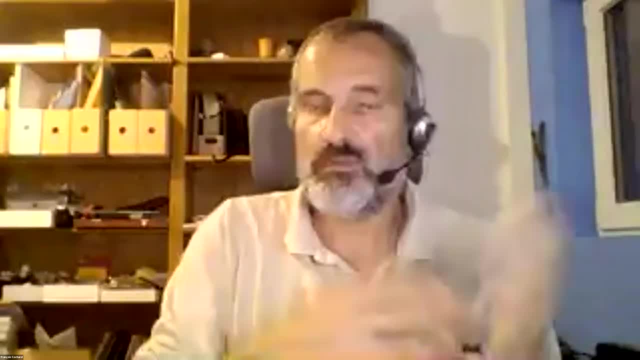 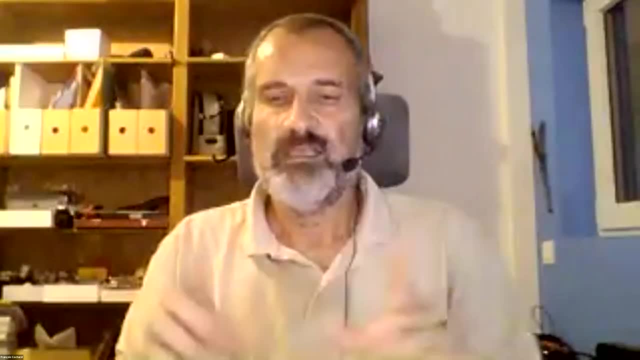 Again, this is not something that you can do with a slitless spectroscope like this analyzer, But if you have a slit spectroscope like DLP or the UX or things like that, because we have a slit and we in fact, 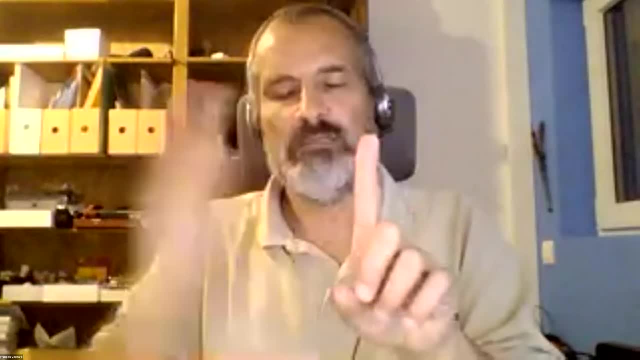 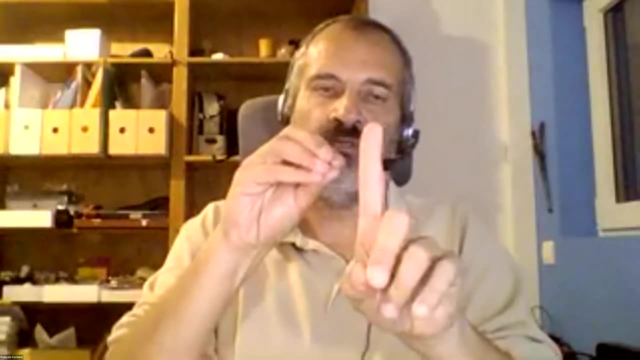 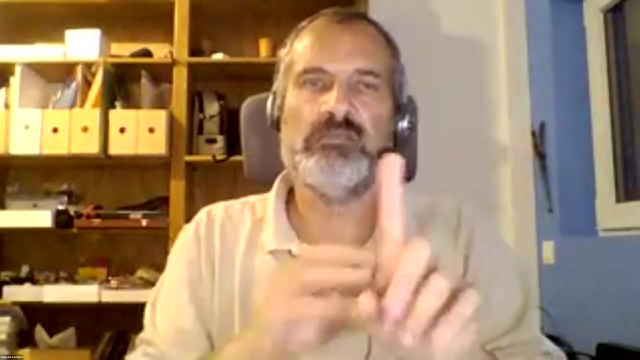 this is all the light going through the slit that is spread out and that is transformed in a spectrum profile. And if you do that, we just put the star at a single position in the slit, which means that all the remaining parts of the slit have the light coming from the sky. 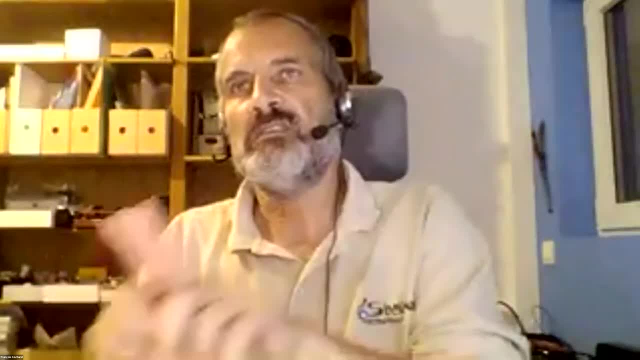 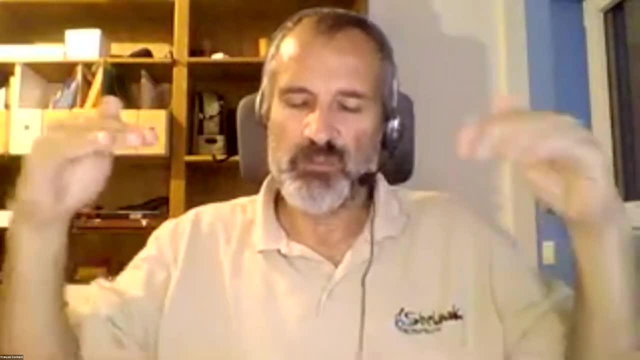 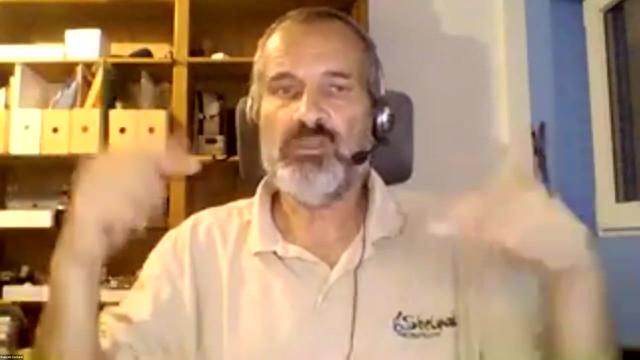 And then when you take a spectrum in city center, you will have in the middle of the image, generally speaking, the star spectrum, But above and below this star spectrum you'll have the sky pollution spectrum And then, during the processing, we 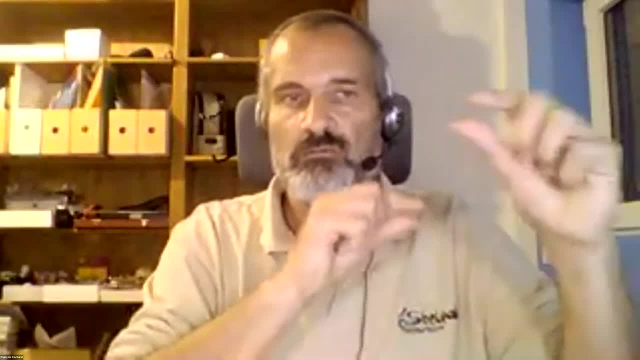 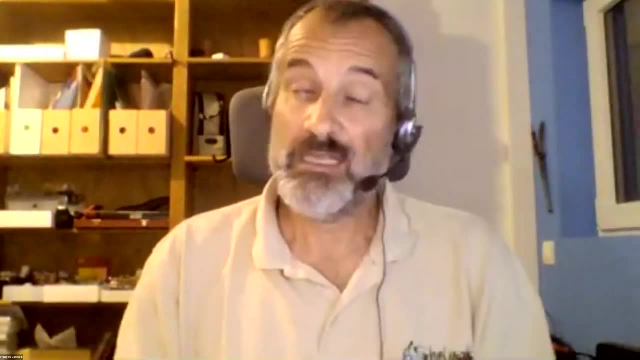 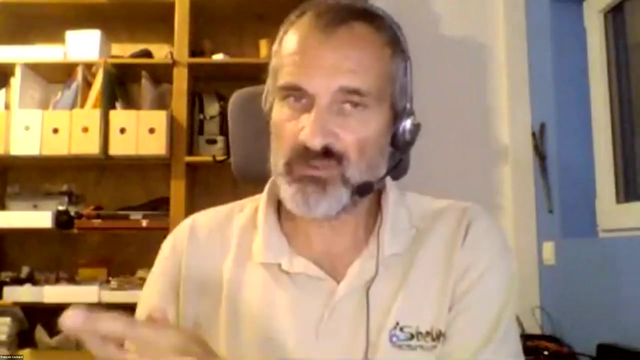 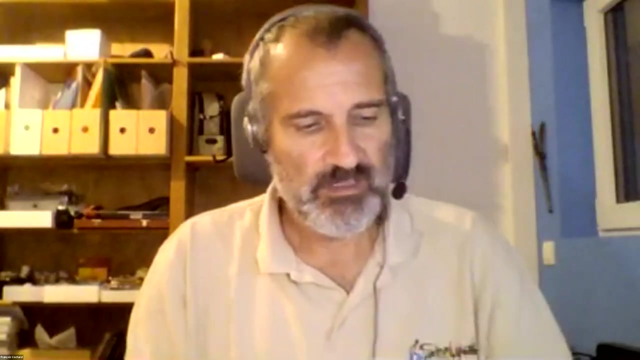 will measure the sky pollution on top, above and below the star spectrum to compensate the result from the system. So this is a very important point that really makes possible to do spectroscopy and to do science in spectroscopy and to compensate for some problems in city observations. 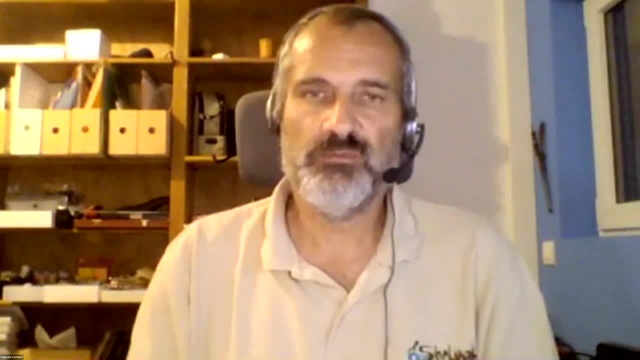 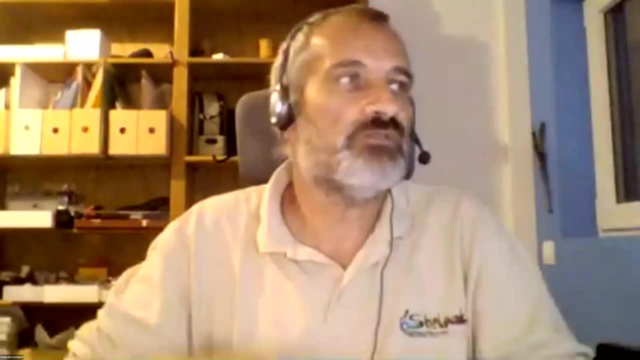 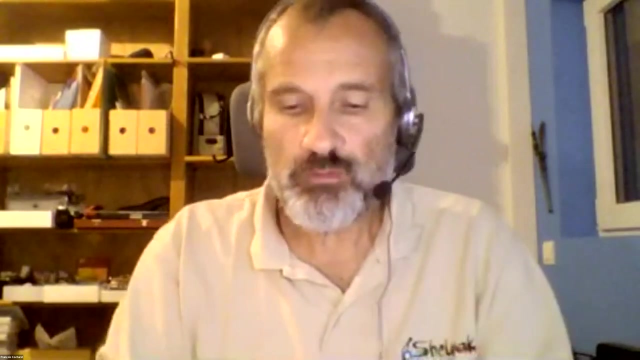 and to do a great observation. You can do spectroscopy in city center, Of course, if you are lucky enough to be in a great country. It's much better to do that in a better sky is always better, of course. OK. 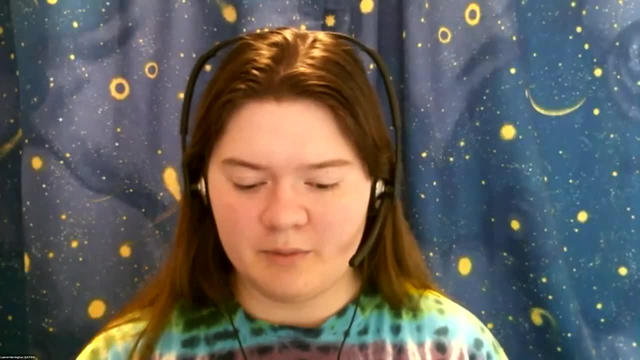 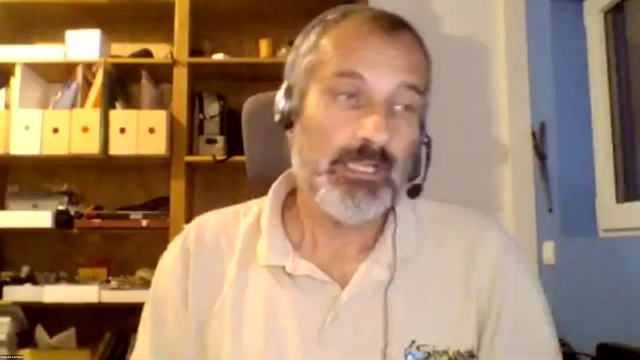 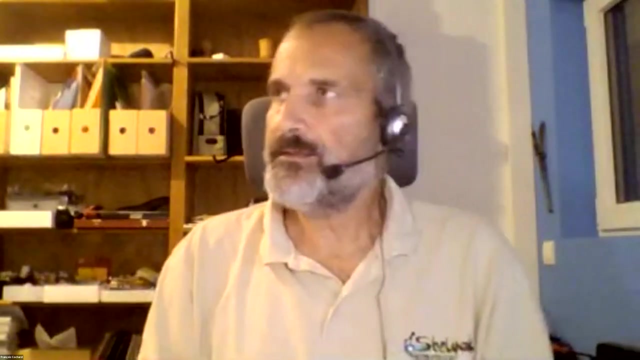 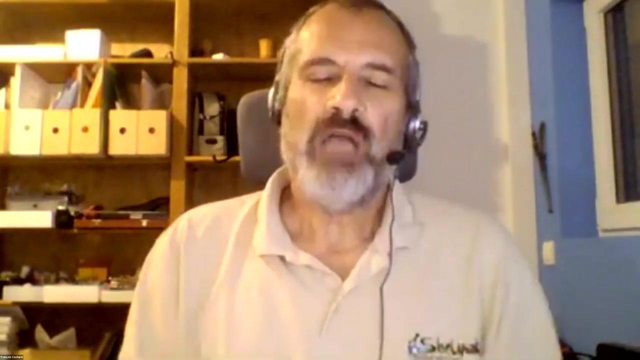 Thank you, And the next question comes from Hamish Barker, who had asked: is the color temperature of the flat lamp critical? It becomes very technical. Yes, It depends on the algorithm that you use behind. We would love to have the ideal flat lamp. doesn't exist. 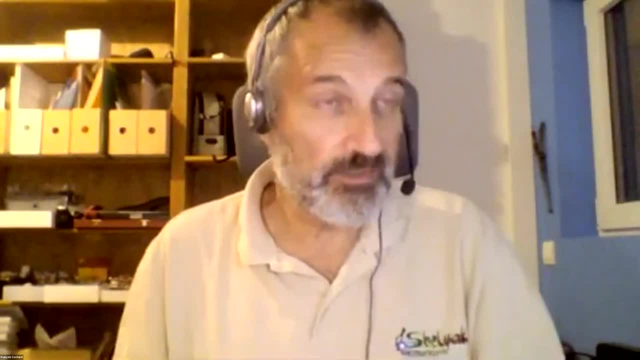 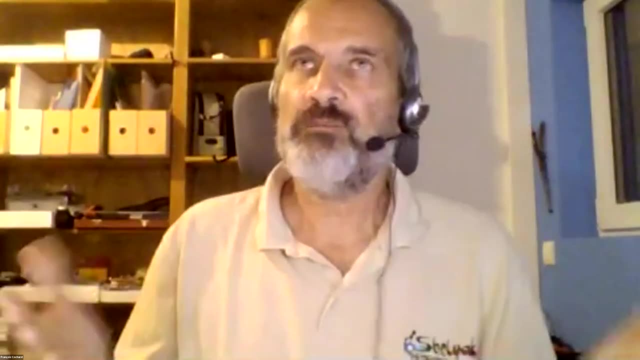 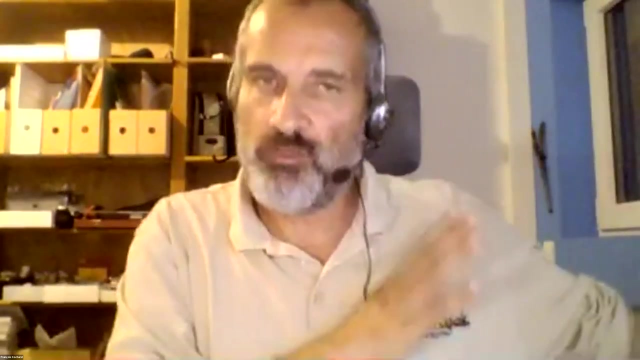 Or maybe I should say like you did, Lauren, doesn't exist yet, Because an ideal flat lamp would be a very, very high temperature lamp, like the stars, to have a lot of energy in the blue part of the spectrum. And the problem is that, when you are, 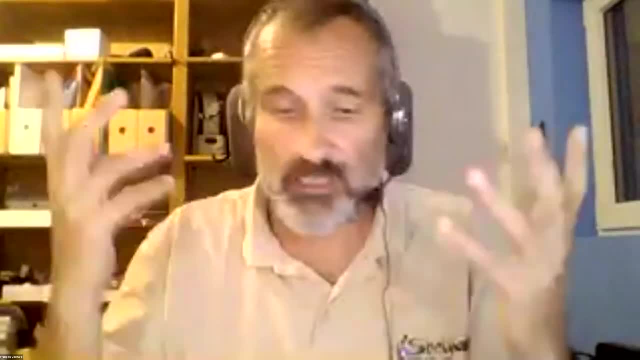 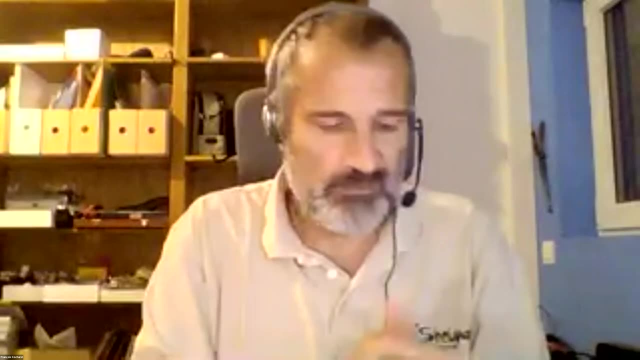 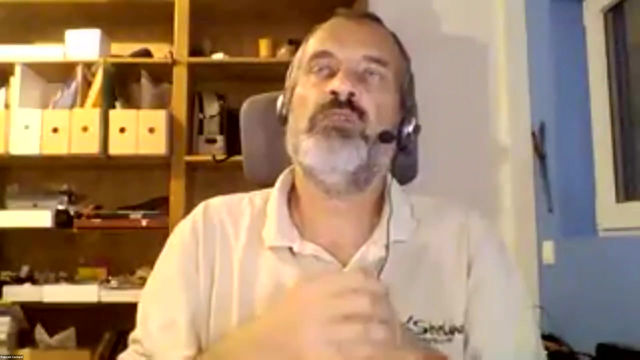 when we were using a halogen lamp or xenon lamps or things like that. the temperature is not is quite high, but not as high as stars, So we don't have enough light in the blue part of the spectrum And the other parameter would be. we would love to have something. 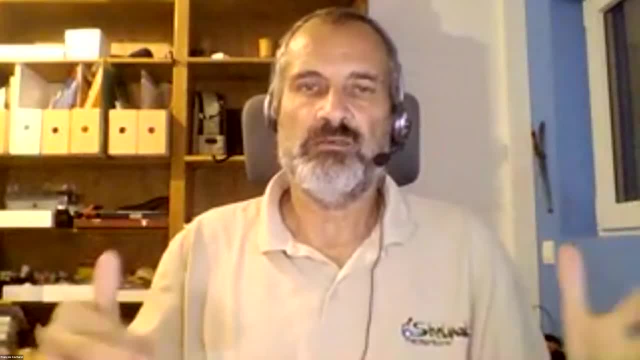 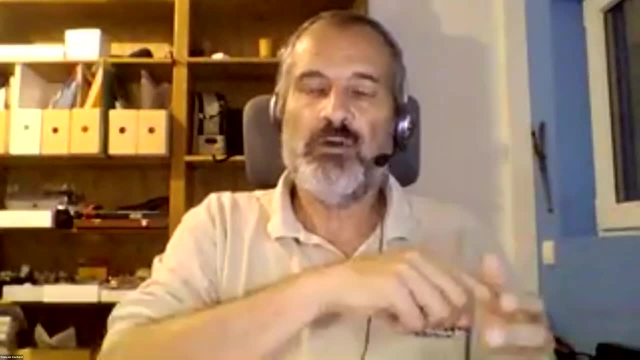 which has exactly a black body behavior. So if we would have that, if we would be able to have the same, if we would be able to have such a perfect lamp, we could say, okay, so this is a black body profile. then we have the theoretical profile of this lamp. 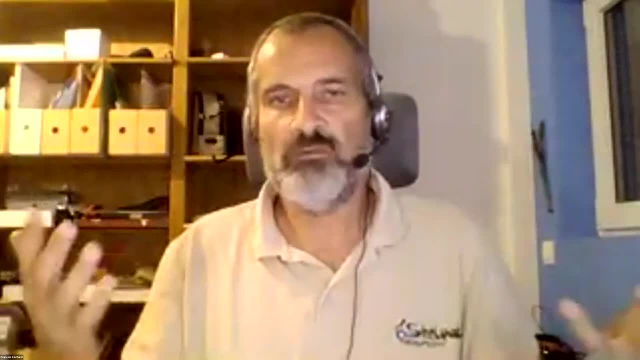 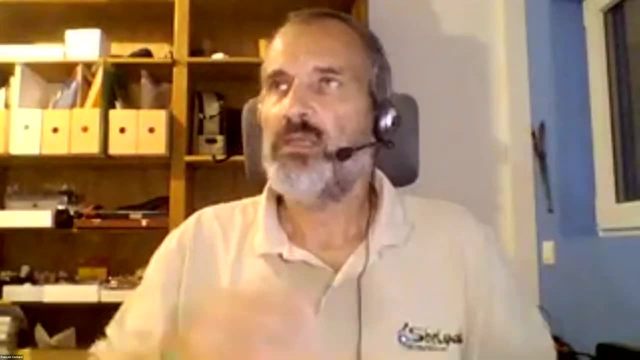 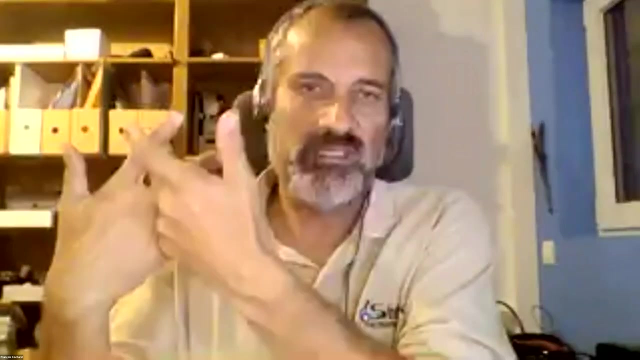 Then we can just by measuring the flat, we have an absolute value. Okay, In fact, this is not the case. This is not exactly a black body profile, and we don't have enough energy in the blue. So, as a result, what we do at the end is that we always take a reference spectrum from a given known star. 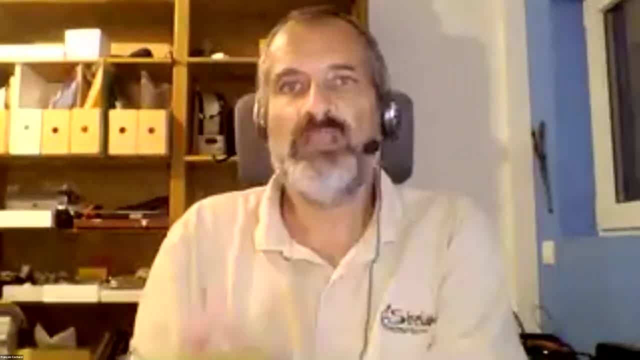 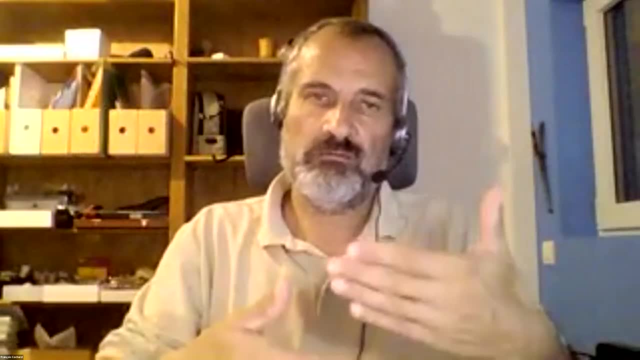 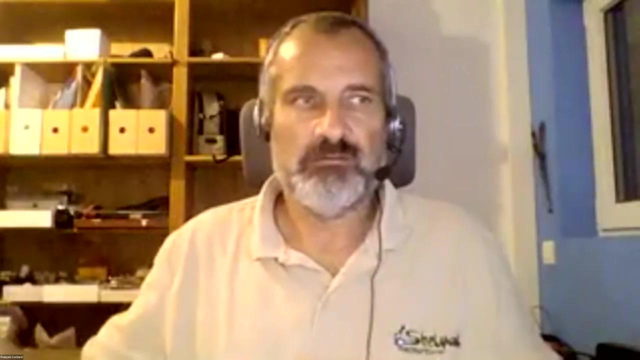 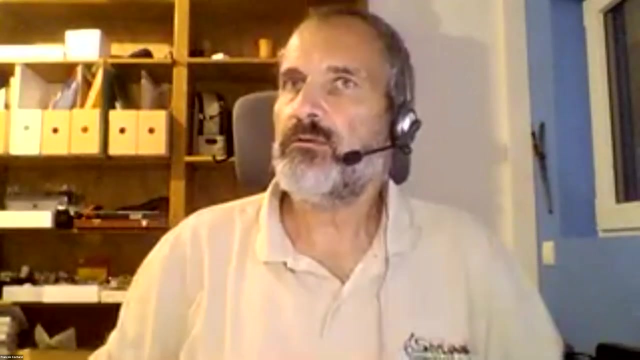 And a known star means a star for which we have a very reference spectrum that we can compare from, And then we use that to calculate the instrumental response. Of course, if the flat is the, how can I say that The better is the flat lamp, the less we have to compensate with the observing? 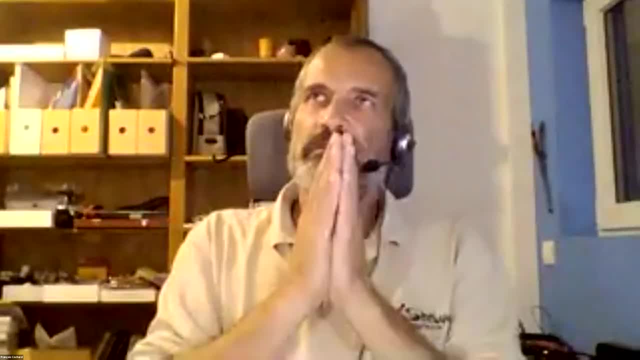 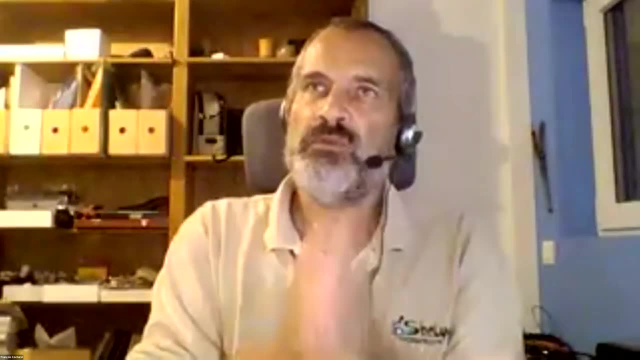 the less we have to compensate with the observing another star. Okay, You have to understand that we are. nothing is perfect, So we are looking, we are trying to do perfect observations with an observation, with an instrument which is not perfect. 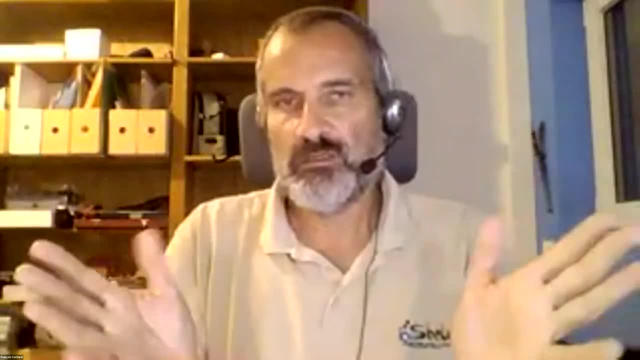 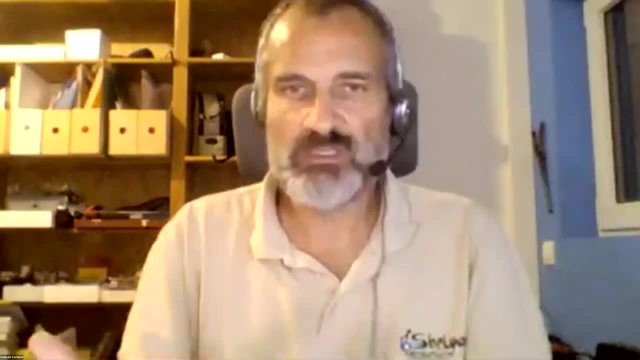 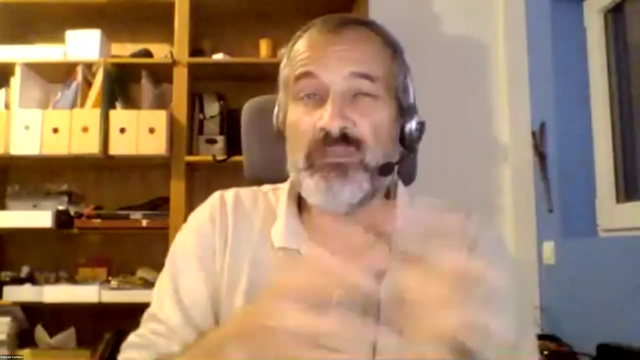 And what makes the difference is really the methodology. So we take what we have, We take not perfect lamp, We take not perfect instruments And because we are clever enough, we can use the computer, We can use some algorithms and so on to improve things and be as close as possible as 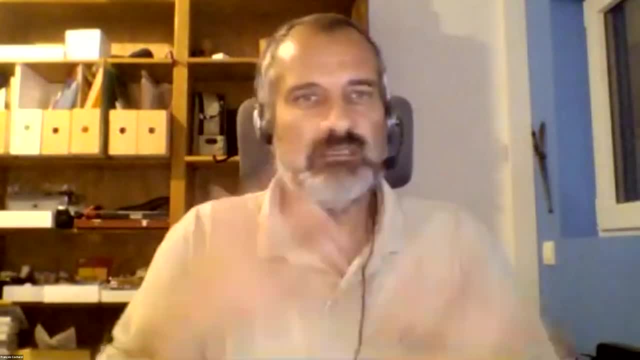 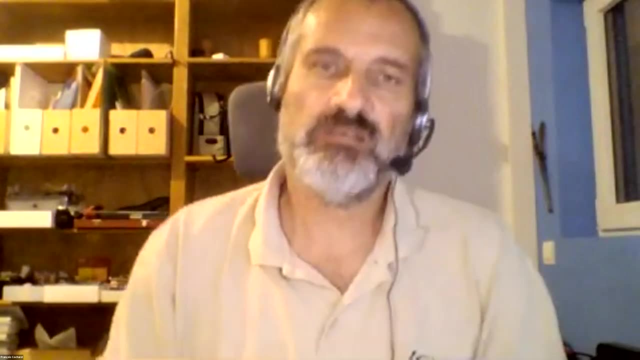 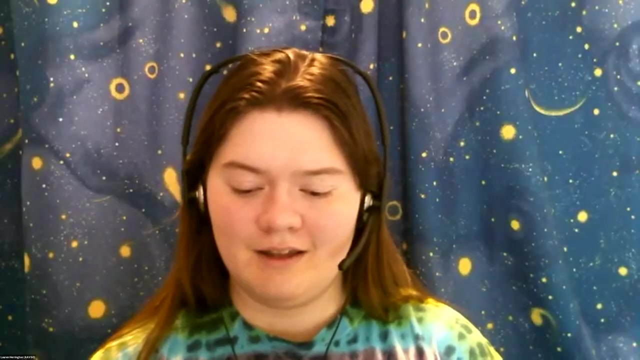 as the truth, in fact coming from the star. But it's always a question of trade-off and compromise And we are in, we are doing perfections with the imperfect device and elements. I like that way to put it. Thank you. 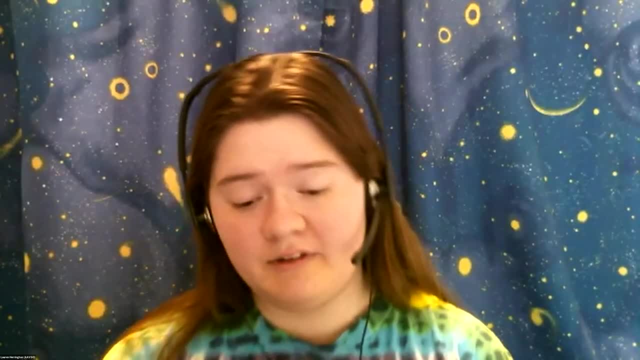 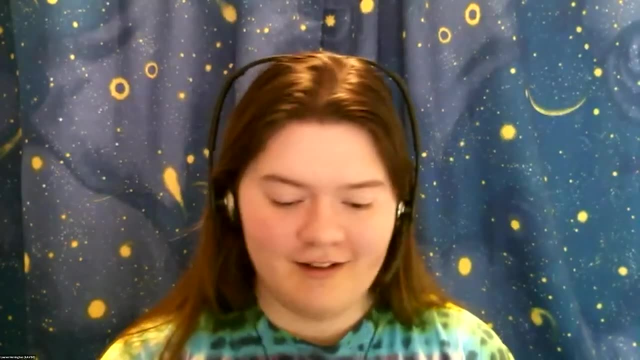 All right. So one comment that just came in from Timothy Weaver. I'm going to read it out while it's relevant- is: if you're looking for a light source that is as hot as a star, maybe a plasma torch is what you're looking for. 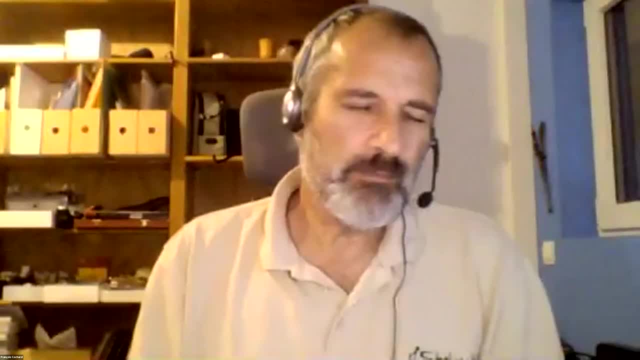 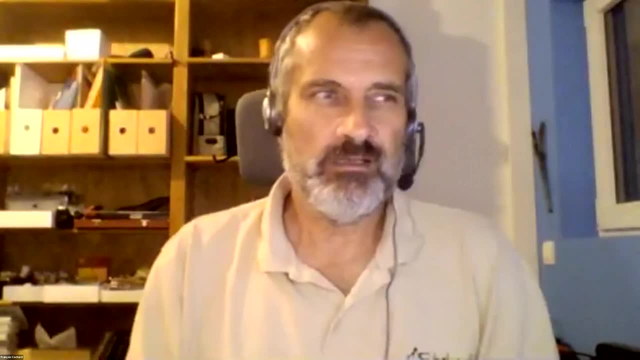 As far as I know, so I know that their system so well. this is a. I keep keep the door open in case of. we have very good news. I think that the plasma torch has is as a lot of lines. 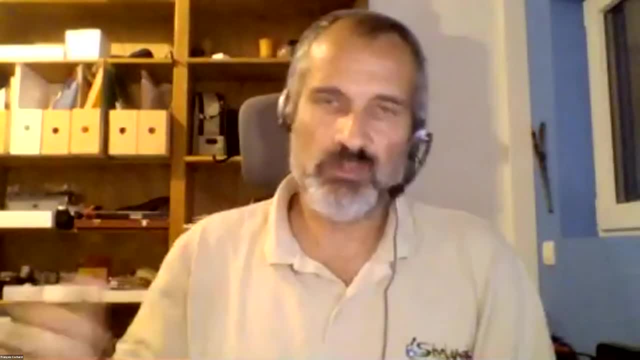 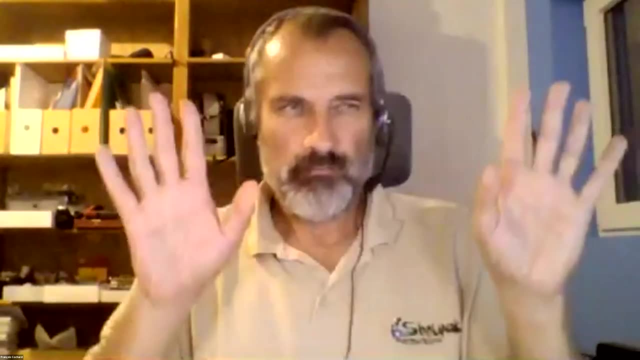 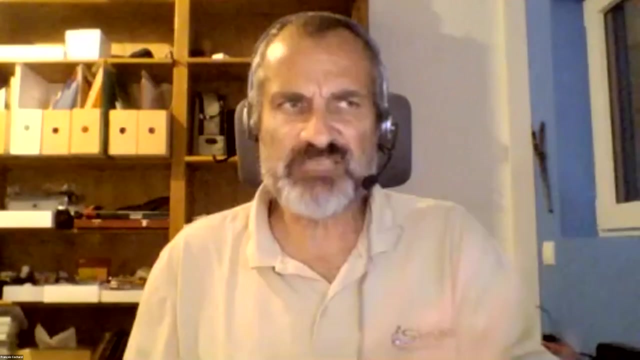 if I'm right, this is absolutely not a continuous, continuous lamp, continuous profile, so it's not an ideal system for a flat lamp. Maybe I'm wrong Again, I know that there are some systems, maybe there are some systems, but for me, plasma lamp means that you have emission lines. 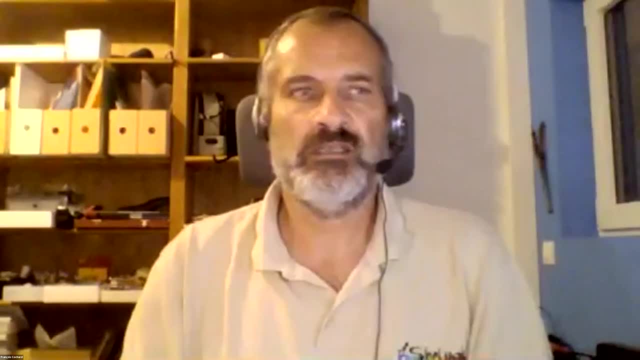 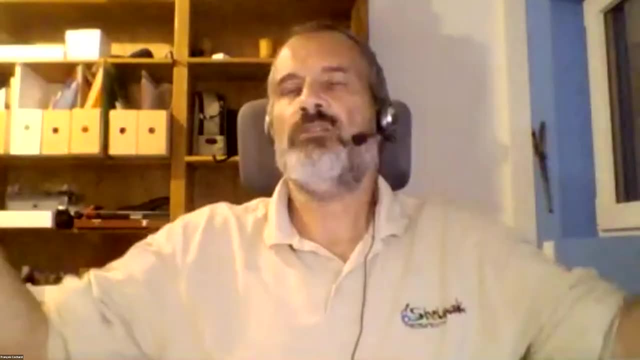 and then this is absolutely not something that we can use as a lamp. This is the same. for instance, we could use the sky. We could say: well, the sky has this is the light coming from the star. so the source has a very high temperature. 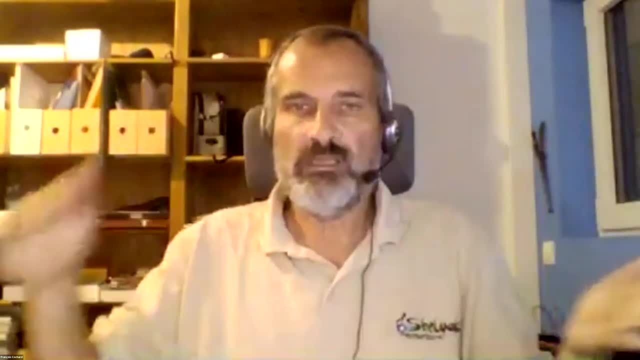 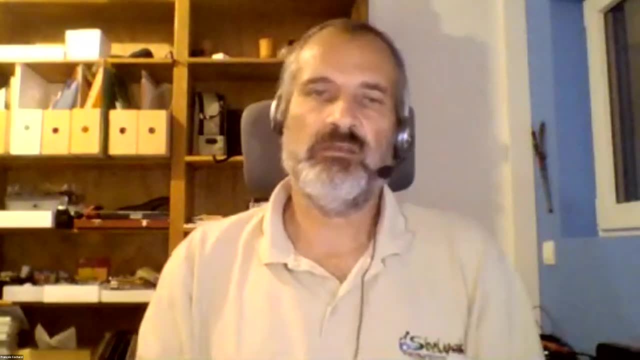 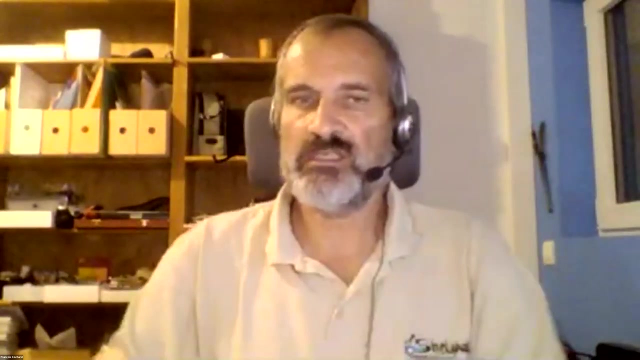 Yes, but the problem is that it is absolutely not a Planck profile lamp and light source, so we cannot use it as a flat. Yeah, that makes sense. It's a pity which is also different with imaging, because for imaging we can use the sky as a flat source. 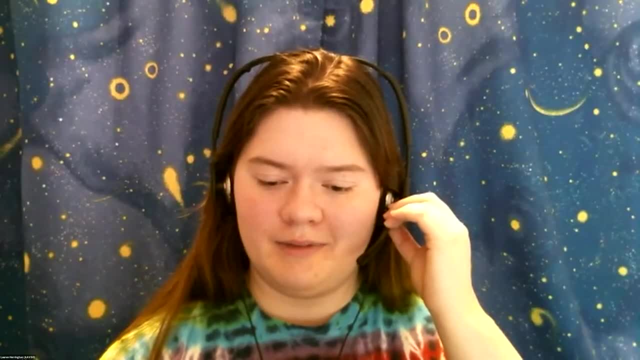 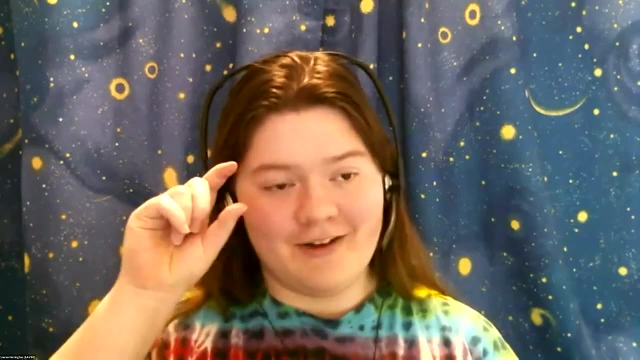 Yeah, I think you're correct about plasma torches having a lot of emission lines. I've looked at a small one through a diffraction grading before and it's a very beautiful spectrum to look at because of all those little emission lines. 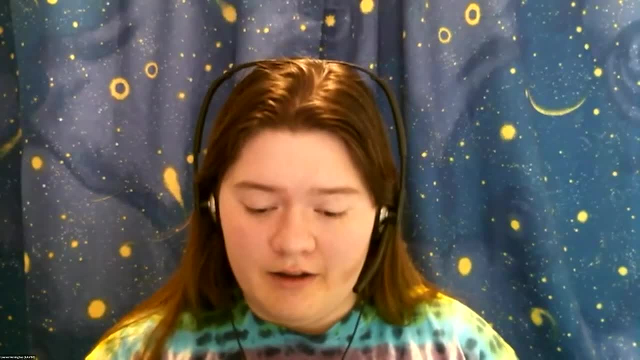 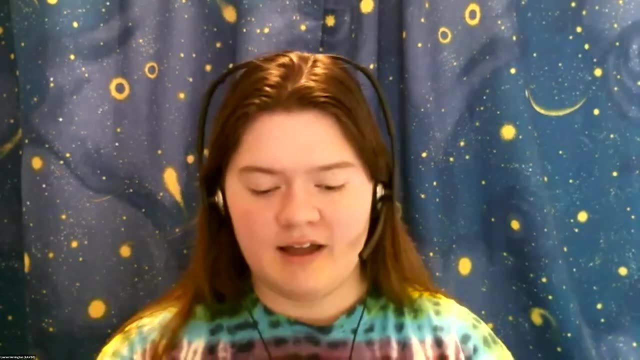 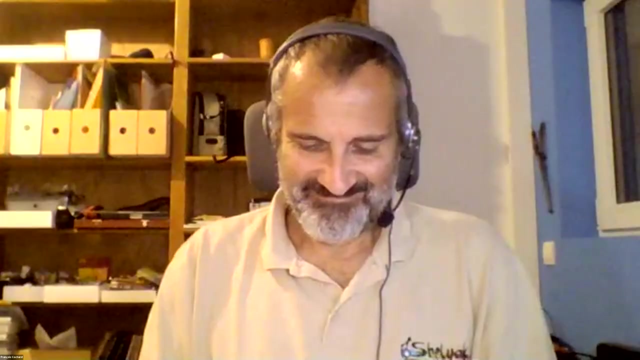 but it wouldn't work well for a flat. All right, Let's see. So one more question on this topic comes from Pradeep Karmakar, who had asked: is it always compulsory to do the instrumental correction, or can we sometimes just stop after the wavelength calibration? 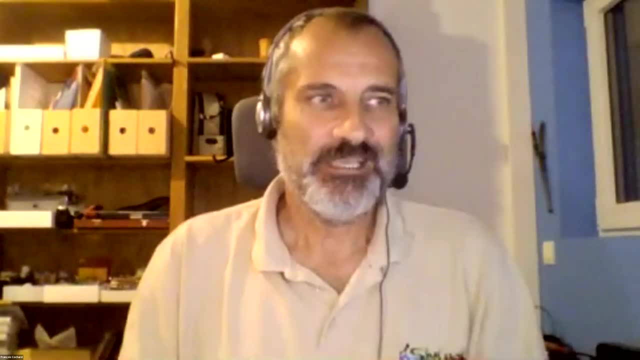 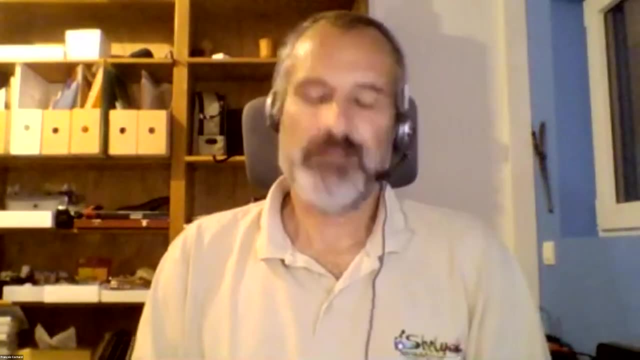 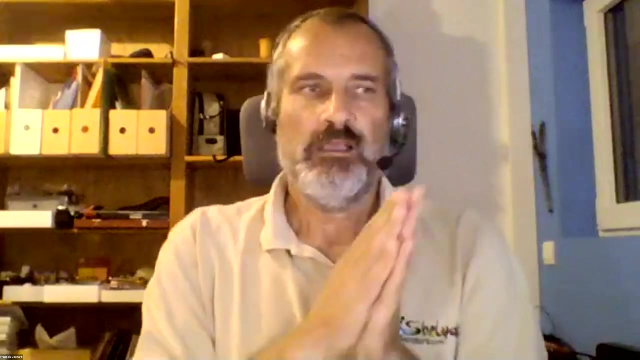 I love this question. Thank you, Pradeep. This is a very good and important question. I would say two things. The first one is: it all depends on what you are looking for, Okay, so again, you have to know why you are doing what you are doing. 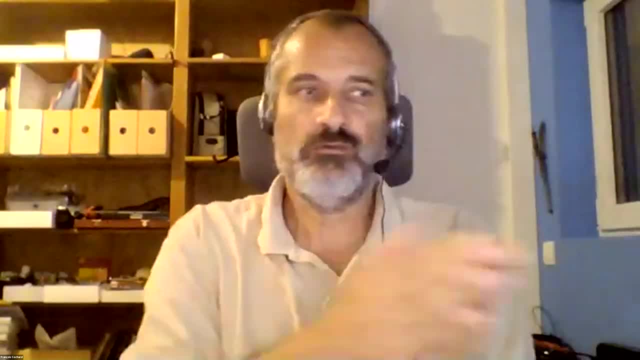 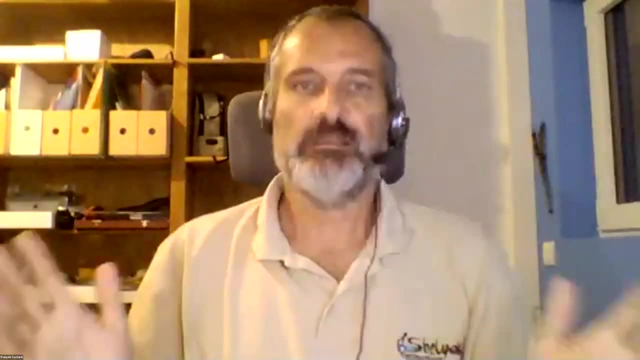 So you don't have to do the calibration or to do the instrumental response correction because you have been told that you have to do it. It's not an enough reason, Okay? So it really depends, And I like this example, A wonderful program, for instance. 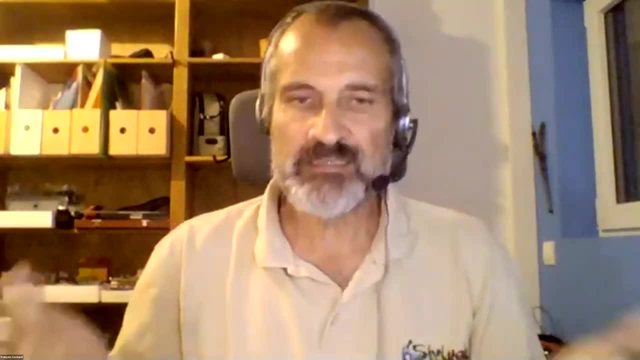 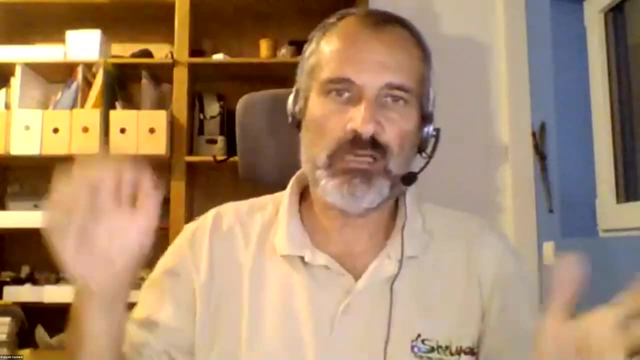 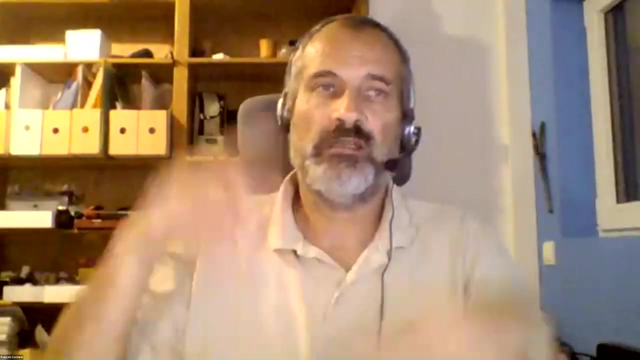 is to observe as many B star as possible to detect new BE star. BE star is a B star in which you have some emission lines, Okay, And these emission lines are, in some stars they are permanent, But in a lot of stars they are varying over the time. 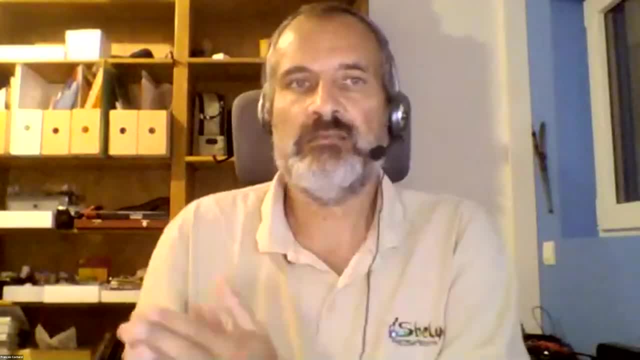 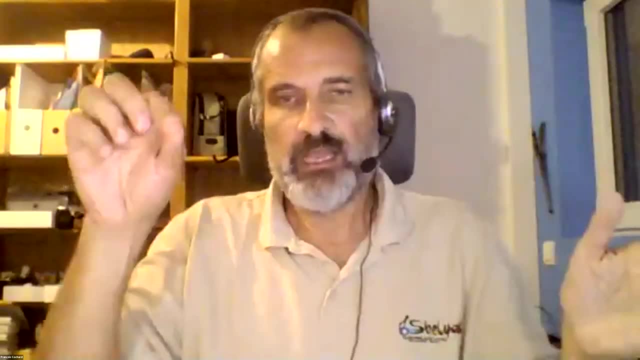 And we know that we still have a lot of BE stars to discover. So to do that in this case, you just have to observe a lot of B stars and look at the H alpha line and look if the H alpha line is in absorption or in emission. 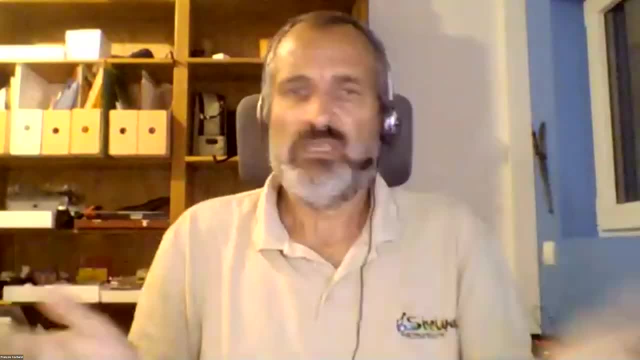 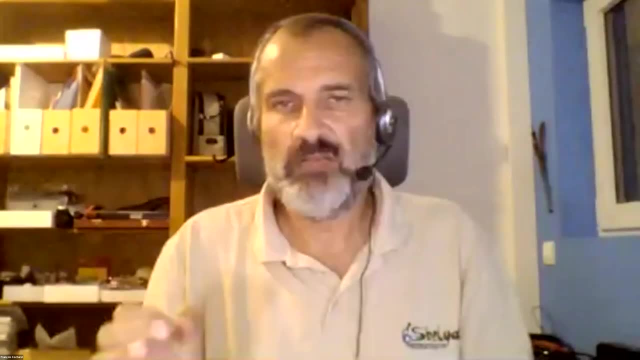 And if you have this kind of observation, you don't care about the calibration, even the wavelength calibration. So it's not precise. We know in the system why is the H alpha? We can recognize it very easily because B stars are hot star with a smooth profile with 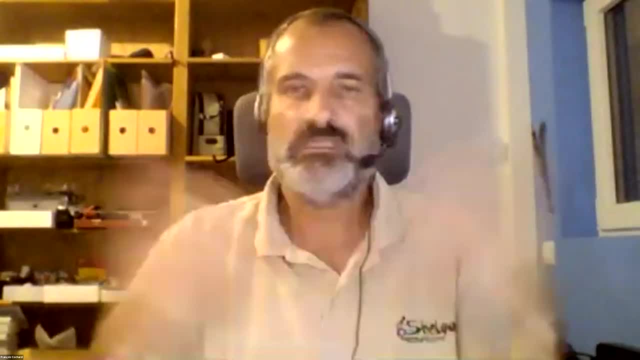 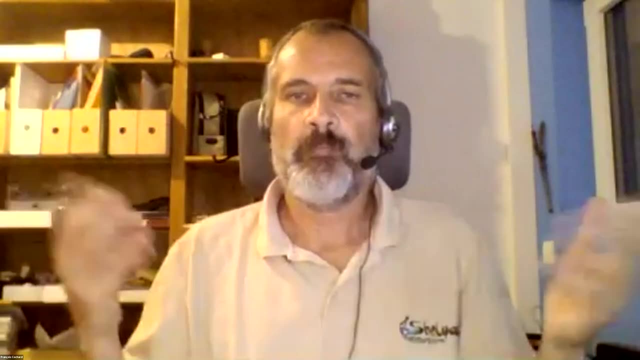 a few H hydrogen lines, So it's obvious to see. So you can just use the raw image and you don't need to process anything. Okay, So in this case it's enough. So it's important. So you do the calibration if you need it. 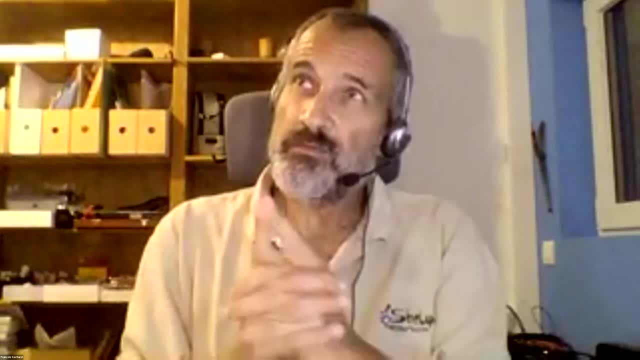 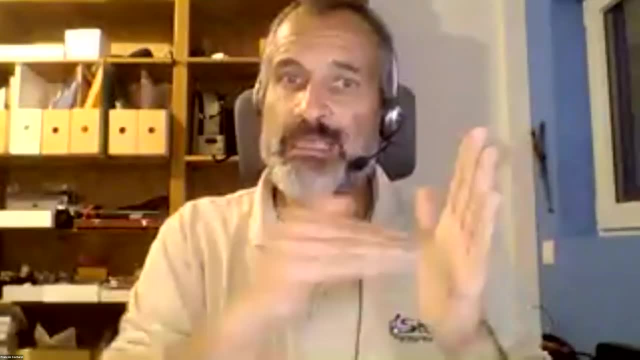 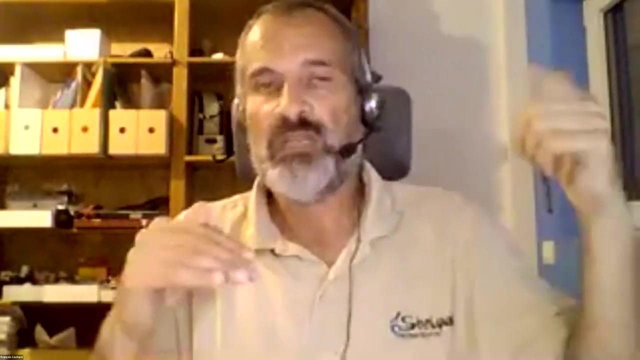 Okay, And don't do it if you don't need it. Also, you have to remember that in a spectrum we have roughly two kinds of information. The first is along the X axis, which is the wavelength, And the other one is along the Y axis, which is the intensity, the relative intensity. 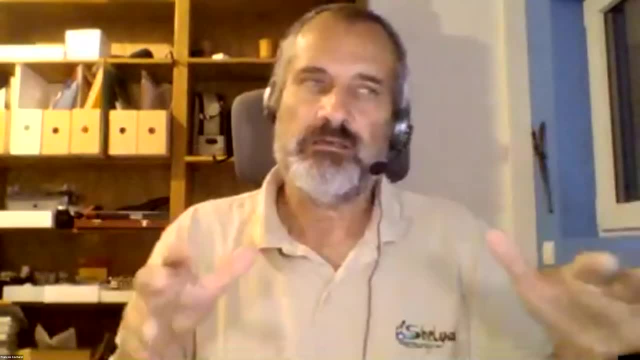 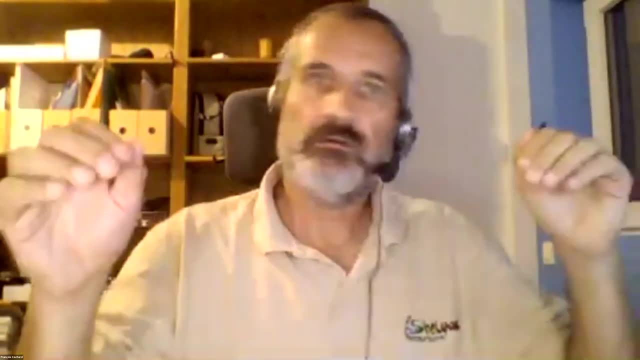 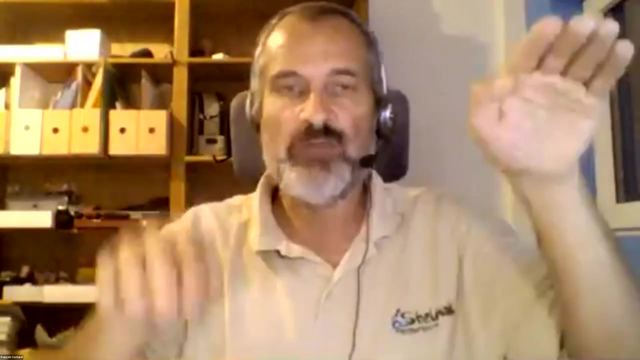 of the profile, Depending on what you are doing. for instance, if you are measuring the relative density of this gas versus this other gas, the question is more related to the Y value of it. You have to look at the intensities. Now, if you are looking for exoplanets, in this case, the key is that you have to look. 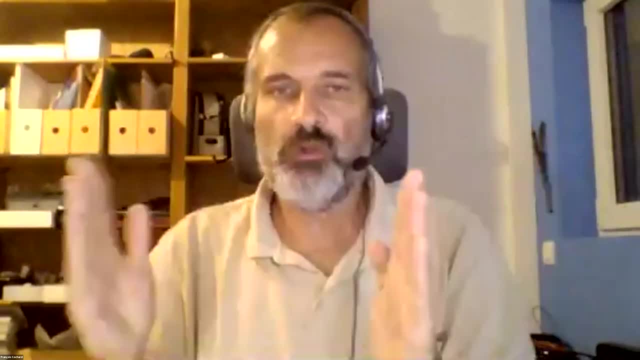 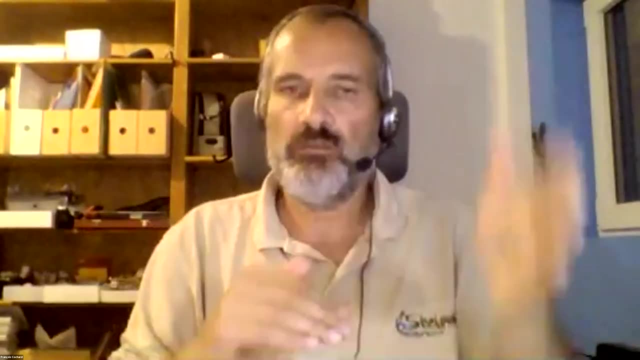 at the Doppler effect, and the Doppler effect is linked to the wavelength calibration. So, depending on what you are doing, you are more looking at the X axis or at the Y axis of your spectrum. Okay, So really keep in mind that it depends on what you are doing. 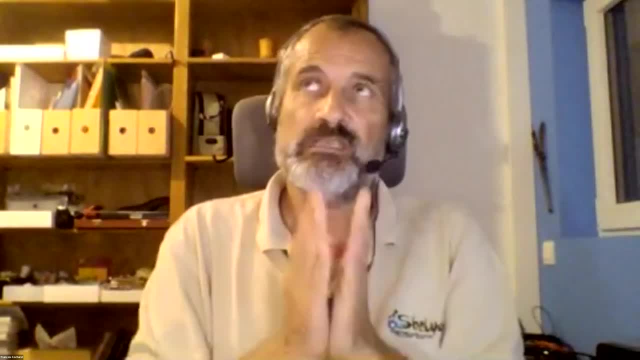 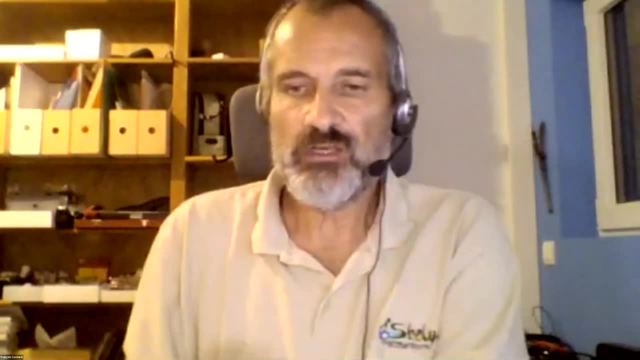 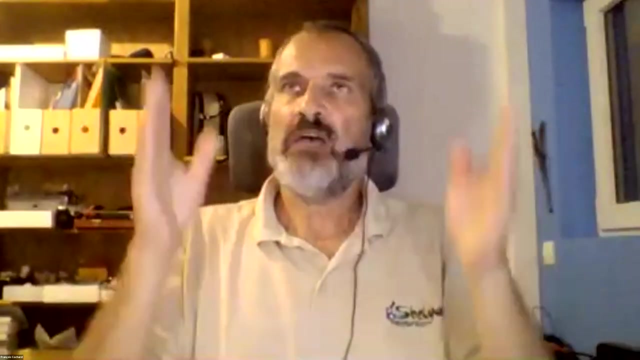 Now there is another reply to this question, which is when we are doing spectroscopy as an amateur community together with the professional community, to have new observations. It's important to say that. okay, when I do an observation, I probably have a good reason. 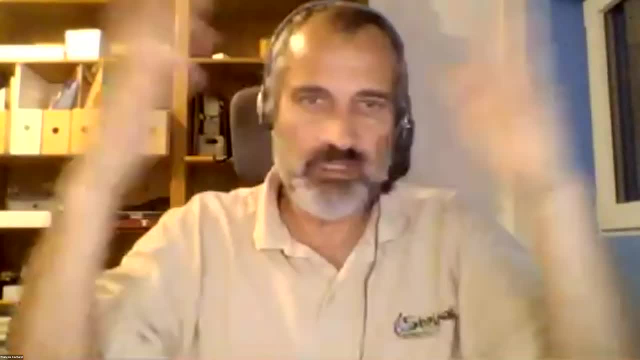 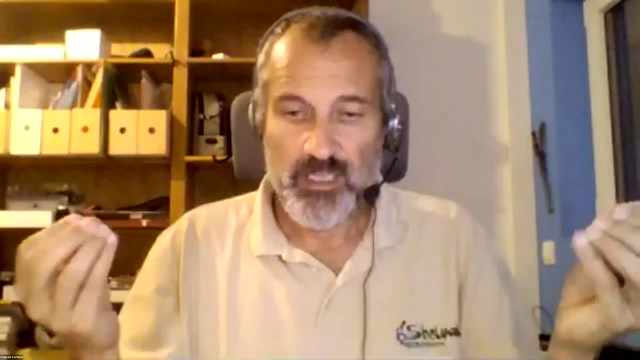 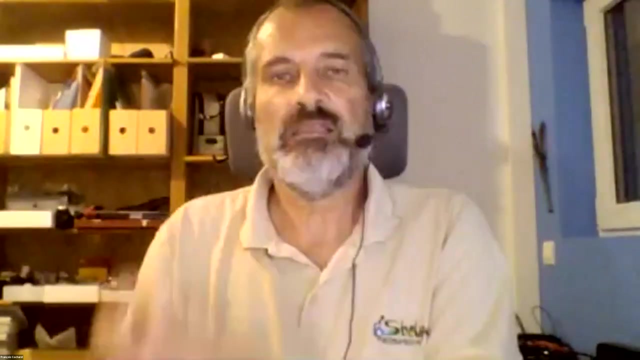 to do that because we are doing a survey of these kind of stars- B stars, for instance, for the best program, And so we have good reasons to do it. But the most important is that we keep this observation in memory. We put that in a database that can be used by anything else, by anybody in the world. 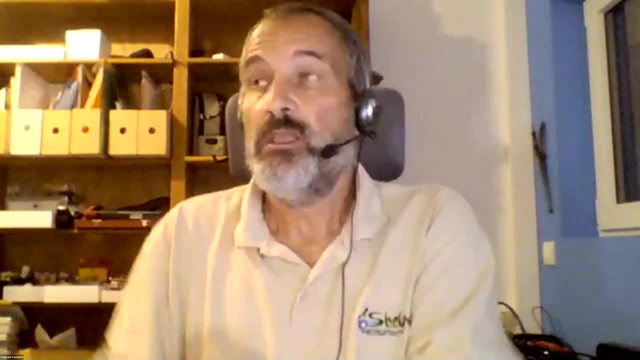 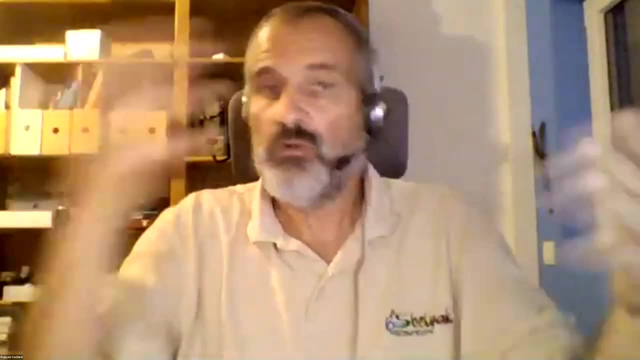 And it may happen, And it may happen that this observation will be useful in 10 years from now, because there is a star that is exploding somewhere, I don't know. We need a reference to measure the period of a variable star, or something like that. 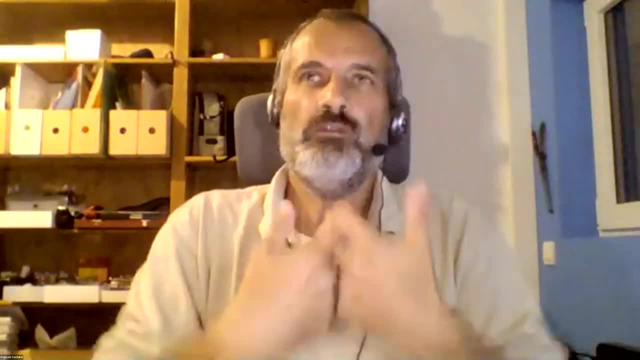 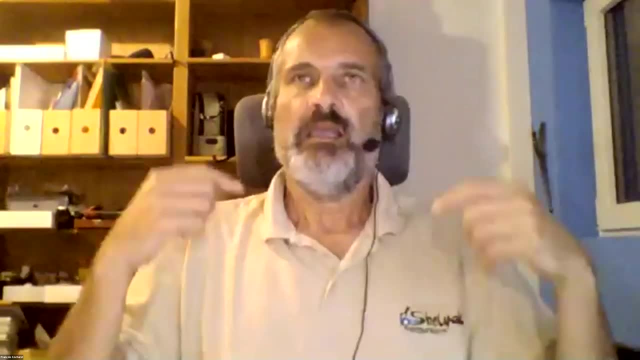 And in this case it's important to say that. okay, so when I do my observation, I do it for my own need and I know why I'm doing this observation, But on top of that, I will put it in a generator. 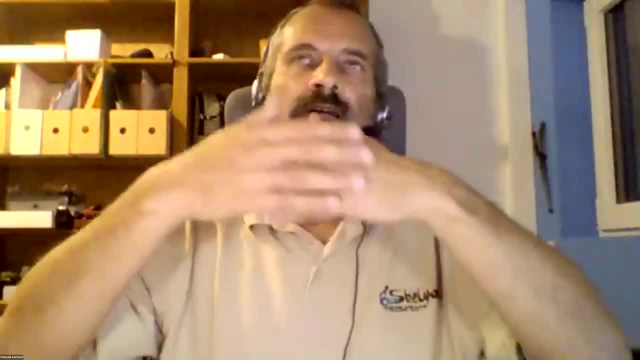 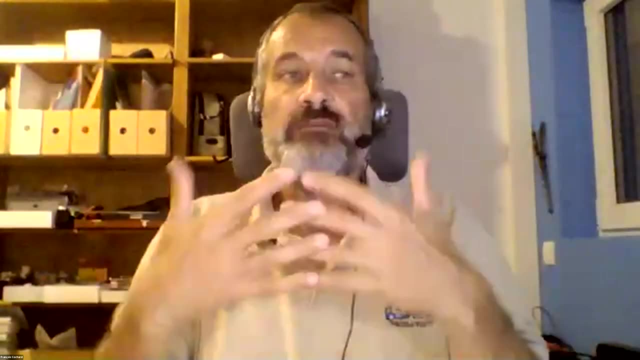 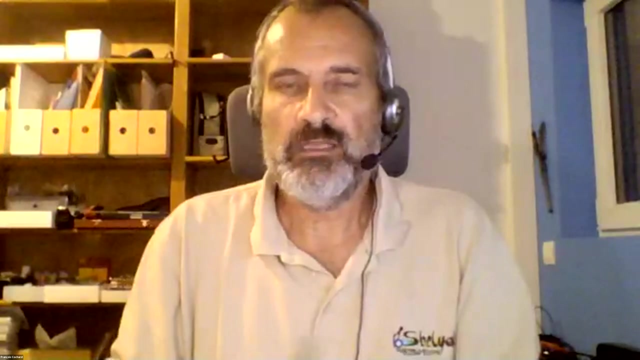 I will put it in a generic format and make it. I will do my best to make the best possible corrections to have a good observation that can be used by anybody And we don't know why it will be used for. Okay, So, and in this case, it is better to have a data reduction process which is still to 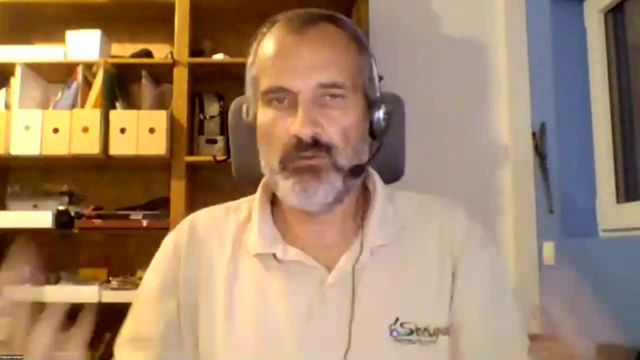 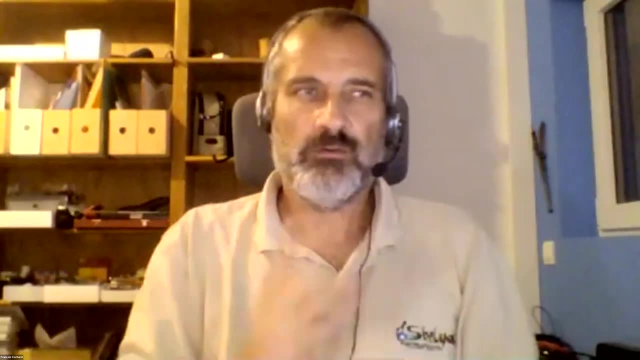 make sure that we have a good correction of the instrumental effects, a good wavelength calibration and so on, Okay, So that we can do something as pure as possible to be used by anybody. You know, if you look at, this is something that was very surprising to me when I started. 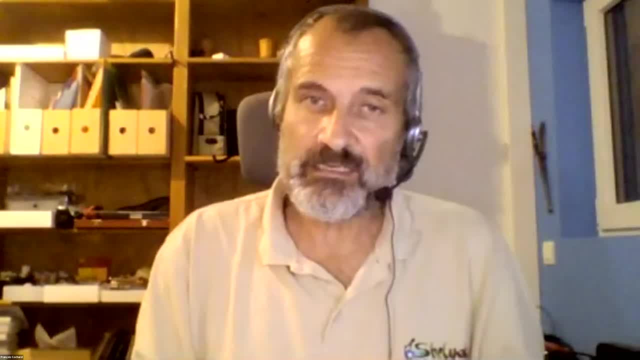 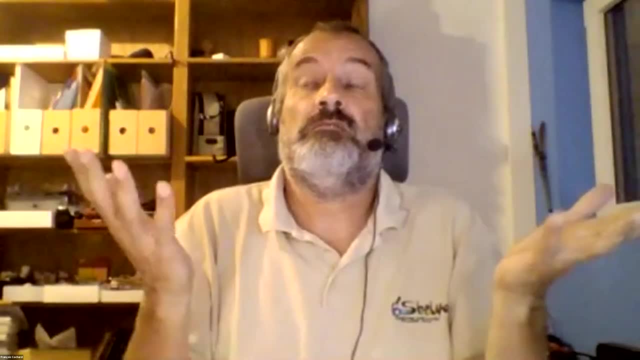 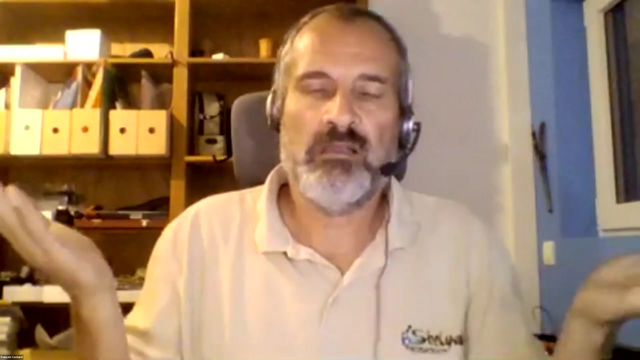 in spectroscopy We looked at some professional data- professional data, so very high level data- And in some of them we have seen some poor. it was a PT, so it was bad. bad measurements And you say, hey, professionals are not good. 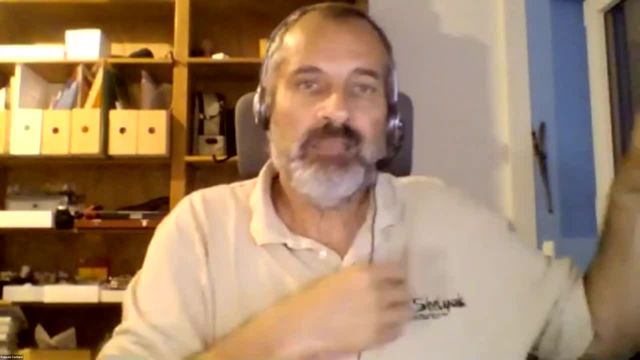 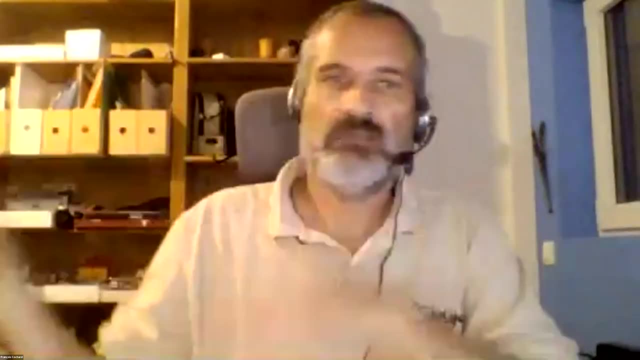 And in fact, if you, if you look at the reason for that, it was done for a given purpose, for a given goal. That was absolutely not, for instance, the wavelength calibration. So they didn't care. And so we say: oh, there are bad measures. 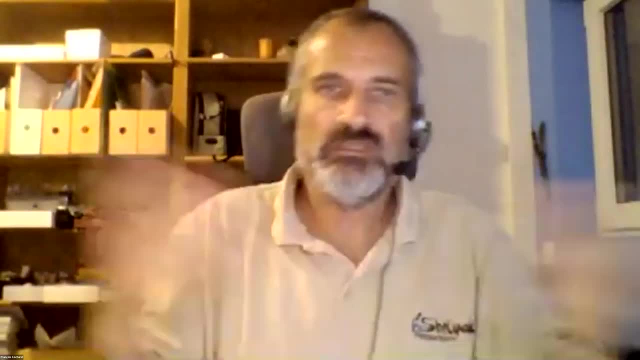 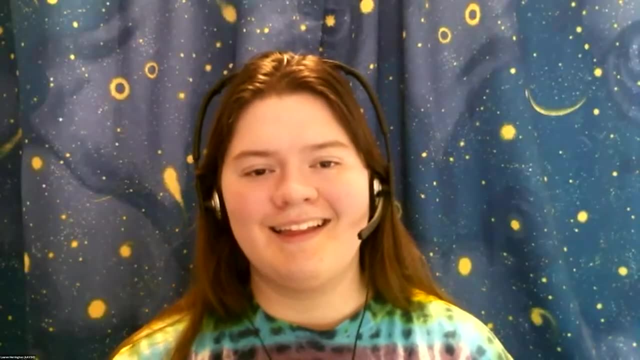 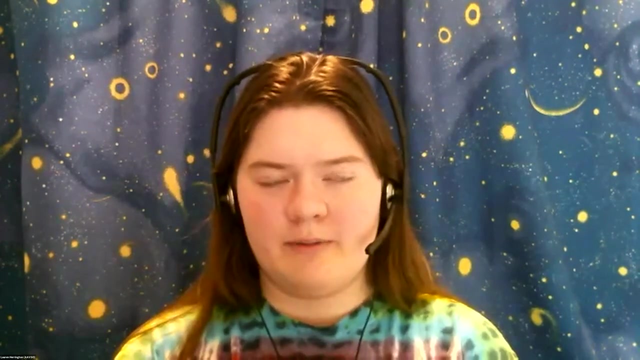 No, they are not bad measures. There are measures that was made for a given goal, which is not mine today. Good enough for its purposes? Yes, Yep. And I would like to add on to that that the AVSO spectroscopy database, AVSPEC, will. 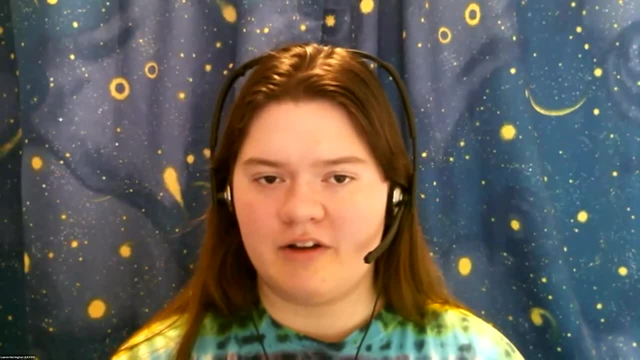 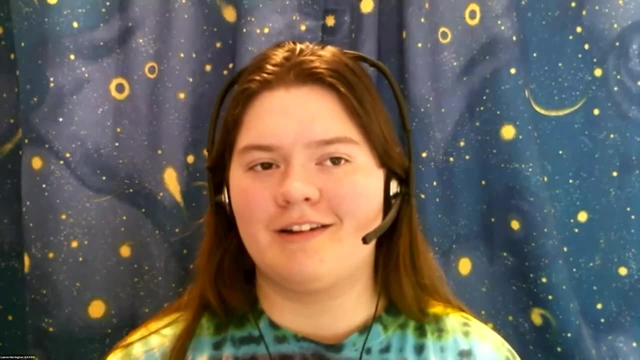 accept non-instrument response corrected spectra as well as instrument response corrected spectra. You're correct, Francois, in saying that it's you know. you should aspire to instrument response correcting your spectra so that they are most useful for people in the future. 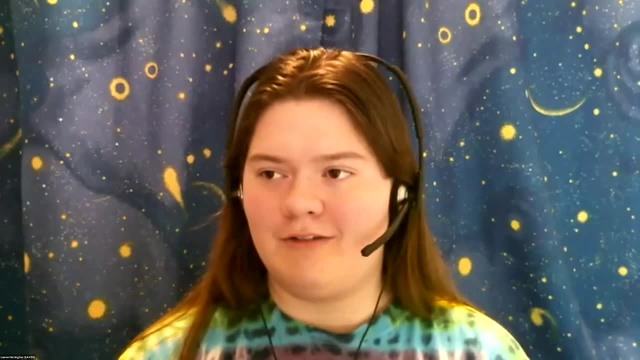 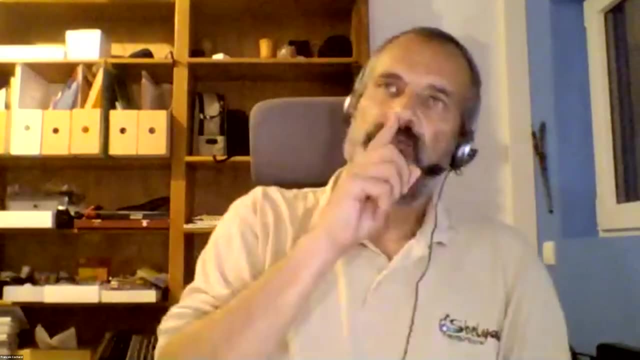 But we do, we do encourage you, you know, even if you forgot to take a reference star spectrum or something like that, We do encourage you to submit your spectra anyway. And also, something that I can add here is that, in fact, the correcting, the correcting, 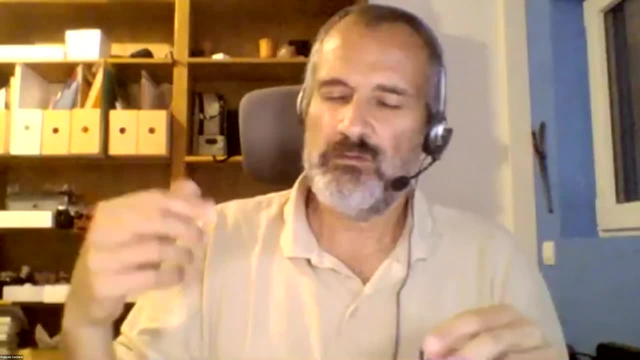 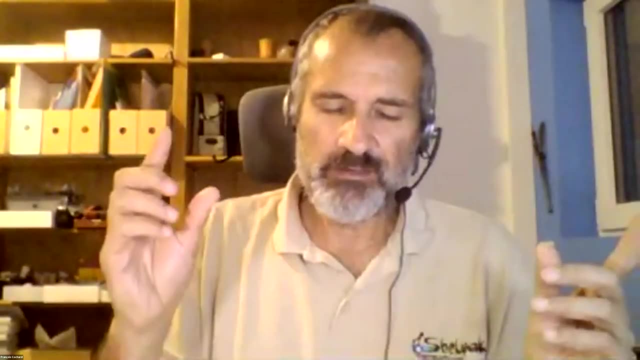 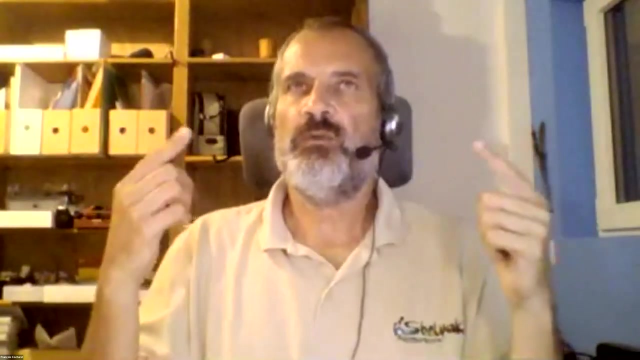 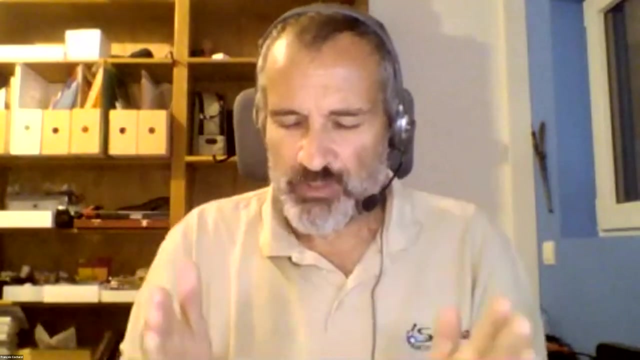 or not, the instrumental response, response, well response, for instance. sorry, this is something that belongs to the data reduction process And in fact you have to understand that. when you become a little bit rigorous, you will see that the data reduction process is linked to the instrument more than to the observation. 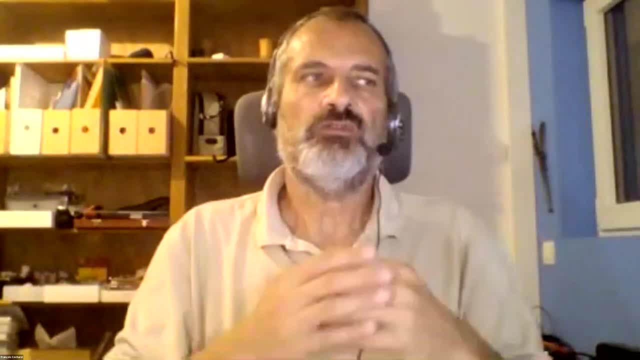 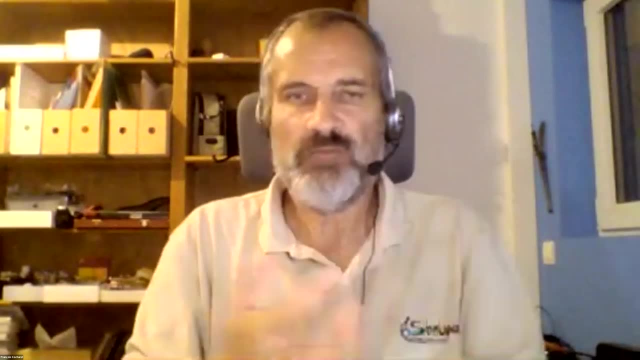 Okay, So if you have an instrument, you should always process the data the same way, And then the intrinsic quality of the calibration, the response, correction and so on is always the same. It depends on your instrument, And the data reduction process belongs to the instrument. 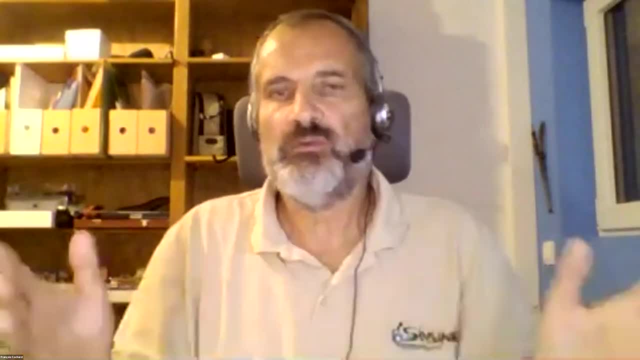 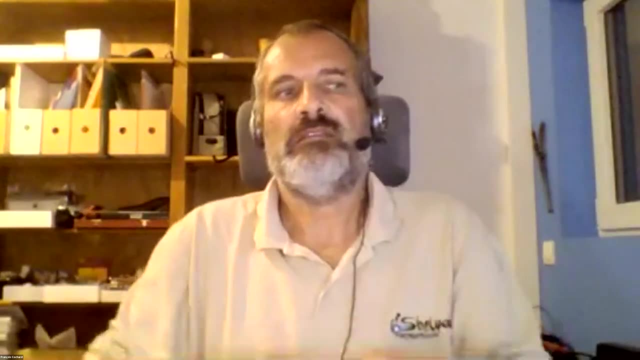 Okay. So whatever is the observation you do, you will always use exactly the same process. It will be easier for you, It will be more repeatable And then, in this case, it's better to include this response correction. I hope I'm clear enough. 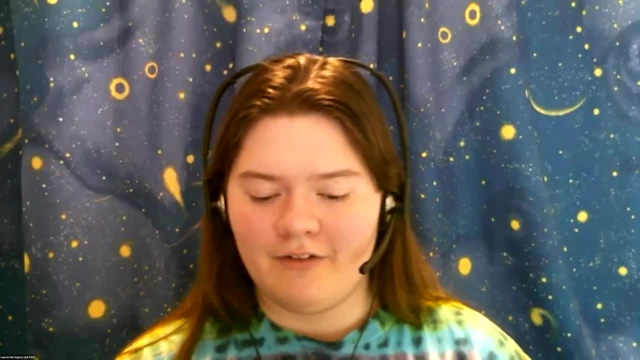 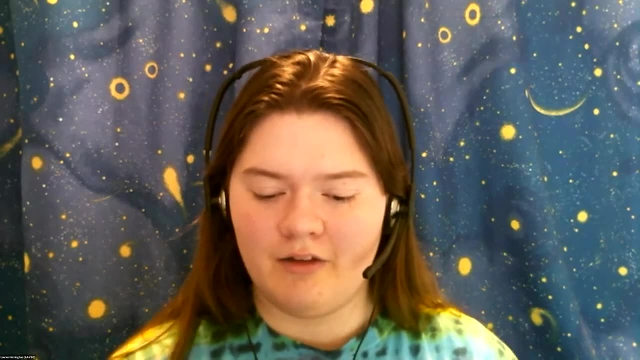 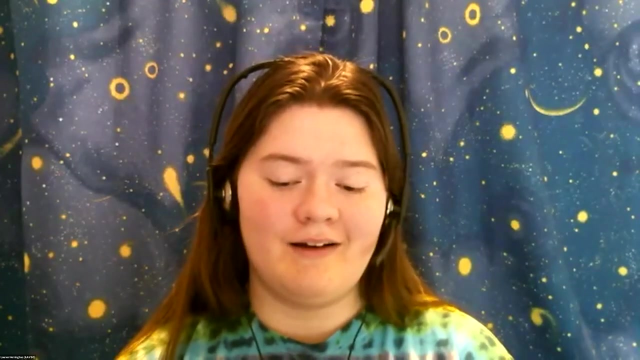 Thank you, I think that was quite clear. So our next few questions that we're going to take are on the topic of equipment. So first of all we have a question from Conrad Cardano, Who has asked: is there any company that is working on an objective grading spectroscope? 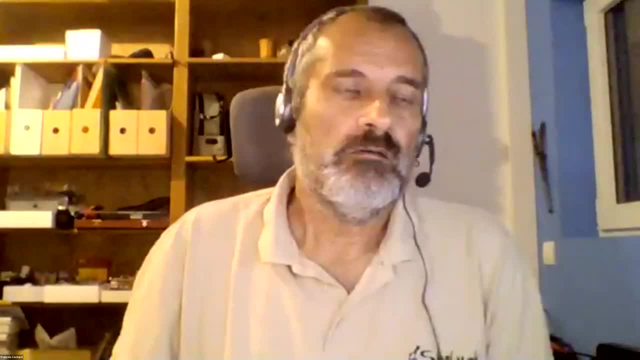 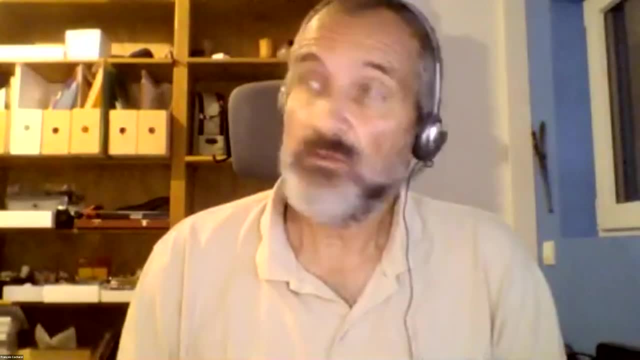 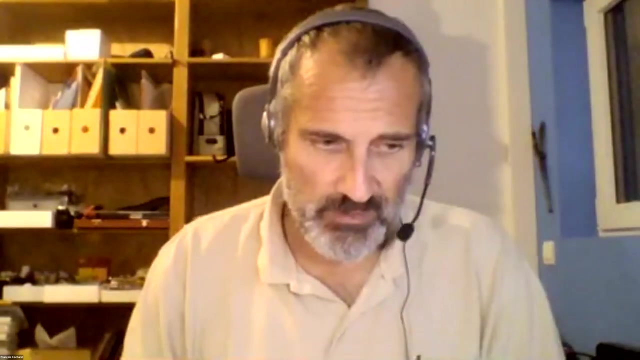 for a telescope? Well, I don't have a clear answer. I know that we don't have such a device. Well, the only grading we have is the STER analyzer. I know that some people put the STER analyzer in front of the lens of a telescope. 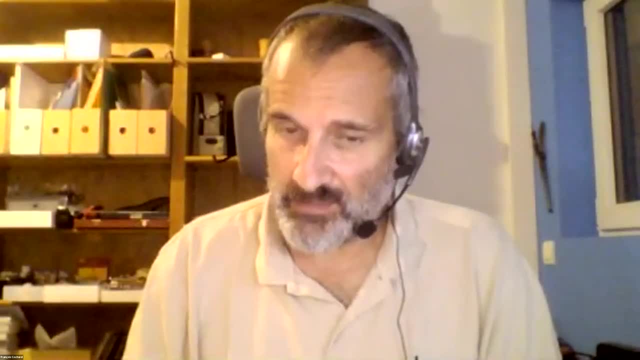 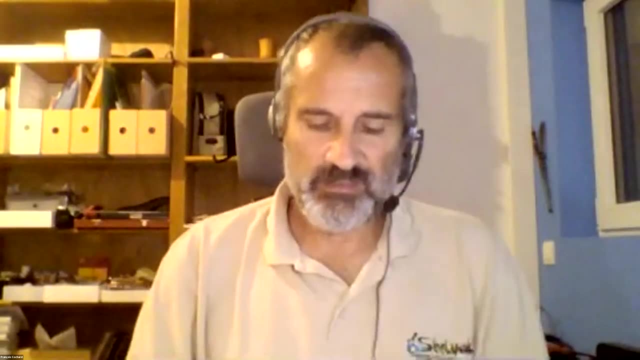 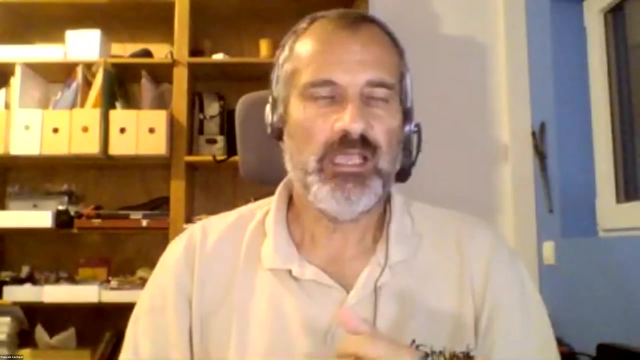 So it's a device of DSLR, for instance, and it works, But this is what we call the objective grading. But I know that the problem with STER analyzer, for instance, is that we are very limited by the maximum diameter of the system. 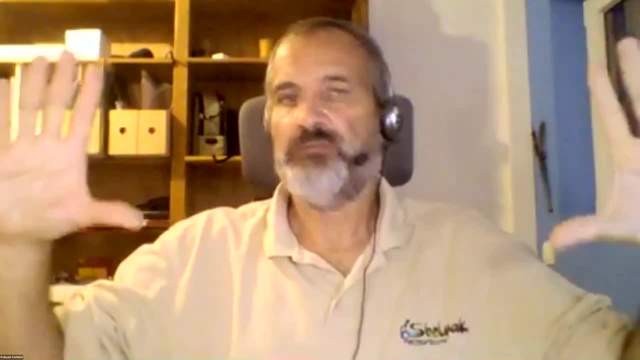 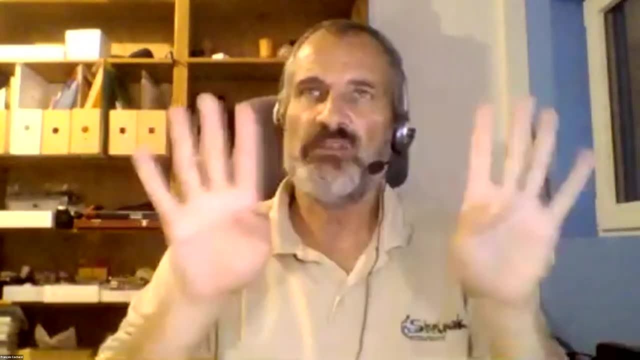 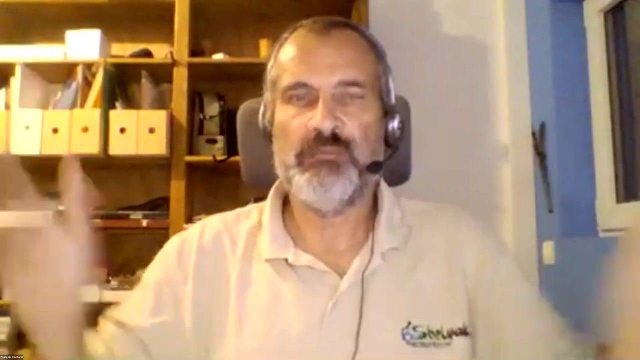 And of course, if you want to put a grading in front of the telescope, it will have a huge diameter And the price is huge And you have to have something early And keeping the same density of lines all along the whole diameter. 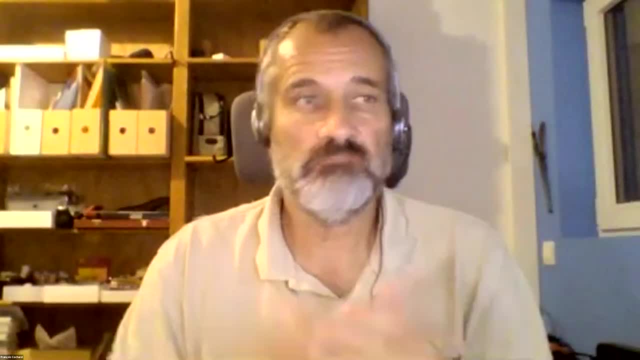 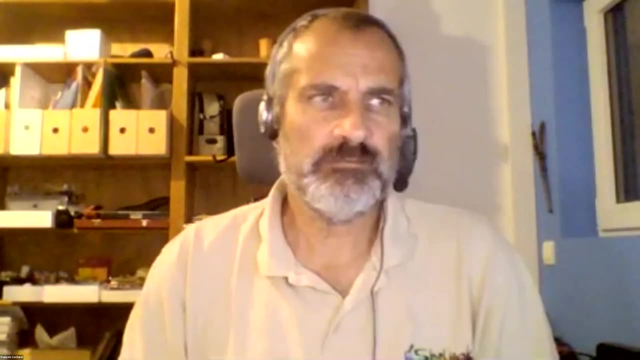 And then this is something I've never seen. it, In fact, I don't know. I know that we have some prisms- objective prisms- But well, I don't have a lot of experience in that. Yeah, I have not seen anything like that either. 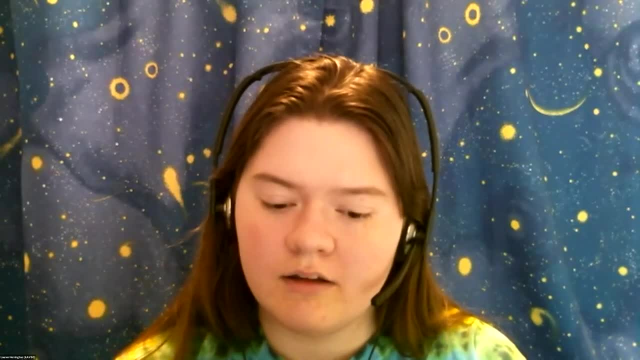 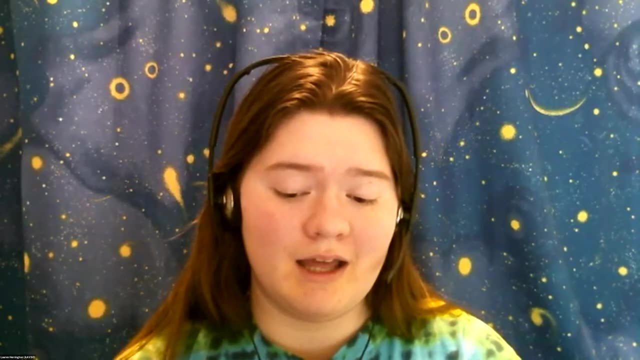 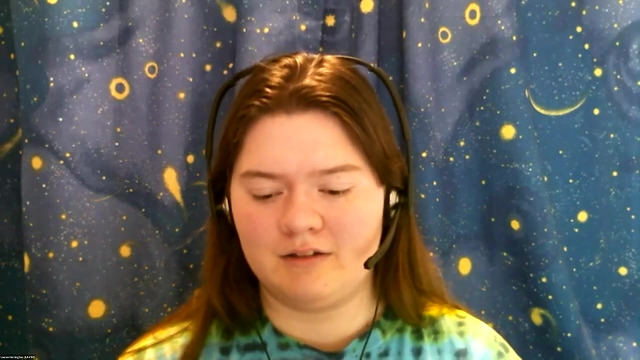 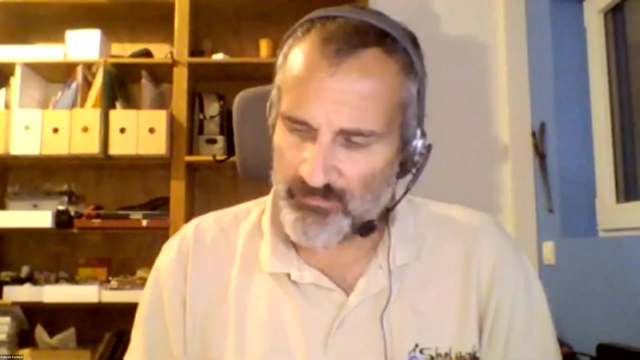 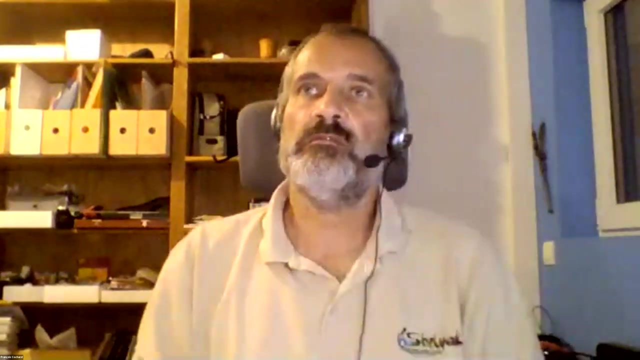 All right. Next question from Michael Nuss: What real world results or differences are there between a purely reflective system such as an RC versus one that incorporates lenses such as a Schmidt-Cassegrain? Also, this is a good question. If you have a purely mirror instrument, the direct effect is that it is achromatic. 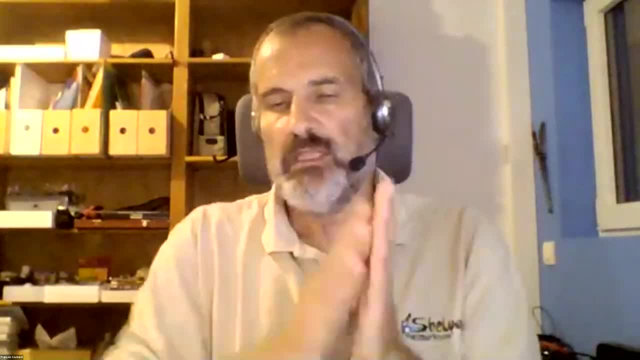 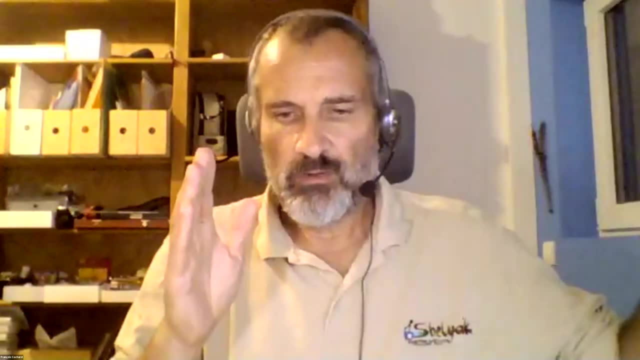 Achromatic means there is no chromatism And the chromatism is the effect that makes that if you take a lens, for instance, if you take all the red rays, they will not focus exactly at the same plane, at the same focal. 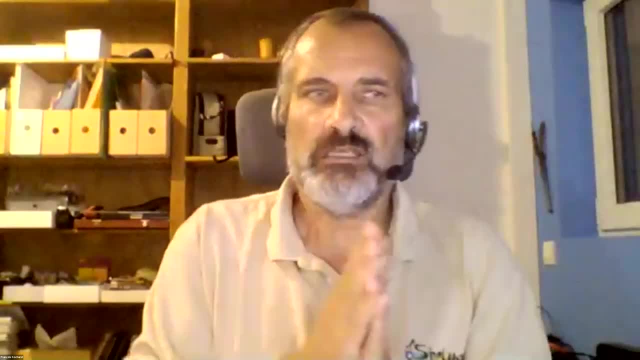 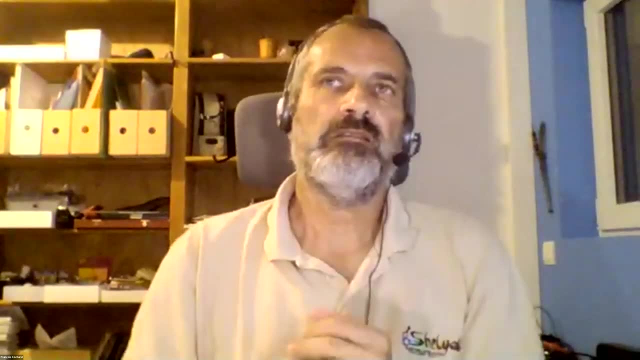 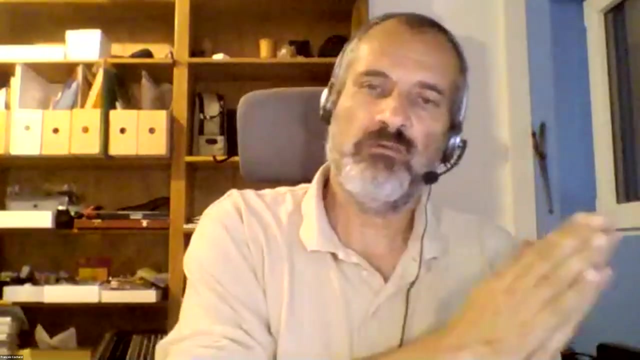 plane as the blue rays, Okay, And then, depending on the way of the wavelengths, you will not have exactly the same focal plane, And so this is what we call the chromatism, And of course, the result is, if you want to observe from far blue to far red with glass, 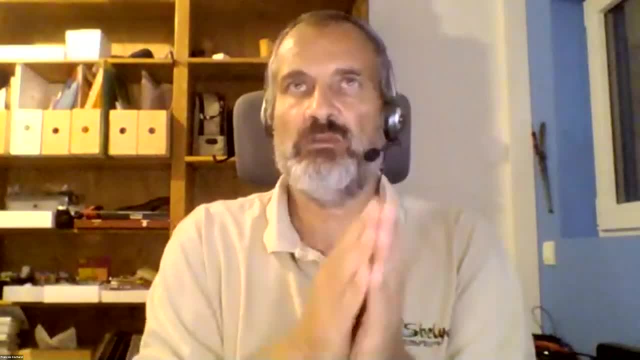 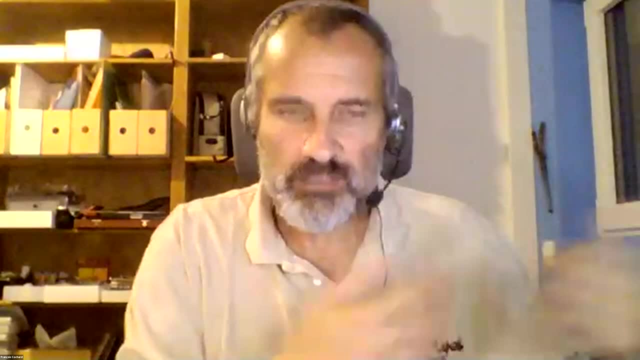 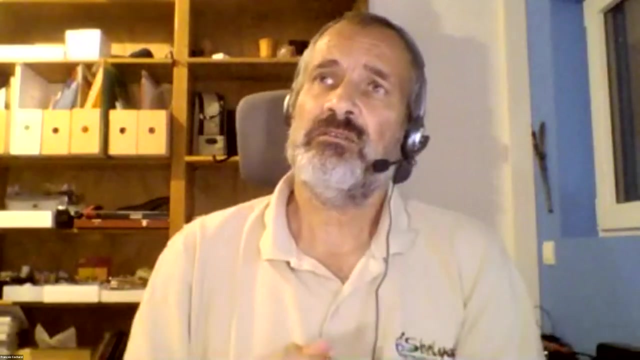 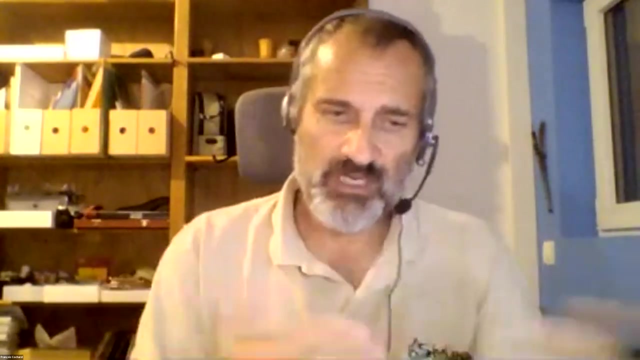 it is very complex. Okay, It is very difficult, And especially when you do optics, the problems appear mainly in the blue part of the spectrum. Okay, If you can see it, we have seen some very odd optics And for each the blue part was poor, in fact was bad. 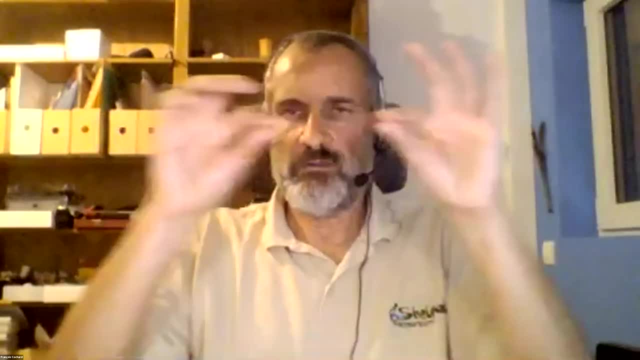 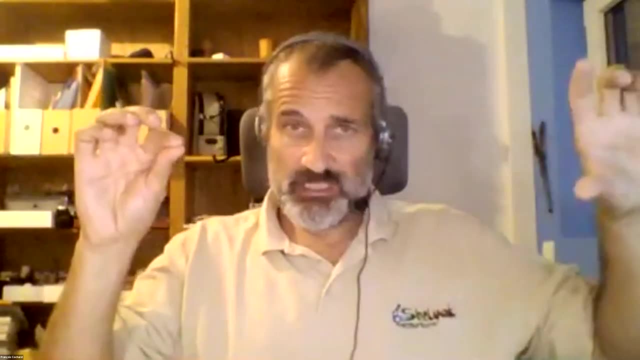 And the result is that if you take the spectrum, this is not a thin line, But when you arrive in the blue part it becomes wider, And this is what we call the fishtail effect, because the spectrum becomes wider in the blue part. 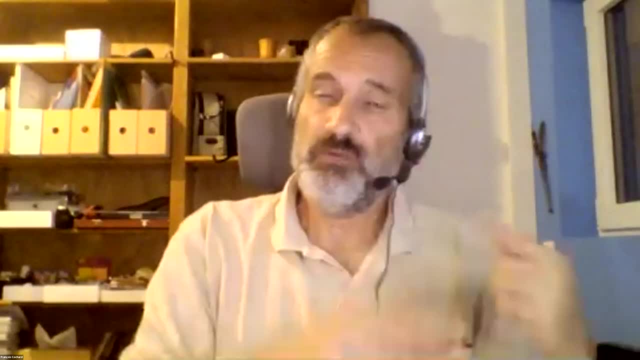 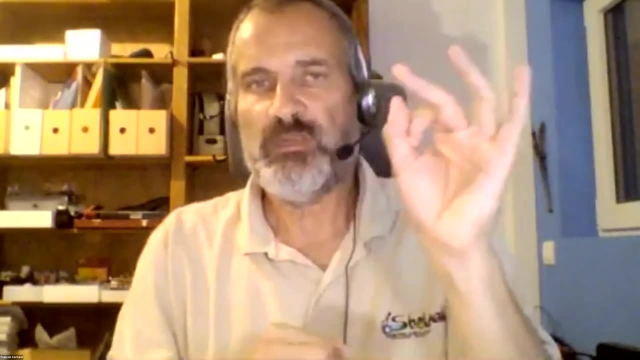 So it's not necessarily a big deal, but you will lose some resolution for sure, You will lose some light for sure. So you can imagine that if the spot in the red part is very well focused on the slit, so all the red energy will go in the slit. 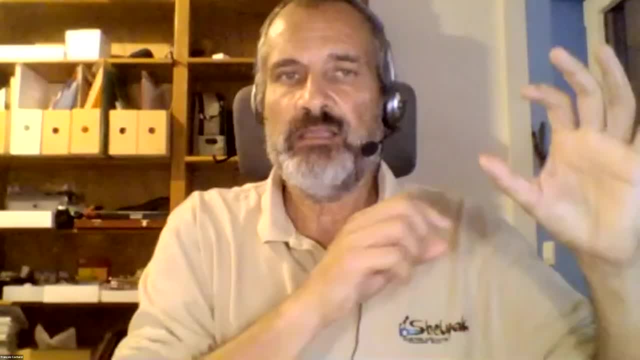 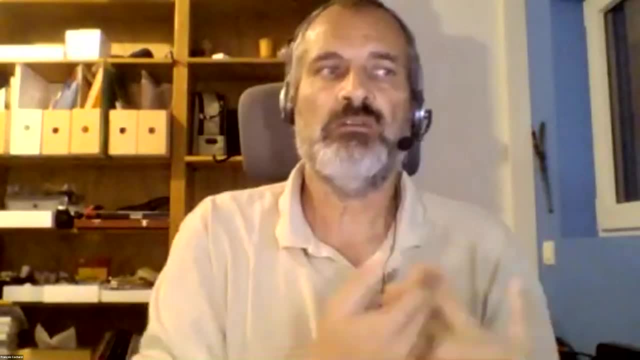 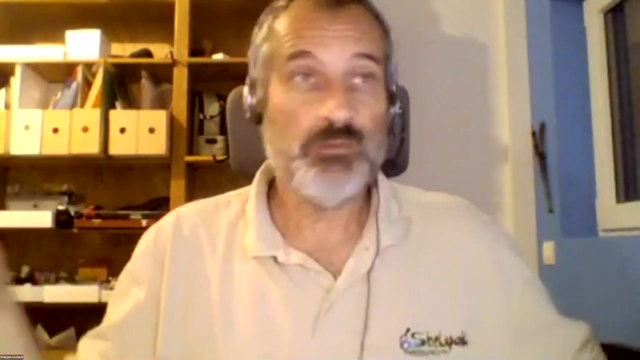 But if the blue is bigger, then only a few percentage of the blue rays will go into the spectroscope. So we lose some sensitivity and you will lose also some resolution. So it's better to have something achromatic Now if you are observing in high resolution in blue or red. 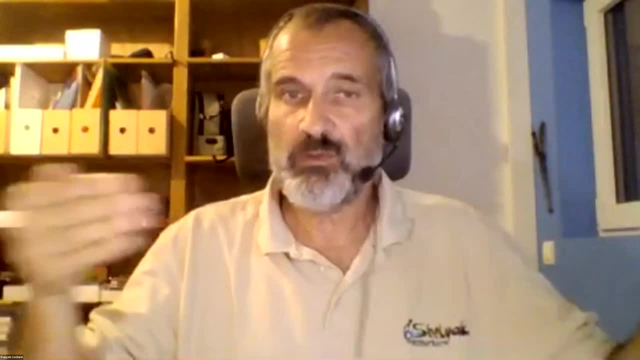 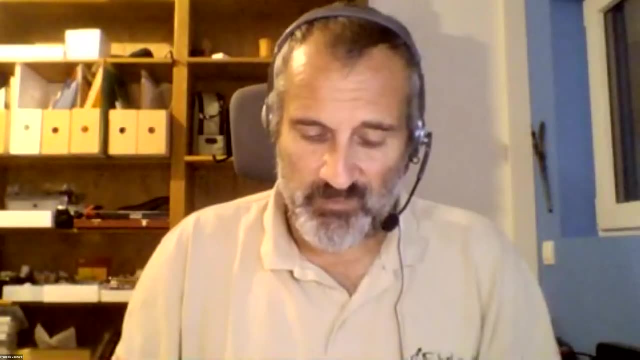 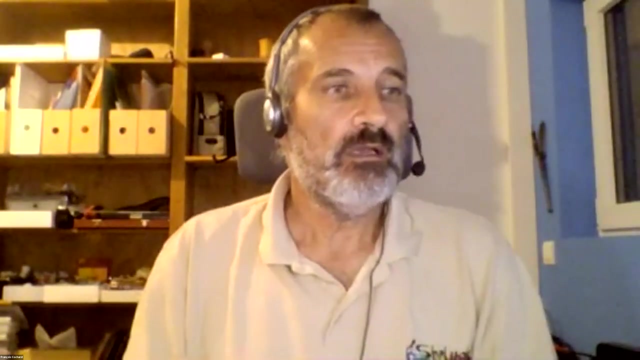 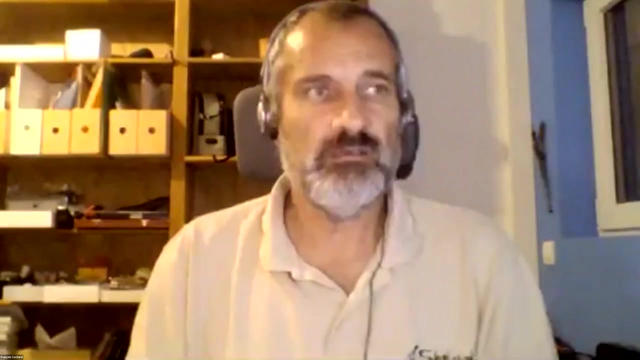 it's not a big deal. You just have to refocus or to focus differently if you have this kind of instrument. So, to make it short, nowadays we like to go more and more towards the blue and the infrared, And this is really one of the main reasons for which we have developed the UVEX instrument. 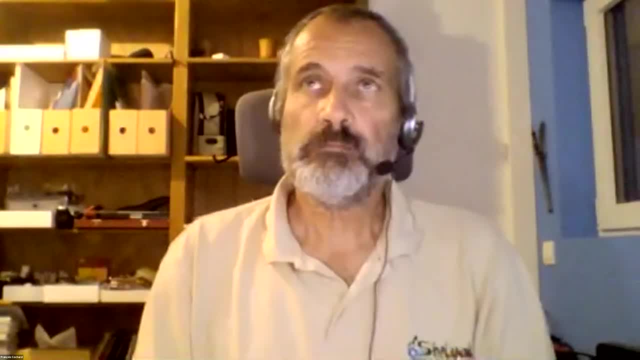 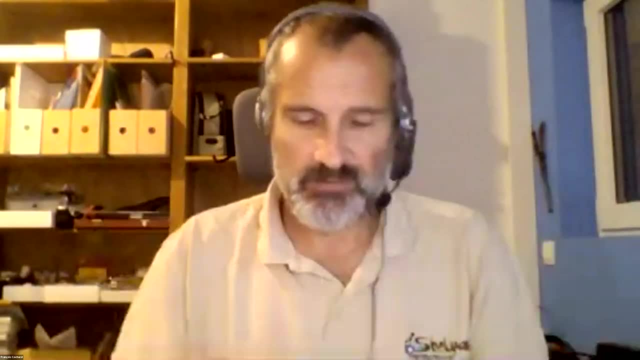 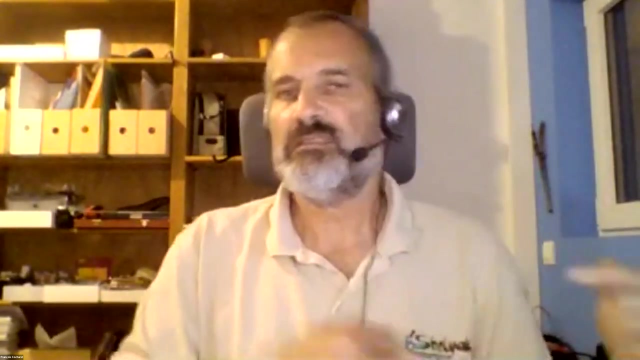 which is a purely mirror instrument also. So we use cylindrical instruments. We use cylindrical spherical mirrors for the collimator and for objectives inside the system. So the instrument, the spectroscope itself is purely achromatic. And if you use this with the purely achromatic telescope, like a Richer-Cretien for instance, 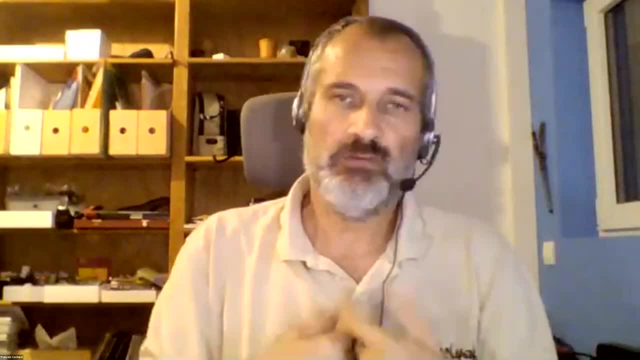 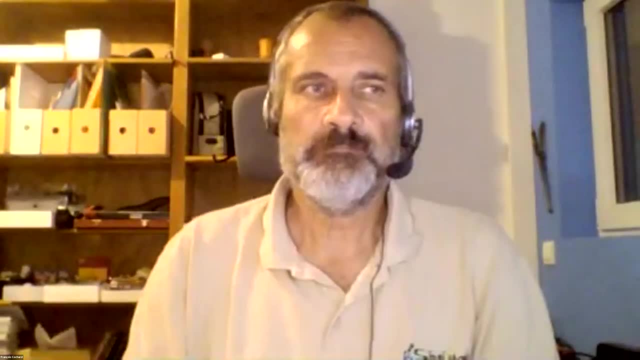 which is made only of two mirrors. there is no glass. then you have a perfectly chromatic instrument, And this allows us to go very far in the blue and very far in the red. Okay, All right, Thank you. Next question from Subhash Gadam. 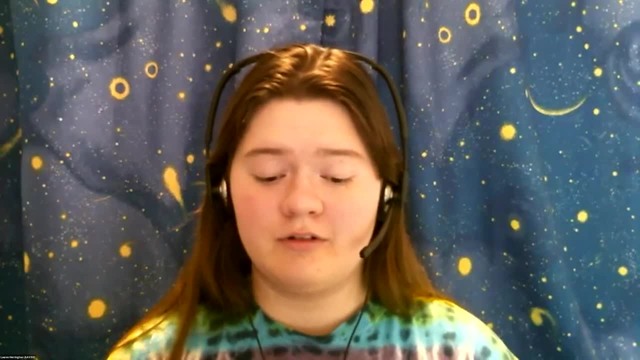 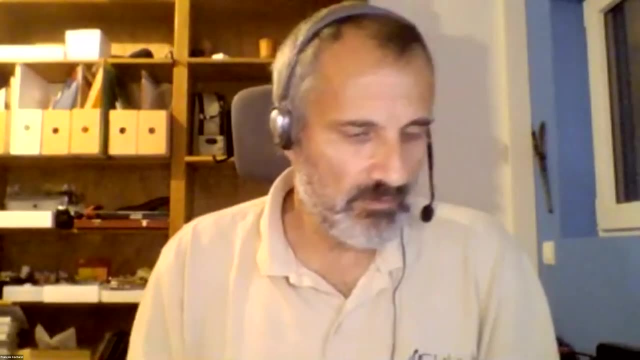 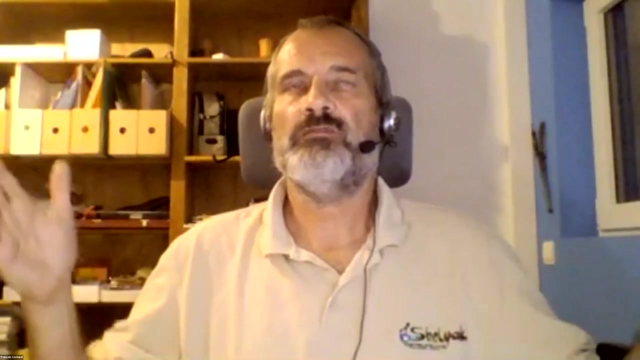 What is the typical width of the slit in a spectrograph? Well, in our instrument, in most of our instruments, the typical slit is something like 25 microns. Okay, So the idea is to have a slit which has the same width of the star image at the focal plane of a telescope. 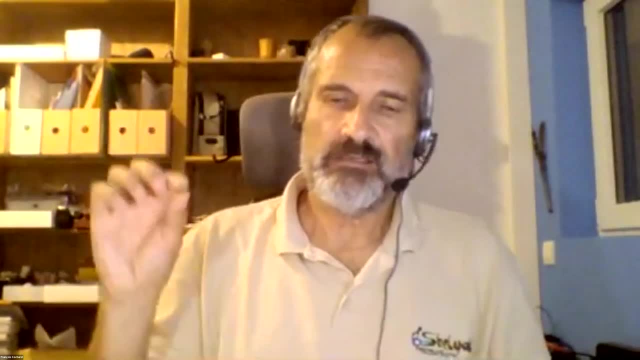 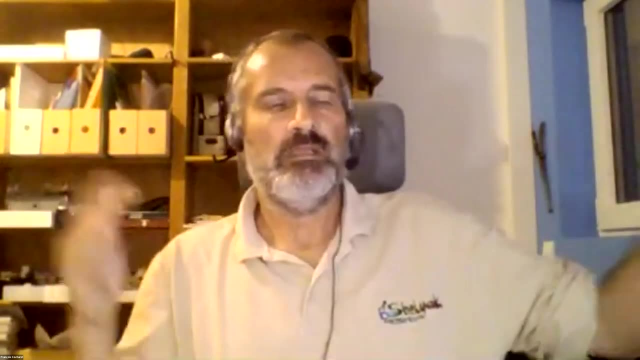 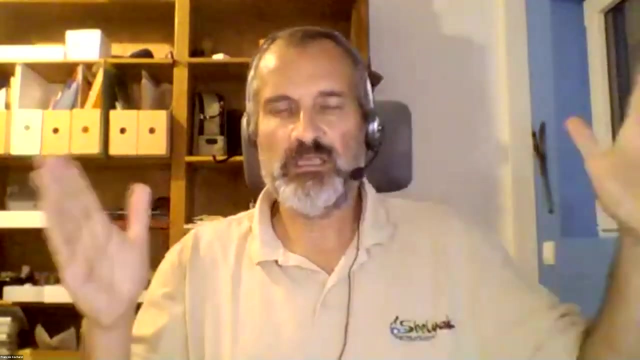 And so the star image size depends on two parameters. The first is the seeing of your observing sight. So if you have a good seeing, you may have less than one arc second of seeing, And in a more usual sky you would have something like three arc seconds. 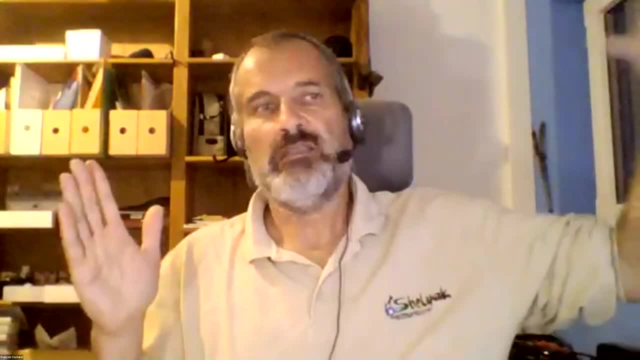 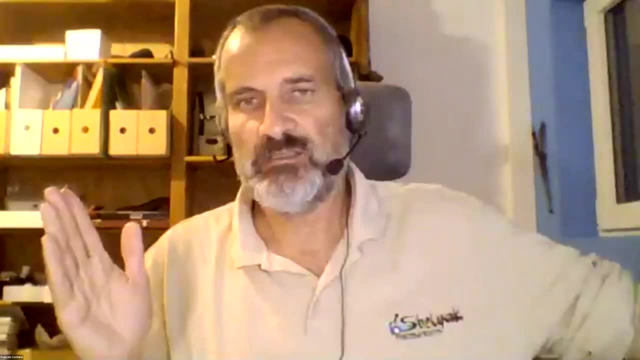 So this is due to the turbulence of the sky, Then the star image is not as sharp, As sharp as possible. And the other parameter is the focal length of the telescope. So if you have, generally speaking, if you have- a bigger telescope, you have a bigger focal length. 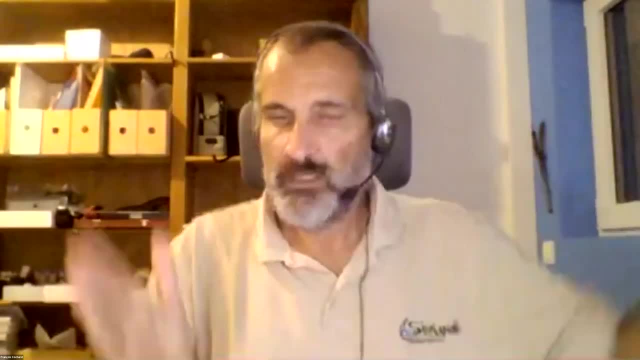 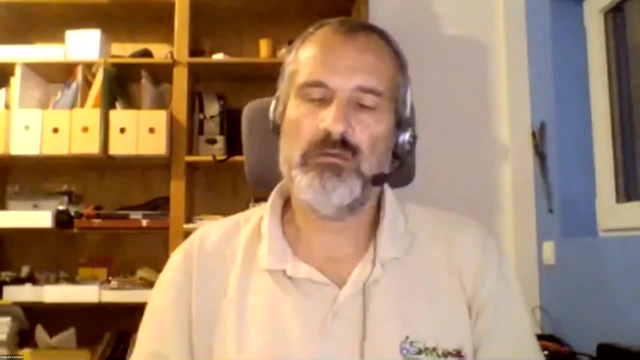 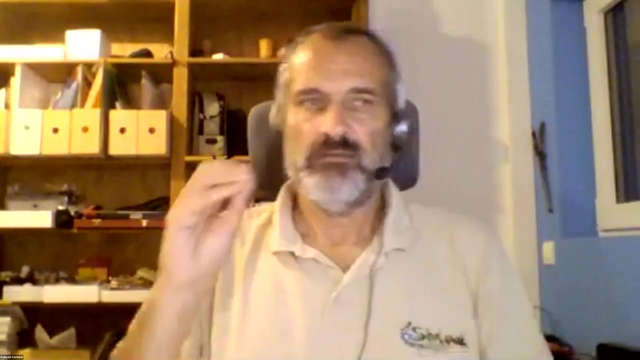 Well, even, of course, if it depends on the f-ratio. the key is really the focal length, But the bigger the telescope, the wider the slit image. This is the reason for which it's something absolutely key in spectroscopy, which is if you have a bigger telescope. 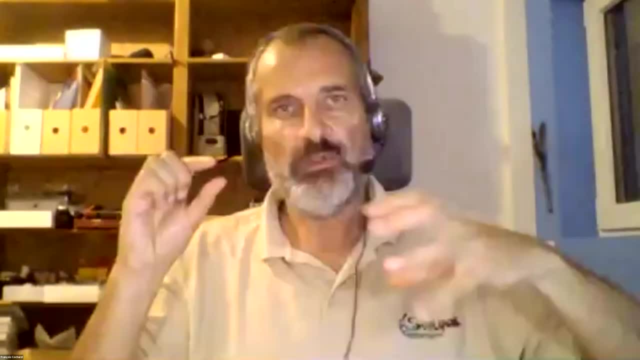 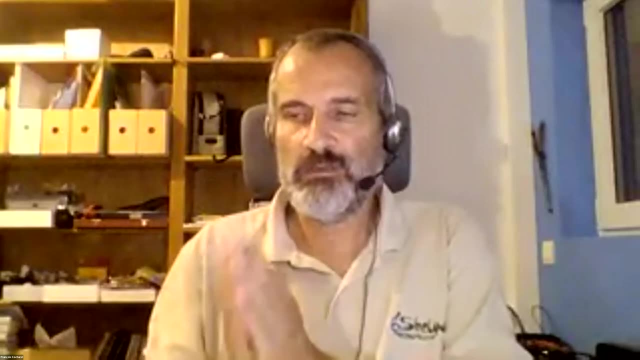 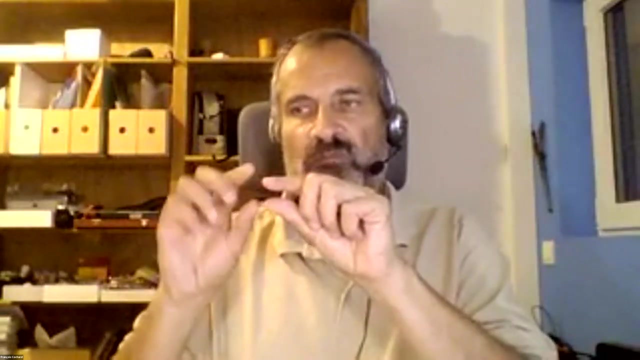 you will have to have a wider slit to catch all the light from the telescope. Okay, And this is not negotiable, Sorry, This is for optics and optical constraints And if you want, if you open the slit to catch more light and if you want to keep the same resolution. 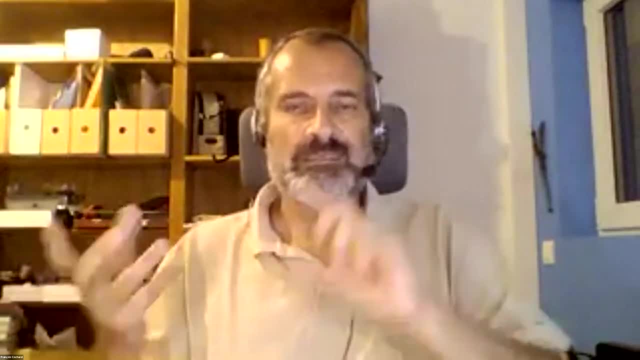 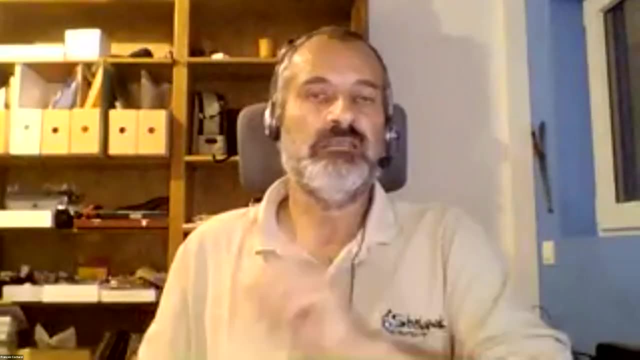 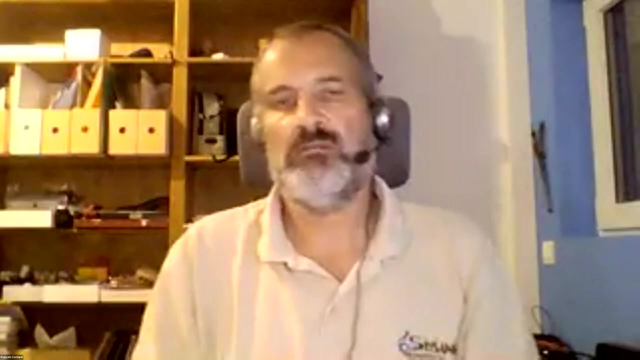 you will have to have a bigger spectroscope. Okay, So this is really: if the telescope is bigger for a given resolution, the spectroscope will be bigger. for this reason- And this is why we are lucky As amateurs- is that we are working with small telescope, which means that we can use small spectroscope to have the same resolution. 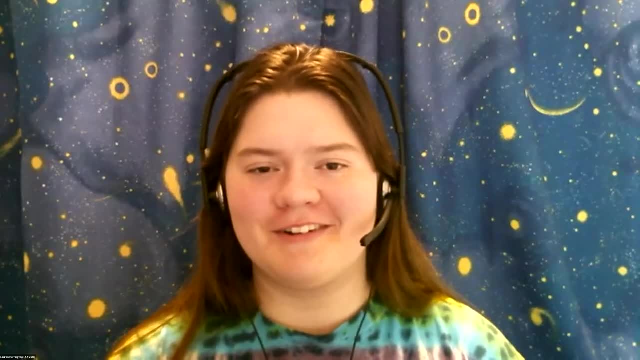 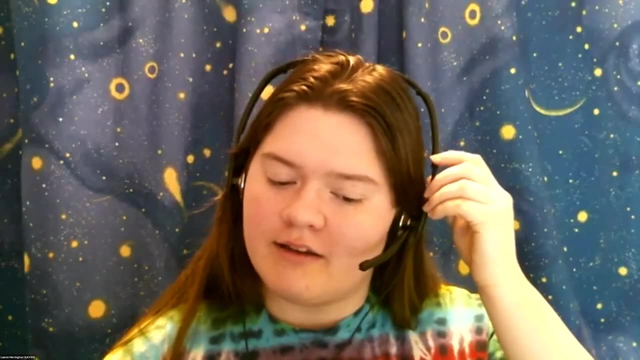 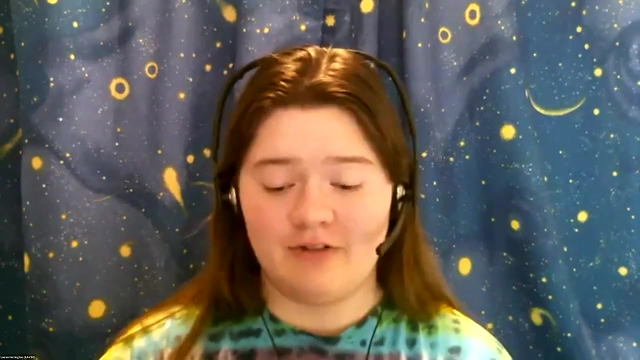 Instead of those spectrographs that take up entire rooms at major observatories. Absolutely, Absolutely, All right. So we've got actually two questions related to that. So first let's go to Bobby Napier's question. Does the focal ratio make a difference in the instrumental effects? 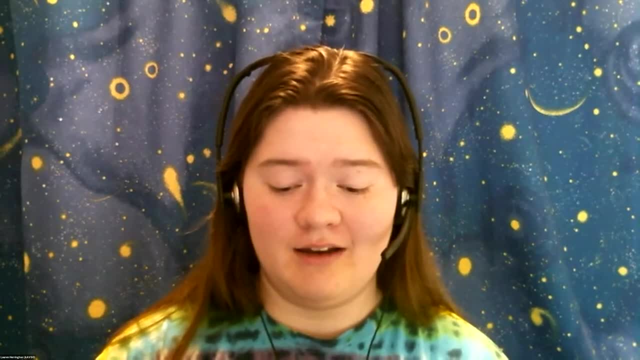 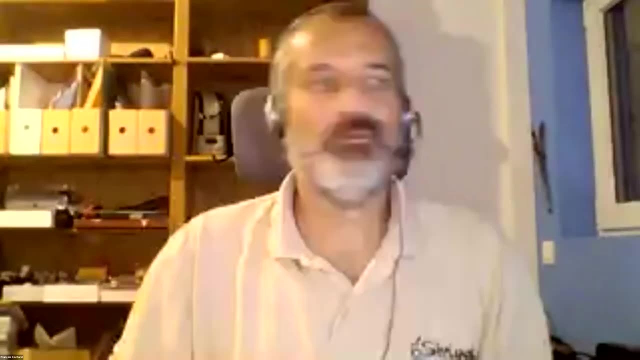 So what's the difference between an F10 Schmidt-Cassegrain or an F6 scope in terms of spectroscopy? Again, they are wonderful questions, So we can continue for hours and hours. Your questions are wonderful. Thank you very much. 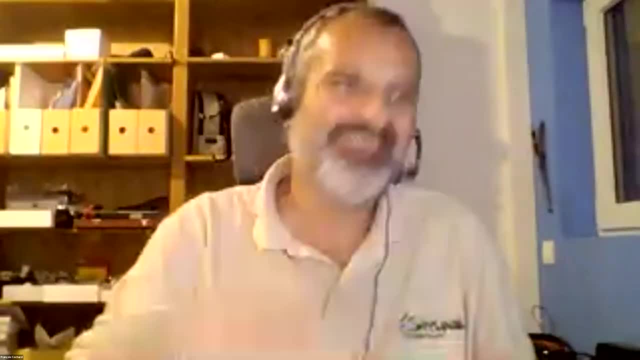 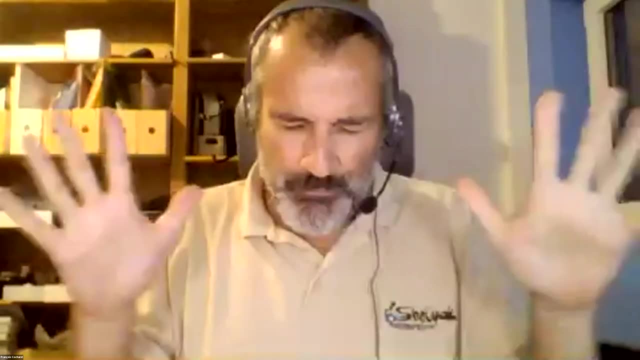 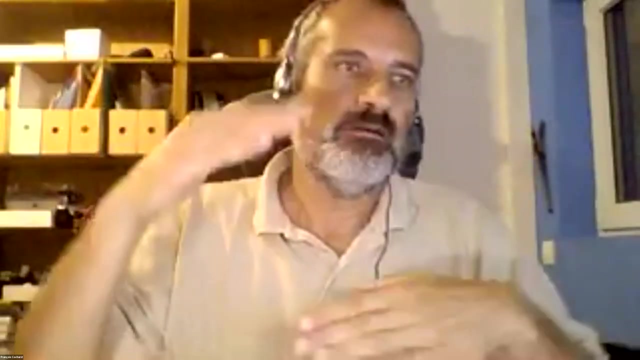 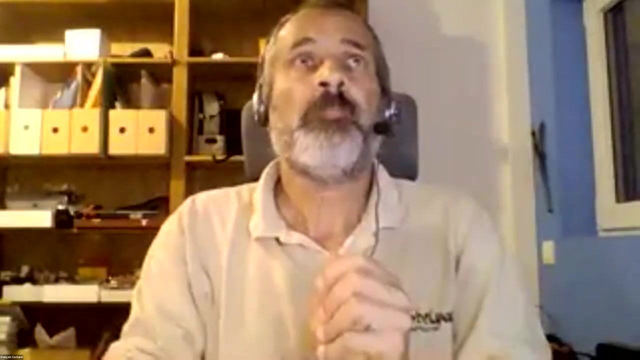 We have a little bit more than 10 minutes left. Okay, Thank you. This is, of course, well in two words. I try to make things simple. If you have a fast telescope, so say a Newton telescope at F5, F3, well, F5, F4, F3, well, F3 is really the maximum. Of course, for a given diameter you will have a shorter focal length. If you have a shorter focal length you will have a smaller image, star image size at the focal plane, And then you can close the slit and then increase the resolution. 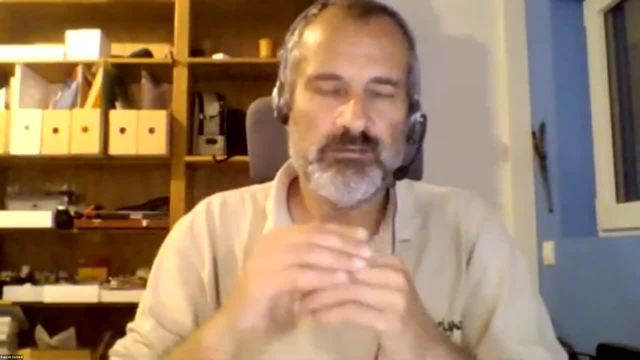 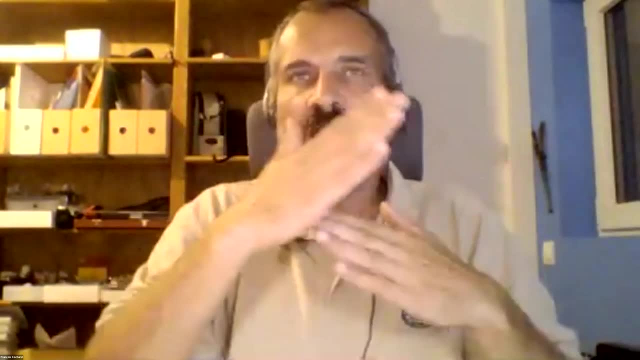 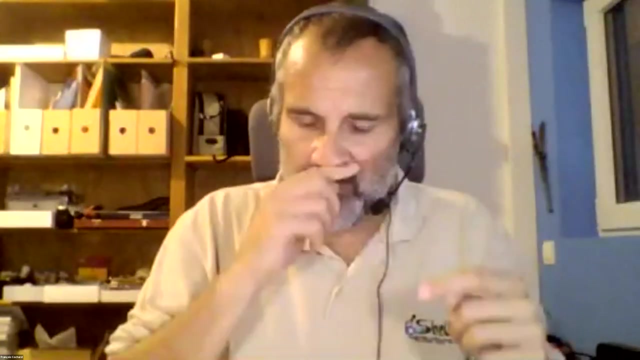 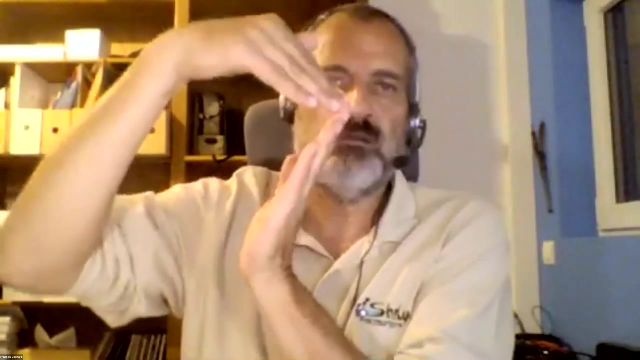 Or put more light in the slit. Okay, So this is really the key. So for a given diameter it's always better to have a fast aperture, low F-ratio. But the problem if you do that, if you have a beam like that in France with an F3 telescope for instance, it means that the optics of the spectroscope behind 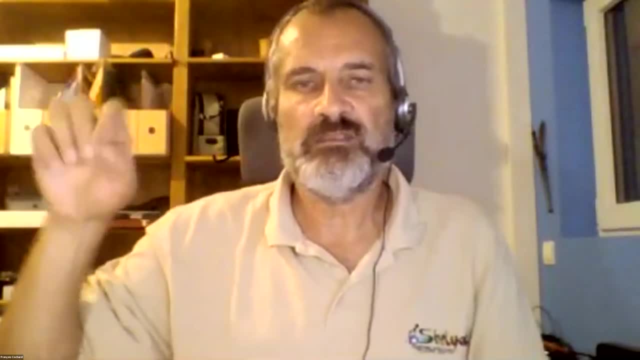 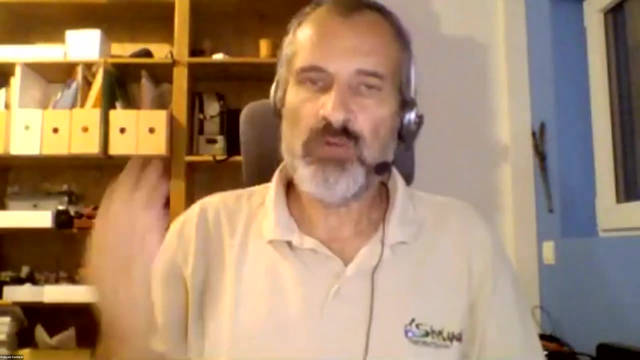 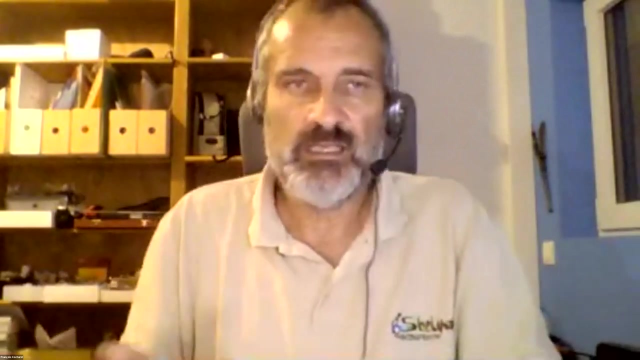 must be able to take all these images, So it must also have the same F-ratio. And having a high F-ratio for an instrument is always, optically speaking, it is always complex. This is the reason for which, in photo, if you take a photo lens, if you have for the same focal length of a photo lens, 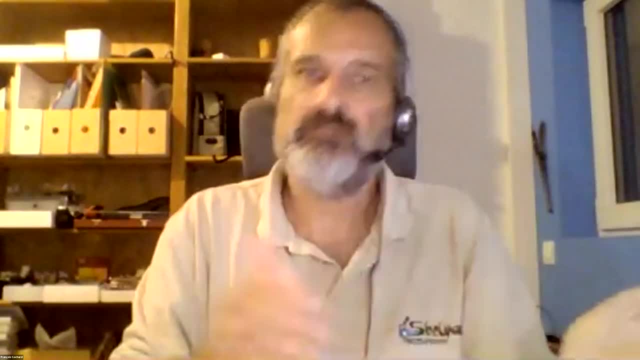 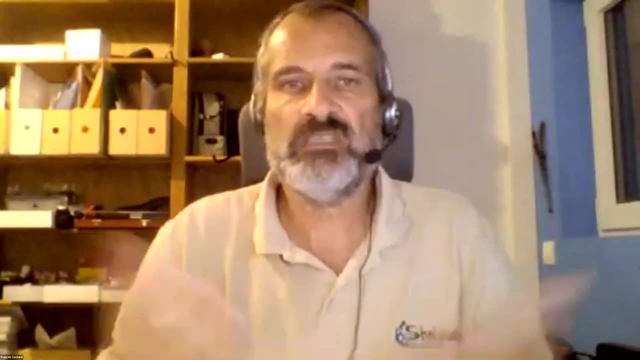 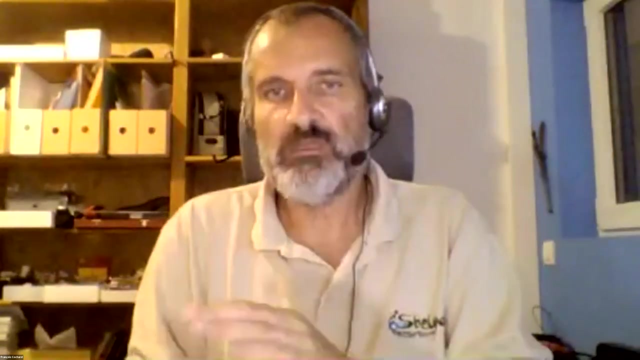 if you have an F2.8 lens, it would be much more expensive than the same wavelength, Same focal length at F4 or F6.. Okay, This is really because you need. it is more complex to manage a very open beam, a fast beam. 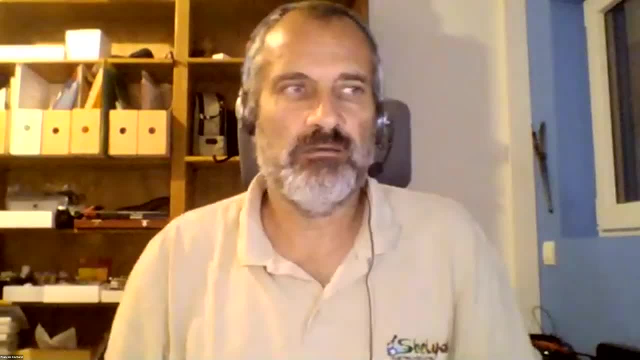 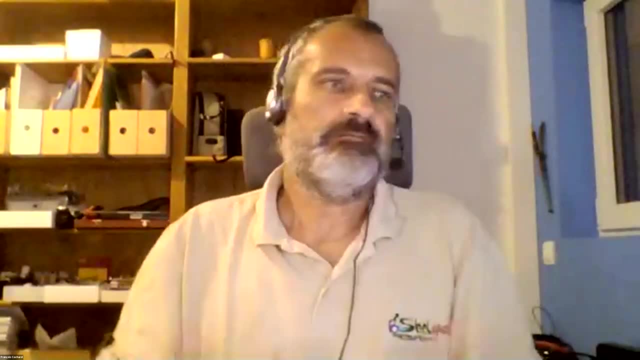 And it must be optically compensated by a more complex optic. So it's always a question of trade-off. Okay, It's really well, it's a trade-off. So for sure, in optics, if you want to go below F3,. 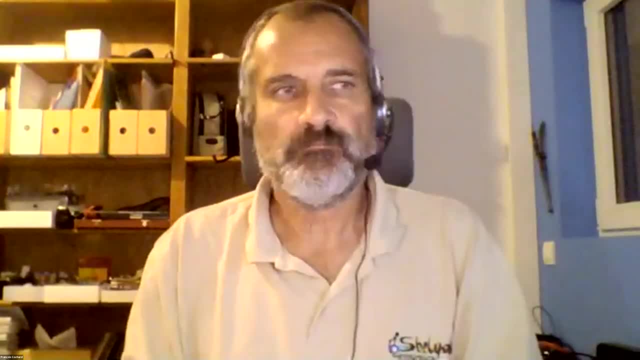 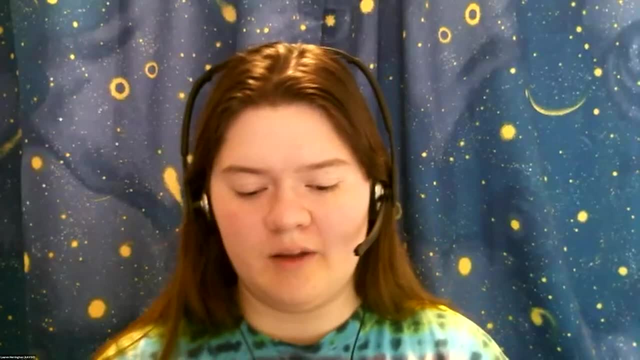 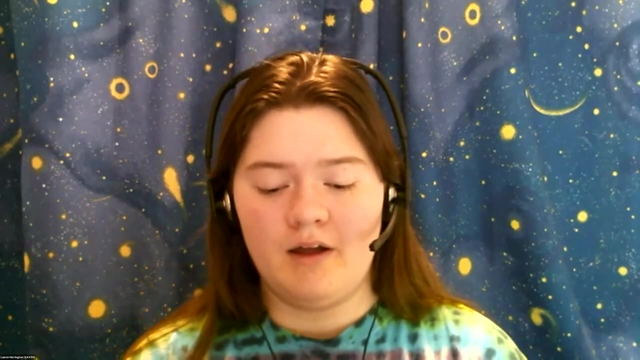 it becomes really challenging. Okay, That makes sense, Thank you, Okay. So Hamish Barker has asked on that topic: if a spectroscope needs a slower focal ratio than is available from your telescope, can you use a Barlow, or will that introduce too many chromatic effects? 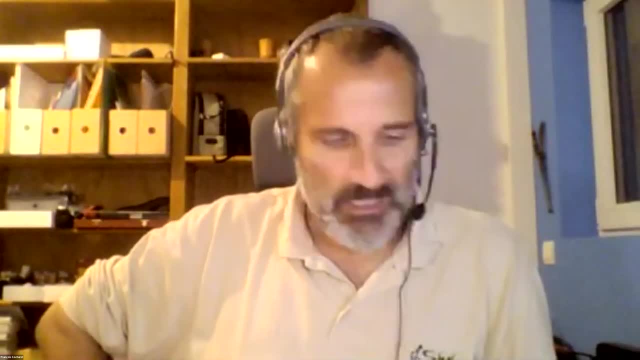 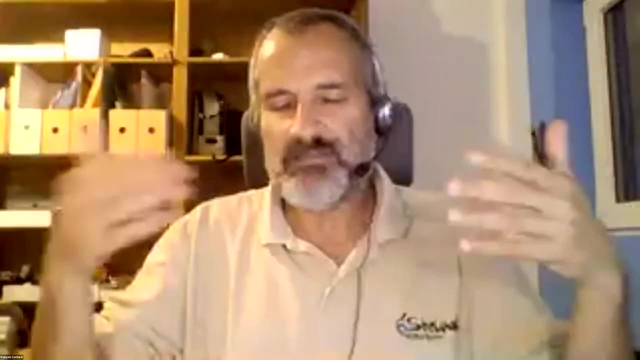 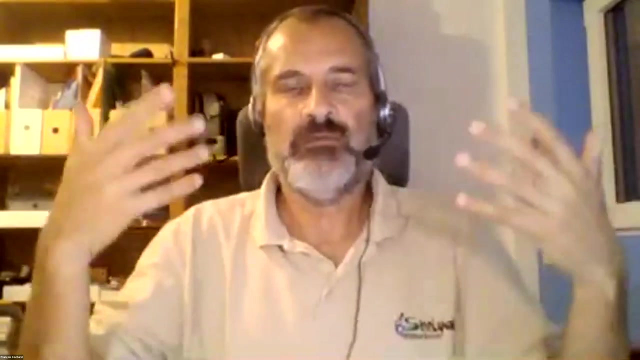 Of course, it's a good question If you have. well, if you, it's always better to have the right F-ratio, the same F-ratio for the telescope and for the spectroscope. This is the best way to have the optimal total efficiency. 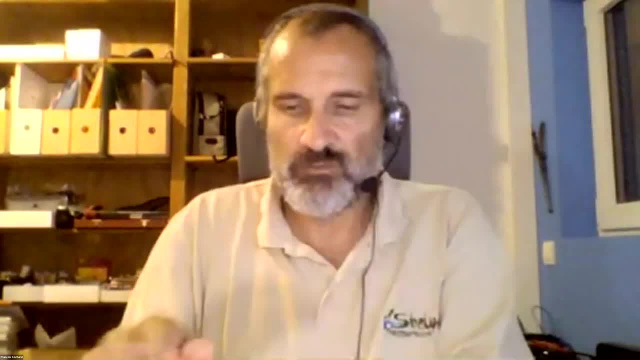 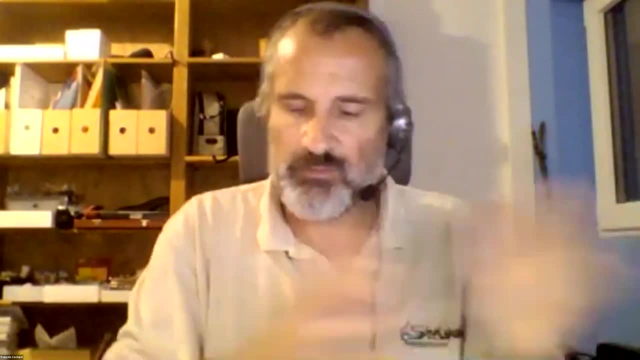 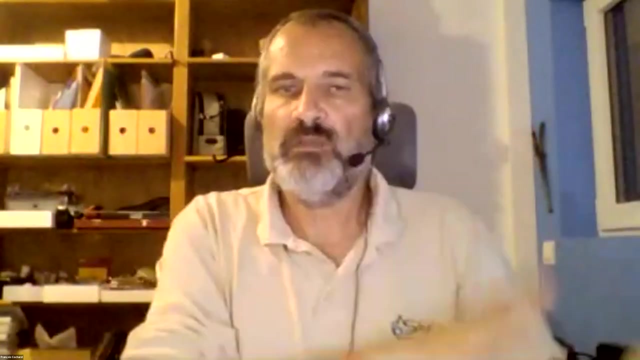 And so it's really it's important to look at the F-ratio of your spectroscope and make sure to match with the telescope And, of course, if you want, if you don't have exactly the right F-ratio, you can change it, either by reducing the focal length with a focal reducer. 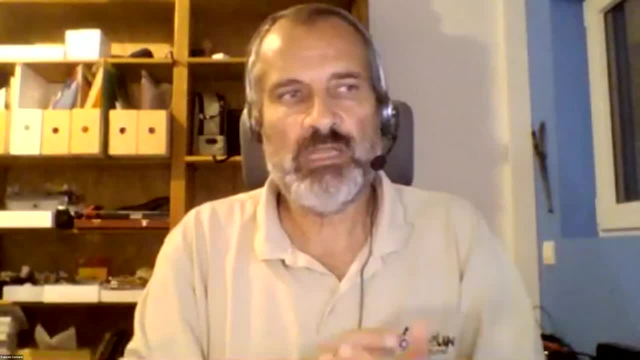 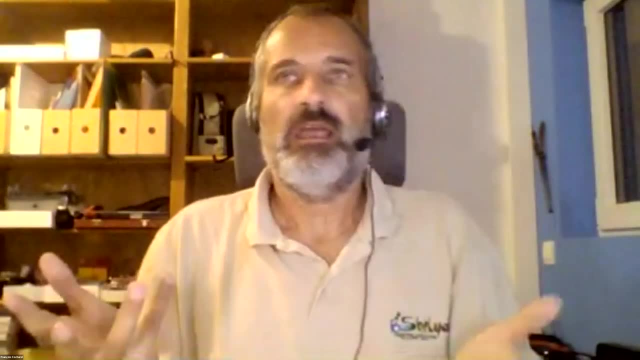 or increasing the focal length with a Barlow lens. Okay, In every case, you will add some glass. That's right, And it really depends on how you will use it. So it's always it's a question of trade-off. 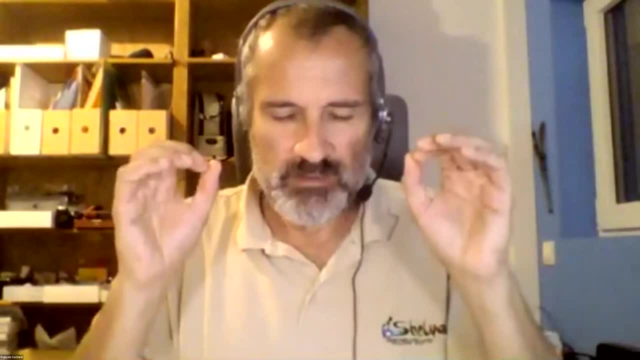 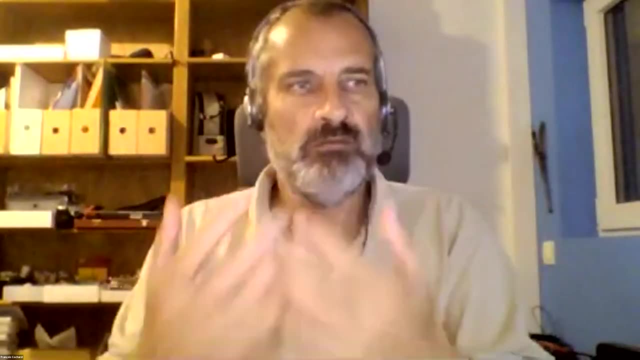 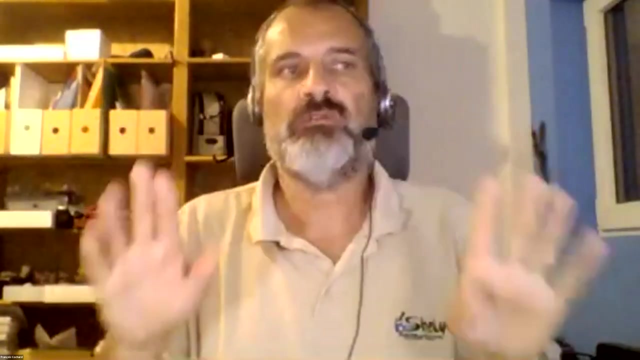 Well for sure for me, if you are starting spectroscopy, don't take care of everything. Just make your first spectrum, and it will be time afterwards to look at these details. These are not details. This is very important to have an efficient instrument. 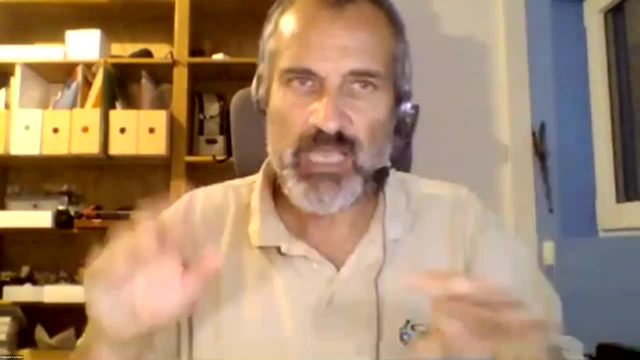 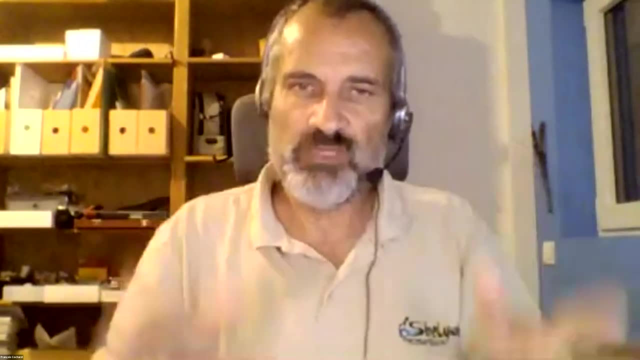 But at the beginning, if you don't have the right F-ratio, this is not a problem. Your observation will work. You will have a spectrum and you will be able to work with it. So it will not be optimal in signal-to-nose ratio. 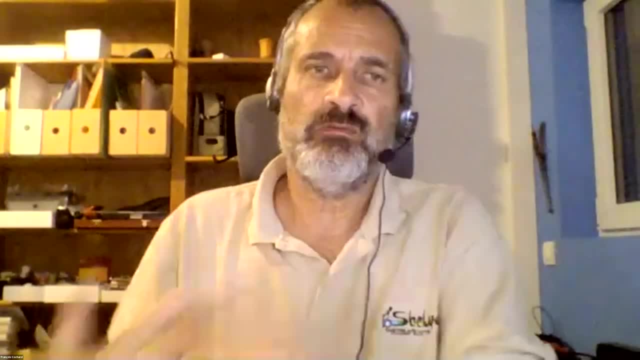 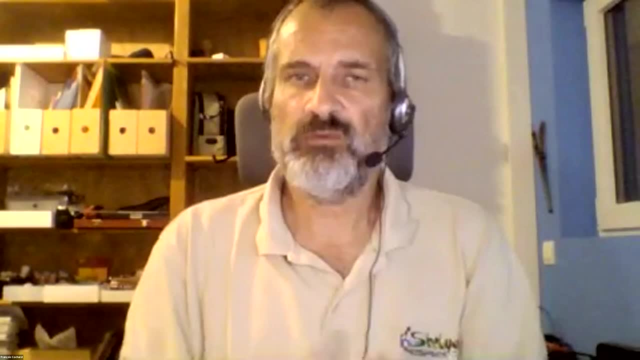 Maybe you will not take care of it, Maybe you will not take the benefits of your telescope or your spectroscope, But anyway, on a bright target you will always have a spectrum. So this is very important for beginners. Okay, So don't spend too much time to start in spectroscopy. 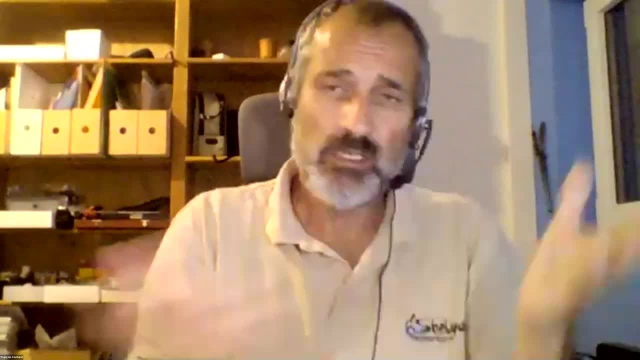 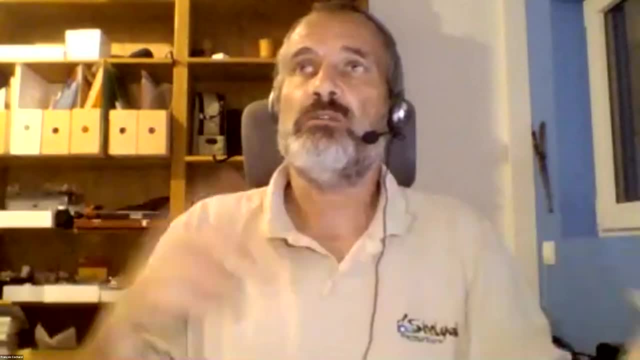 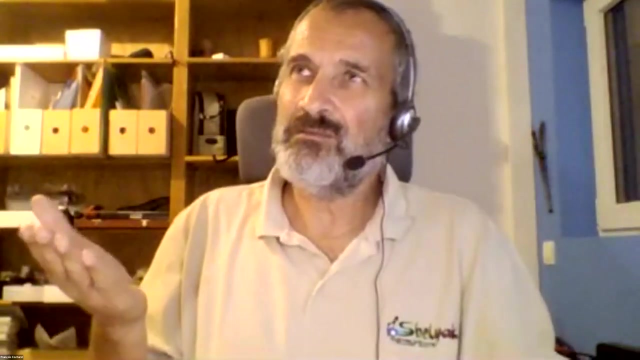 Observe with what you have Now. if you want to change your F-ratio and your focal length with a Barlow lens or a focal reducer, this is a trade-off, So we'll get there. We'll get some advantage. What I will win and what I will lose by adding this device. 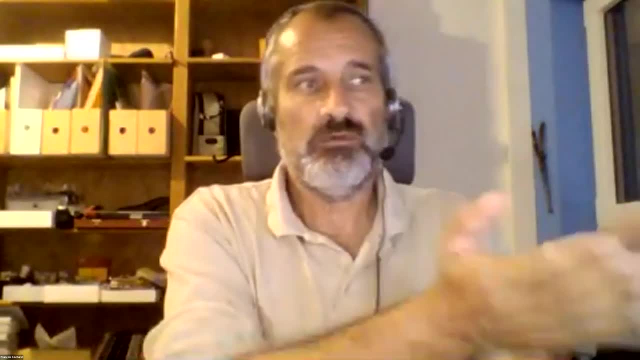 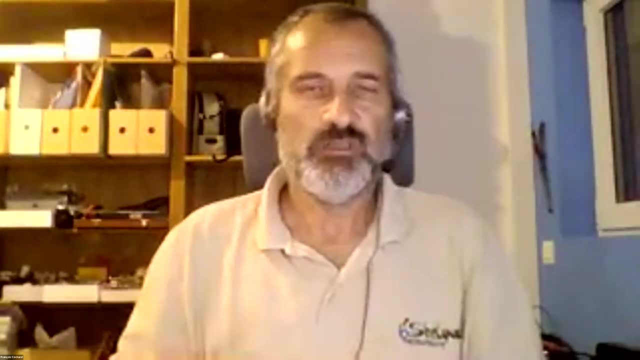 So if you have, for instance, an F10 telescope, a Schmidt-Kass-Groen telescope, usually at F10, and you have a spectroscope which is F5, F6, you better have to put a focal reducer, because the difference is too big. 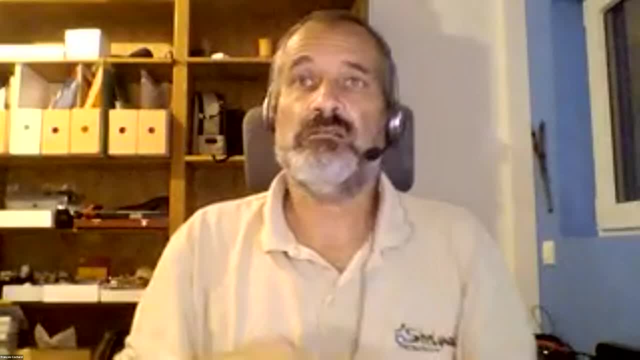 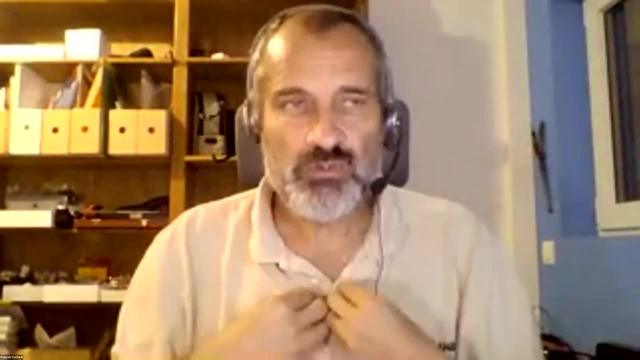 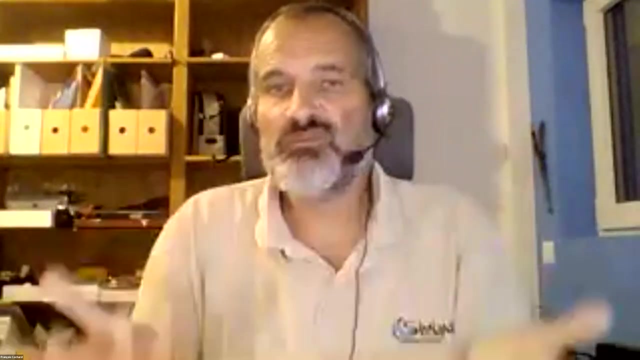 Now, if you have a telescope which is at F8 and you have a spectroscope which is at, I would say, F8.5, personally I think- don't put anything because the gain, the performance increasing, will be so small that you will lose it by adding some glass in the path. 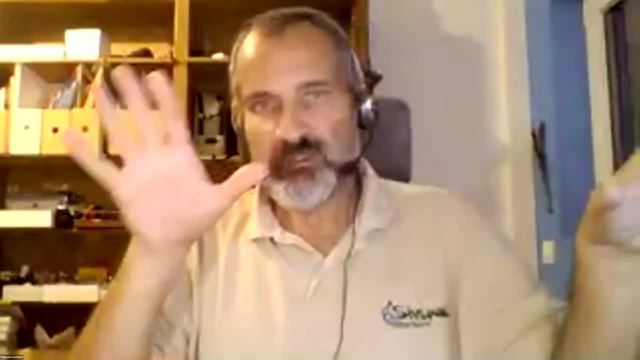 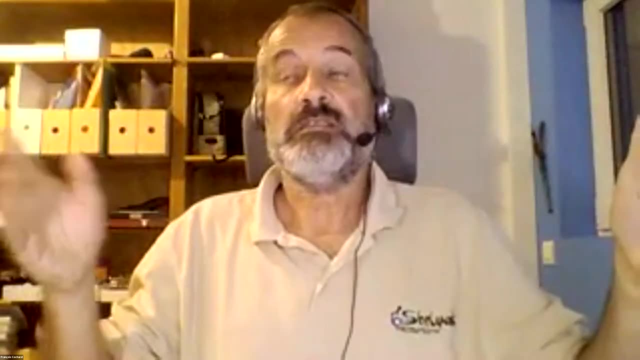 And, by the way, think that if you have a Richer-Christian telescope- purely mirror- and a UV-X telescope, for instance, purely mirror, so you have a fully achromatic system, in this case it's really a pity to put some glass in the middle, because you will introduce, you know, 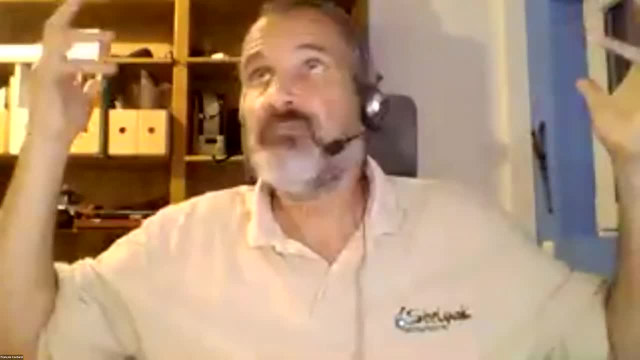 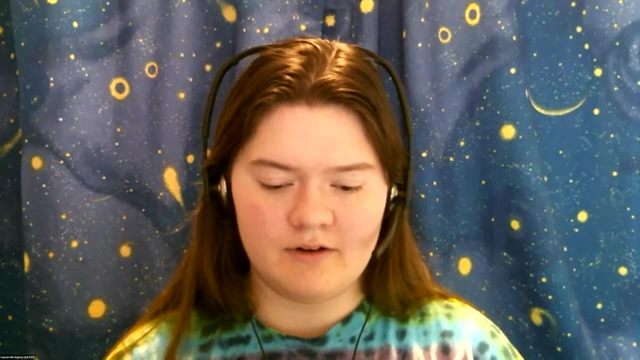 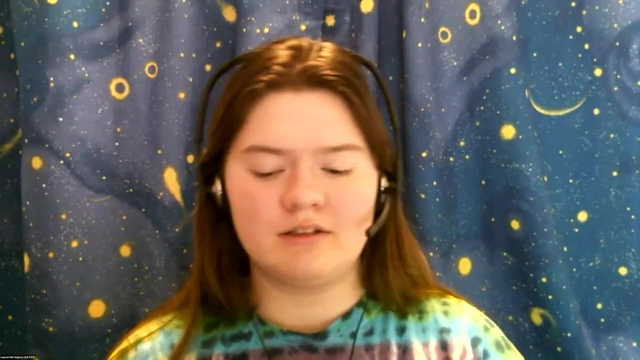 introduce high achromatism. Well, high Depends what you are looking at. Yeah, Okay, thank you. So, speaking of achromatism, we had a question from Bernhard Schultz, who has asked: how do you deal with atmospheric refraction? 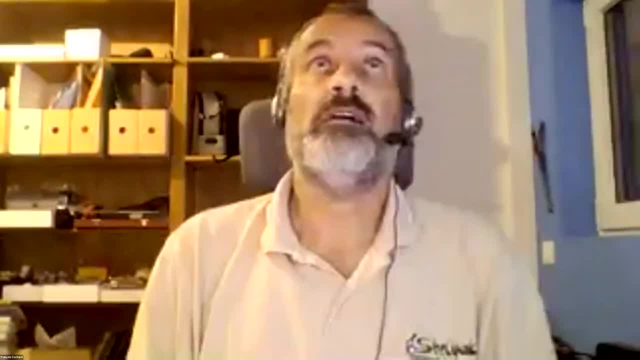 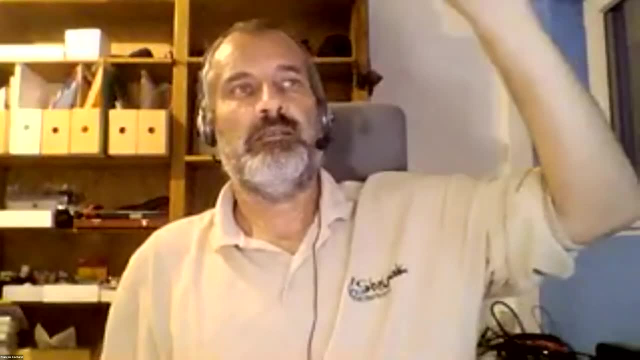 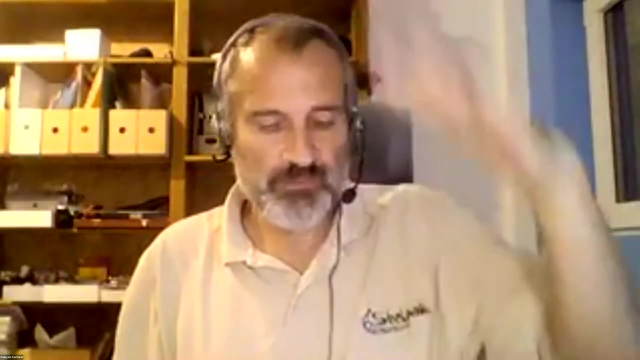 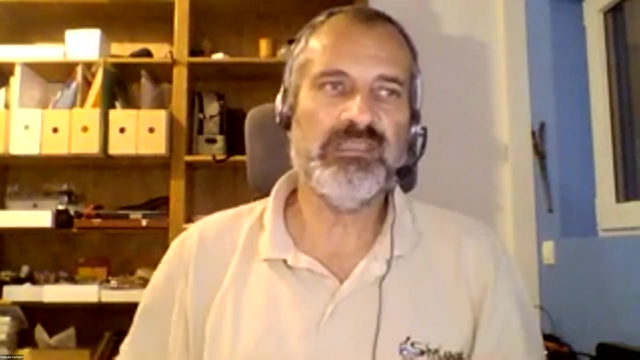 That's also a very good question. So the atmospheric refraction means that the star is not a pure point, but it's a small spectrum, vertical spectrum, because of the refraction of the atmosphere. And well, I would say that the first way to deal with that 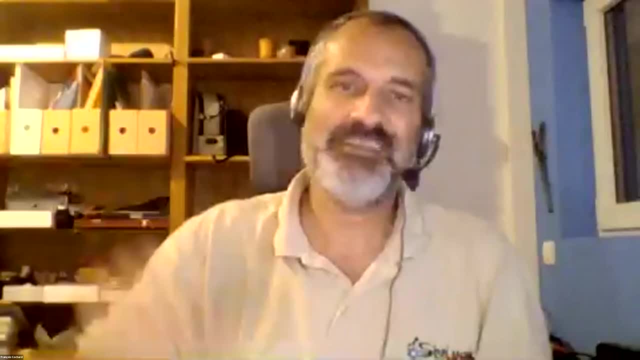 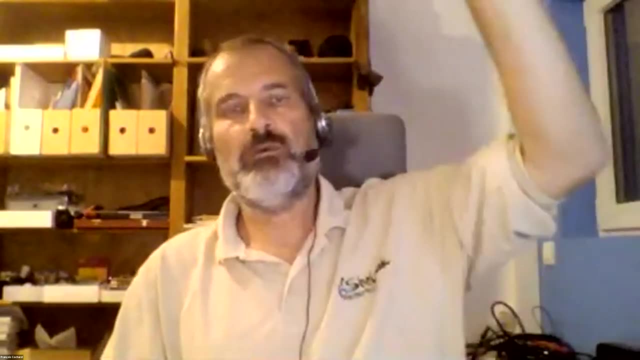 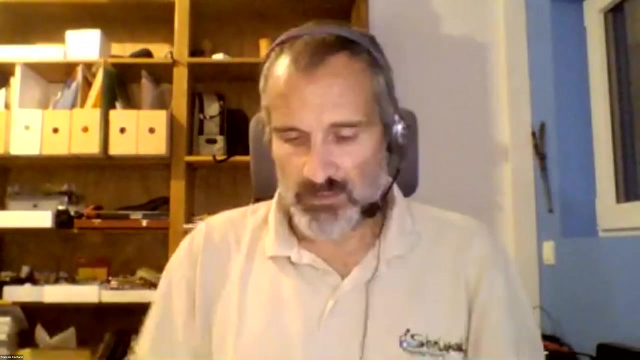 is to not observe too low at the horizon And, of course, it's better to observe above 30 degrees to make sure that the atmospheric refraction is almost negligible. Now, of course, if you have an event, if you have a nova that explodes tomorrow, 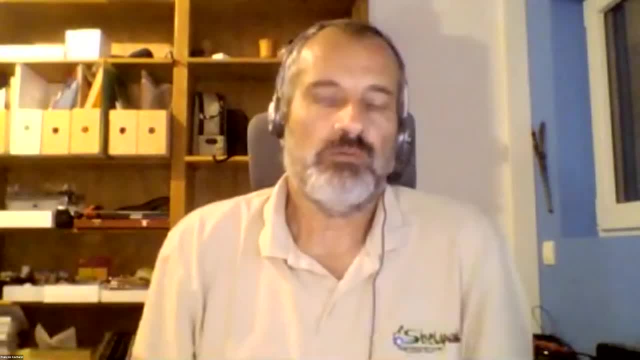 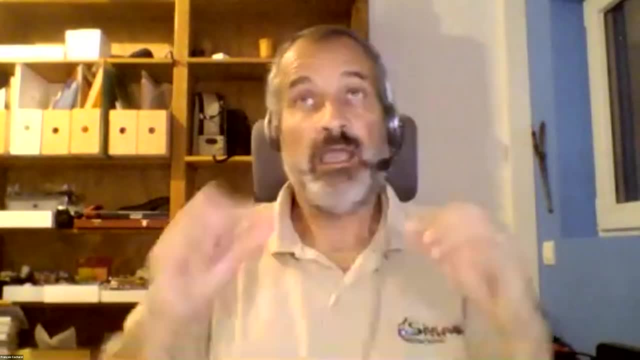 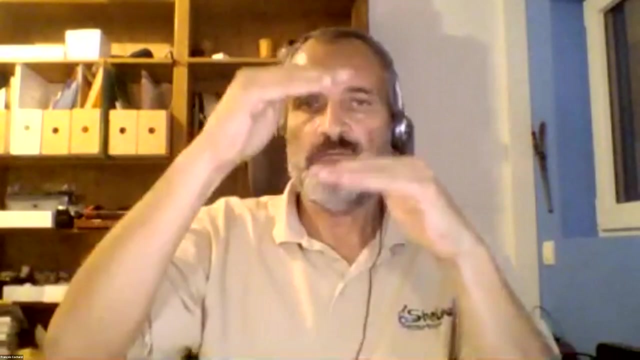 it may be at the horizon and maybe you don't have the choice and you cannot wait. and well, it happens, of course. So in this case. so either you increase the slit width and you lose some resolution, but to make sure that you will catch all the light, 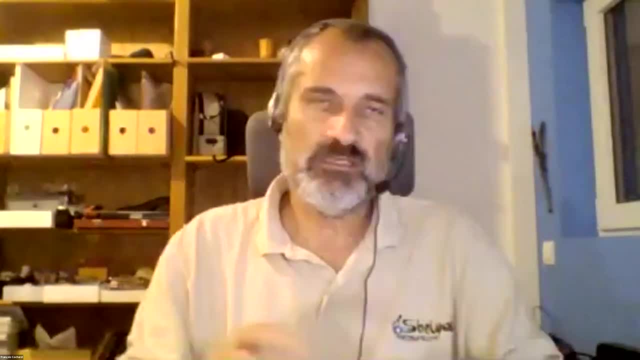 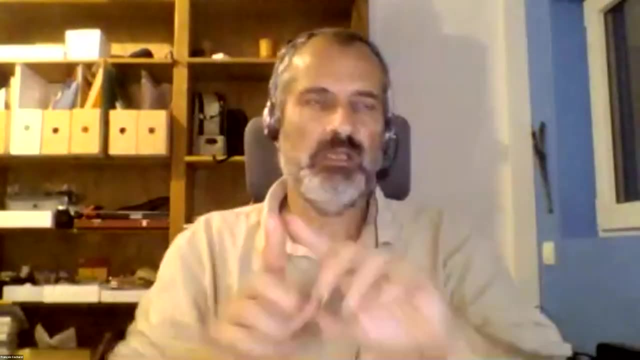 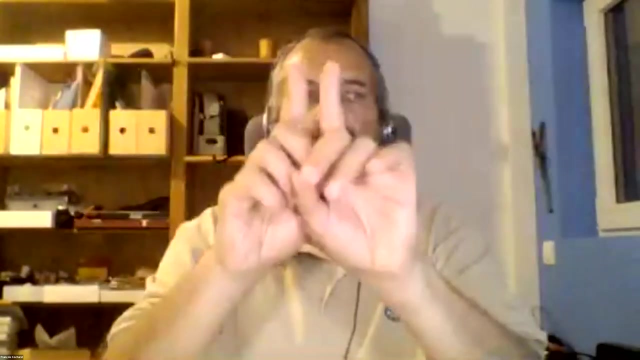 or there is another solution, which is to rotate the whole spectrum, the spectroscope, around the telescope versus the telescope, to put the slit vertical. okay, and vertical compared to the Earth And in this case, the small spectrum that makes the star. 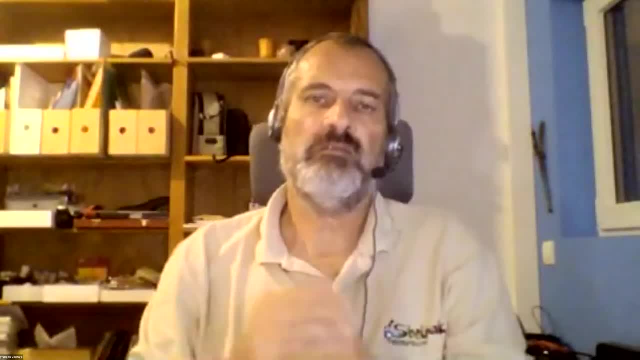 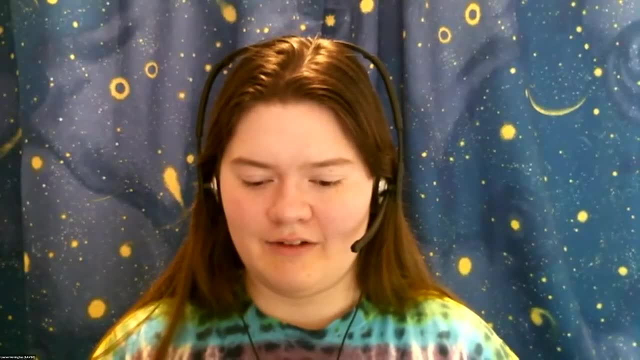 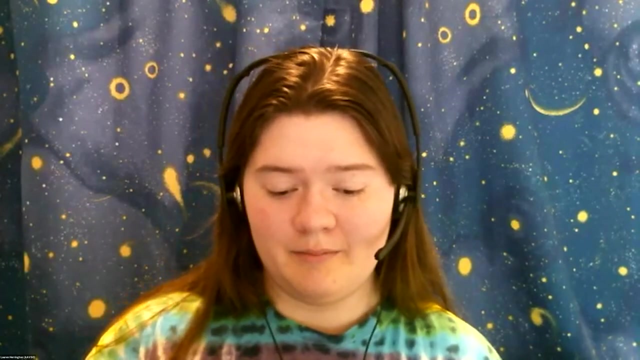 will be included into the slit vertically. I don't know if I'm clear, but this is really the idea. That is clear. Yeah, thanks, good advice. Okay, we have another question here related to the slit. Michael Nuss had asked so specifically for a fairly low resolution slit spectrograph. 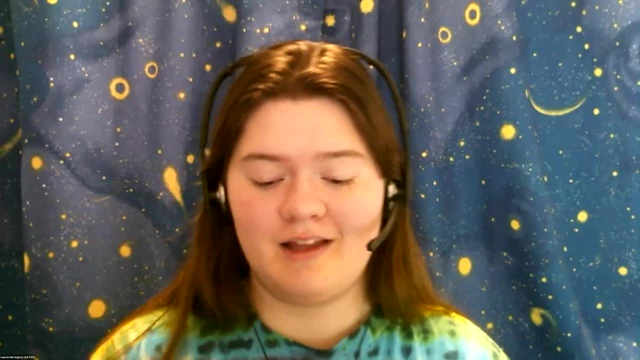 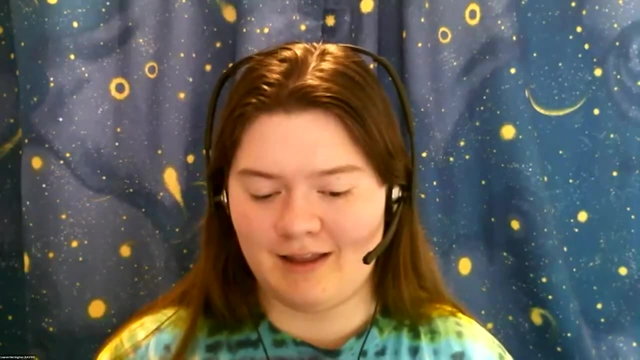 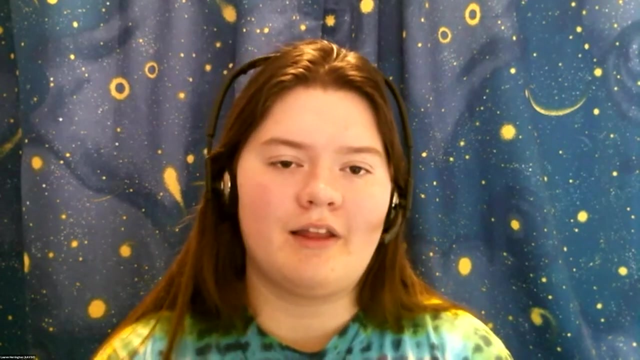 like an ALPI or LISA, if you want to shoot something non-stellar, like a comet, with a long focal length scope. he's giving an example of 2,100 millimeter focal length. what should you do about the slit size? setting the slit size? 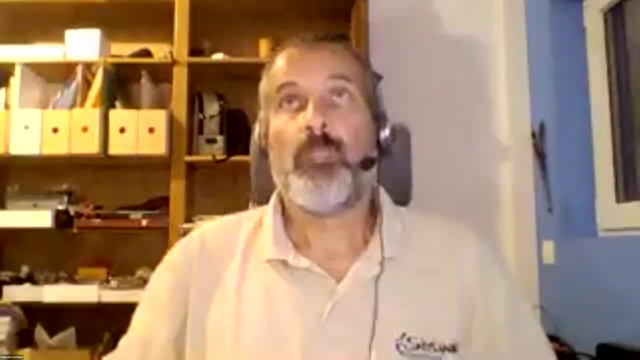 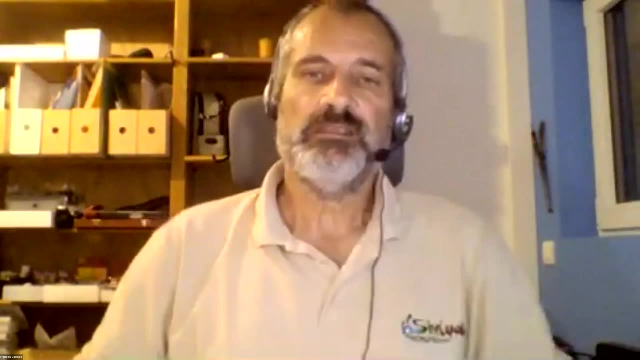 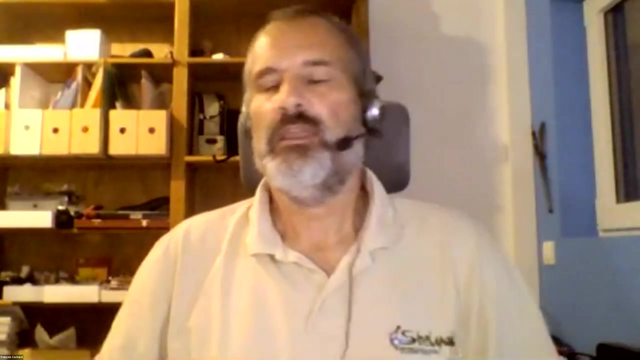 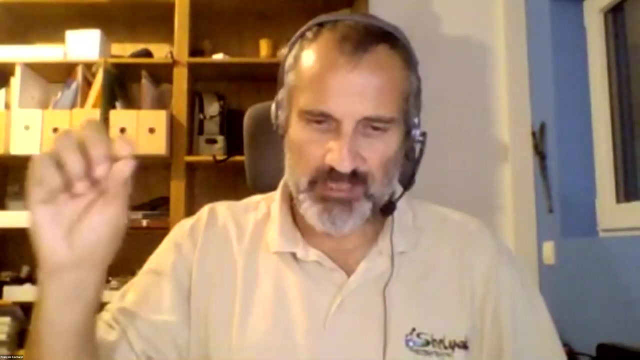 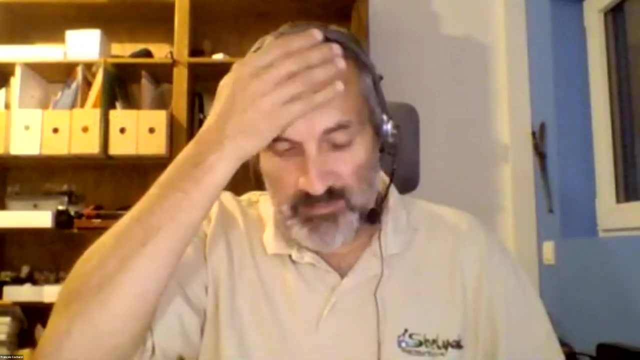 In fact, in this case, for me for sure, this is the standard slit, which is 23 or 25 microns, for a simple reason: With these focal lengths I know that the size of the star image it is typically an RC8 or 8-inch Schmidt-Casman telescope. 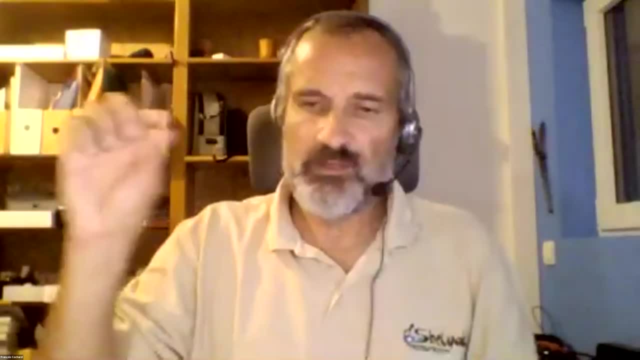 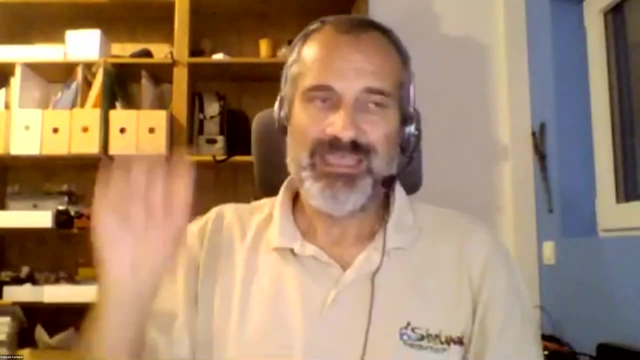 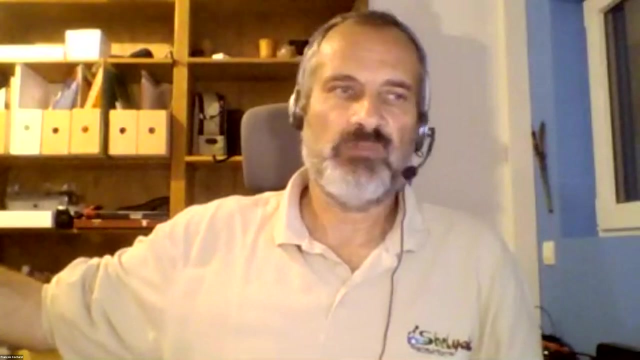 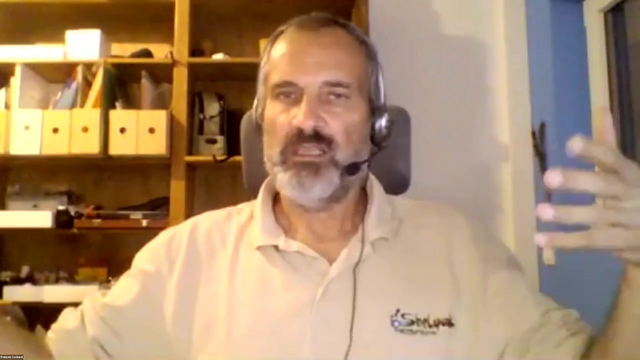 For these focal lengths you will have roughly 20, 25 microns FWH, so width of the star image in the focal plane, And this is also the optimal slit size for the ALPI or the LISA resolution. So for such a small telescope we are very lucky because this is the good value. 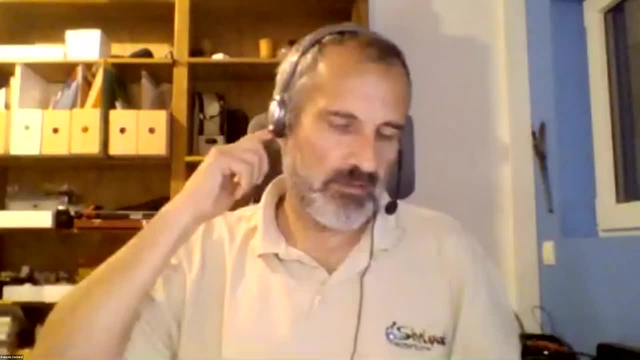 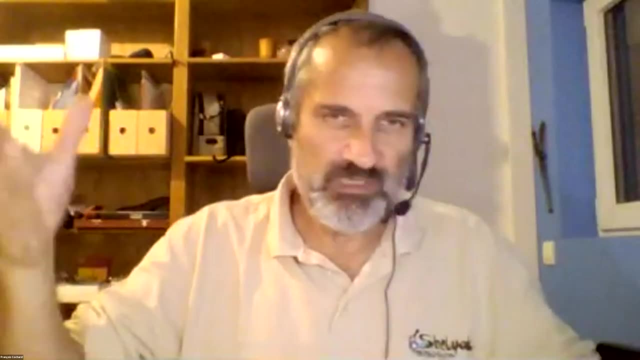 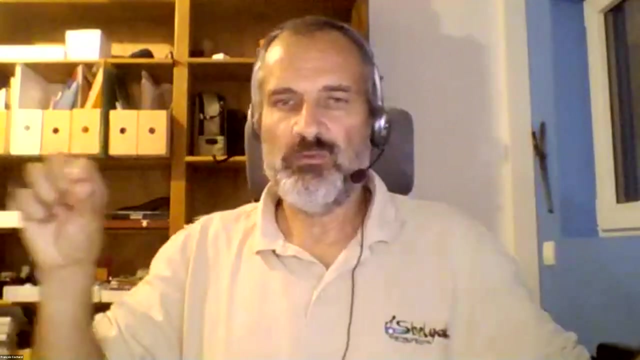 for both the telescope and the spectroscope. The problem appears if you take a bigger telescope- If you have a 400 millimeter telescope, for instance- then the star image will be bigger, So depending on what you are looking for. So if you want to have the resolution, you keep the nominal slit of 25 microns. 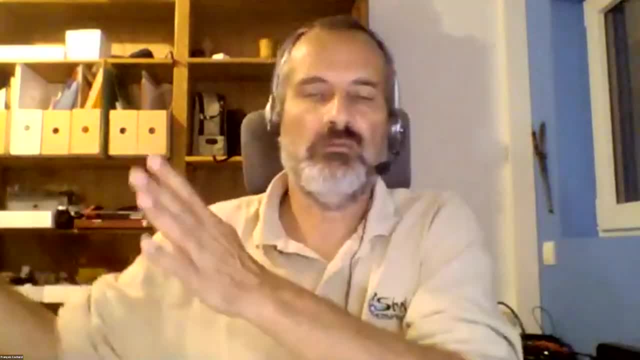 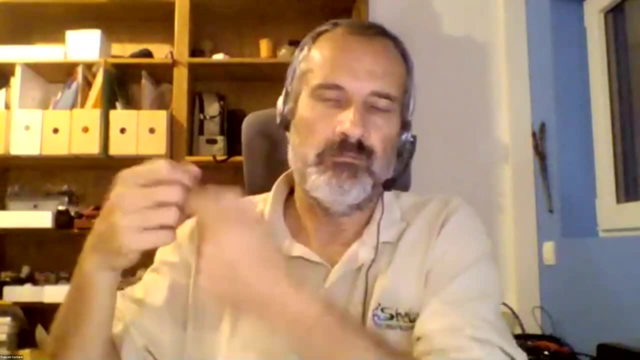 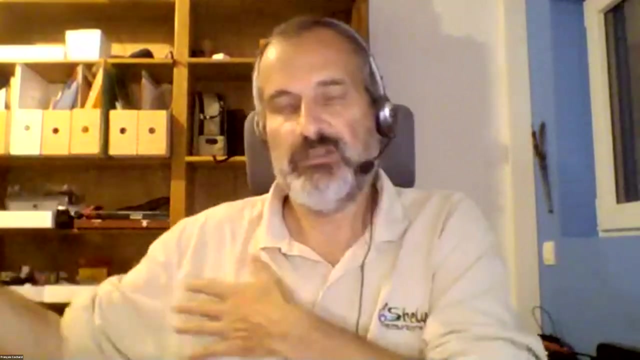 but you know that you will lose some light. You will have the full resolution of the instrument, but you will lose some light. If you want now to get some faint target and to go for very faint object, you may open the slit. And if you may open the slit, if you open the slit, 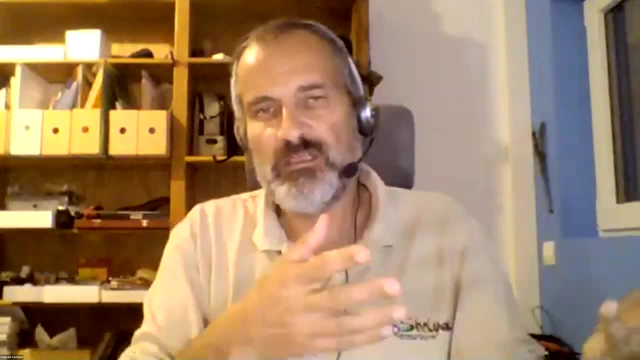 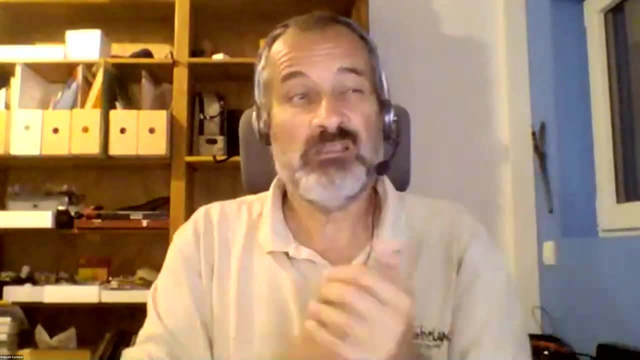 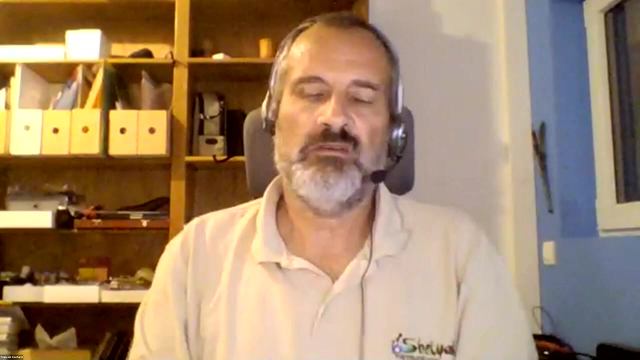 you will lose some resolution, But you can. for a bigger telescope, you can really choose between the resolution or the brightness. But at 200 millimeters diameter, which is two meters focal length, this is almost the same. And then if you increase, in fact if you increase the slit, 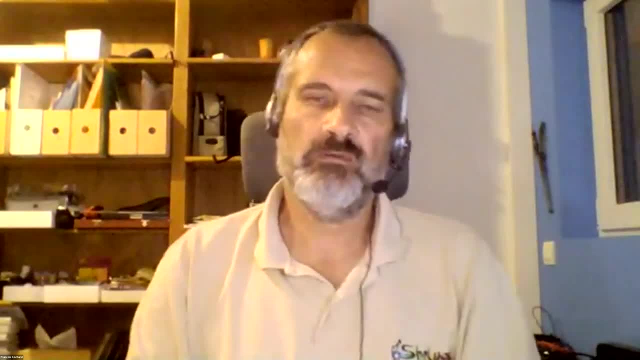 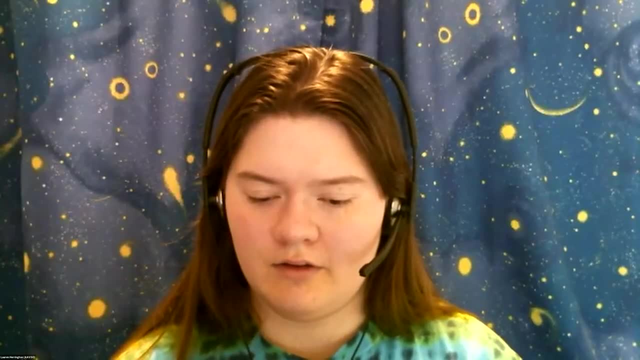 you will not increase the detection of the system and you will lose some resolution. So it's a pity. Okay, thank you. So looks like we've got four more questions. I think we're going to need to speed up a little bit to get through all of them. 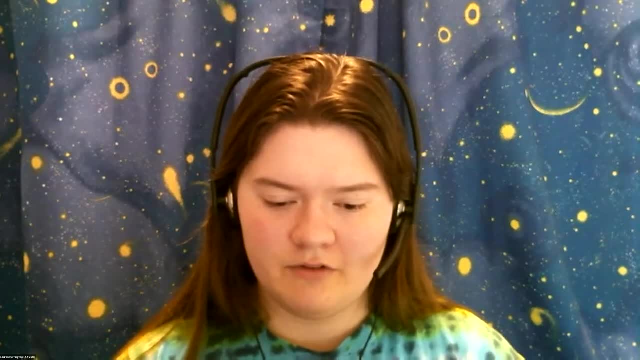 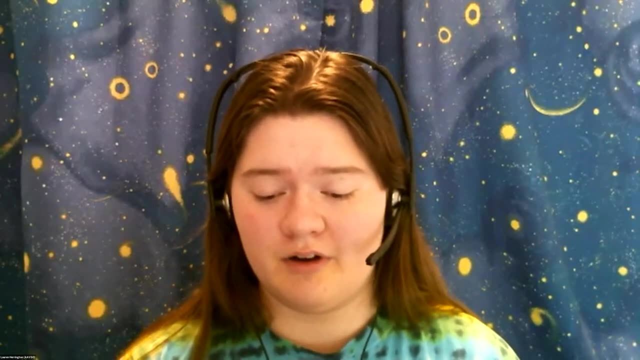 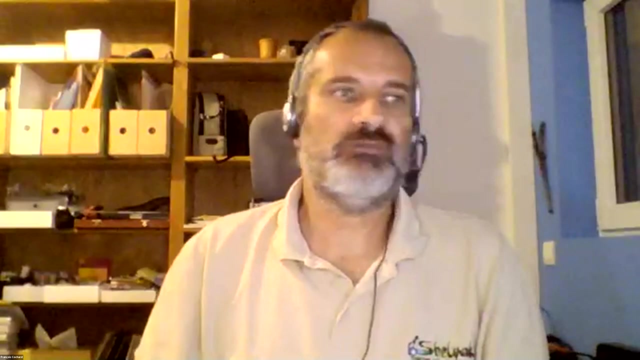 before we have to close things down. First of all, Michael Nuss has asked which objects or phenomena would be best as targets to observe at a medium resolution. So somewhere around R1000 to 5000.. Your life will not be enough. 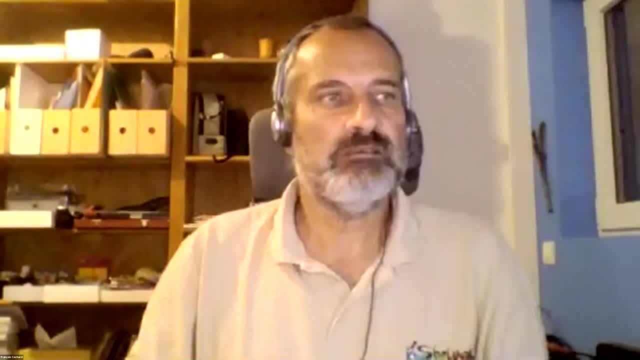 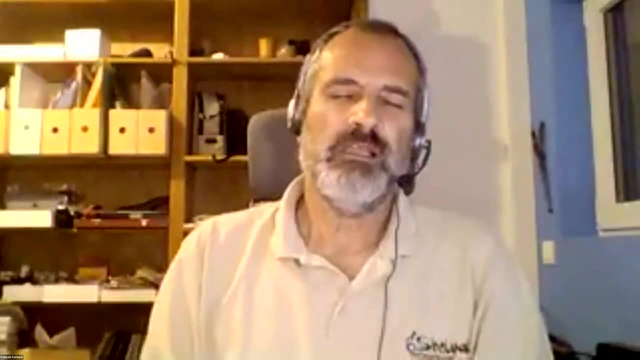 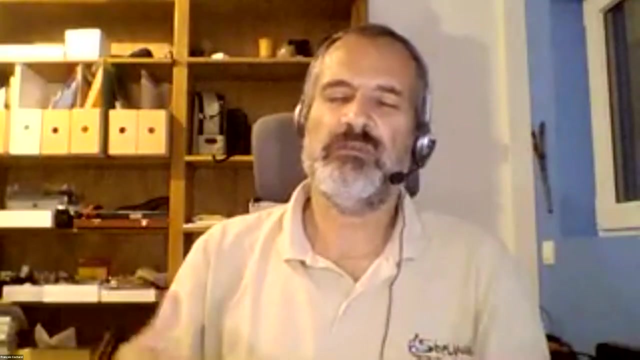 And so you have many, many, many things. Well, it's difficult for me to reply to this question because you have thousands and thousands of objects that we can observe with our instruments And, of course, if we go lower in resolution. 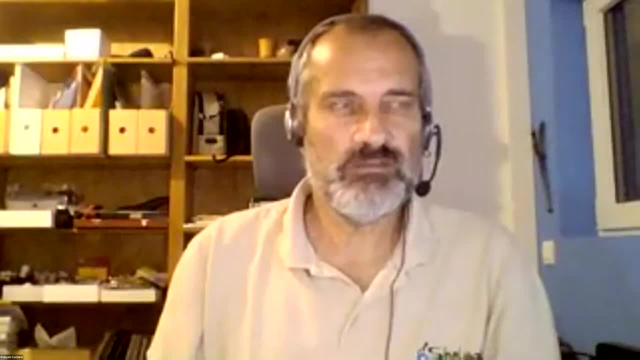 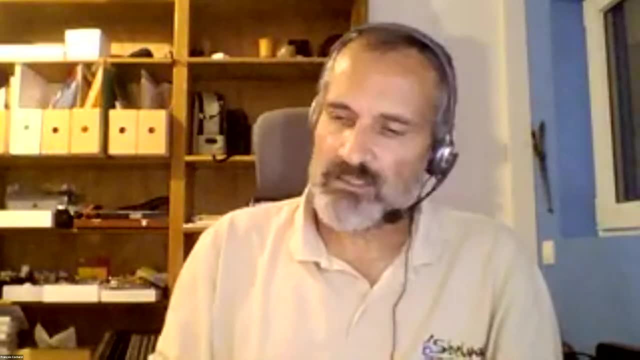 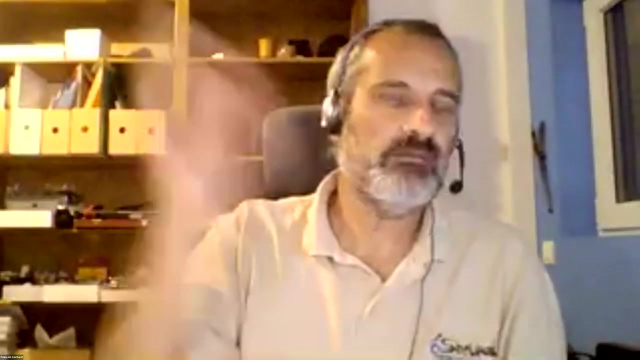 so the resolution of 1000, resolution power of 1000 is something really a medium resolution. You can access so many objects, So you can object a lot of stars, a lot of nebulae, a lot of planetary nebulae. 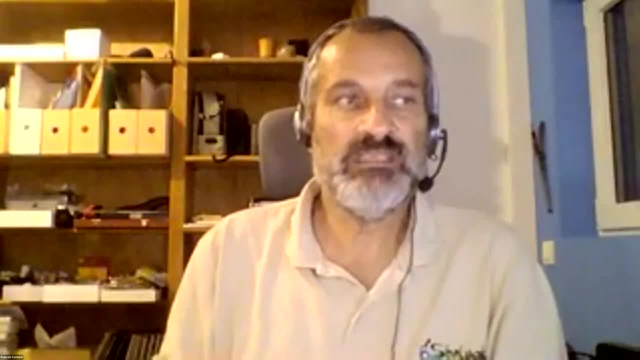 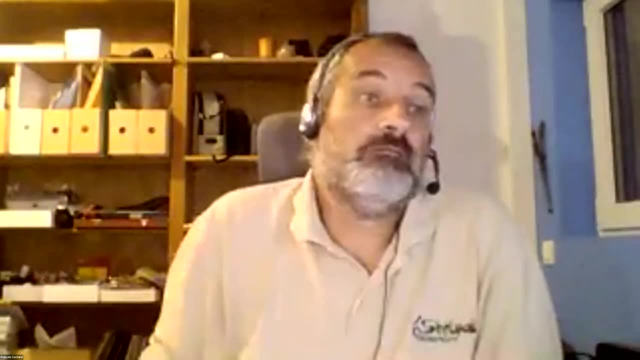 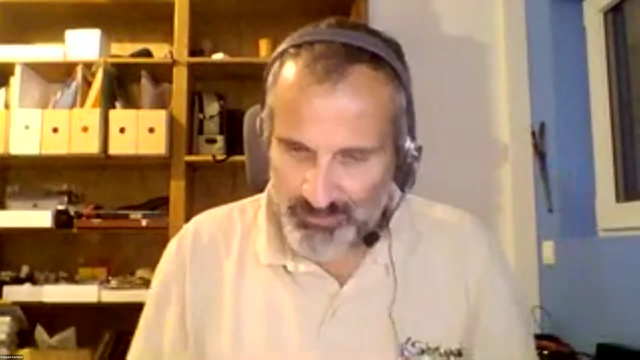 a lot of well, really, there is no limit. There is absolutely no limit. So well, I cannot. I don't know what I can answer to this question. So you will see that when you do spectroscopy, even in spectroscopy, 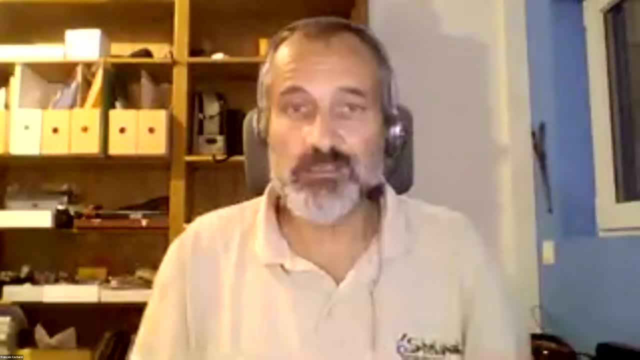 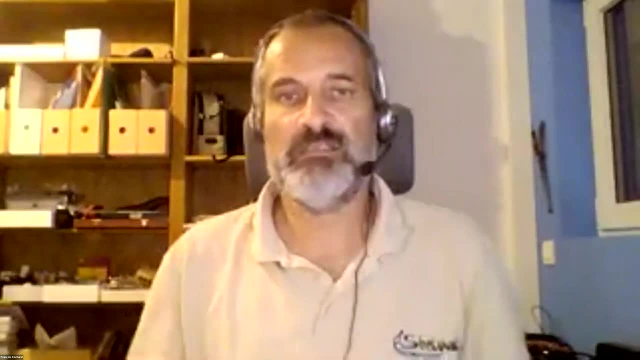 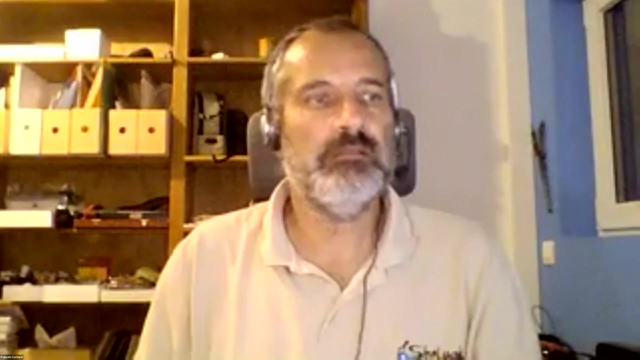 well, spectroscopy is somewhere, it is a niche in the astronomy, but you have to be specialized. specialized in one area, because you cannot observe everything in spectroscopy. I've shown you the, the picture of a star field in the in the skies. 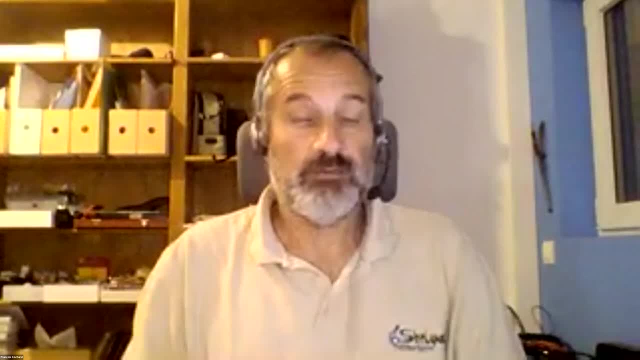 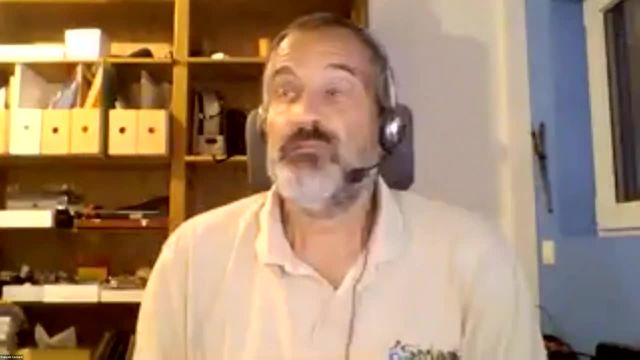 There are so many objects, so there is no limit And and you will, you will know, you will see if you want to observe Personally. you know, I'm a mechanician, I'm a mechanician and I like the Doppler effect. 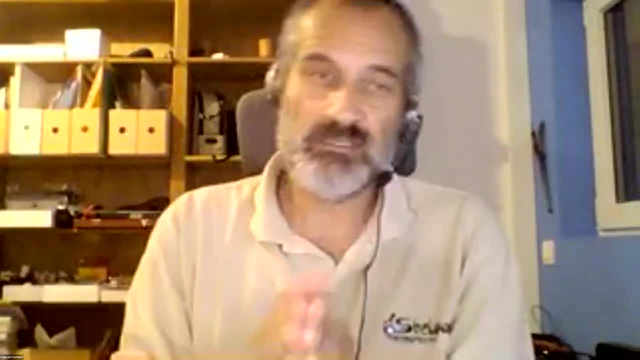 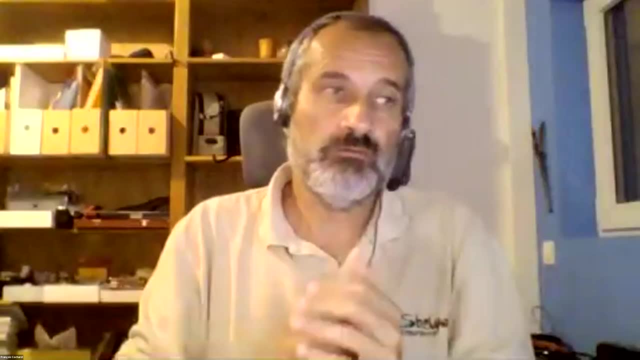 because I understand it perfectly, because this is basic, This is not quantum mechanics and so on, And and to do that, I prefer to to work with a high resolution, but it depends on what you are looking for, what is interesting. 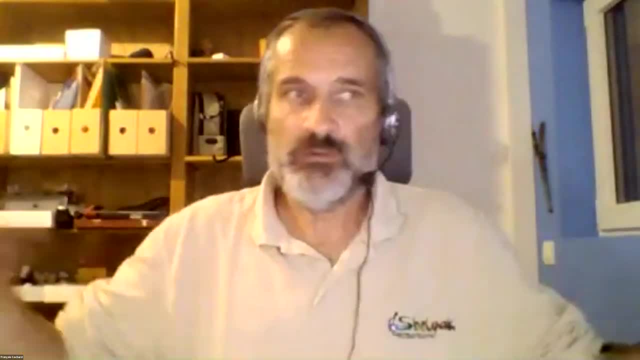 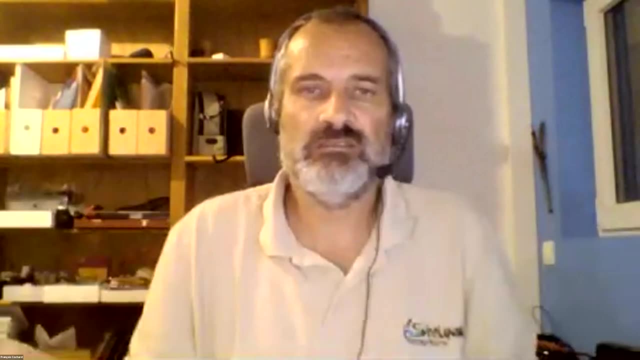 So do you want to, to observe for years and years the same type of object, or do you want to just jump off any event that arise in the sky? There are so many things to define to do that There is really no limit. 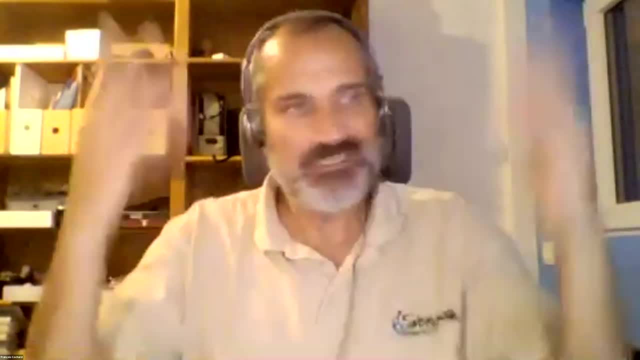 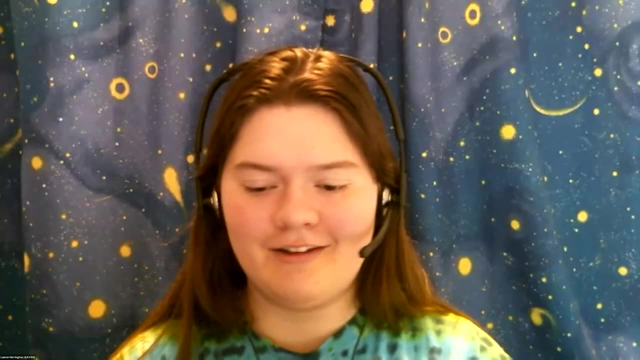 I'm sorry, I'm not sure that this is a good answer, but this is a so open, so open question. I think it is a good answer. It's really. yeah, you can observe just about anything. The AAVSO actually has a list. 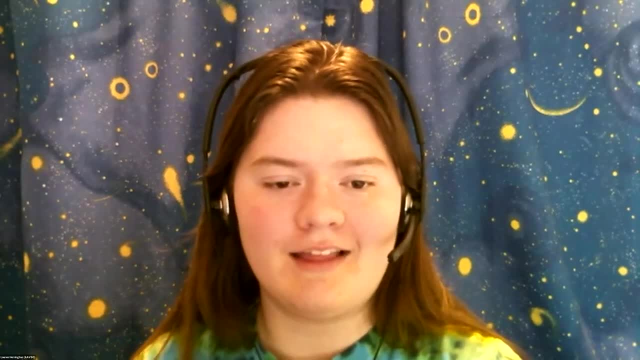 which I'm going to go ahead and paste into the chat. It's on the spectroscopy observing section page and it just has some suggested types of targets with suggested resolutions for observing them and making various kinds of measurements. So I'm going to put that in the chat. 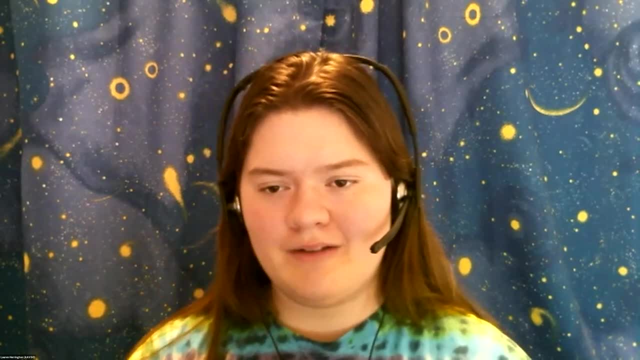 Well, you are answering the next question, which is from Patrick Cavanaugh, And Patrick asked when would be a good time to observe for a long period of time. Well, you know, it depends on what you are looking for. It depends on what you are looking for. 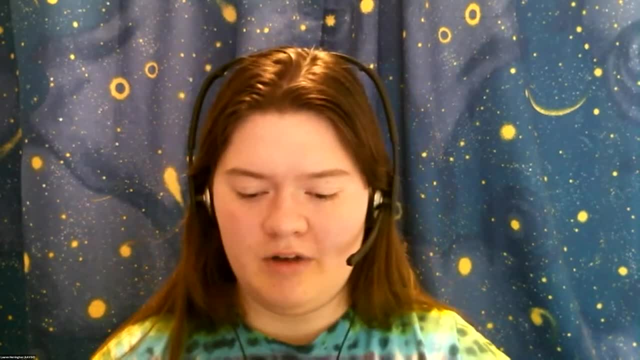 So you know, it depends on what you are looking for. It depends on what you are looking for. It depends on what you are looking for. So I think that's a good question And I think the next question, which is from Patrick Cavanaugh, and Patrick asked: 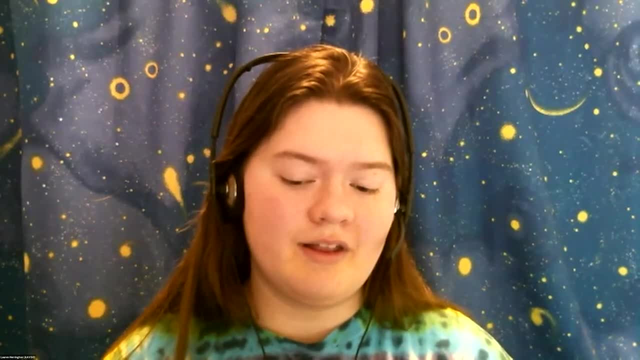 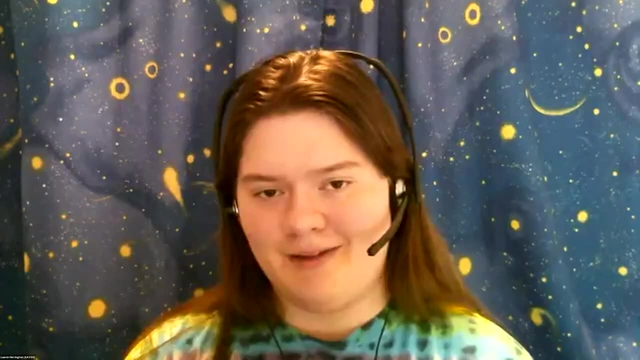 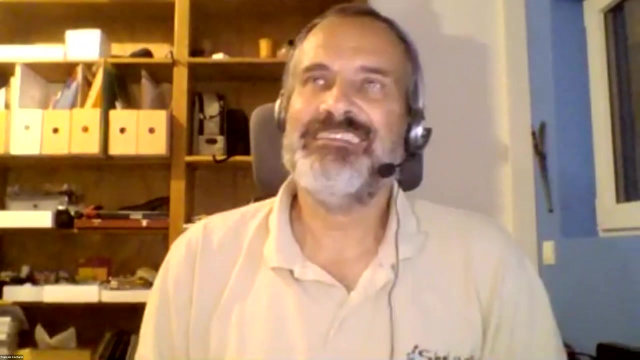 when would be a good time to migrate from low resolution spectroscopy using slitless diffraction gratings such as a star analyzer to slit spectroscopy with a fancy spectrograph? Wow, Again, this is a very open question. I know that. 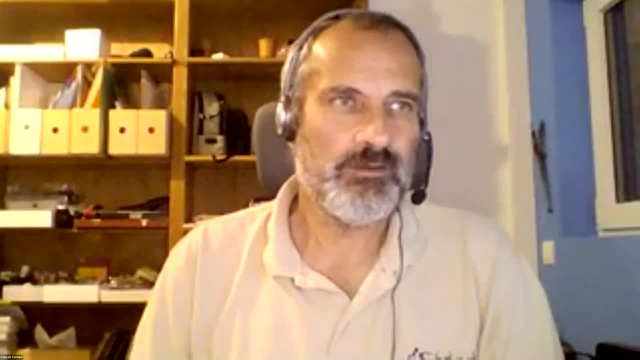 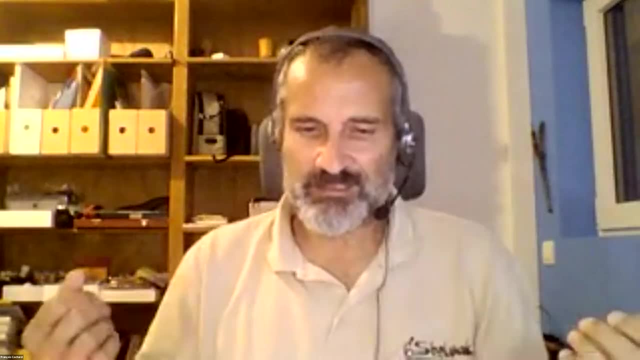 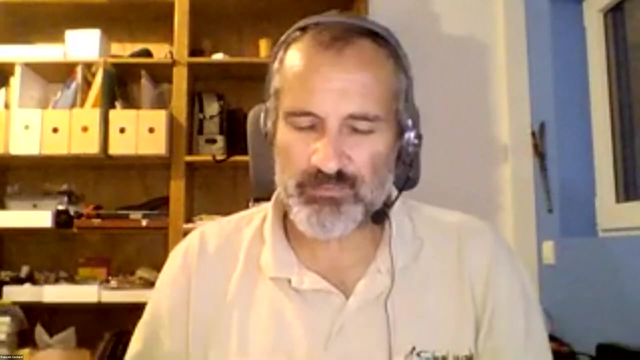 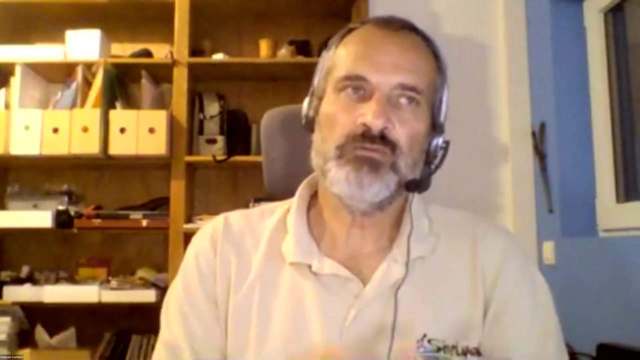 well, the star analyzer and and low resolution diffraction gratings is is a wonderful system to to to jump into spectroscopy. this is cheap. this is close to the setup that you usually usually use for imaging and photometry, so there is a lot of advantages. now the switching to slit spectroscopy means that you can. there are a 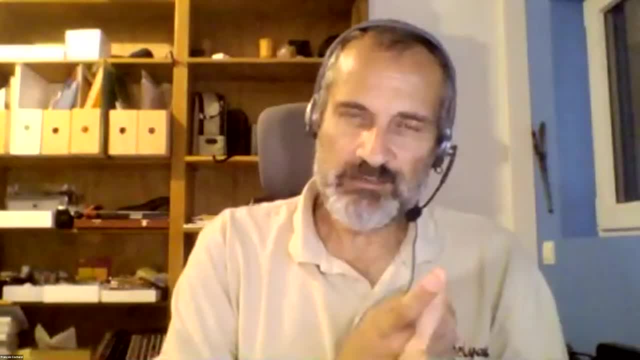 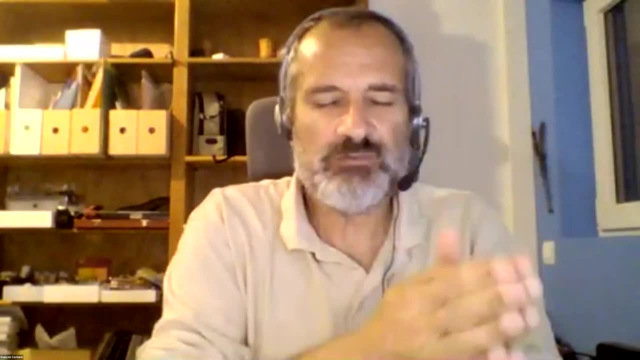 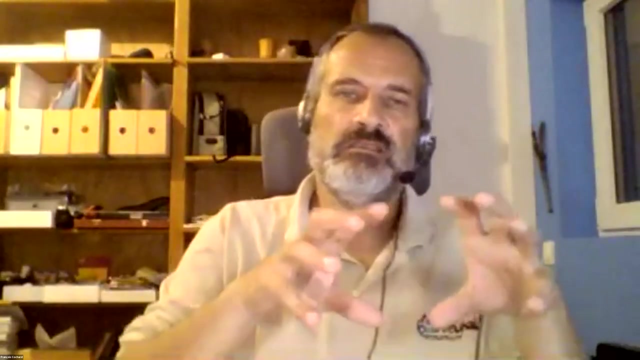 lot of advantages. so you can use some calibration light, because you will. the calibration light is an extended object and in fact with the slitless, with the slitless spectroscope, you cannot observe an extended object. you are limited to stars because the, the, the extended object, will make. 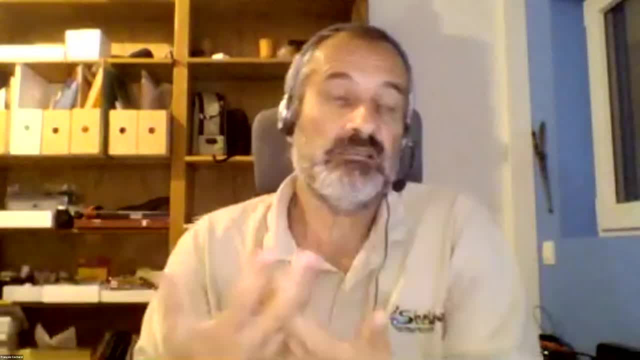 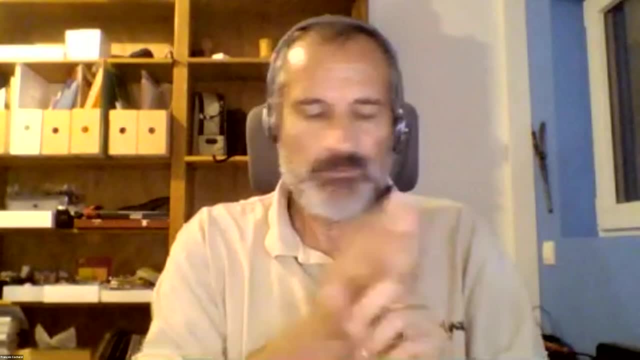 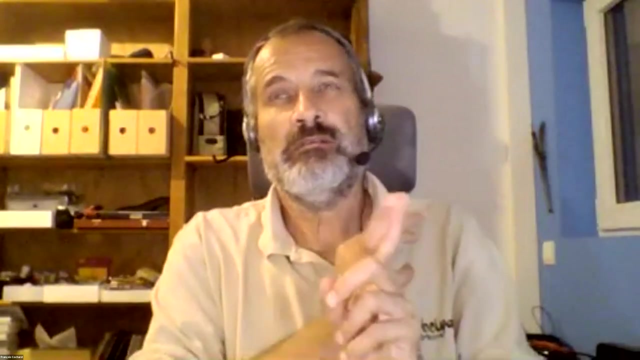 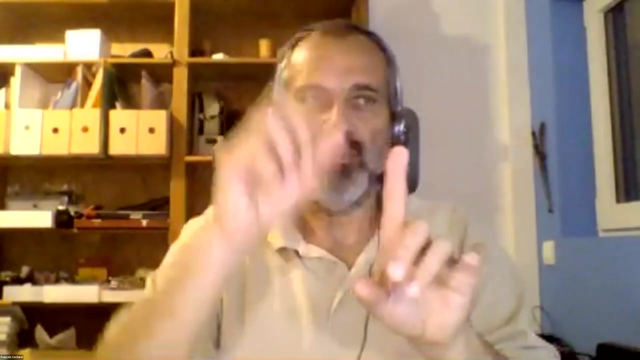 an extended spectrum and which is totally confused. and then you, you don't have, you, you cannot use the, the spectrum. so you can use calibration, you can use, you can observe extended object, you can correct from the sky pollution because, as i explained, at the same time as the star spectrum you will observe the, the sky background spectrum. so you, 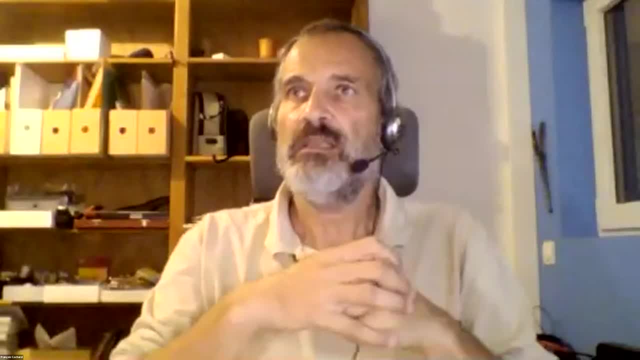 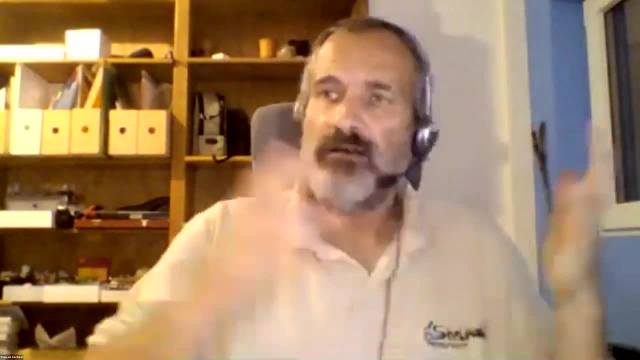 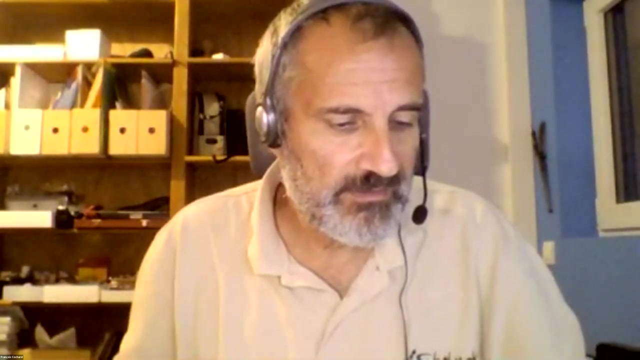 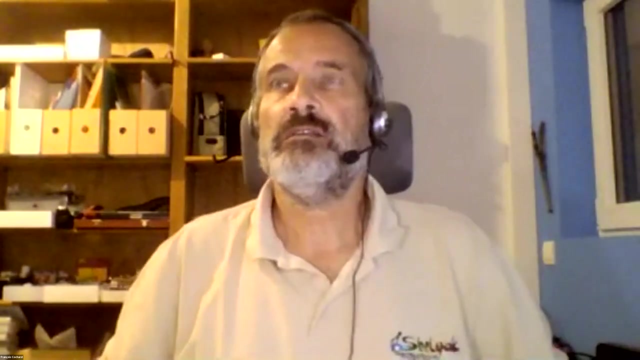 can correct it from the observation and there are a few other good reasons to switch to slit spectroscopy. but the, the, the, this, the, the standardizer or smaller devices like this uh have still have advantage. i know, for instance, robin little in in uk: uh, he's using uh, uh the star analyzer and he loves to observe nove with this. 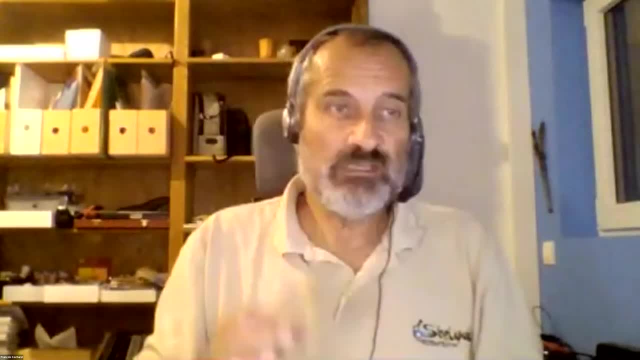 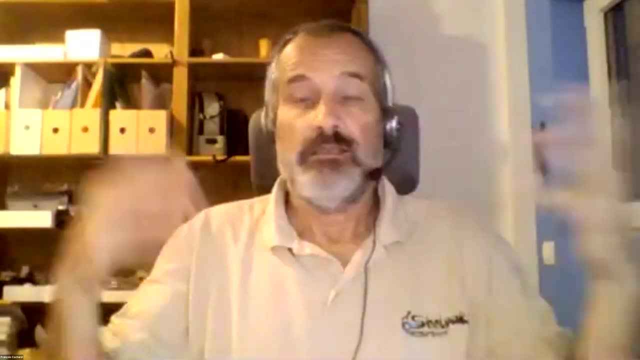 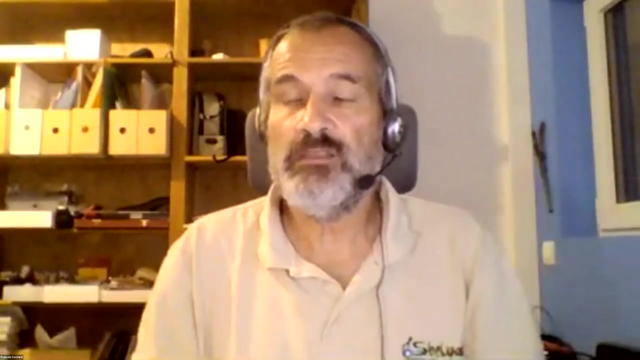 kind of system, because the the advantage is that it's very simple. you are not losing a lot of light, so you can observe very faint object with a star analyzer. okay, so it really, it really happens. now i can tell you that i would say that, uh, nine, 95% of the observations in spectroscopy 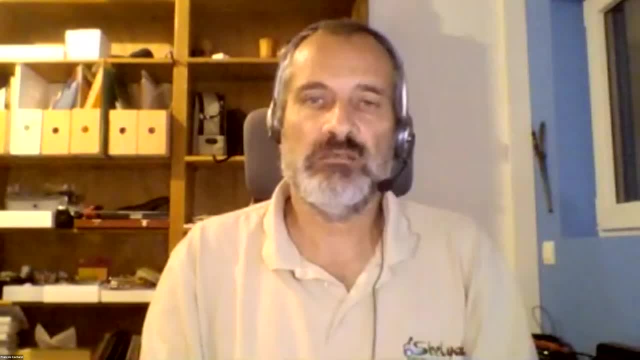 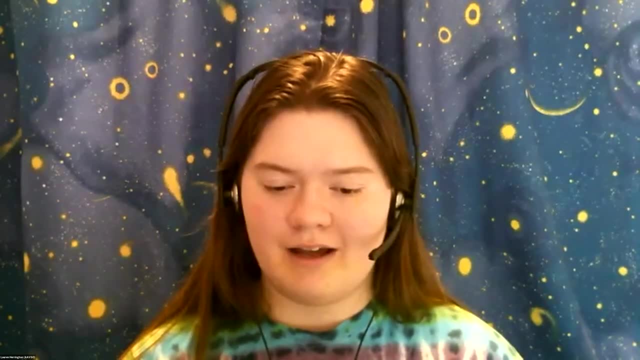 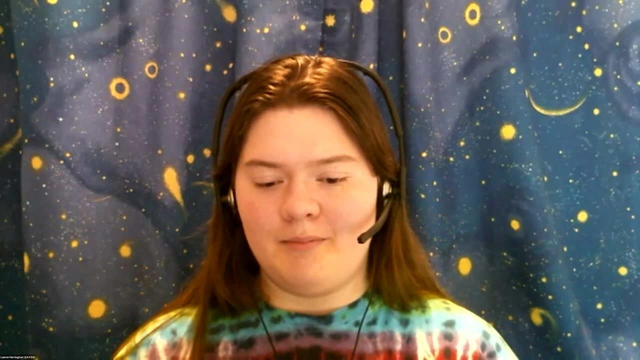 or, or even more, 98% are made in with the slit spectroscopes. okay, thank you, and this is our uh last question for now comes from patrick cavanaugh, again, who has asked um: in your experience, what is the background of most of the people in amateur? 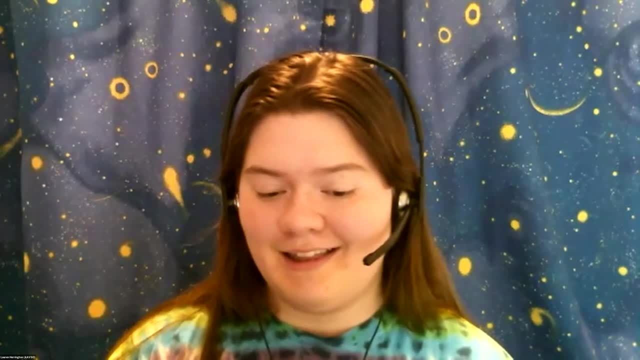 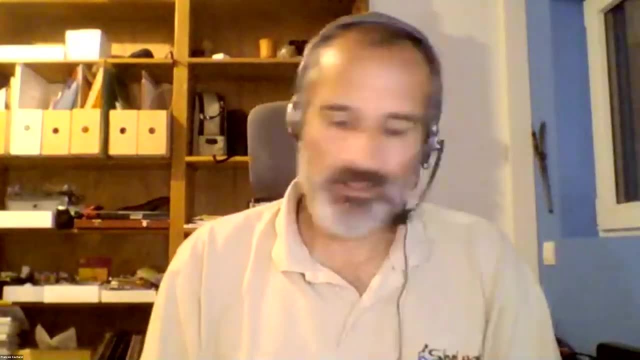 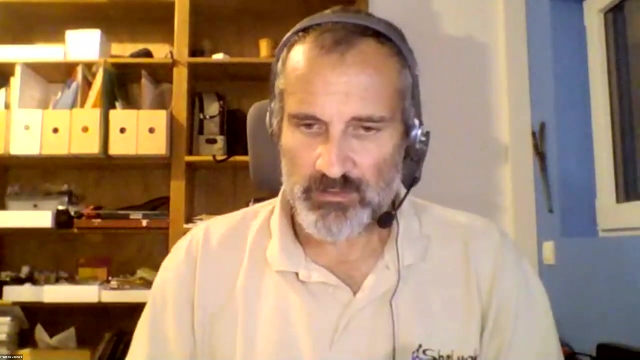 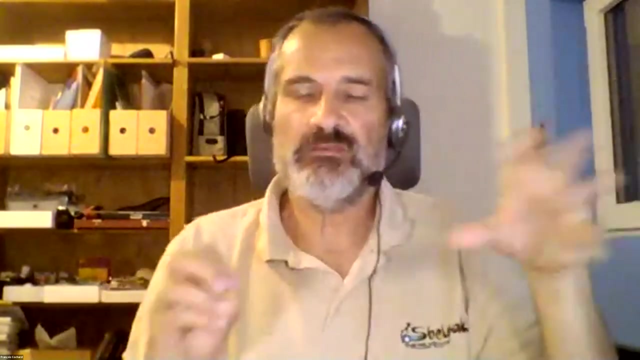 amateur spectroscopy. Engineers, scientists, teachers, liberal arts majors- what have you observed? Well, I know in my book I start with that When I see people doing spectroscopy, I like to say that in fact there are people coming from the science itself, so they want. 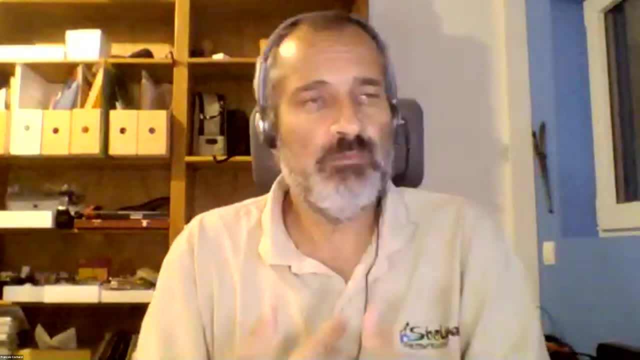 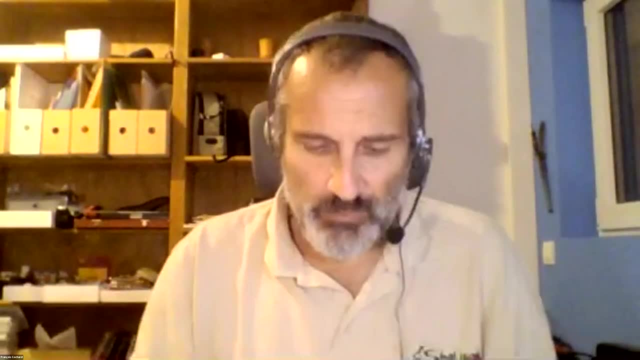 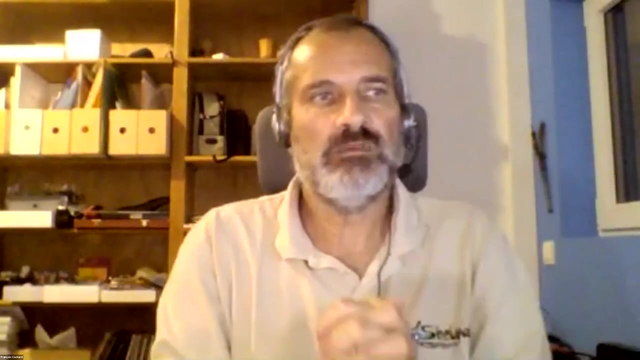 to understand. the read books about physics and astrophysics and they want to understand how the universe works. So these are part of people are coming from science and then they are most of them- they are scientists, they are engineers or things like that. Besides that, 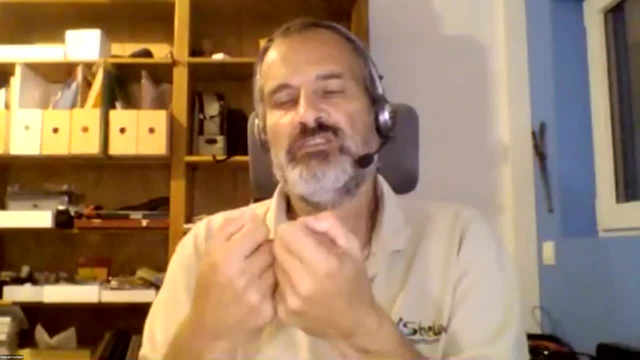 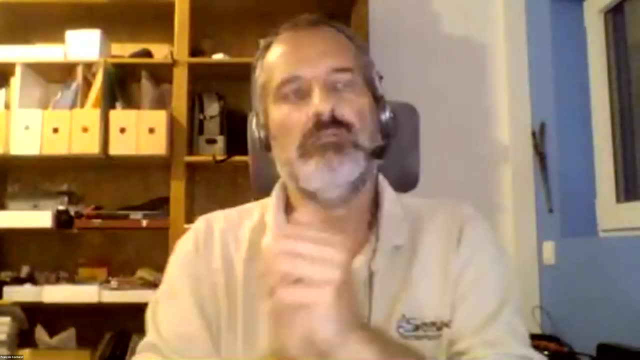 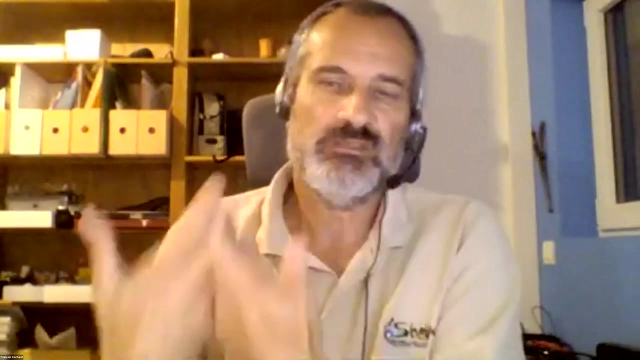 you have people who love to make their own instruments, to do it yourself, to polish the mirror, Or to do some computing, some software development, or to make their mount and so on, And then for that a spectroscope is just a wonderful instrument, because it's a fun. 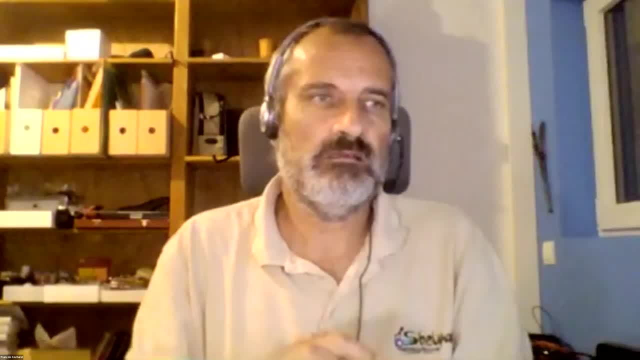 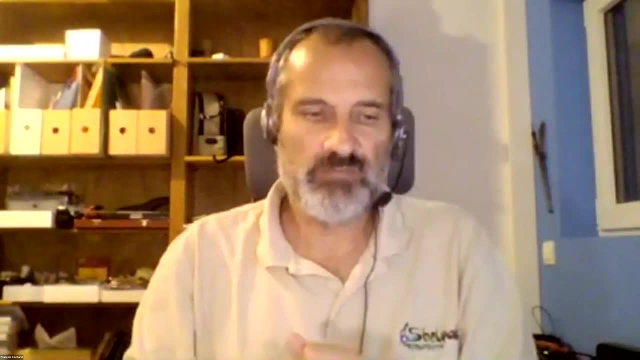 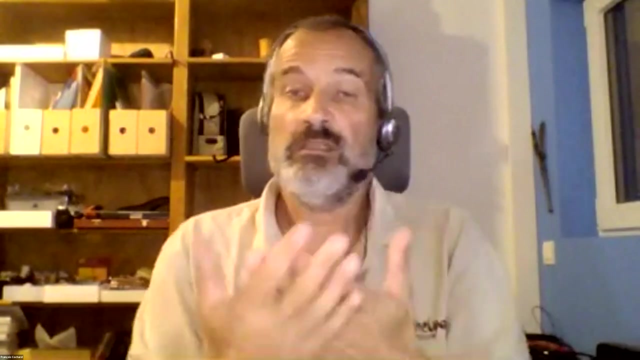 part of a piece of optics, and this is something very great, And so we have a part of people doing spectroscopy that comes from this area. And the third area is people coming from the observations They are already. they like to use their telescope on the sky and to make real observations. 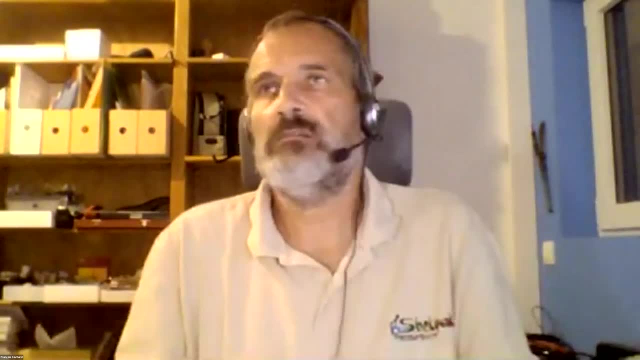 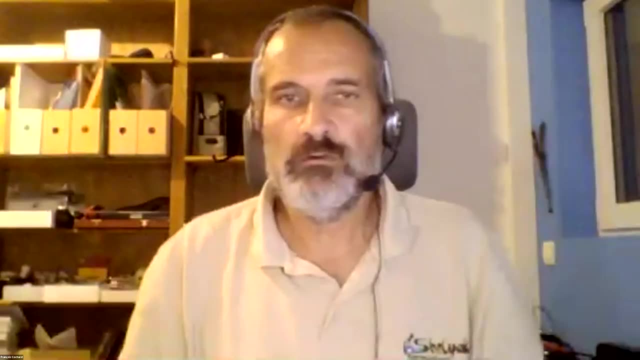 And I know a lot of people saying, well, okay, I've made great images, I've made wonderful images. now I'm tired to do always the same kind of source and I'd like to do something else. And then this spectroscopy is something wonderful. 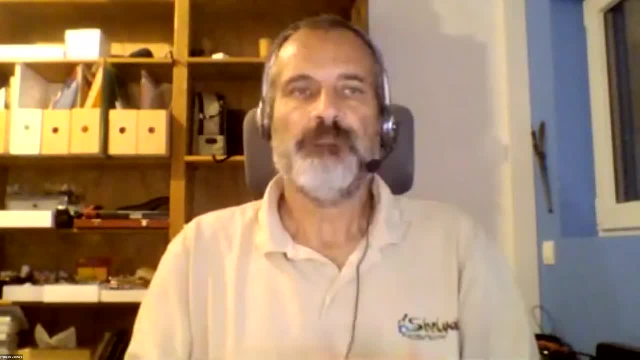 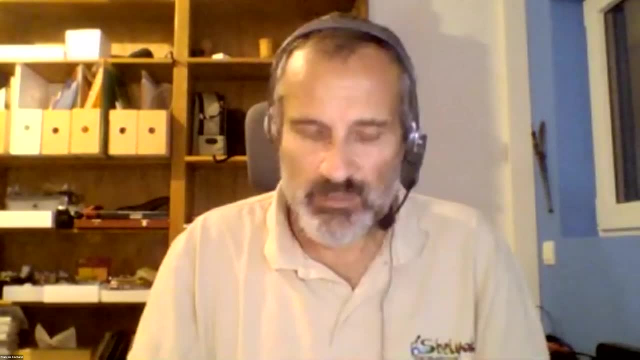 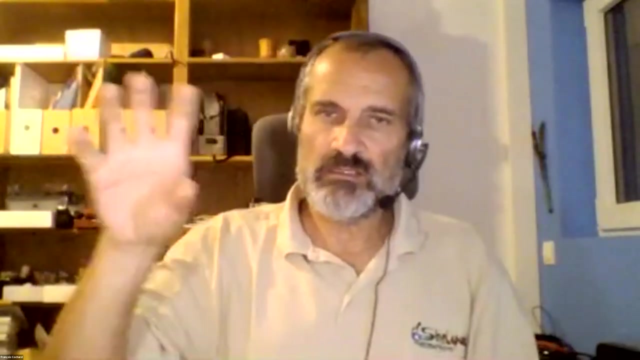 It is infinite. we will never see the end of this story, and so this is a wonderful new field of game for these guys. So, really, I like to say that you have people coming from science, you have people coming from techniques, from the instrument, and you have people coming from the observations. 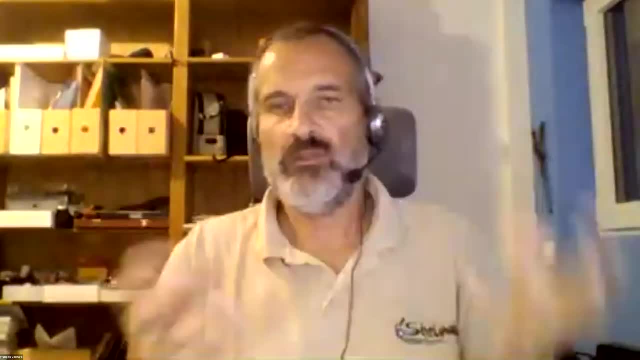 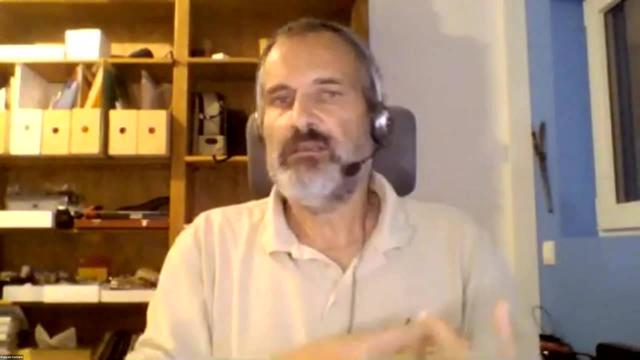 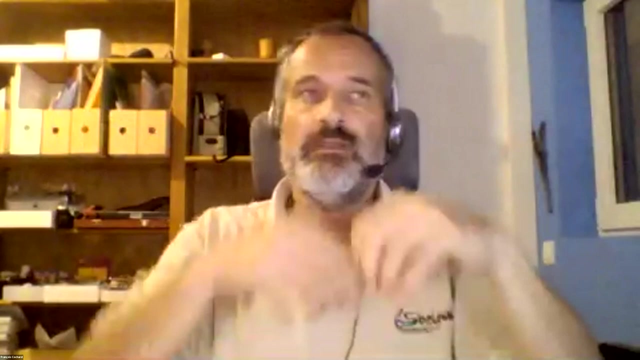 And when doing astronomy, in fact, we need the three of them, And in astrophysics and in science, I like to say that any discovery is made either thanks to a new science discovery, scientific discovery, a new model, for instance- or it comes from a new instrument. 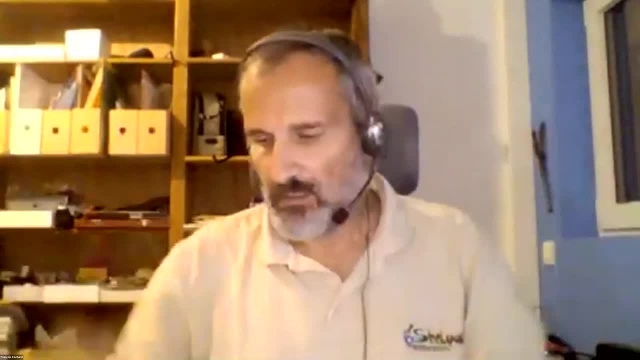 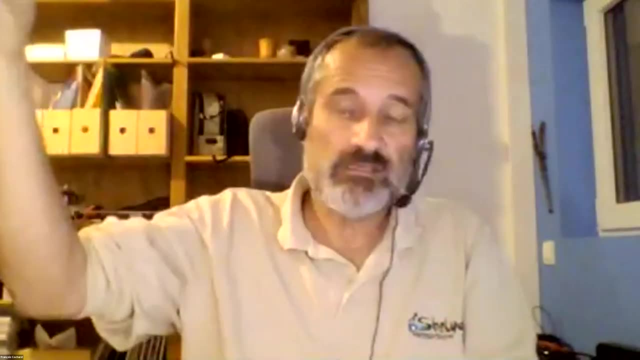 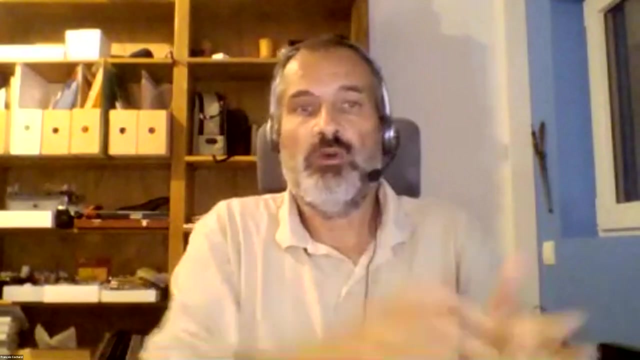 like the fiber or the CCD cameras or adaptive optics or things like that, or it comes from the observers, because you have an event that has been discovered, like a nova in the sky in early August, or somebody who did observe the same star during 20 years and after that. he knows the periods, the many. 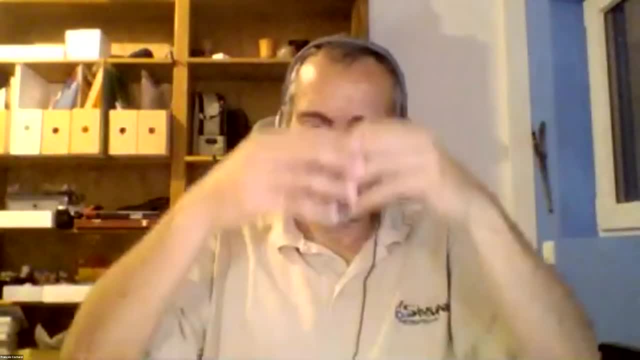 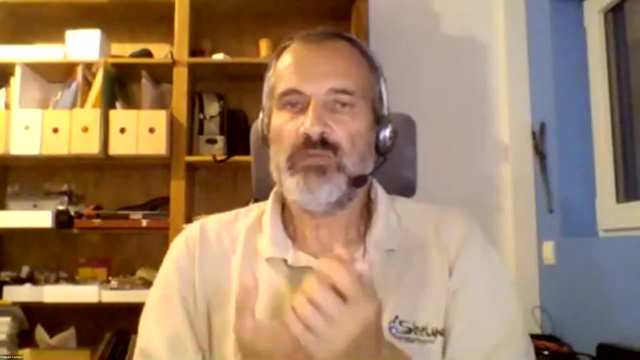 different periods and so on. So it's a very interesting field. It's a very interesting field. So this is the astrophysics is a permanent discussion between these three kind of people. And when we do spectroscopy, whatever, wherever we come from, we have to manage a little bit. 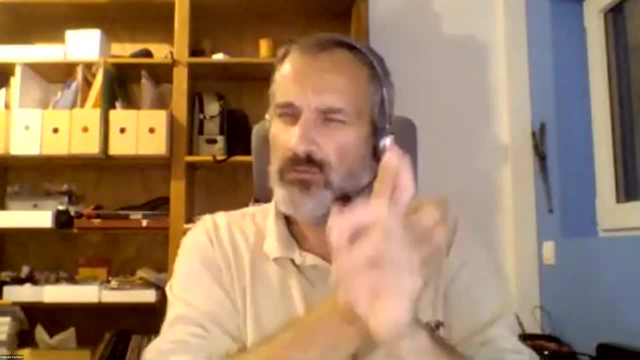 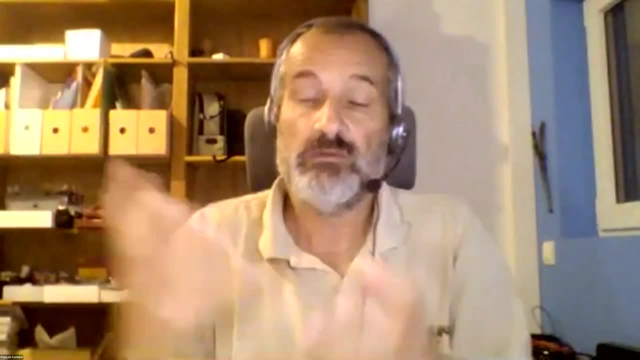 all these fields. We have to be in the field to do observations, We have to understand what kind of science we can do and what means these observations, And we also have to understand how works the instrument. So this is why spectroscopy is so wonderful activity. 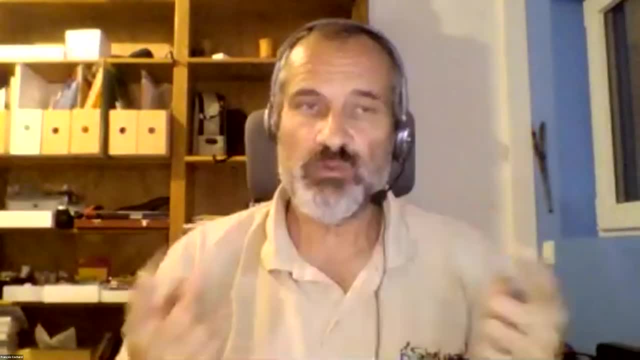 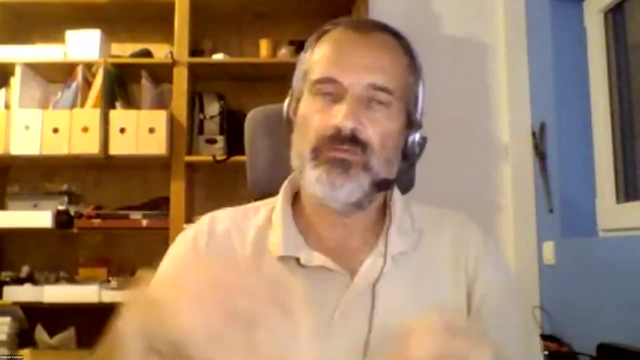 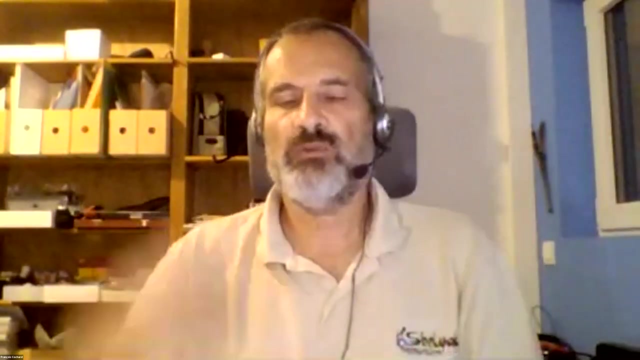 Because it requires to make things And I promise you that when you do that, you are really better understand the challenges of all the most advanced research in the world today And we better understand and we can discuss with all the professionals that are working. 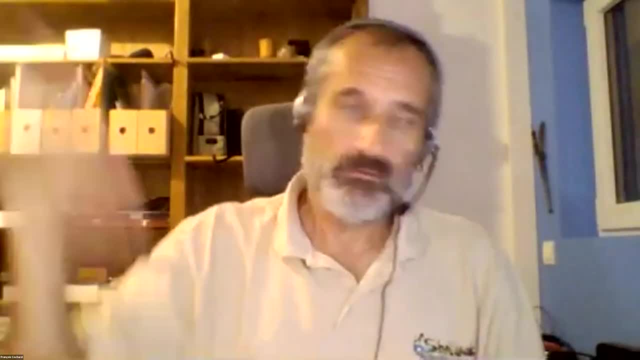 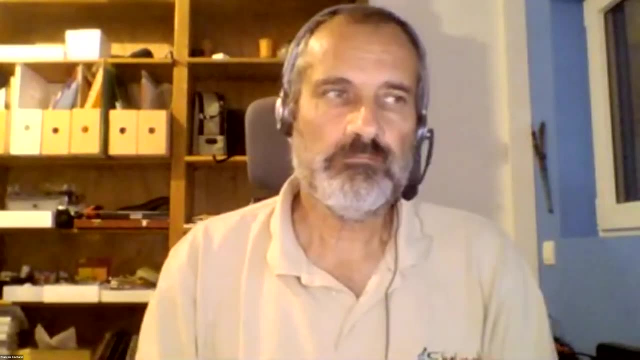 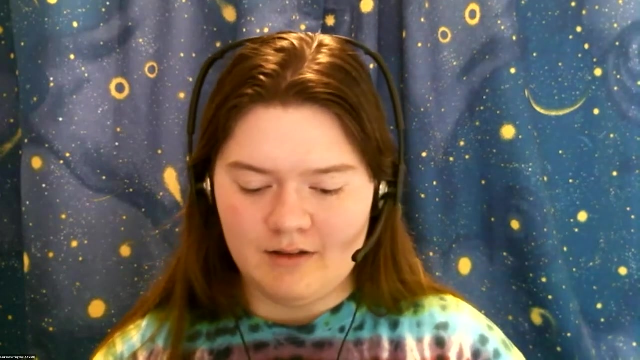 on trying to understand if there is some life elsewhere, or the multi-universe, or things like that. Thank you, Francois, That's very well said. Okay, That's it for our Q&A. I'm going to go ahead and start sharing my screen here. 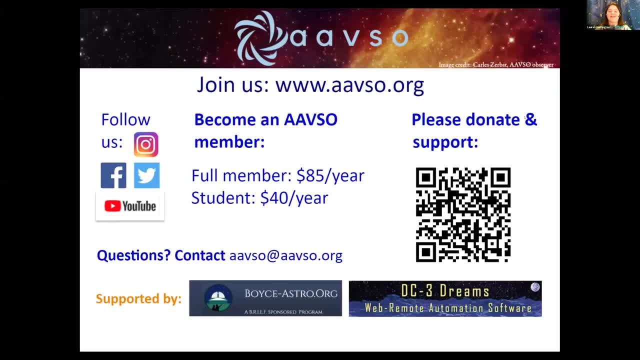 All right, There we go. So time for the closing announcements. First and most importantly, I want to give a huge thank you to you, Francois, for sharing your time and knowledge with us today. This was really excellent, And I've seen that we've had a whole flood of thank yous coming in through both our Q&A. 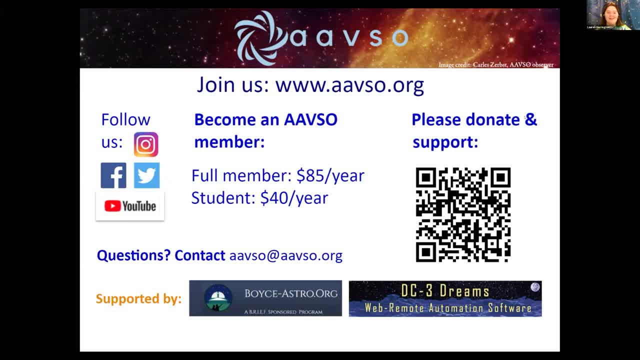 And I'm so happy to have you on the Q&A and chat because people are really happy. after all this wonderful instruction And also before I close the webinar, I would like to thank again our sponsors, DC3 Dreams and VoiceAstro. DC3 Dreams provides high-end observatory automation and web-based multi-user remote imaging. 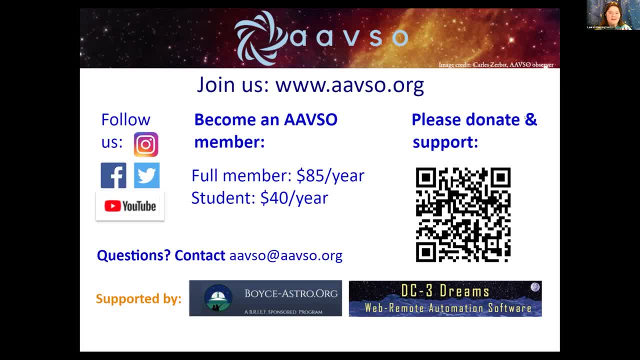 The AAVSO NET observatories use DC3 Dreams, ACP Expert for the Bright Star monitors and other programs. The AAVSO Photometric All-Sky Survey Project, also known as APAS, has used ACP Expert's AI scheduler to automatically acquire over 500,000 star fields hands-off at a rate. 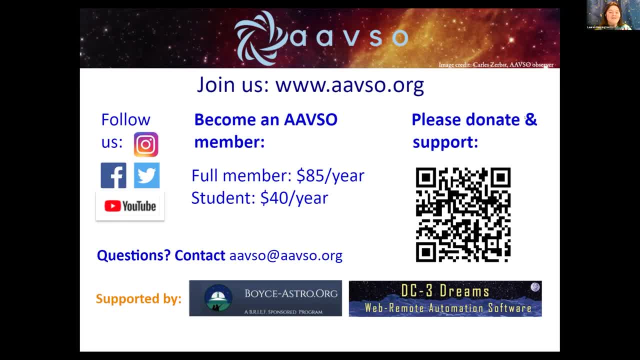 of 1,000 square degrees per night. This has resulted in photometry for over 128 million objects in about 99% of the sky. The Boyce Research Initiative and Education Foundation provides online astronomy education, observatory resources and research experiences to students, student teams and schools in order to learn how to.